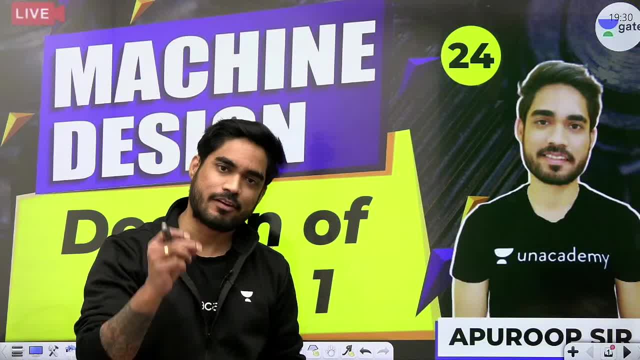 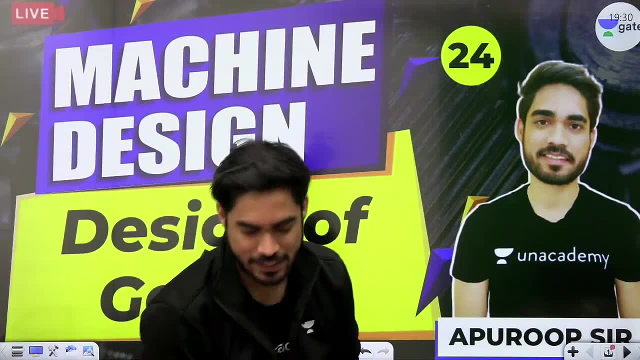 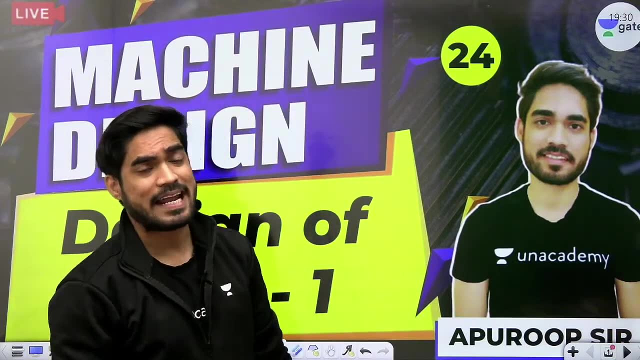 of machine design: design of gears. After this, there will be only one chapter left, that is, design of springs. So we are going to complete the syllabus of machine design by 30th of December, as promised, and on 31st of December there will be an 8 hours marathon session which will complete. 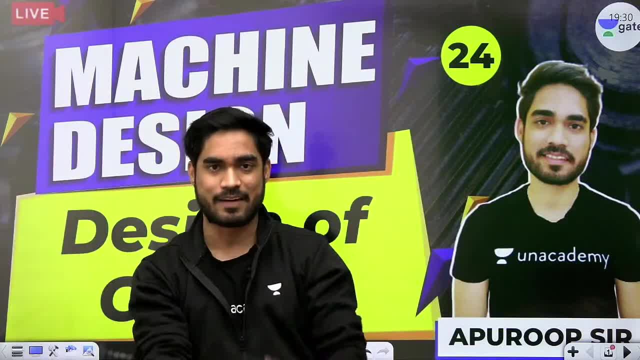 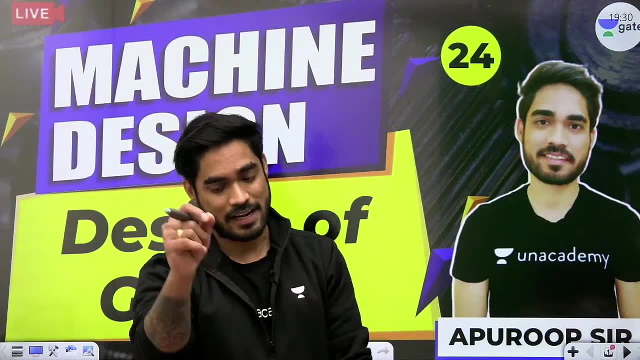 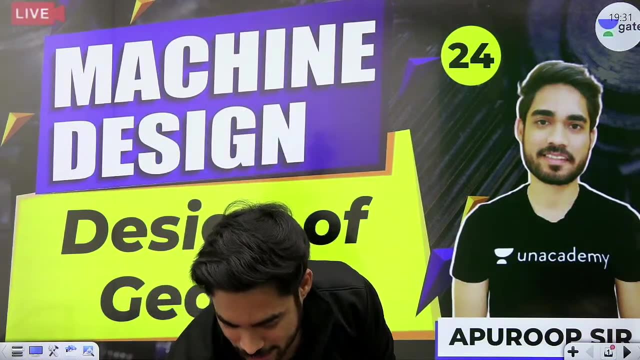 the entire machine design, which will revise the entire machine design in one single class. In one single class, we are going to revise the machine design on 31st of December. Good evening, Divyanshu, Welcome everyone. Please hit the like button and please share Everyone. please share the link with your. 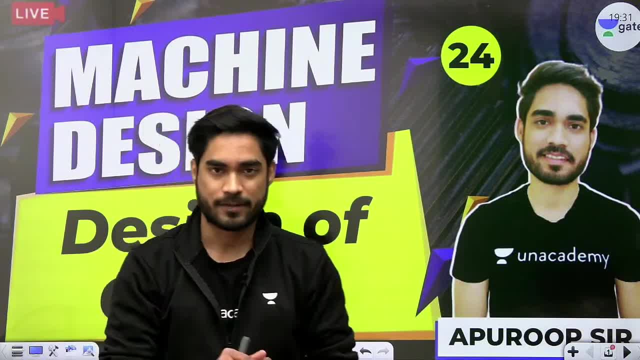 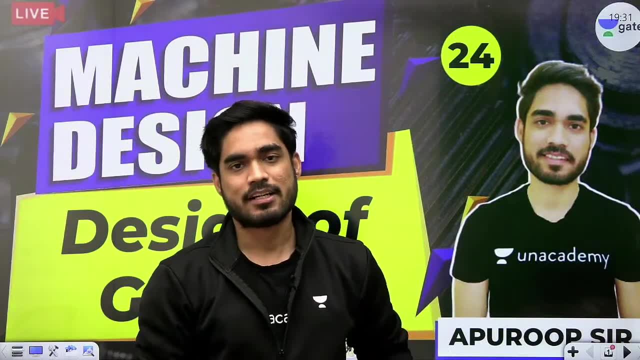 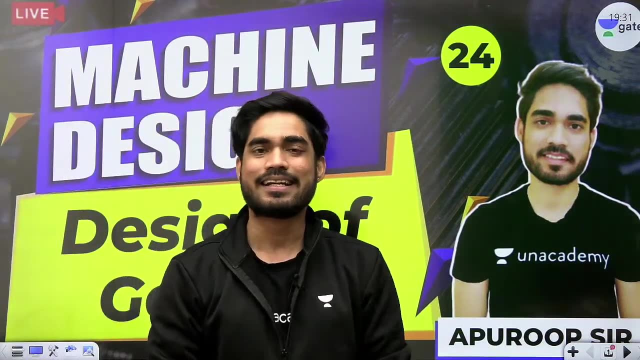 friends, Please share the link with all your groups. So this is design of gears, part 1.. Today we are going to start. what are the different types of gears, what are the different terminology of gears and how the gears are designed? What is the design equation behind the design of gears? 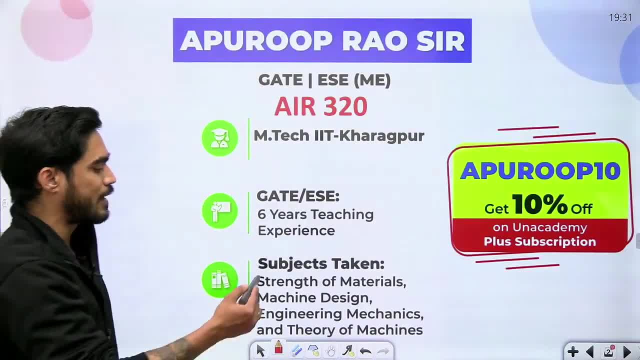 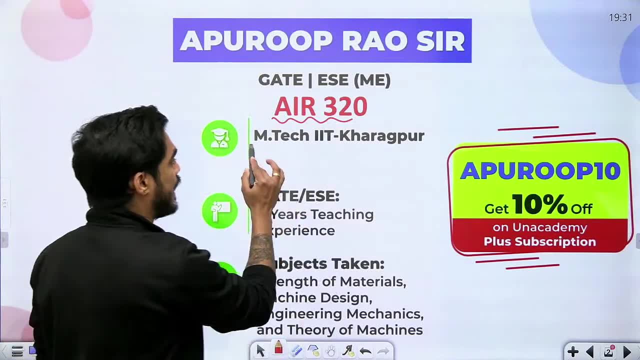 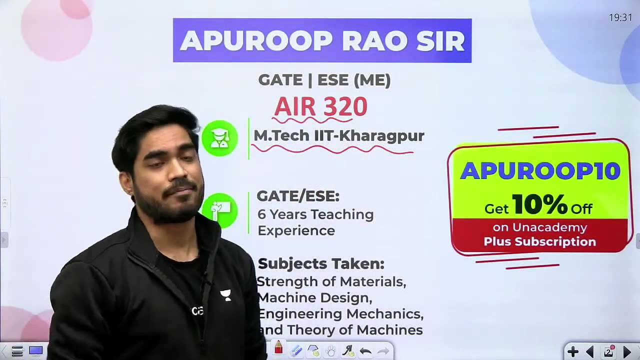 So if you are watching me for the first time, let me quickly introduce myself. My name is Aparoop Rao, All India rank 320 in gate mechanical. I have done my MTech from IIT Kharagpur and my specialization was mechanical systems design. Then I was recruited by Mahindra and Mahindra 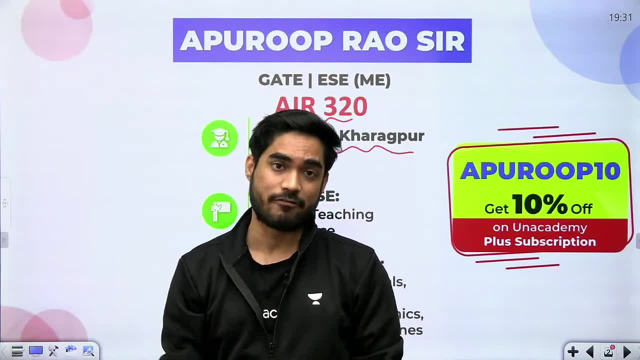 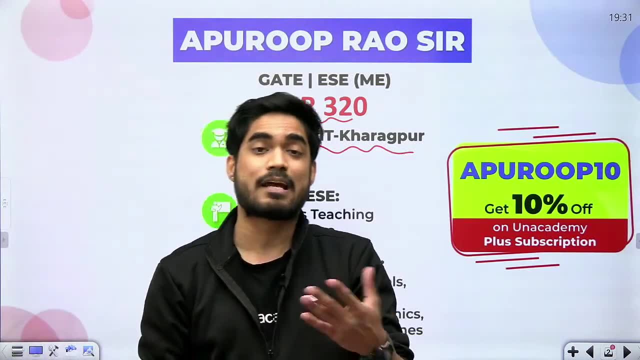 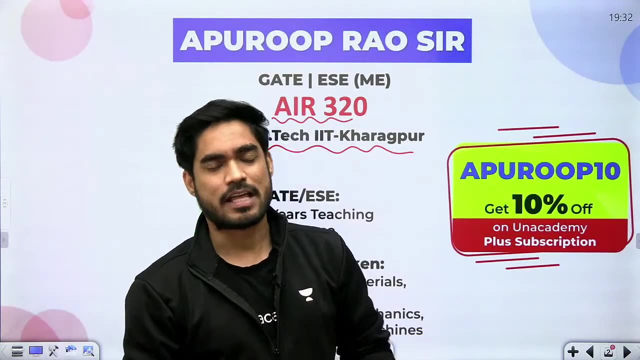 in my final year and I was placed at Mahindra Research Valley, where the cars and tractors of Mahindra are designed. So I worked there in the field of design for two years as deputy manager, But then I decided that I don't want to work in like this, I wanted to teach. So then I 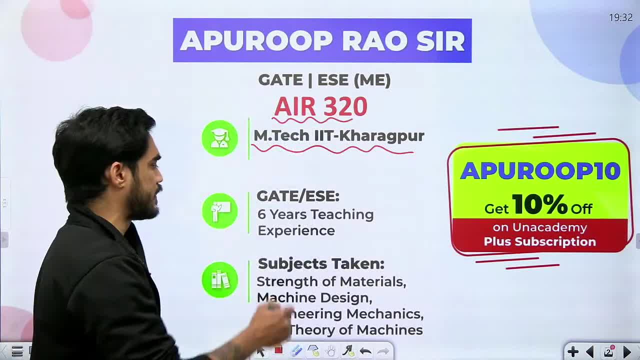 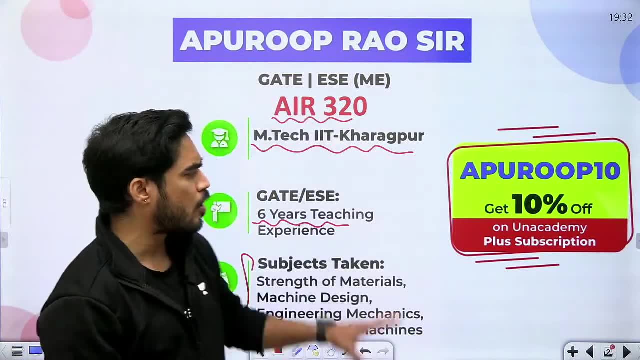 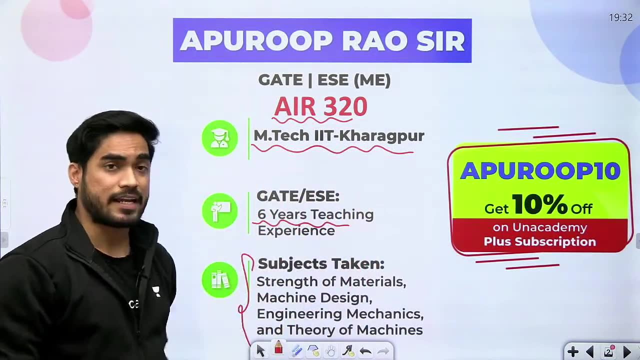 quit my job and I started teaching. So I have been teaching for more than six years now and I teach subjects related to design- SOM, MD, EM and TOM- And I have taught all of these subjects. You can watch all my lectures of strength of materials, machine design, engineering, mechanics and now. 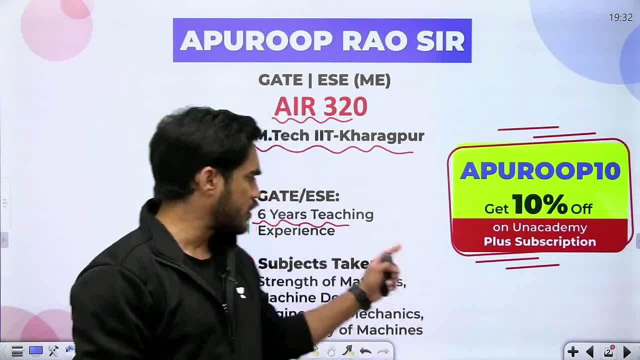 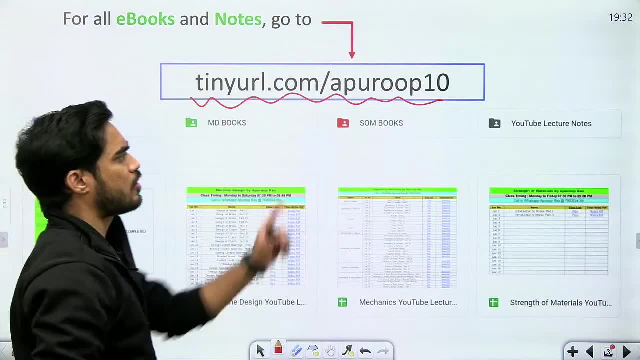 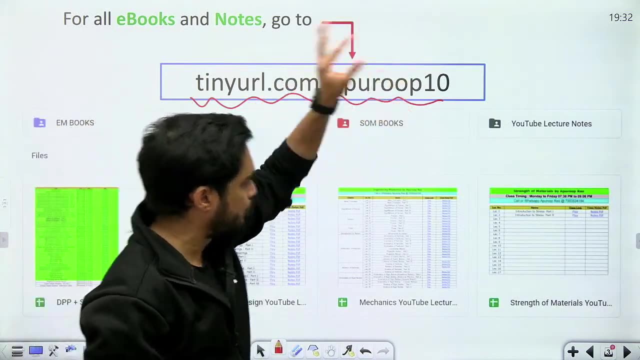 even theory of machines. What do you need to do to watch my lectures? All you need to do is access this link. Go to this link: tinyurlcom slash Aparoop 10.. Open your web browser and type tinyurlcom slash Aparoop 10.. Enter and you will open this page where you 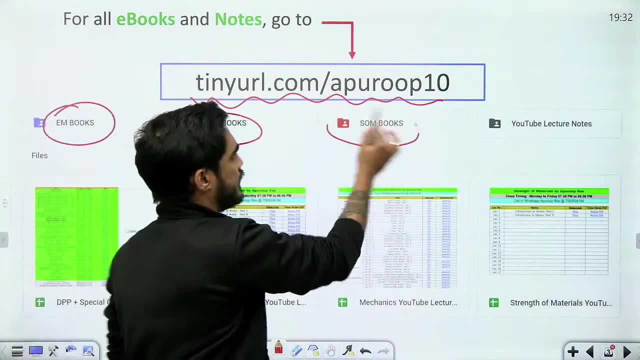 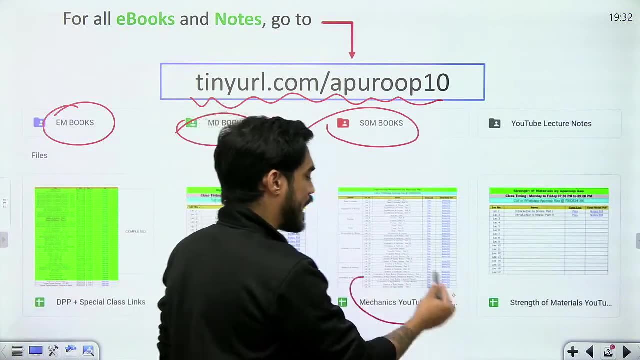 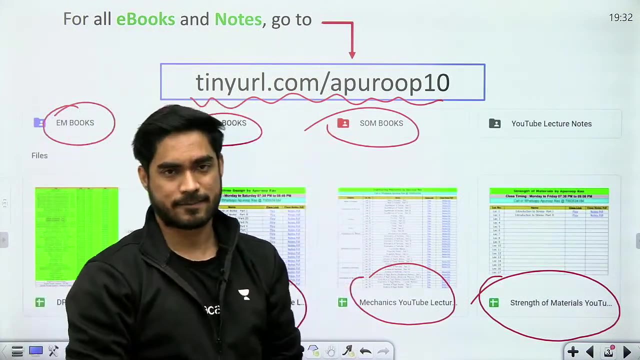 will find the e-books of all different subjects of design and you will find these excel sheets. What are these excel sheets? These excel sheets are like digital books Which contain the links of all my classes in one place. If you open the excel sheet of any one, 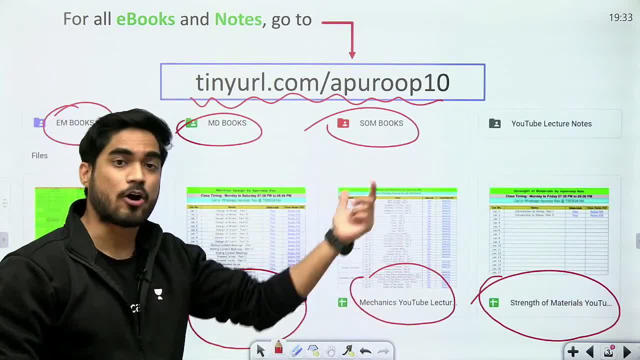 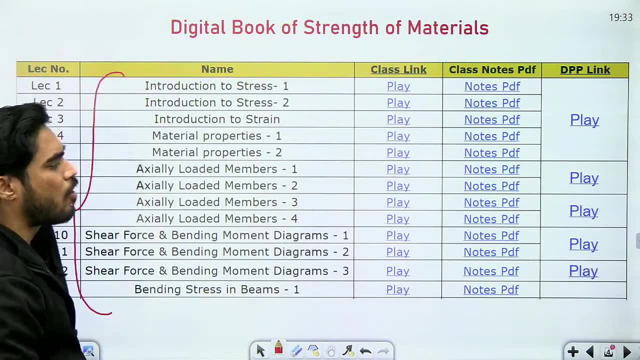 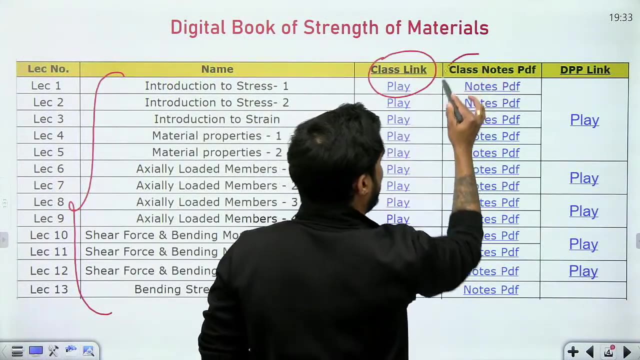 subject: There is an excel sheet of EM, SOM, MD, TOM. If you open the excel sheet, let's say of strength of material, You will find that I have placed all lectures of strength of material in this excel sheet. You will find the YouTube class link. You will find the lecture PDF, Everything. 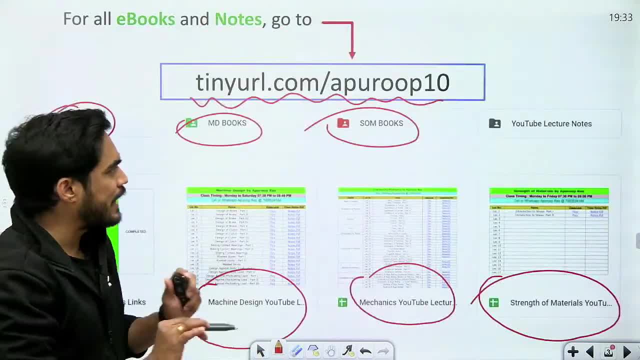 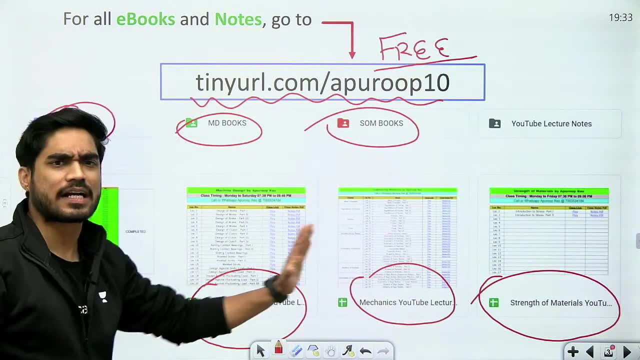 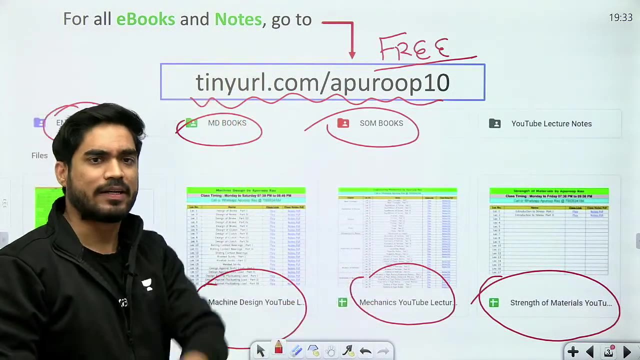 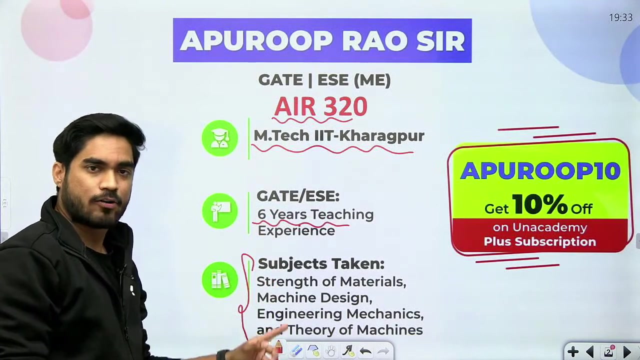 uploaded in one excel sheet And the entire content in this excel sheets are completely free. The entire content is free of cost. You can access all the lectures, You can download all the PDFs. Everything is entirely free. So if you want to prepare the subjects of design, then all you need to do is go to this site. 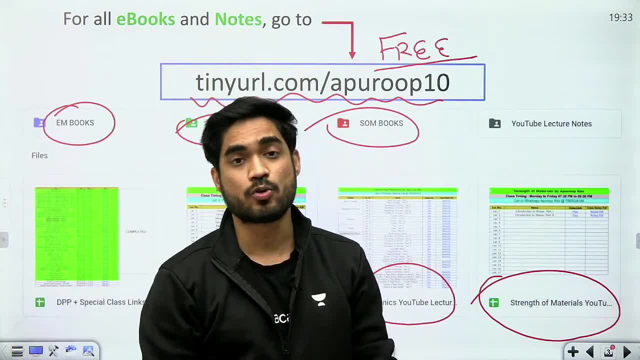 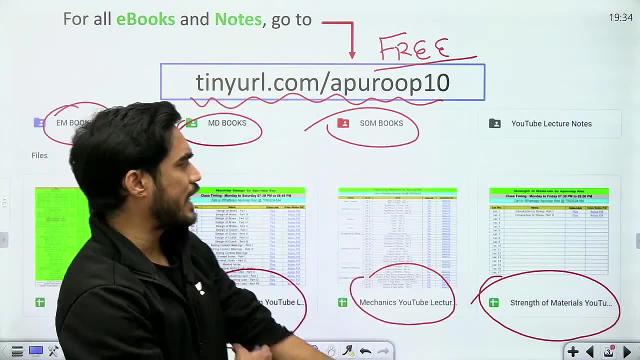 tinyurlcom. slash Aparoop. 10.. Tell your friends, tell your juniors, tell your seniors, everyone Who is preparing for any competitive exam related to mechanical engineering, that he can watch the entire lecture series of SOM, EM and BM in this. 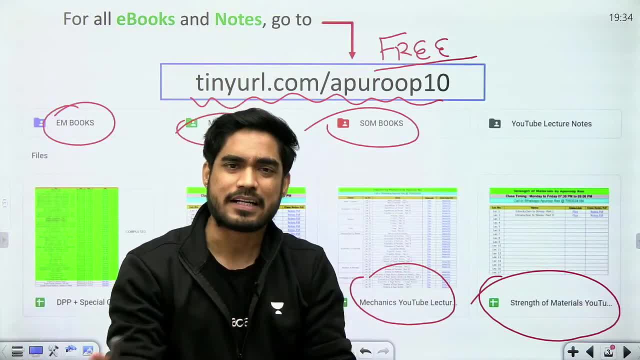 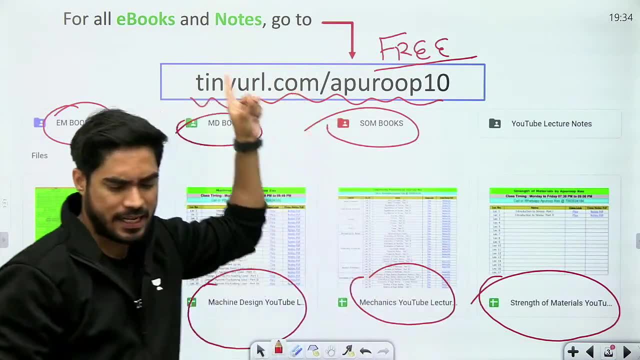 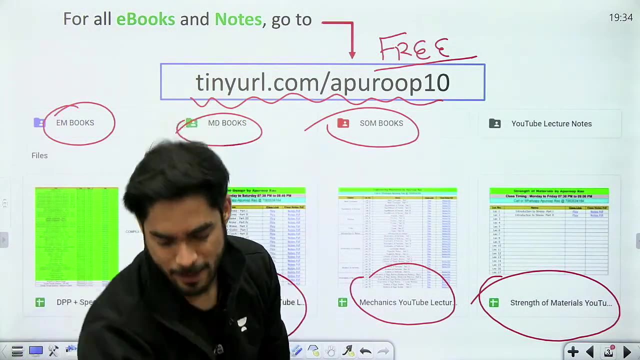 So, son, the entire content is free. If you are self-preparation, then you don't even need to go anywhere. you just have to go one place and access this one site. Good evening Akshay. Good evening Deuvooshish, Good evening Parth. Welcome, everyone, Welcome. 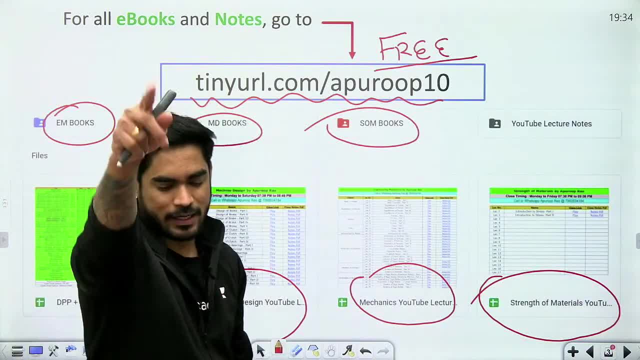 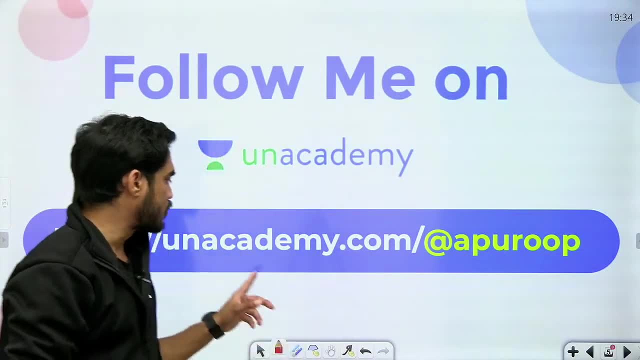 Please hit the like button. Please hit the like button. Please hit the like button. hit the like button and please share the link. share the link. share the link. And if you want to access my Unacademy profile, just go to unacademycom. slash at the rate approved You. 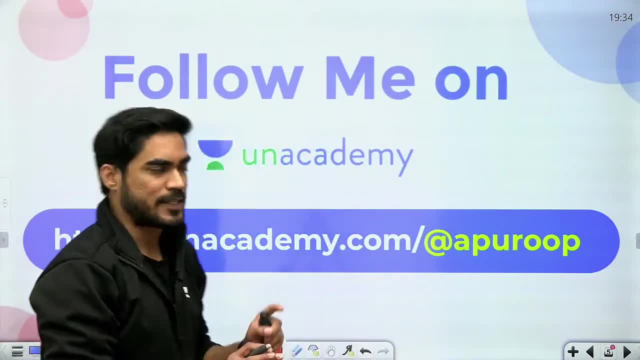 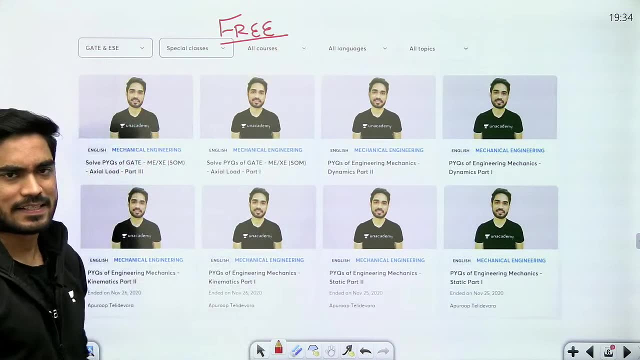 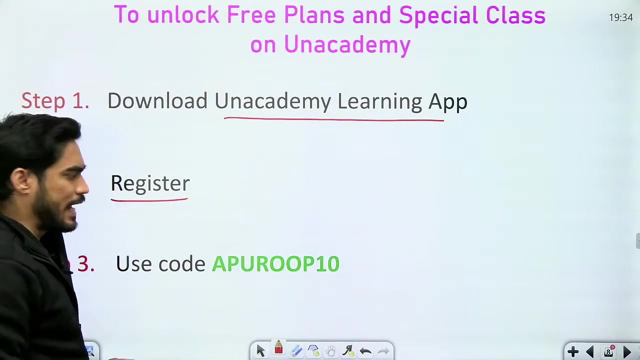 will find my entire profile there. You can watch all my special classes in one place. Special classes are completely free. If you want to see the special classes, then all you need to do is just download the Unacademy learning app, register yourself and use the code APPROVED10.. 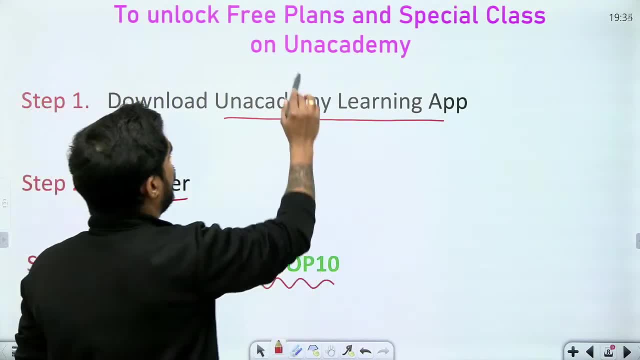 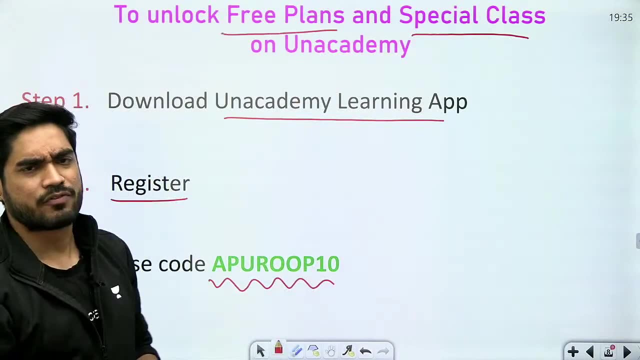 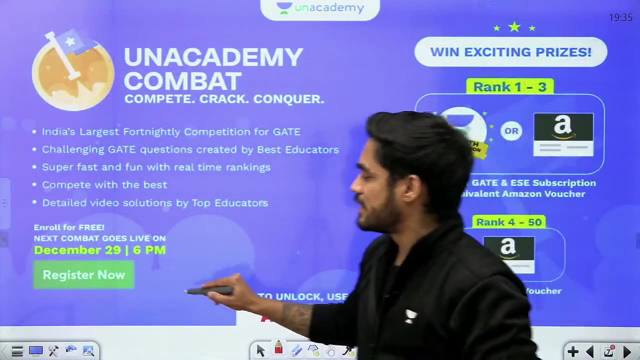 By using the code APPROVED10,. you will open all the special classes, You will unlock all the special classes and you will unlock all the other free plans. What are these free plans? So it is very important news for you that there is another Unacademy combat this Sunday. 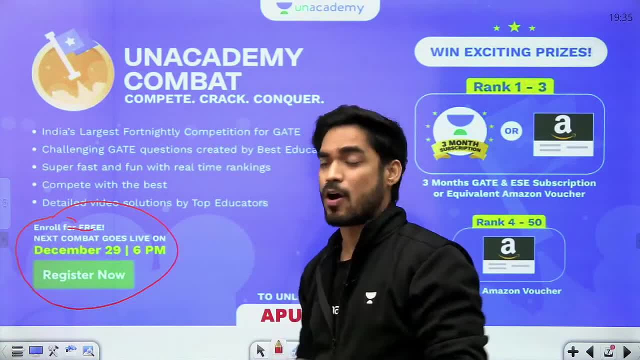 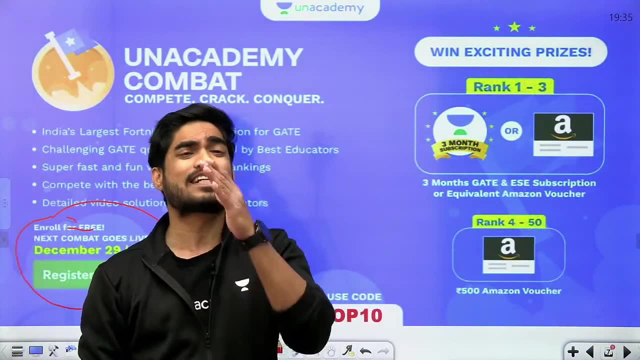 sorry. on 29th of December There is another Unacademy combat. There is another Unacademy combat on 29th of December. There is another Unacademy combat on 29th of December at 6 pm. What is Unacademy combat? Unacademy combat is the biggest quiz. 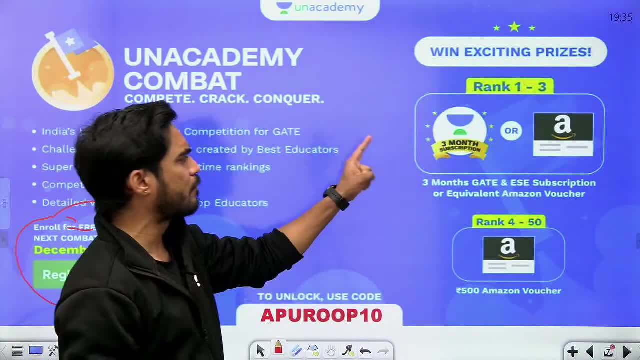 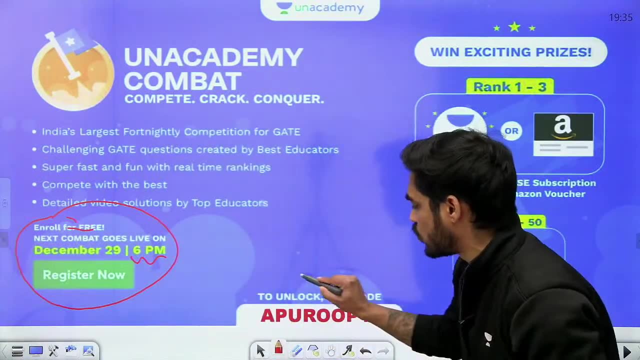 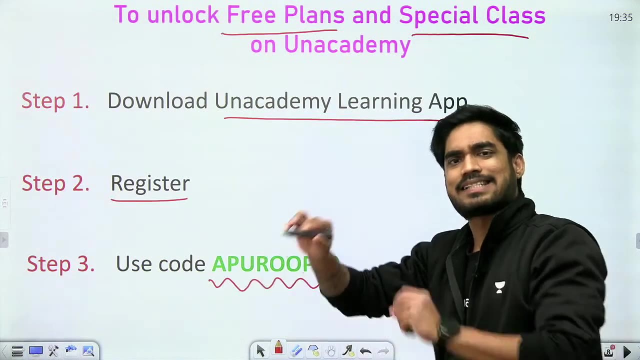 competition based on GATE, where you can win exciting prizes. So beta. the enrollment is completely free of cost. All you need to do is use this code APPROVED10 in order to unlock Unacademy combat. So beta, Unacademy combat, special classes- all the free plans of Unacademy. 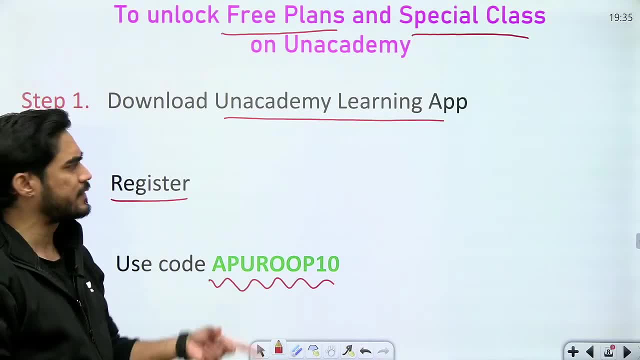 can be unlocked by using this code: APPROVED10.. All you need to do is use this code, APPROVED10, and all you need is go to Unacademy learning app. You can download it from Play Store, You can download it from Apple Store and then register yourself and when you will try to access Unacademy. 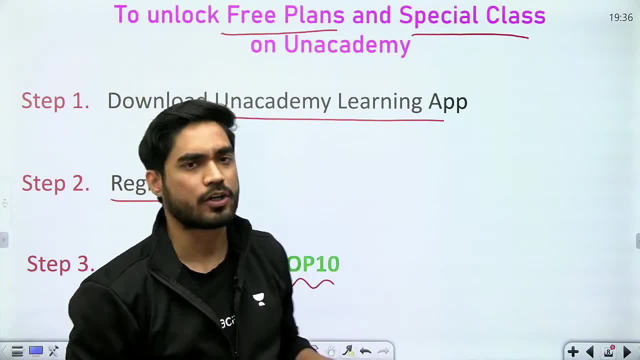 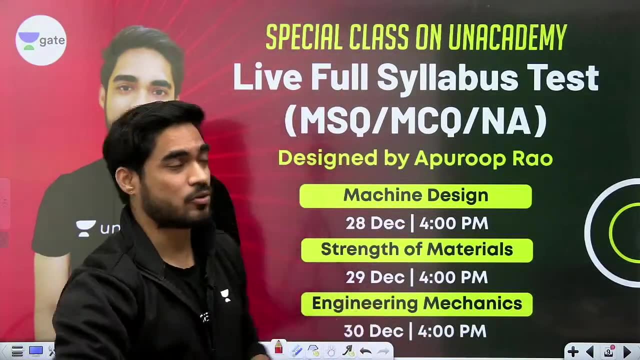 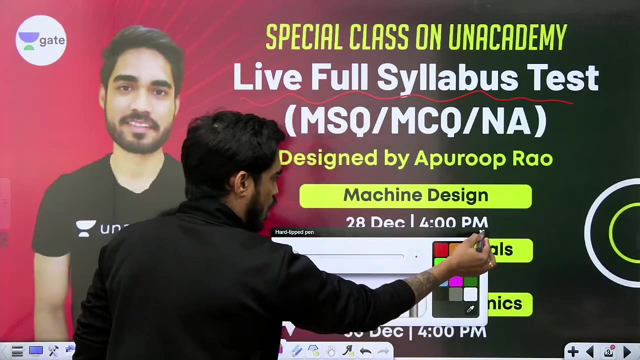 combat or any special class. they will ask you this code to unlock the special class. Then beta, use this code. okay, And I have started to take live full syllabus test of all the subjects of design beta. Today there was a test of machine design. 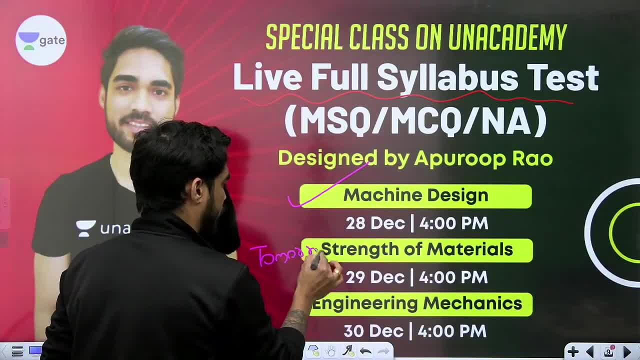 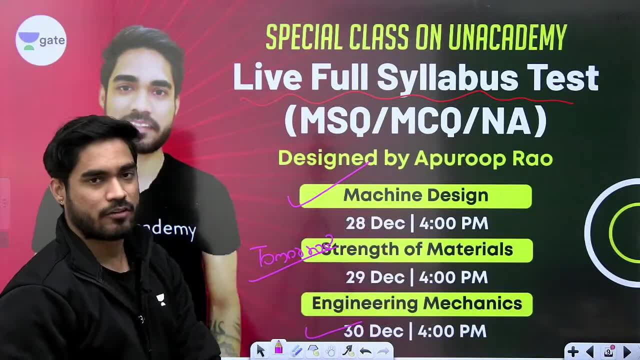 Tomorrow. tomorrow there will be a test of strength of material and then day after tomorrow there will be a test of engineering mechanics. okay, So all the subjects of design. if you want to see where you stand among the other students, then beta you need to appear for. 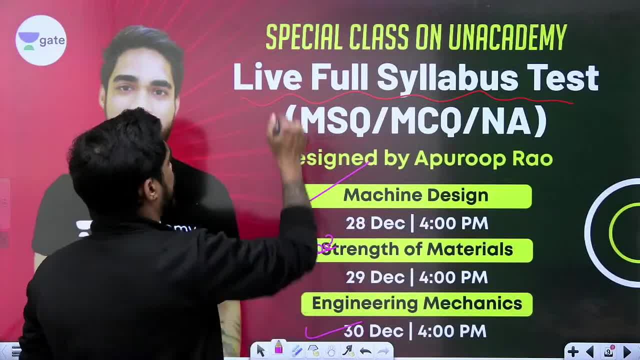 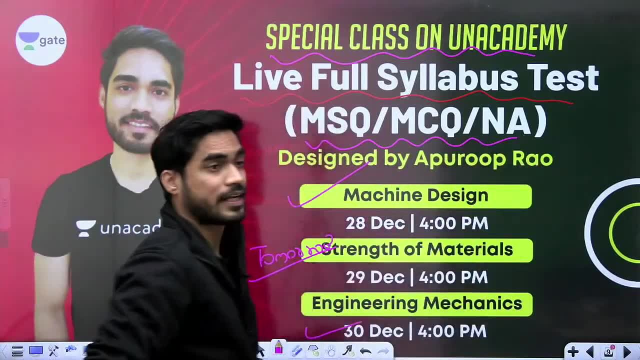 this test? okay, These tests are also completely free. They are in special classes. They are in special classes and the test will include MSQ questions, MCQ questions, numerical answer type questions. okay, So beta, if you want to see the test of engineering mechanics, then you need to. 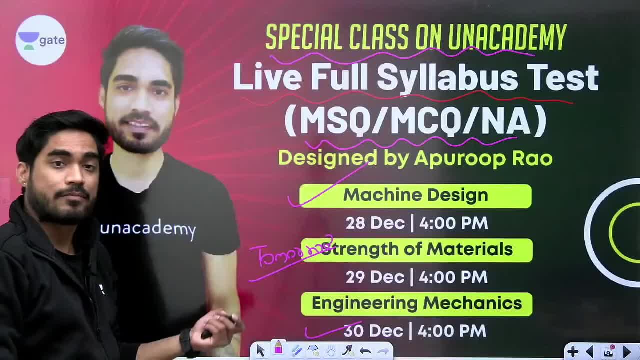 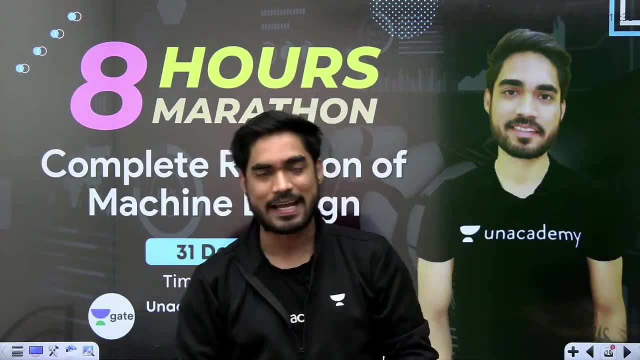 access these tests. All you need to do is download the Unacademy learning app and use approve 10. And beta. another very important news: 30th of December, machine design course will be completed and on 31st of December we will have 8 hours marathon session where we will completely 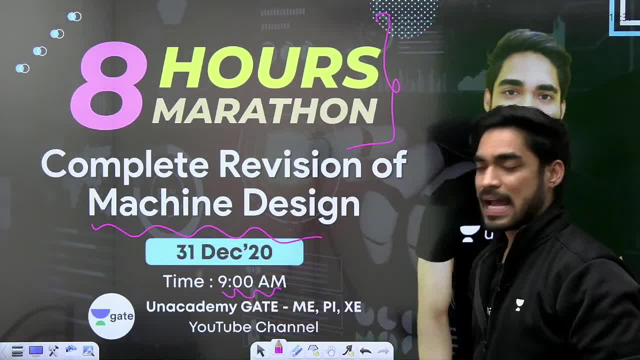 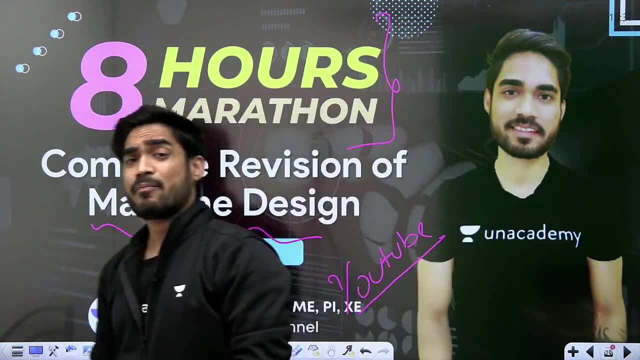 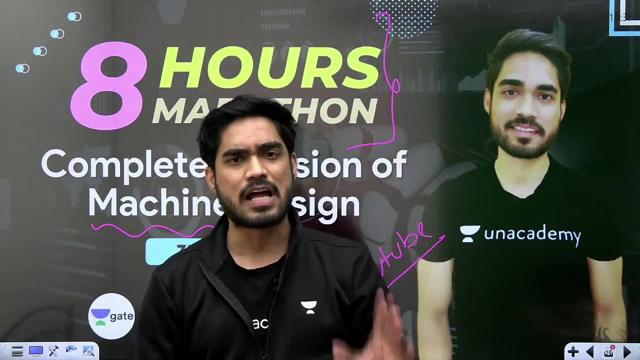 revise the entire machine design. 9 am will be the timing and this session will be on this YouTube channel, only This will be on this YouTube channel, my brother. We will revise the whole machine design 8 hours. All important concepts, all important formula, all examples, So beta, everything will. 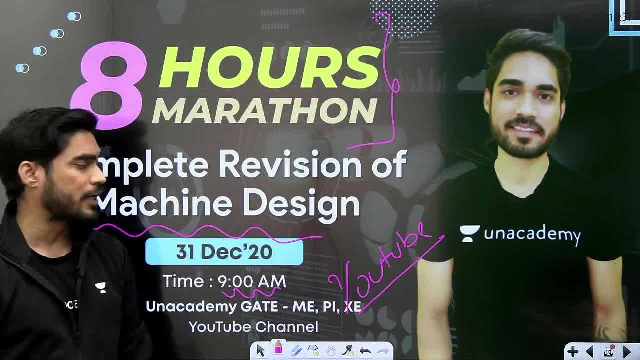 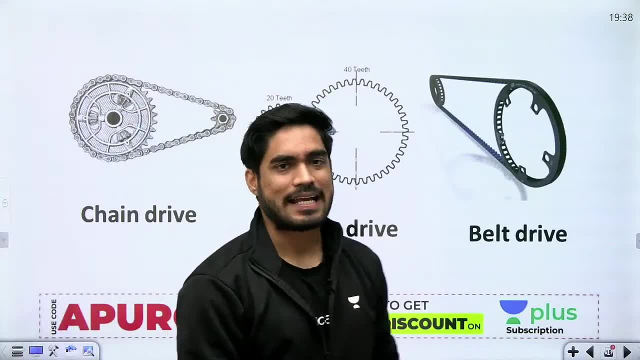 be completed in 8 hours. okay, So don't forget to tune in to this YouTube channel at 9 am on 31st of December. Gear- design of gear. okay, So what exactly is gear? So beta gear is a power transfer. 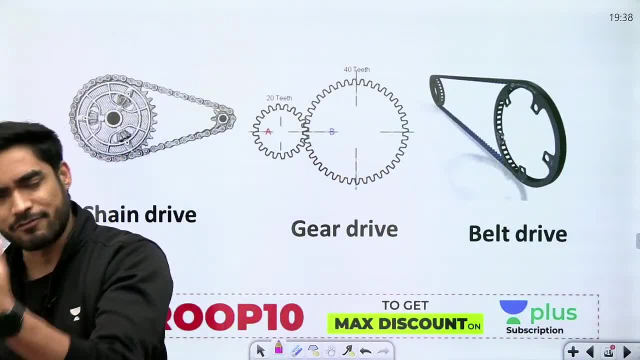 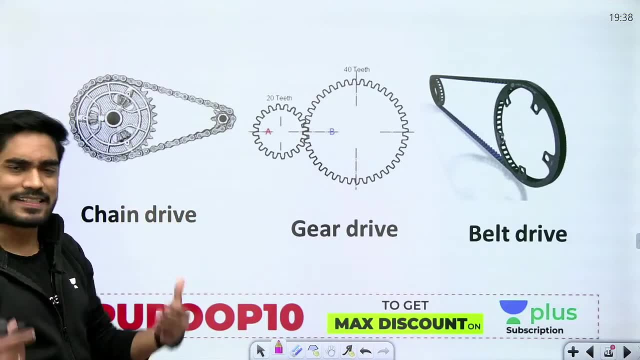 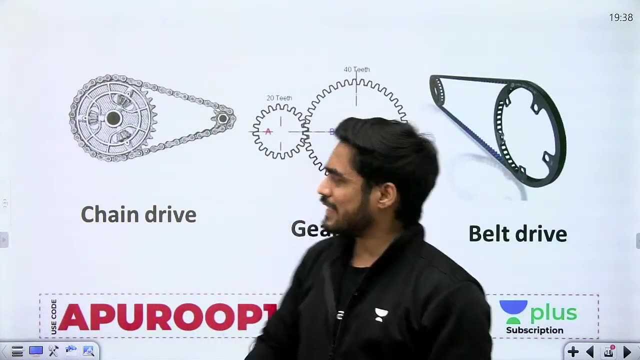 device. Gear is a device which we use to transfer power from one shaft to another shaft. okay, Now there are other devices also. Just like gear drive, there are other devices which use to transfer power from one shaft to another shaft. There is a belt drive, then there is chain drive. okay, So all these are used to 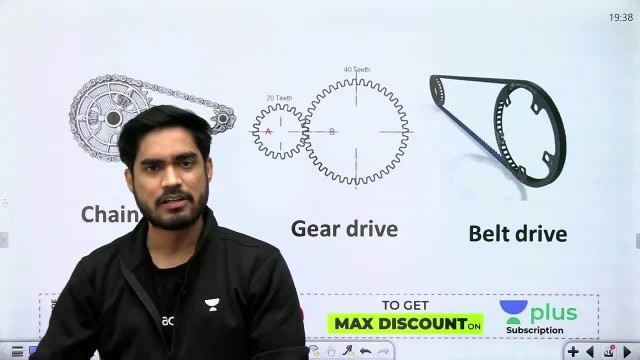 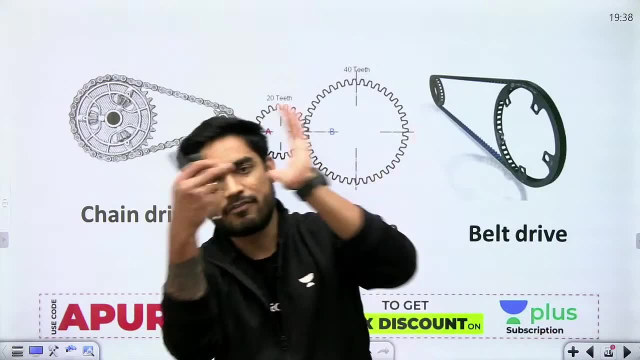 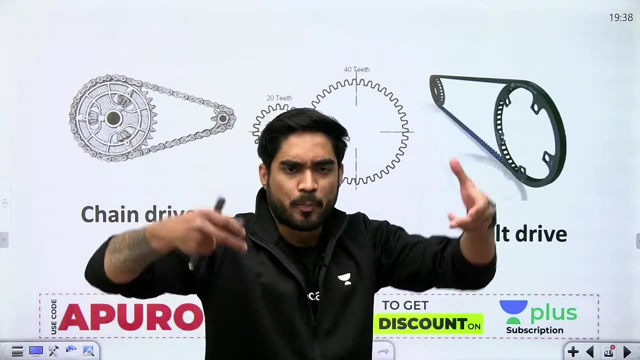 transfer power, or you should say torque, from one shaft to another shaft. okay, There is an input shaft, there is an output shaft, So you will take power from input shaft and you will transfer that power to the output shaft. okay, So in case of belt drive, we simply put two pulleys on. 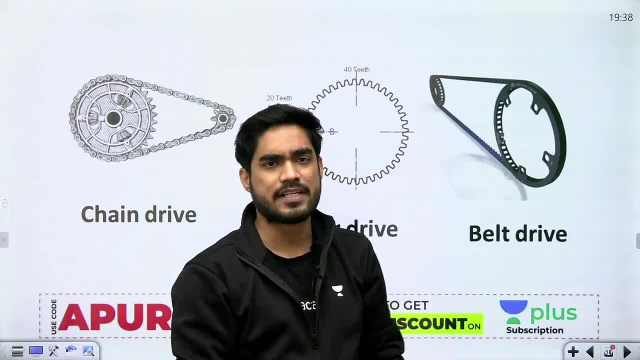 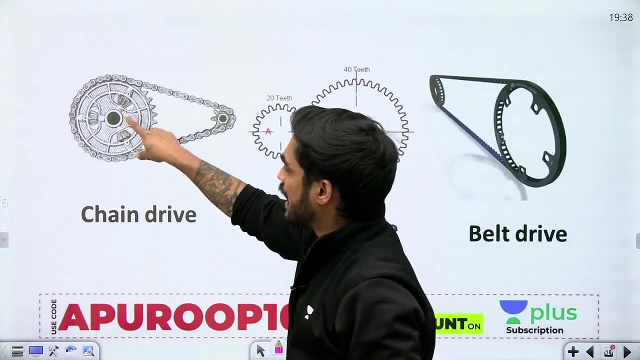 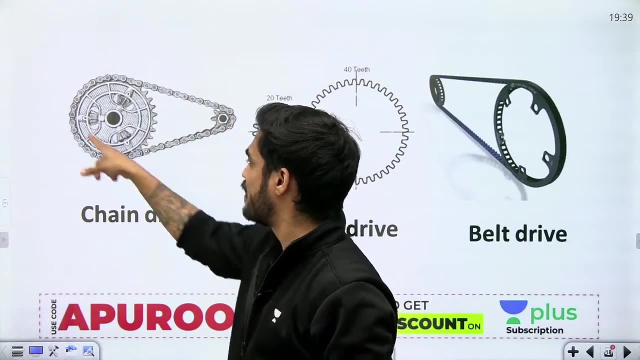 input and output shaft and then we connect those pulleys using a belt, flexible belt. okay, In case of chain drive, instead of belt we use this chain and sprocket. So instead of pulley there is a sprocket which has teeth, and instead of belt we have a chain, So there is a direct force transfer. 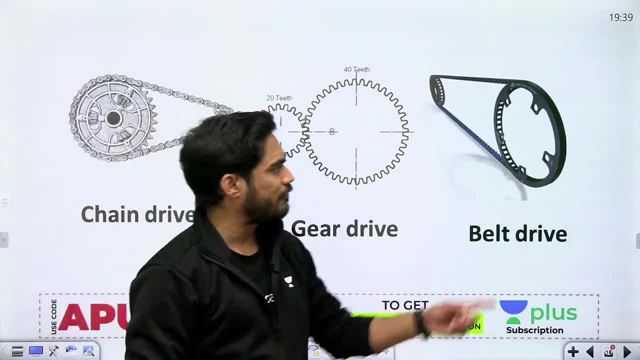 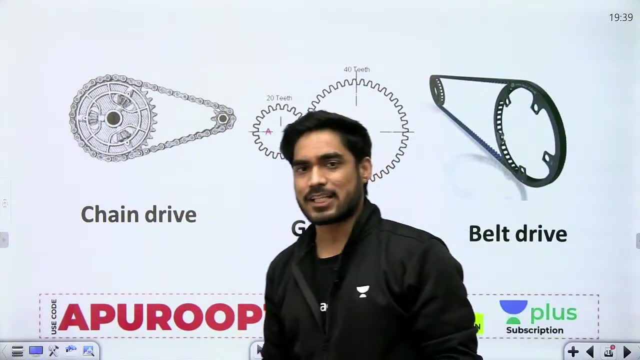 between the chain and the sprocket. In case of belt drive, the power transfer takes place due to friction, But in case of chain drive and gear drive, there is a direct force transfer between the chain and the sprocket. The power transfer takes place due to the direct force applied by this one. 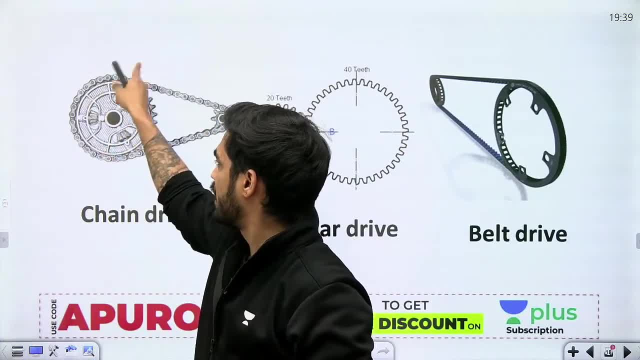 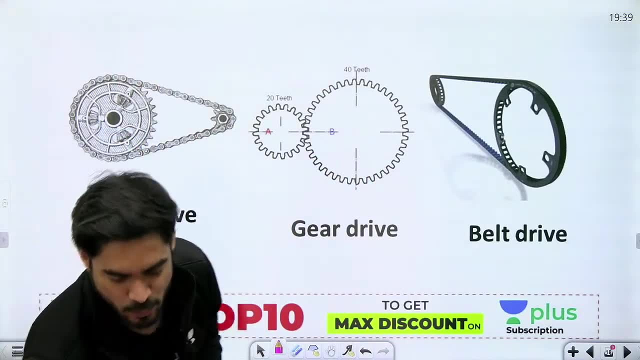 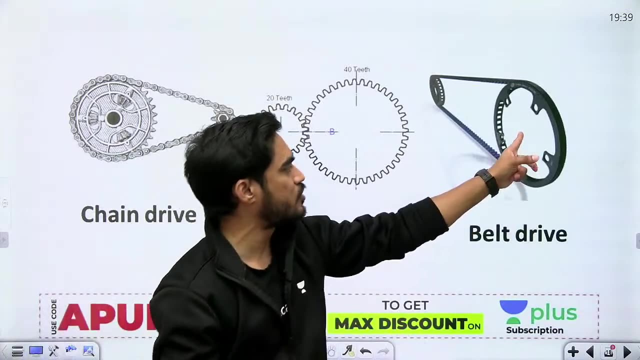 gear on another gear or applied by this sprocket on the chain or on chain on the sprocket. So the engagement is positive. The engagement is positive. It is like this: This is known as positive engagement. There is a direct force transfer- okay, But engagement is not positive. 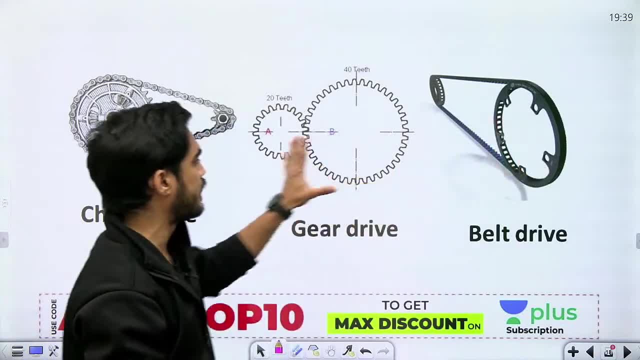 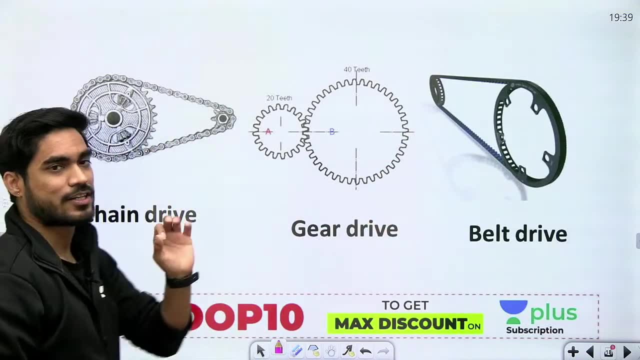 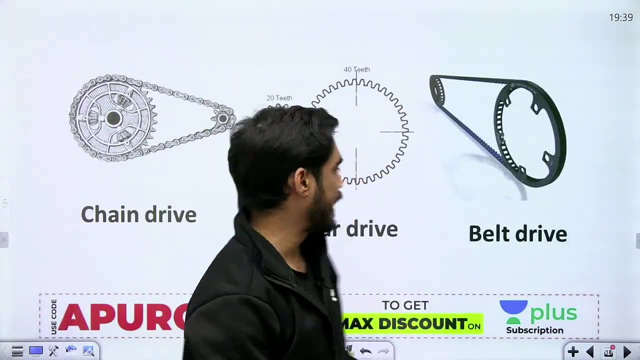 Here there is friction. So what is the difference between all these three drives? In case of belt drive, there is friction, there is slip, But in case of belt gear drive and chain drive, there is no slip. okay, In case of belt drive and chain drive, the velocity ratio is not constant, But in case of 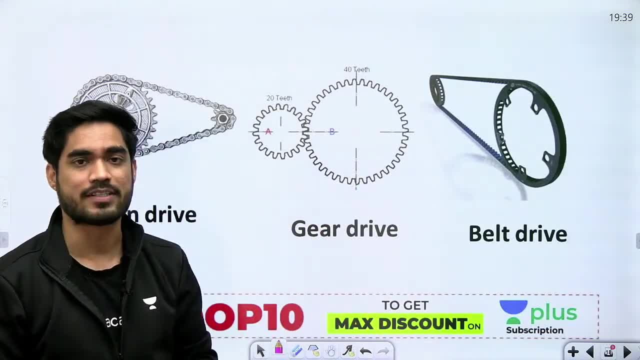 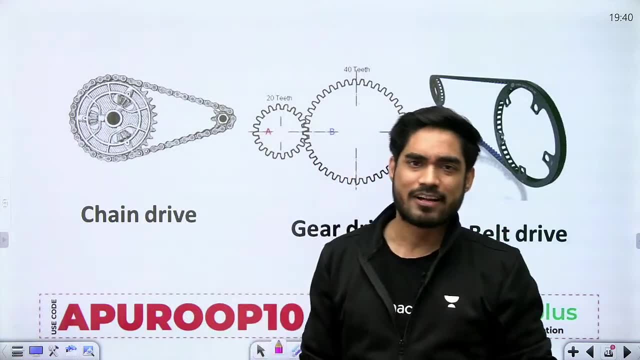 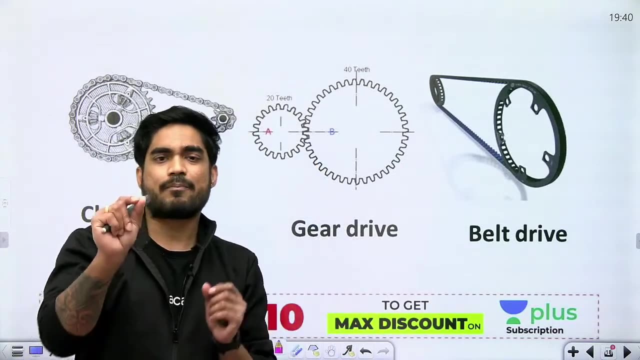 gear drive, the velocity ratio- input velocity by output velocity- is constant. So there are different differences between gear drive, belt drive and chain drive. According to your need, you will use one of these transmission devices. There are different advantages and disadvantages of all these drives. 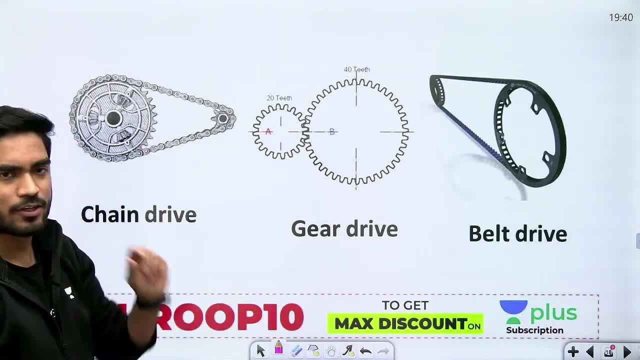 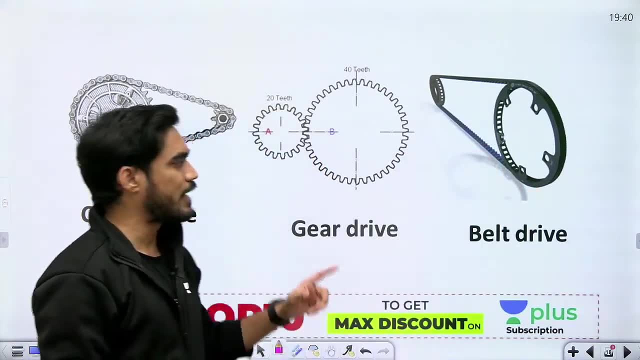 Where will belt drive and chain drive be useful? Belt drive and chain drives are used where the center distance is large. There is large center distance between one shaft and another shaft, Then we use belt drive and chain drive. But if the center distance is not too much, 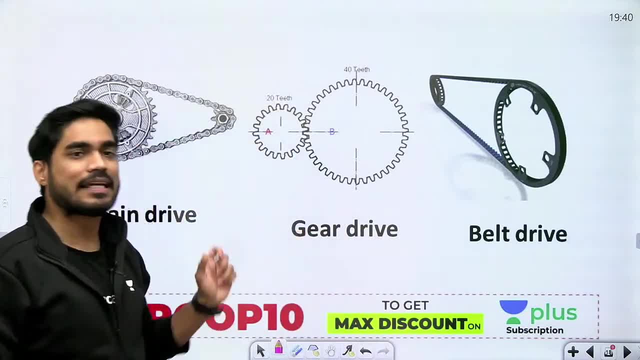 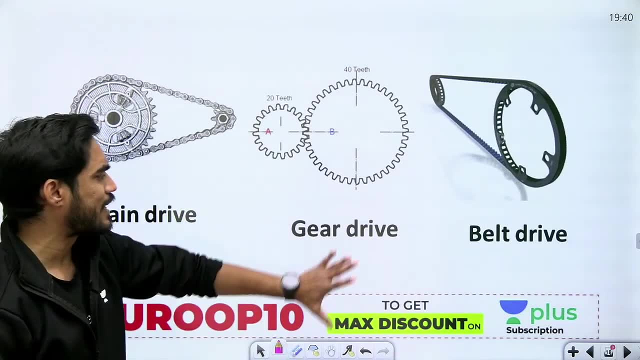 and you need a compact design, then you need gear drive, okay, So there are different advantages and disadvantages. You don't need to memorize them Here in this chapter. we need to discuss only gear drive. okay, Now, first of all, we will discuss: 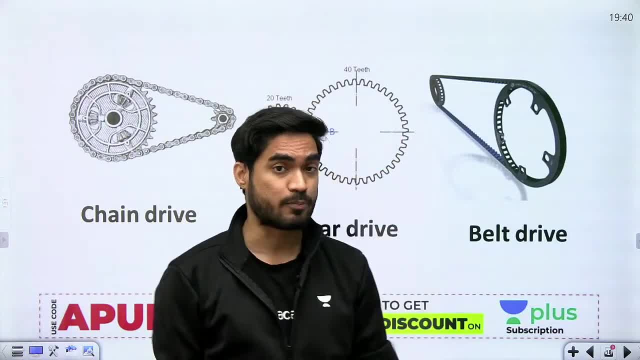 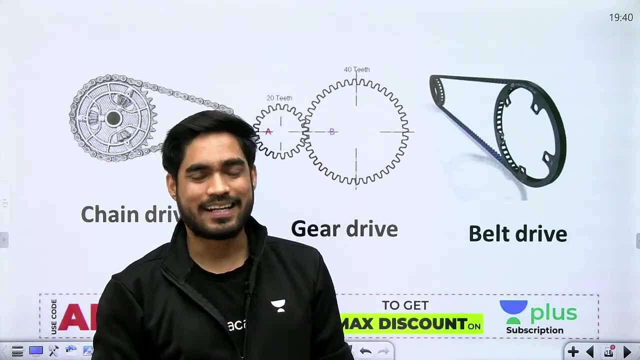 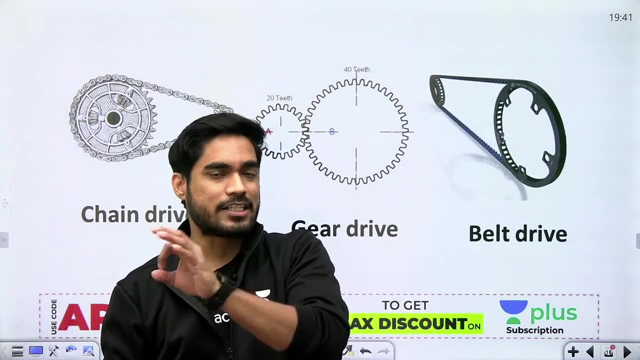 different types of gears because you might get theory questions based on them. okay, So every gear has some special characteristic based on which it is used for different application. So we will see one by one what is that special characteristic and in which application we will. 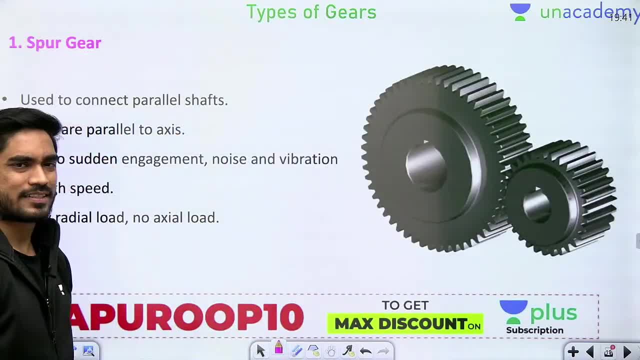 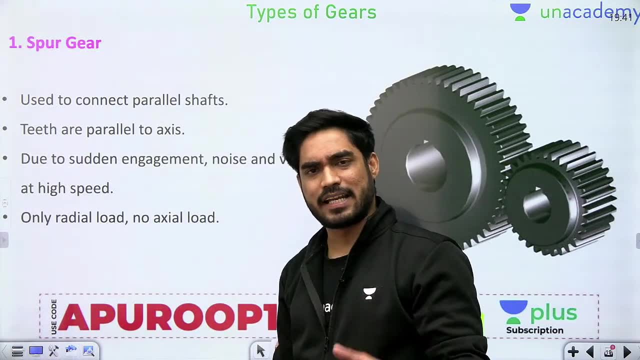 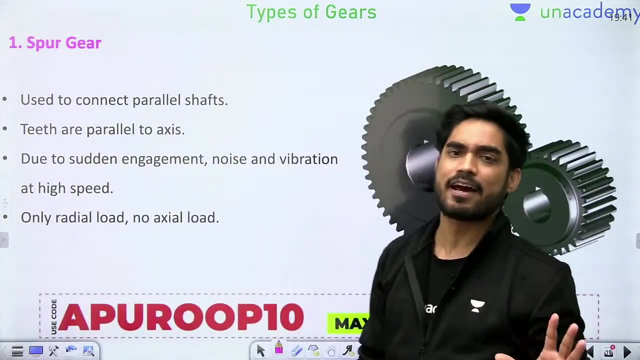 use that characteristic, okay. So first of all, the most widely used gear, which is known as spur gear. Mostly in every application, in every machine, you will use spur gear. only This is the most widely used gear. Why? Because the manufacturing of this gear is. 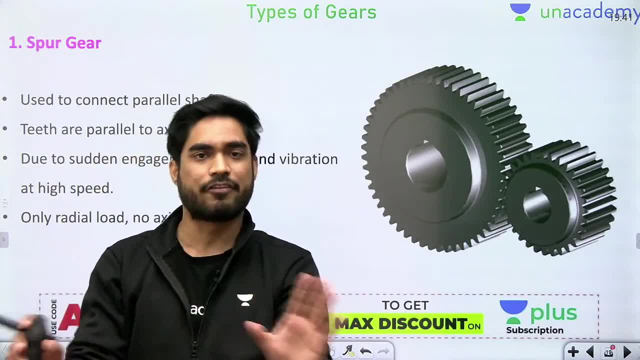 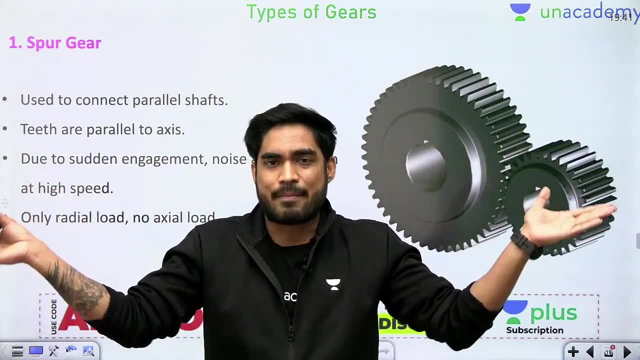 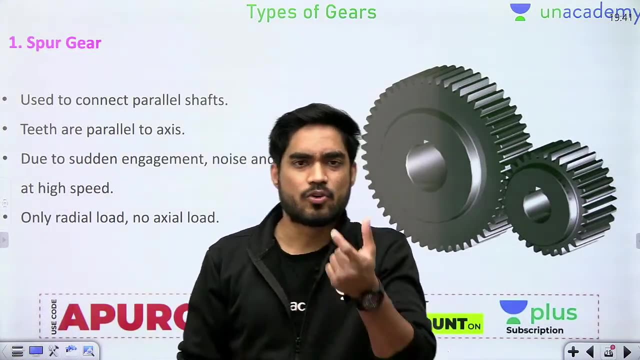 easy. compared to other gears. The manufacturing of gears are difficult. compared to other devices, compared to other elements, Manufacturing of gear is difficult, But among all the gears, the manufacturing of spur gear is difficult, Comparatively easy. okay, So where do we exactly use? What is the characteristic of spur gear? 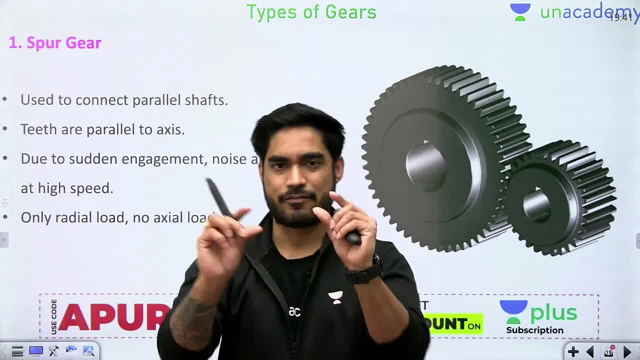 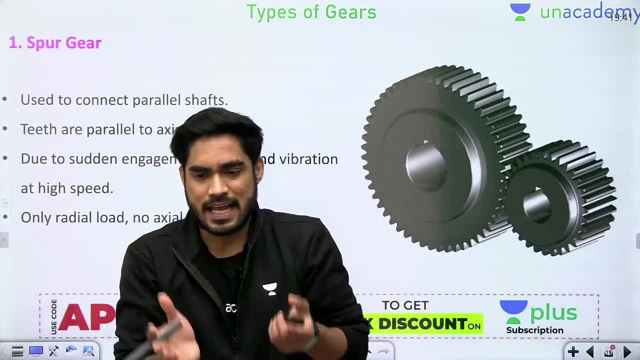 So, first of all, spur gear is used to connect parallel shafts. okay, All the gears are used to connect shafts. Now there can be two types of connection. The connection can be between two parallel shafts and between two intersecting shafts. okay, So beta spur gear is used to 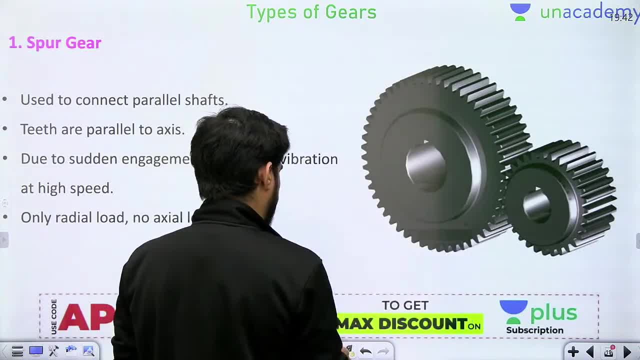 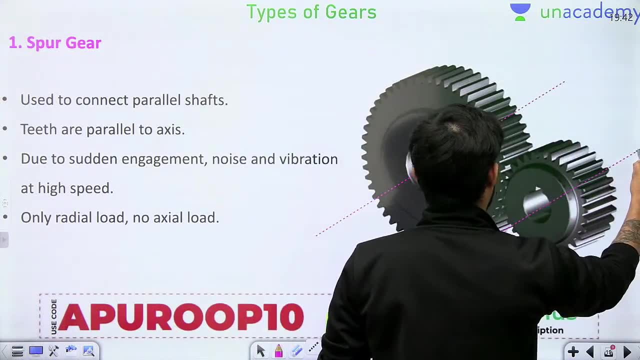 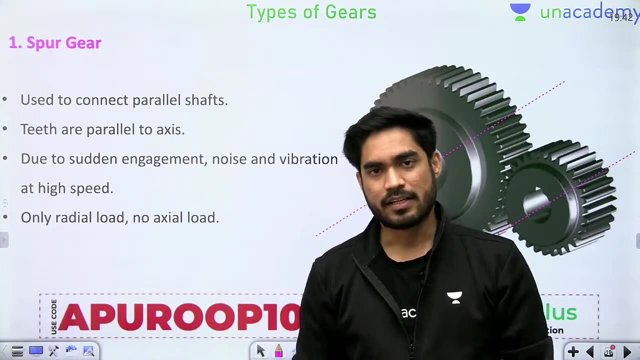 connect parallel shafts. You can see that the axis of the gears are parallel to each other. This is one axis, and this is one axis. You can see that the axis of the gears are parallel to each other. The axis of the shafts are parallel to each other. okay, Now the second point you need to. 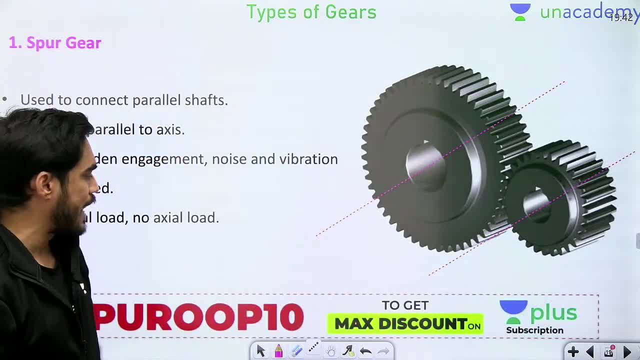 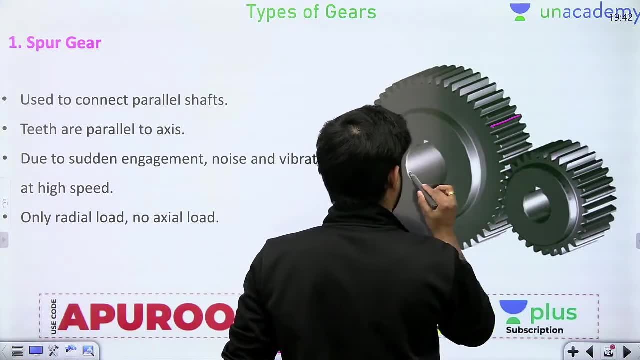 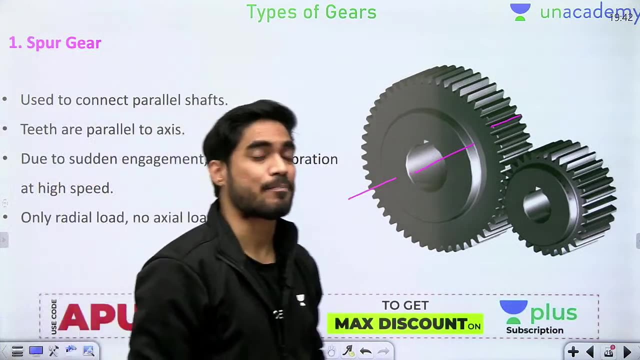 understand about spur gear is: the teeth of spur gear are parallel to the axis. You can see here that these teeth are parallel to the axis. These teeth are parallel to the axis, okay, So beta. that's why the manufacturing of these gears is difficult. So, beta. spur gear is used to connect. 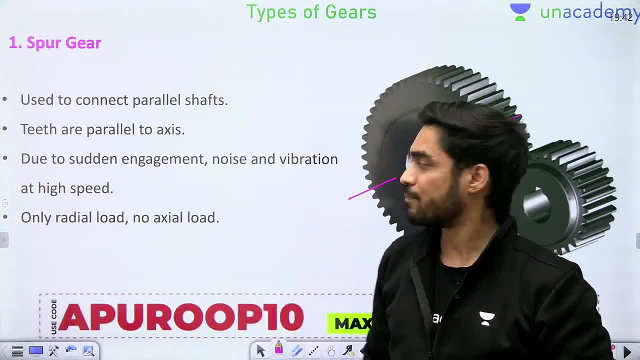 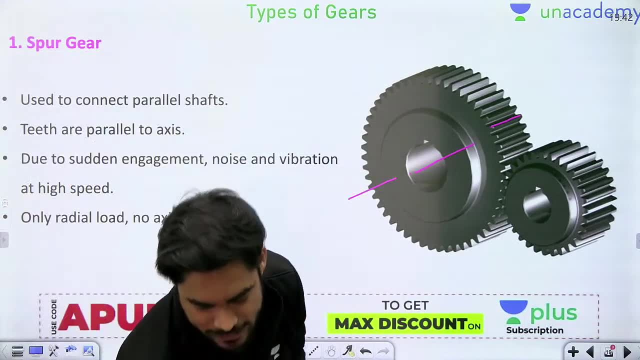 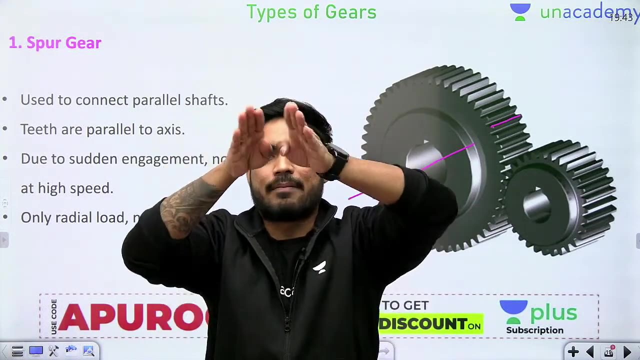 comparatively easy because we need to cut only parallel teeth. okay, But beta, due to these parallel teeth, there is a very big disadvantage. What is the disadvantage due to parallel teeth? understand, When there are two teeth parallel to each other like this, then when the teeth will, 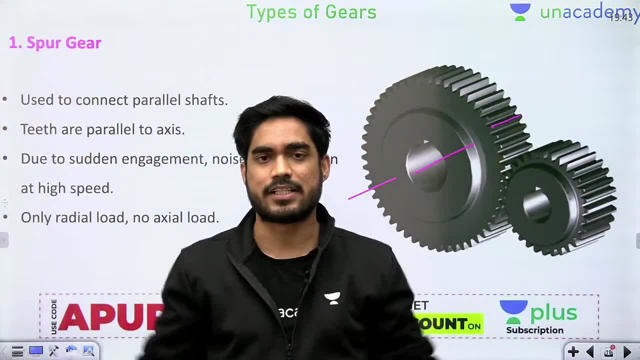 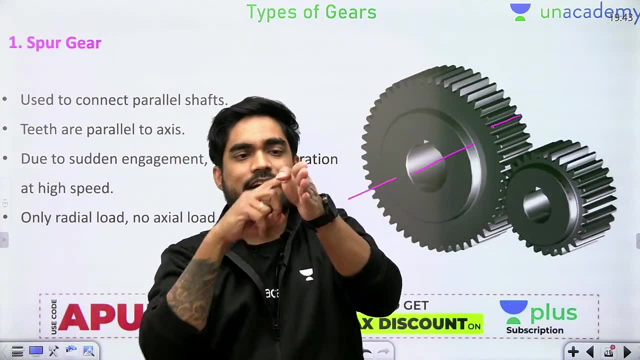 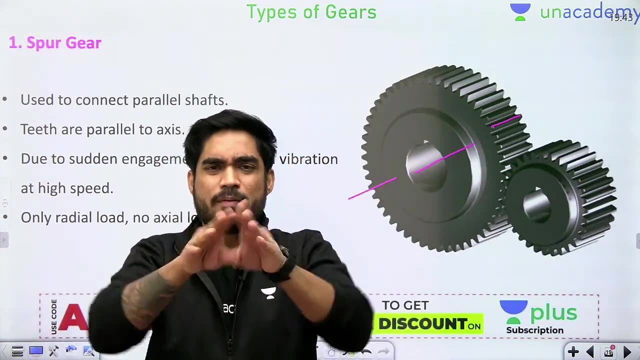 come in contact with each other. when the gear will come in contact with each other, the entire teeth will come directly in contact. The entire width of teeth will come directly in contact. So, beta, there will be a sudden power transfer. Now, what do we mean by sudden power transfer? I 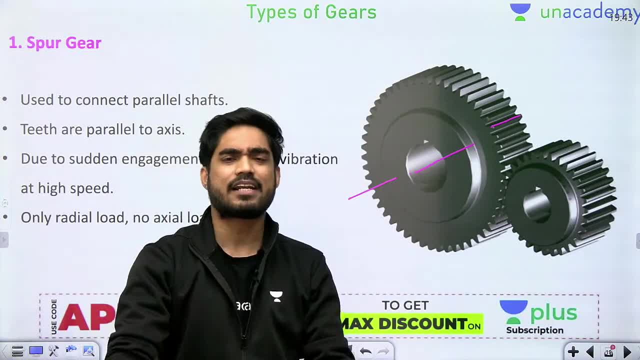 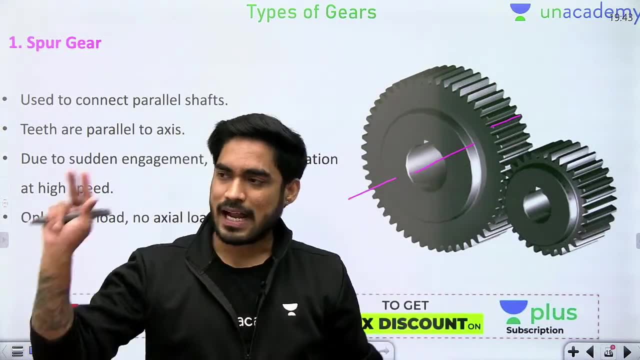 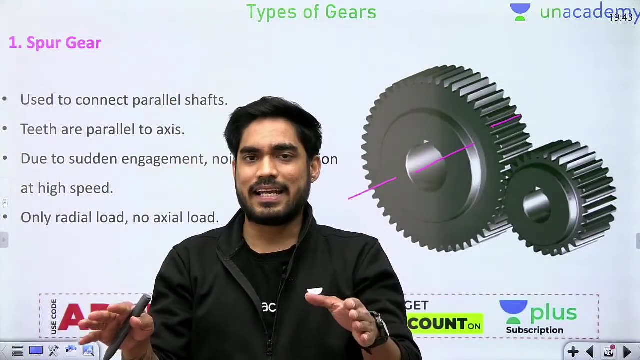 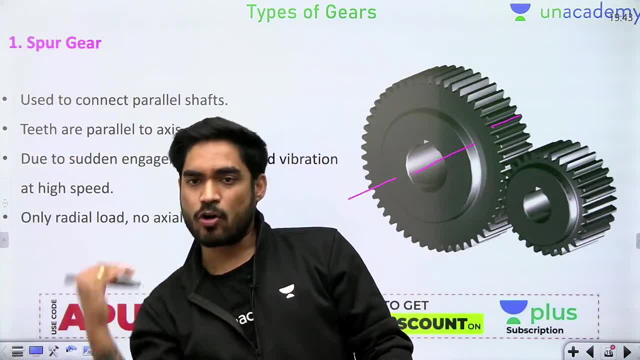 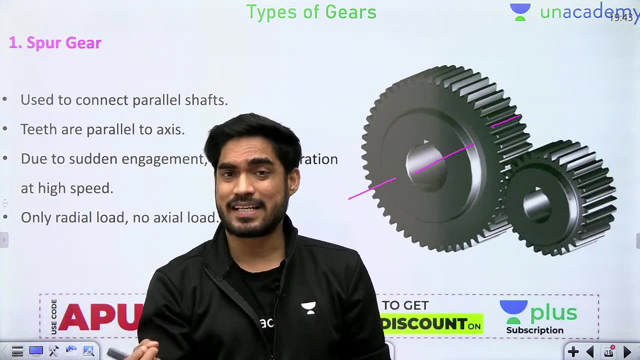 rotating at 100 rpm. This is rotating at 100 rpm. This is rotating at 100 rpm. When I will connect this one, then it will directly grow from 0 to 100 suddenly. then this is known as sudden power transfer. If the speed is going, if the speed is increasing smoothly from 0 to 100, if it is, 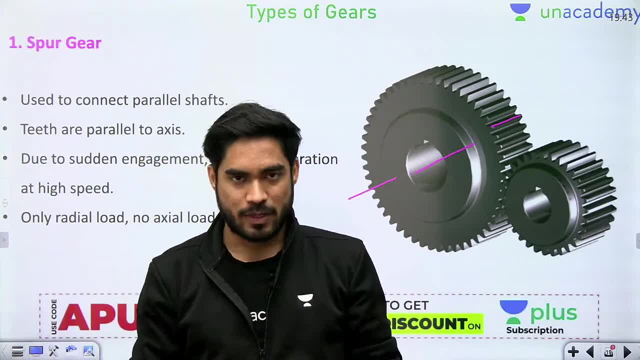 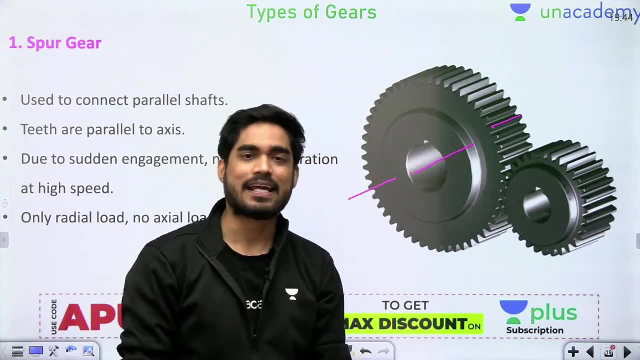 increasing smoothly, then it is known as smooth engagement. okay, gradual engagement, But if it goes directly from 0 to patak 100, then it is known as a sudden engagement. Then what will be due to sudden engagement? What is the disadvantage- Sudden engagement? 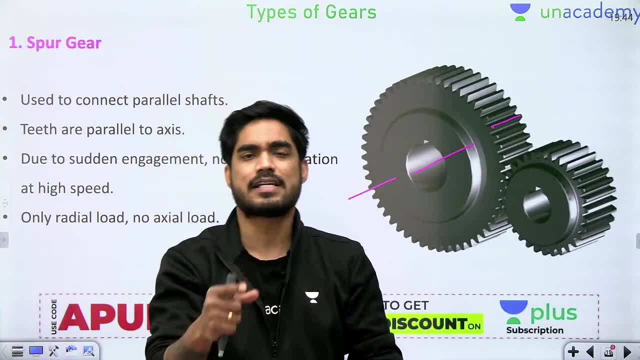 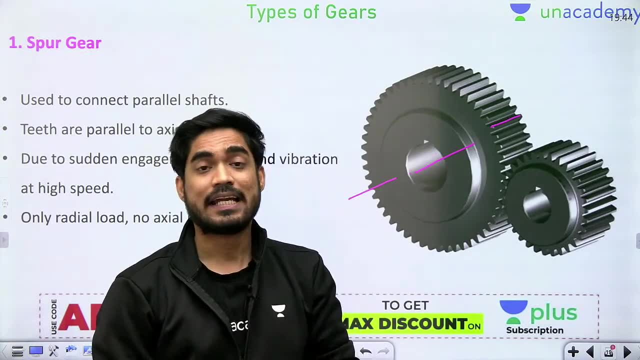 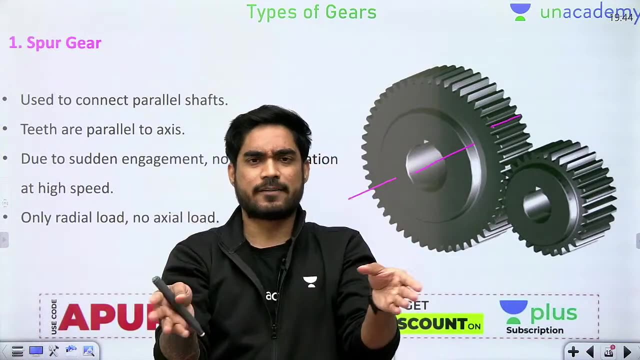 sudden engagement will cause what? It will cause noise, it will cause vibration, it will cause wear and tear. If, let's say, you are transferring the power suddenly between two teeth, then there will be noise. cut, cut, cut, cut. there will be noise. okay, There will be vibration. 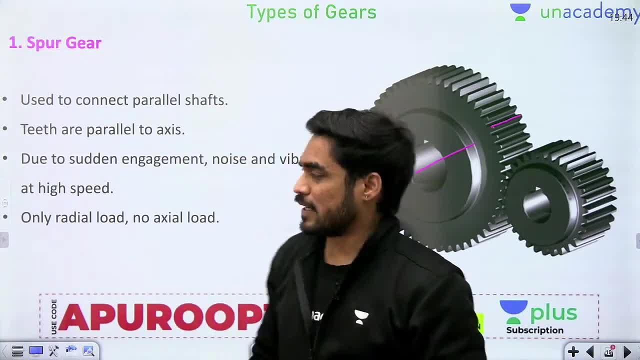 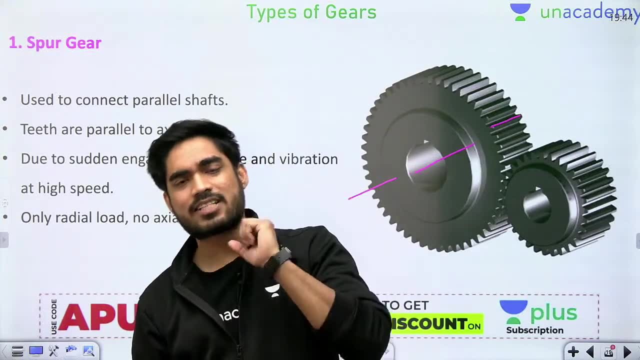 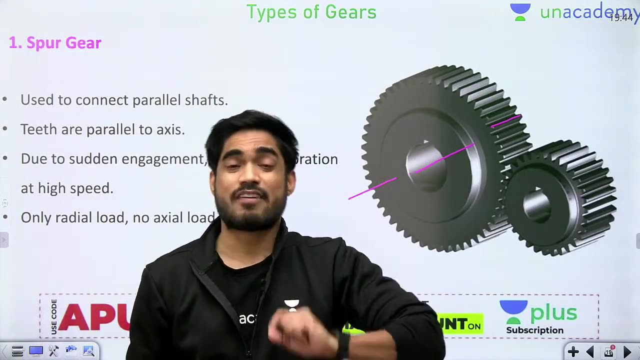 and there will be wear and tear of teeth. So because the teeth of spur gear will wear off rapidly compared to the other gears. okay, So that's why we will use spur gears only for low speed applications. If the speed is very high, then you can't use this gear. Why? Because in that 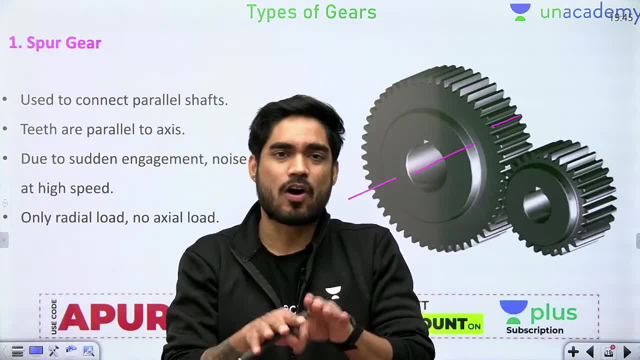 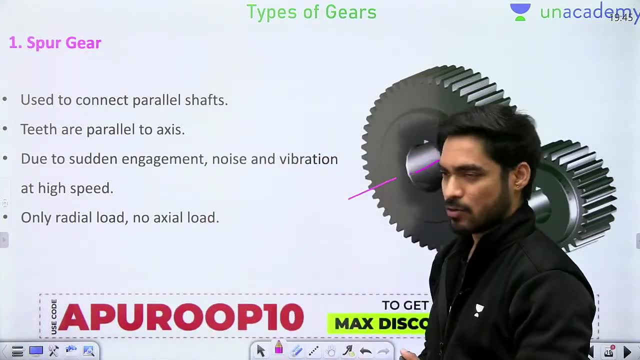 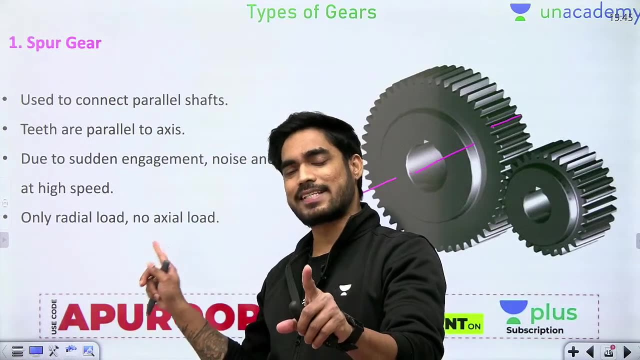 case, you will have a very high noise, wear and tear vibration. So in order to avoid that, we will use it for low speed application. okay, Now another very, very, very important point which you need to remember, because there was a question based on this concept. 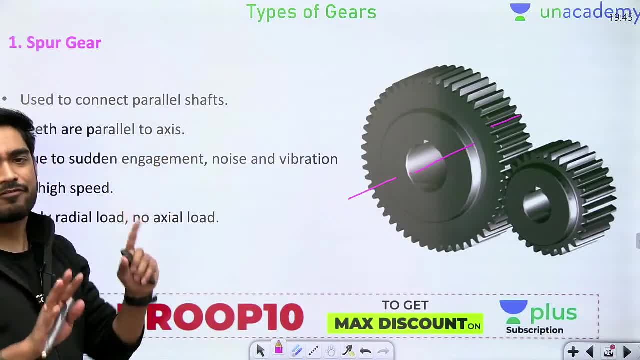 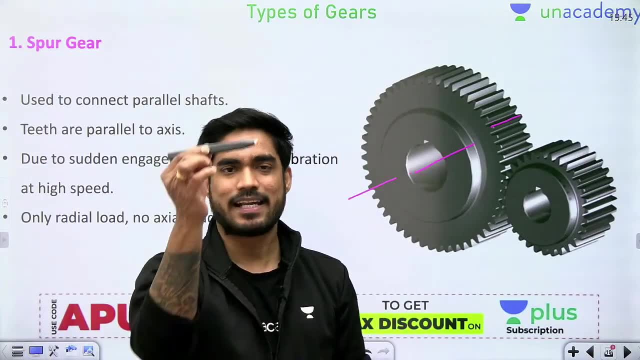 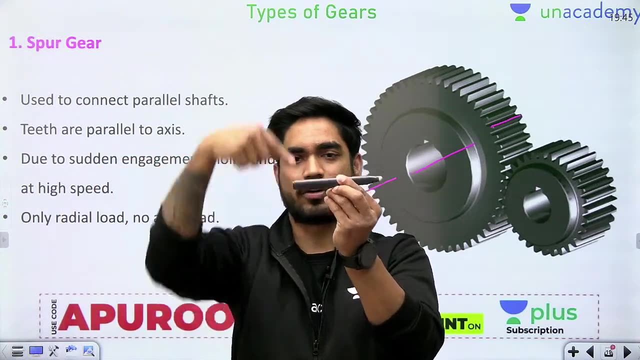 in gate. In case of shafts, there are two types of loads: radial load and axial load. What do we mean by radial and axial load? Let's say this is shaft, then the load along the length of shaft is known as axial load. This is axial load and the load perpendicular to the length is known as. 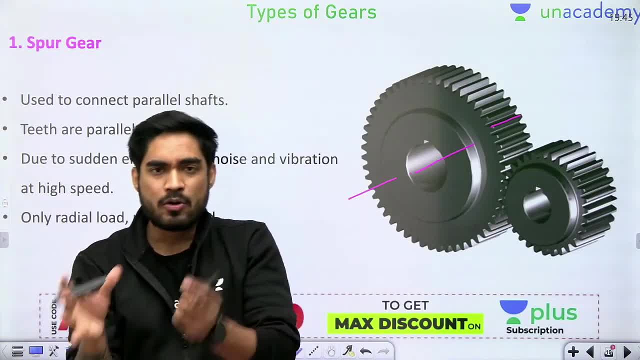 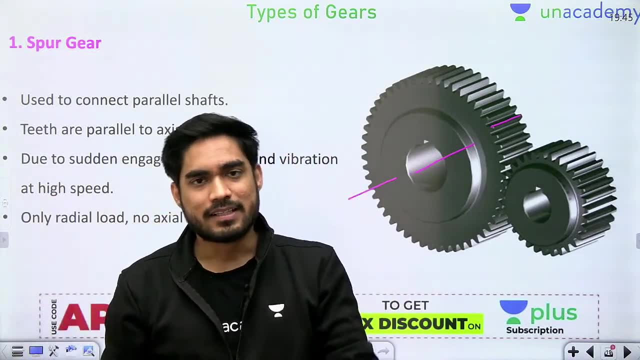 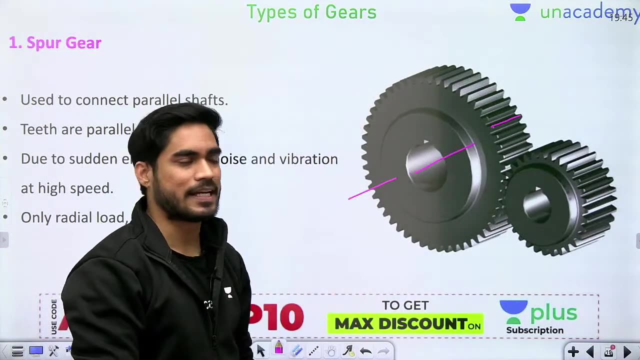 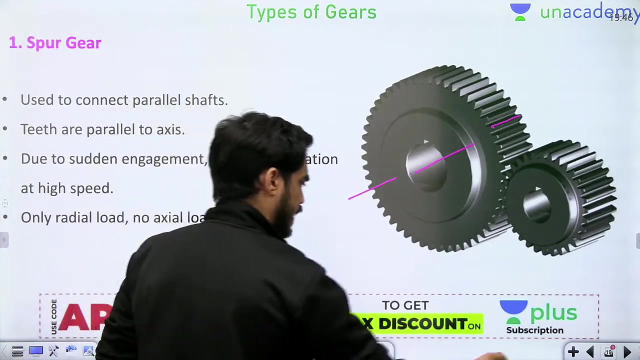 radial load. So, beta, when you mount the gear on the shaft, then the gears, when they will apply force on each other, this force will be transferred to shaft. So, beta, what type of force will be there in case of spur gear? So understand, in case of spur gear, when the gears will apply force on each. 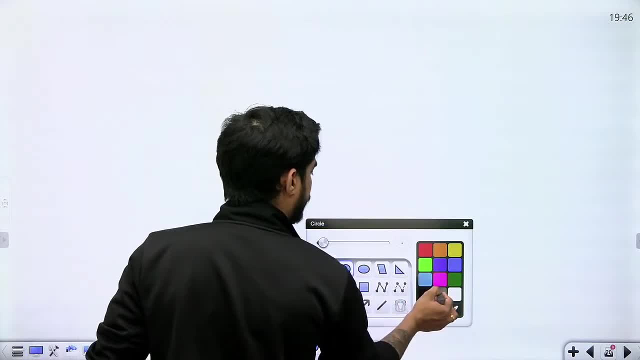 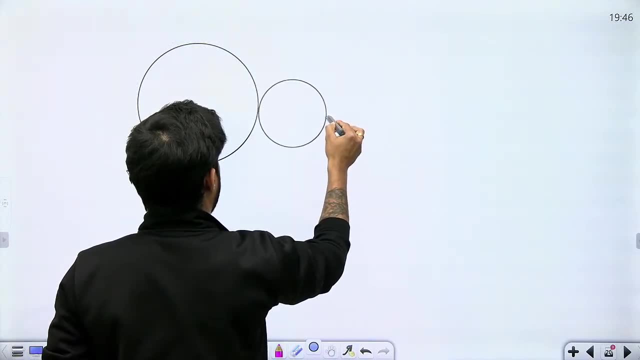 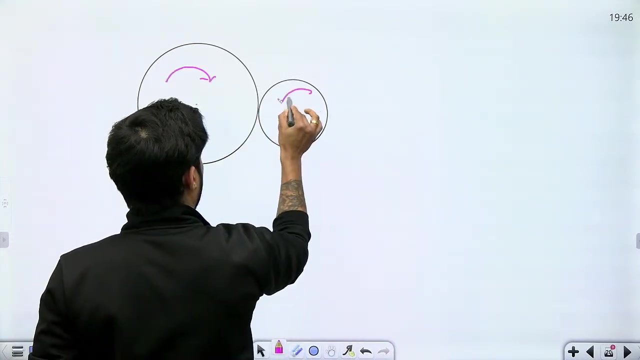 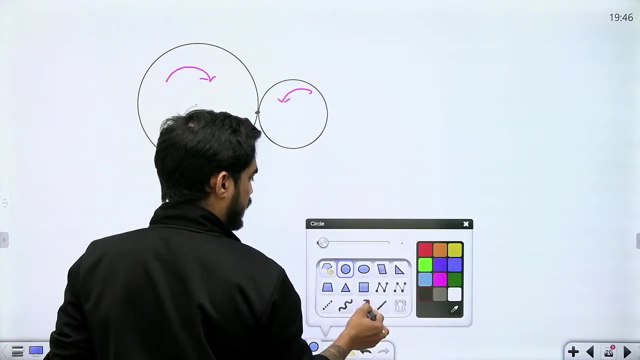 other. when the gears will apply force on each other, then you will see that this force will have two components. Let's say these are the two gears, okay. Let's say these are the two gears and they are touching each other at this point, okay. So at this point the force will be acting like this: 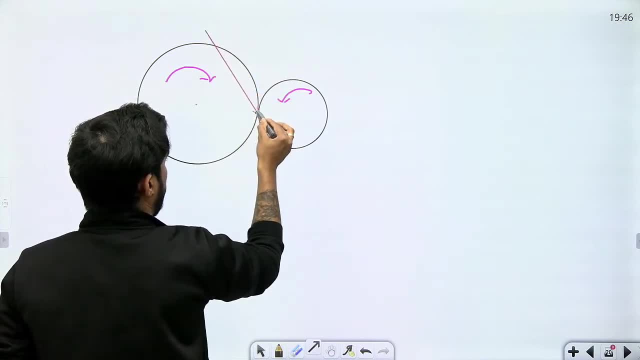 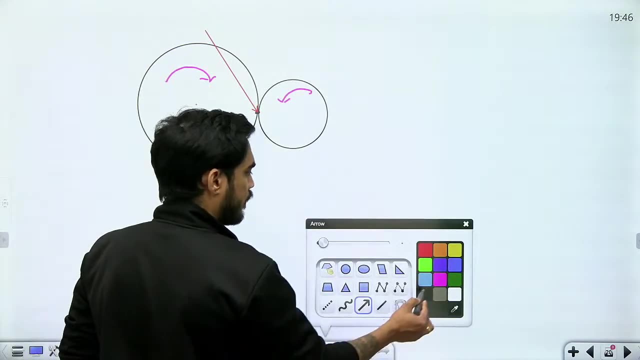 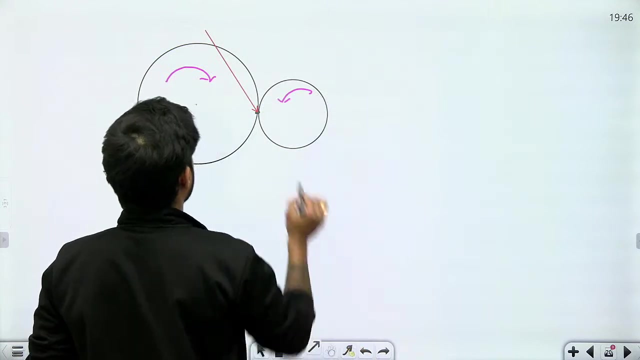 Let's say, this gear is applying force on this gear, So it will apply force on this gear like this: okay, Now this force will have two components: beta. This force will have two component: there will be a normal component and there will be a tangential component. 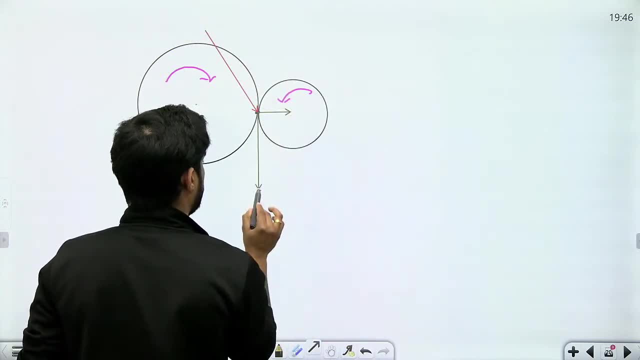 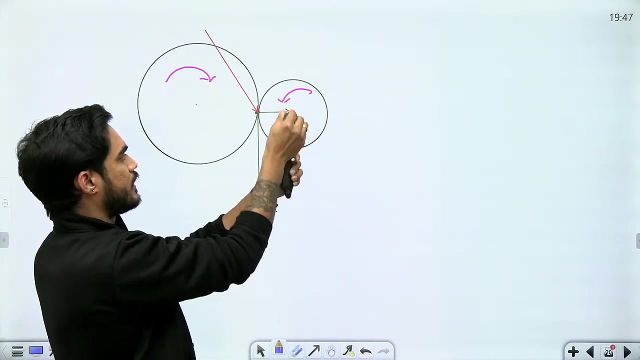 There will be a normal component and there will be a tangential component, like this: Both these forces- Fn and Ft, you will see, are radial forces only because beta, they are acting perpendicular to the length. Look at this. This is the shaft. So this force is acting perpendicular to the length. 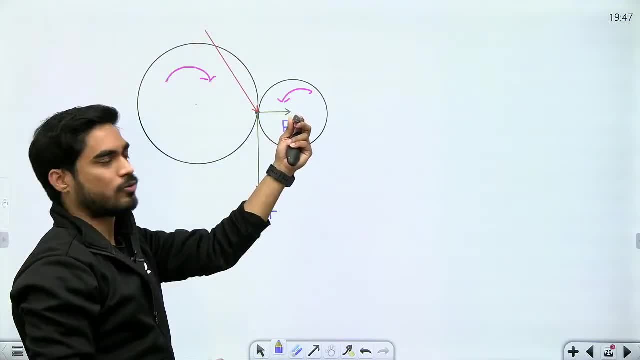 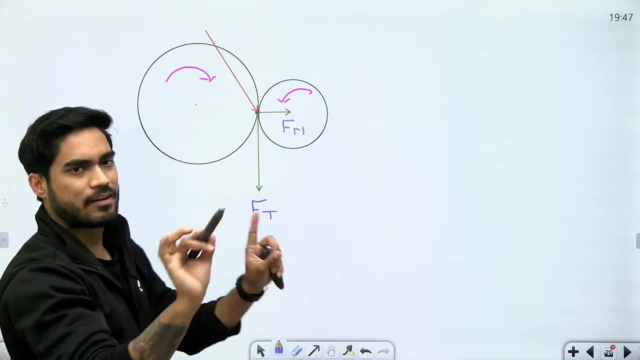 This force is acting perpendicular to the length. This force is also acting perpendicular to the length. right, This force will be along the length. This force will be axial force. So there is no axial force in case of spur gear. okay. 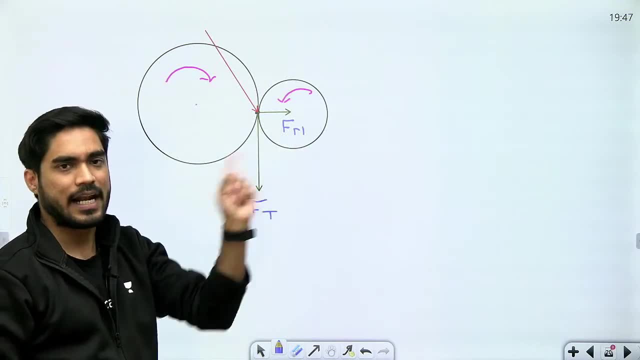 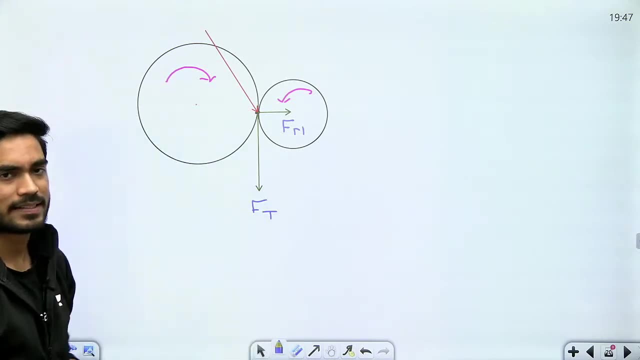 I will explain this force transfer in detail later. I will explain in detail later how this force comes and how it is calculated. But right now you need to understand what type of force is there in case of spur gear. So in case of spur gear, the force 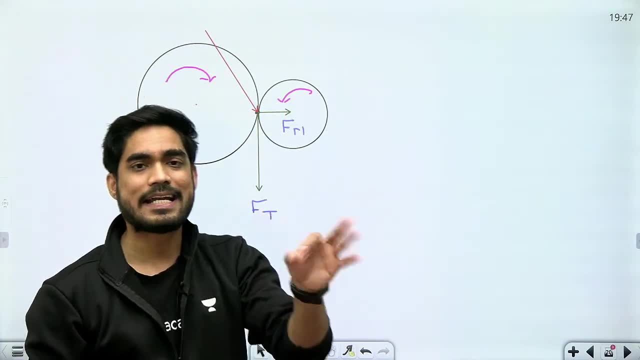 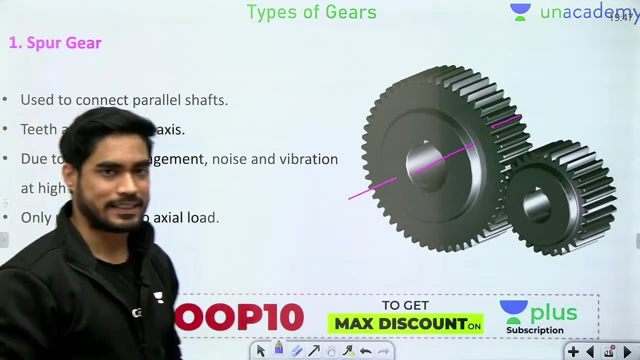 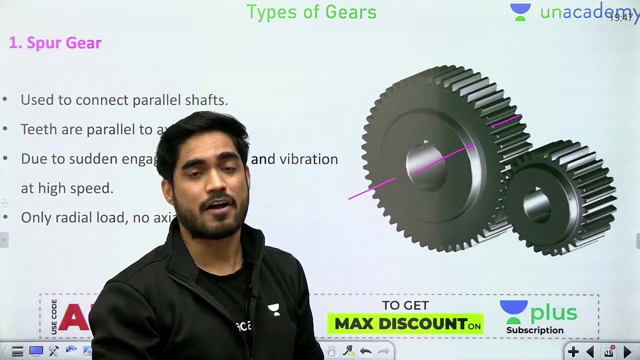 which is acting between the gear will have only radial component. It will not have axial component. okay, Now, this is a very important thing, because you might get questions based on this. okay, What type of question comes That? what type of stress will be developed in case of spur gear? okay, 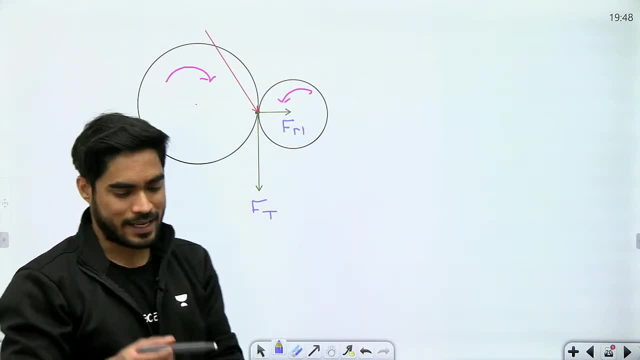 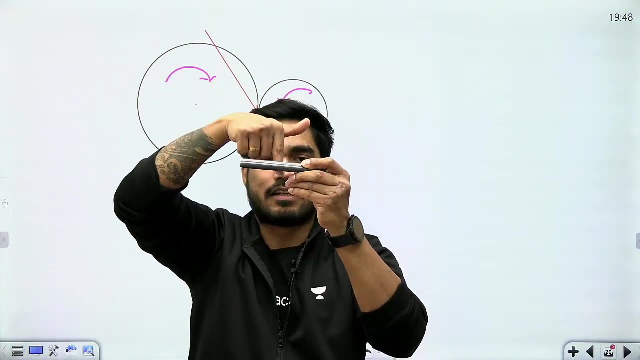 If I apply spur gear on the shaft, what type of stress will come? So if this is the shaft beta, if this is the shaft, then the force applied is like this: So if this is the shaft beta, if this is the shaft, then the force applied is like this: 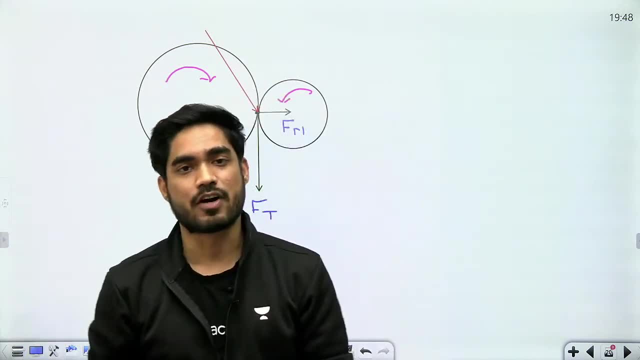 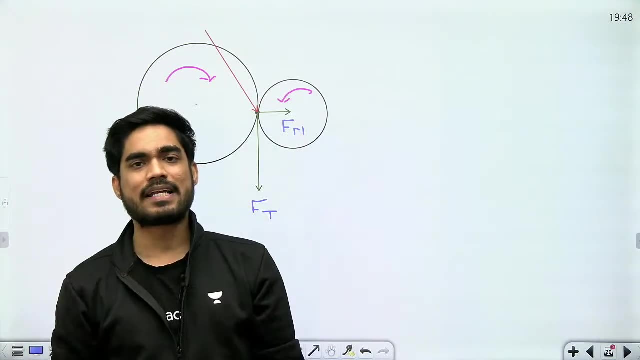 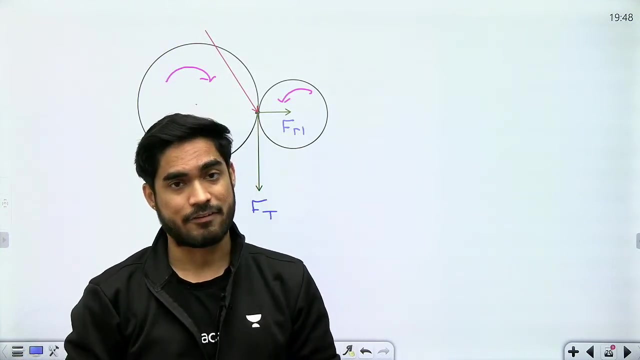 Both these forces are transfers forces which will bend the shaft. So there will be bending stress in the shaft right. But if there is an axial force also, then there will be an axial stress in the shaft. So in case of spur gear, what stresses will be developed in the shaft? 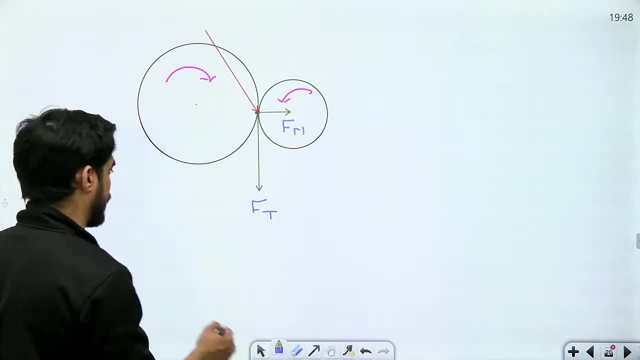 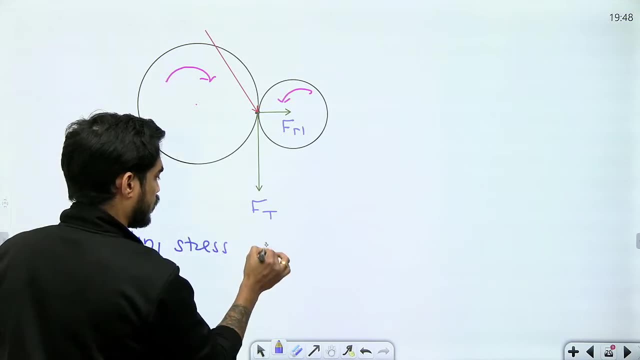 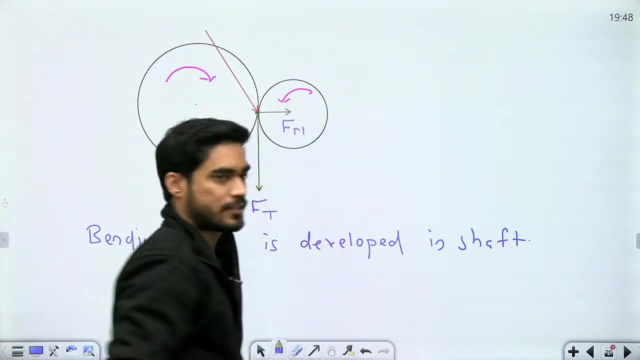 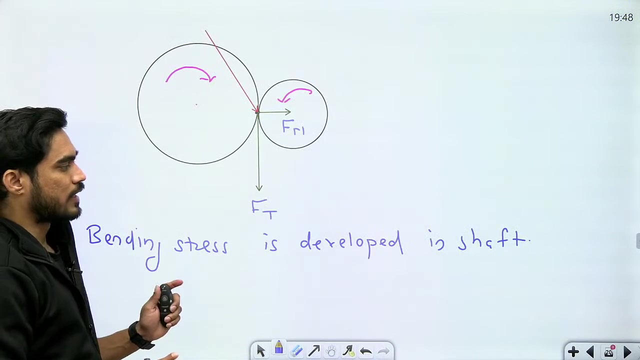 In case of spur gear, only bending stresses will be developed in the shaft. okay, Bending stress, no axial stress. okay, only bending stress will be developed and axial stress will not be there. okay, So this is the okay. torsional shear stress will also come, okay. 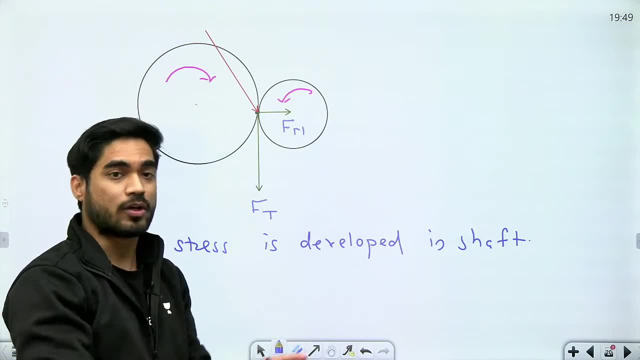 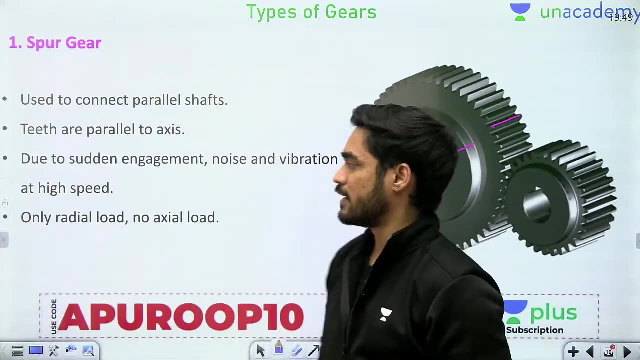 Torsional shear stress because shaft is transferring power. so that will remain, but bending stress will come because of this force. okay, So this is the first type of gears: spur gear. okay, Where it is used. It is used to connect to parallel shaft where the speed is low, okay, 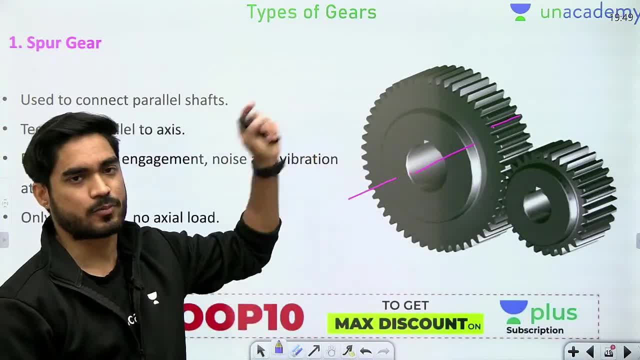 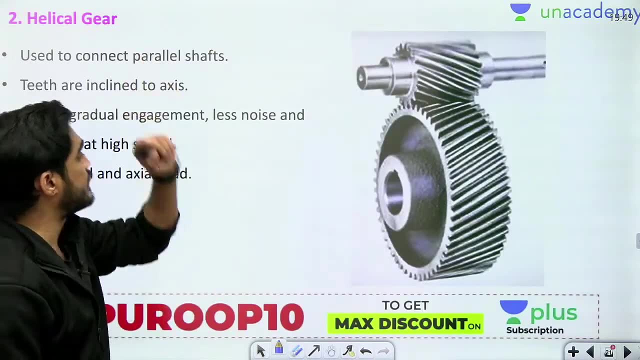 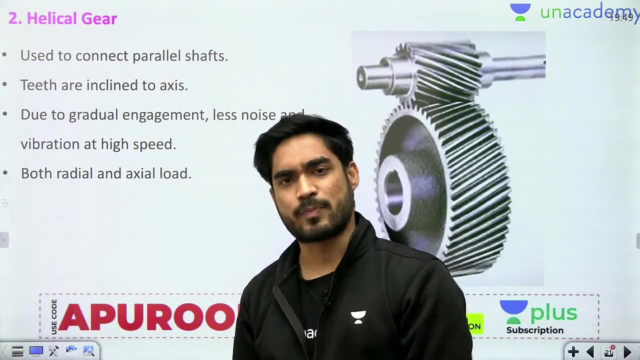 In low speed you have to use spur gear to connect to parallel shaft. Now, beta, overcoming this disadvantage, we have another gear known as helical gear. What is the shortcoming of spur gear? The shortcoming or disadvantage of spur gear is that it cannot be used in high speed application. why? 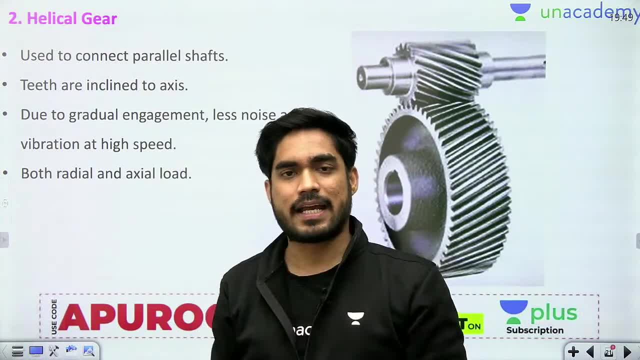 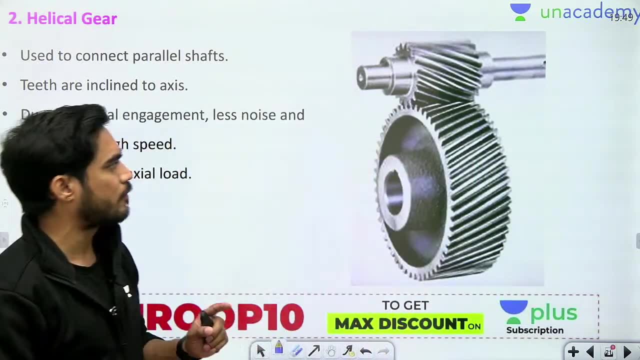 Because the teeth are parallel to each other, so there is sudden engagement. So in order to overcome that, we have made helical gears. Helical gears are also used to connect parallel gears, but there is a difference between spur and helical gear. 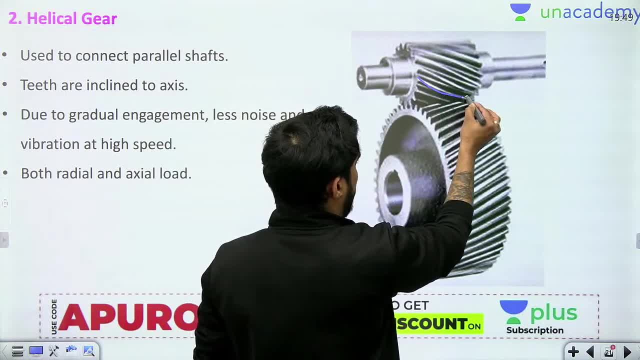 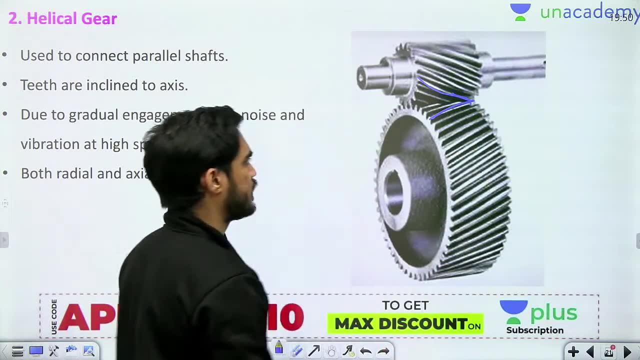 In case of helical gear, the teeth are not parallel to each other. you can see the teeth are like this. you can see the teeth are like this: inclined Now, due to this inclination, what will happen? understand. 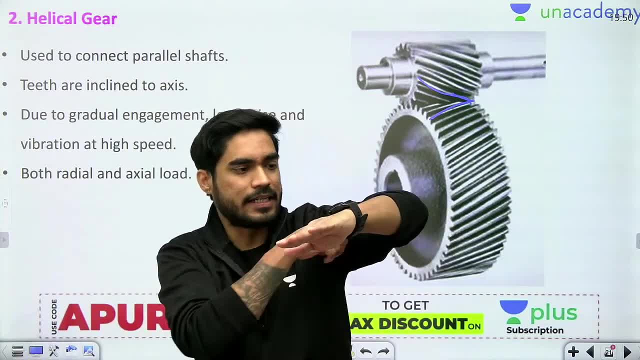 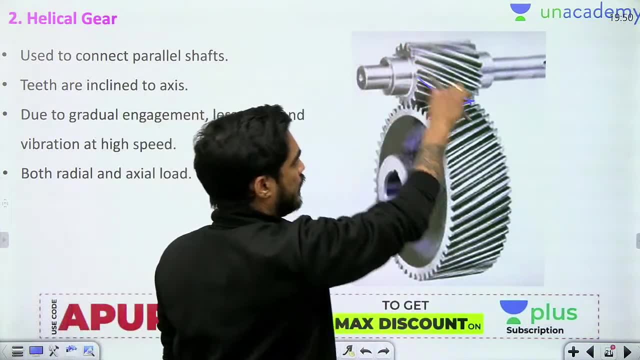 Let's say there is one helical gear like this: okay, the teeth is like this. Then the other helical gear will be like this: Okay, You can see that the inclination is opposite. In one case, if it is like this, then in other case it will be like this. 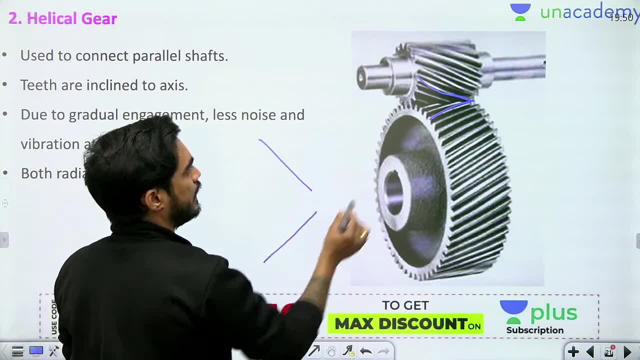 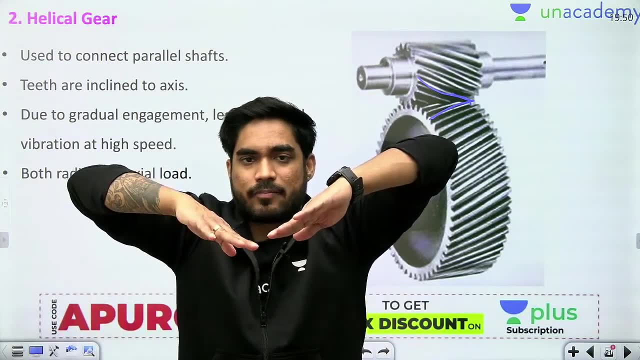 If there is such an inclined teeth in one gear, then there is such an inclined teeth in the other gear. you can see it here, okay? So due to this, what happens is, let's say this is one teeth, this is second teeth. 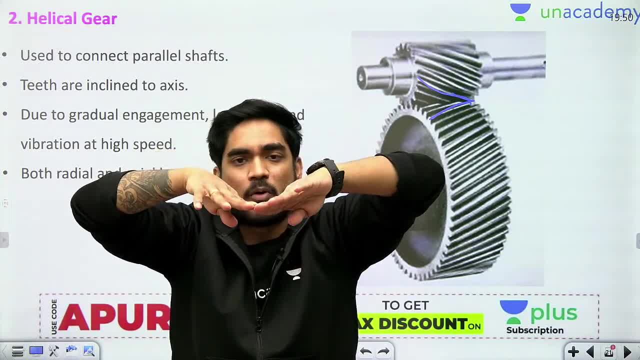 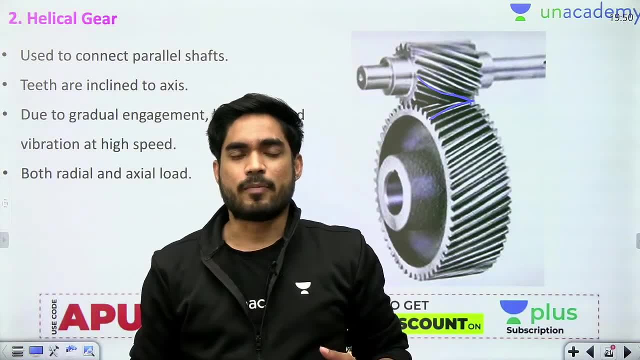 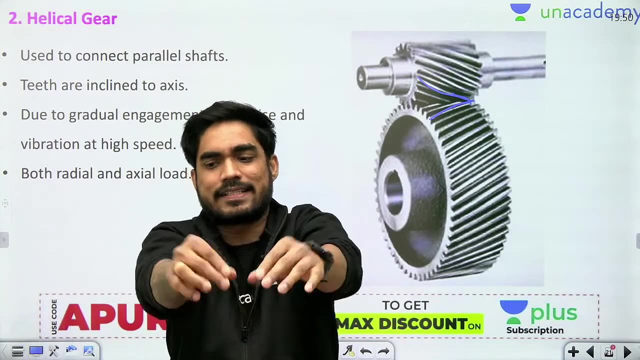 So when they touch each other, they only touch each other at one point, And when I will move the gear, then beta, they will come in contact completely. But the inclination here is smooth, because the inclination starts at one point and it gradually increases. 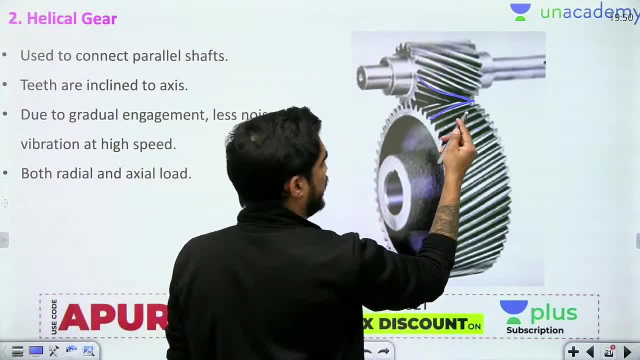 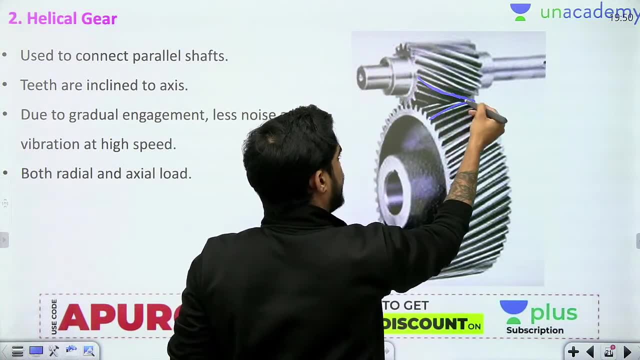 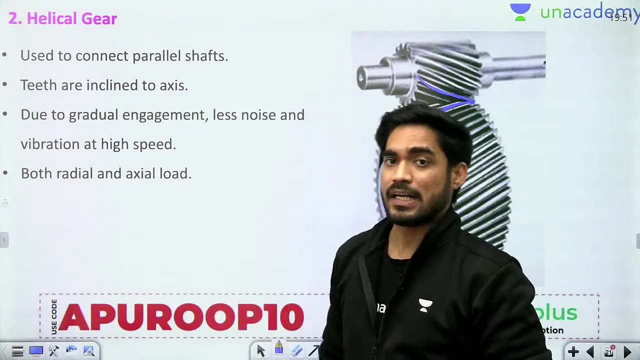 The contact. the contact starts from one point, The contact will start from here, and when you will rotate the gear, this entire width and this entire width will come in contact. Okay, So here the inclination is smooth and, due to smooth inclination, even at high speed. 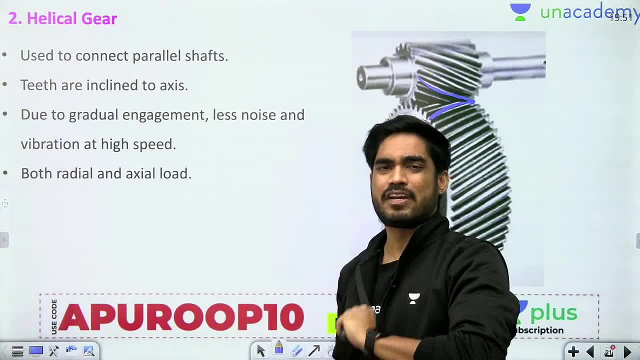 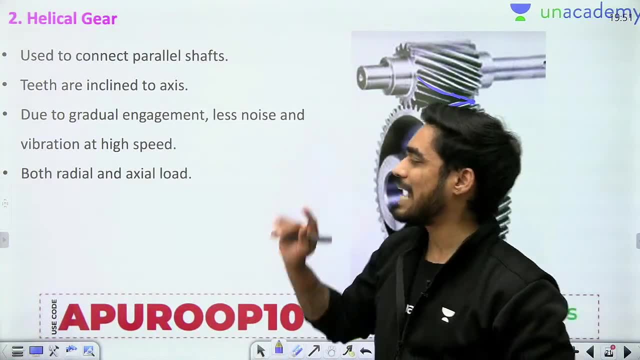 there will be no noise, no vibration, no wear and tear. okay, It will happen, but it will be very less compared to spur gear. okay, So that's why they can be used at high speed application. But beta, if there is advantage, then there is disadvantage also. 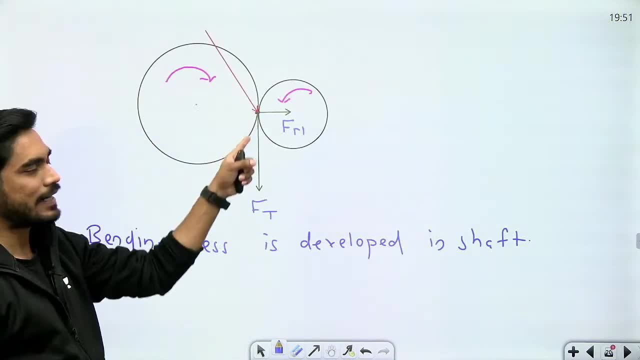 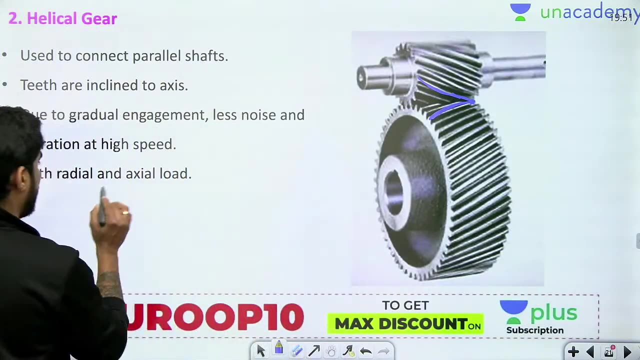 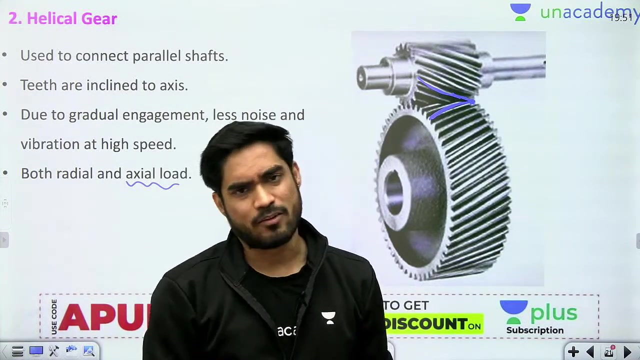 What is the disadvantage? In case of spur gear, we only get radial components of the force, But here the force will have another component known as axial component. So beta- there will be radial component As well as axial component. Now, due to axial component, what will happen? 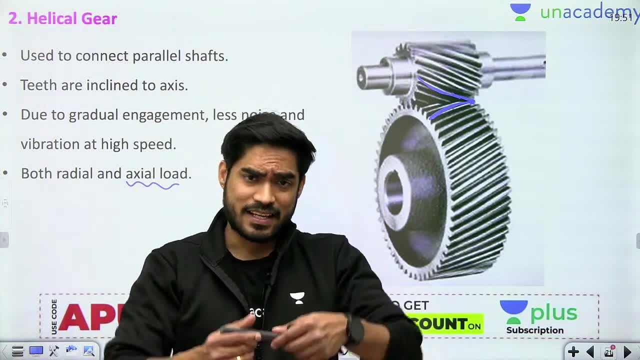 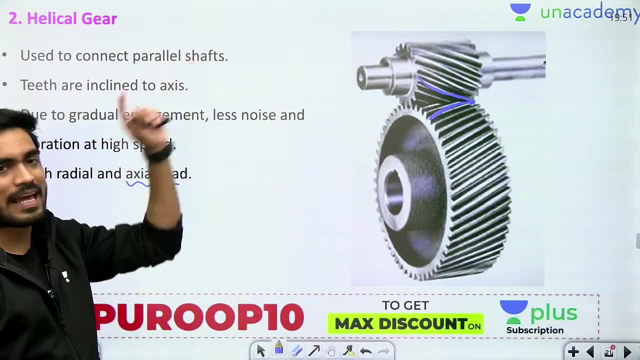 Due to axial component, there will be additional stress. There is already bending stress, Now there will be an axial stress also. okay, So that is the disadvantage of helical gear, But we can overcome this disadvantage also using double helical gear. 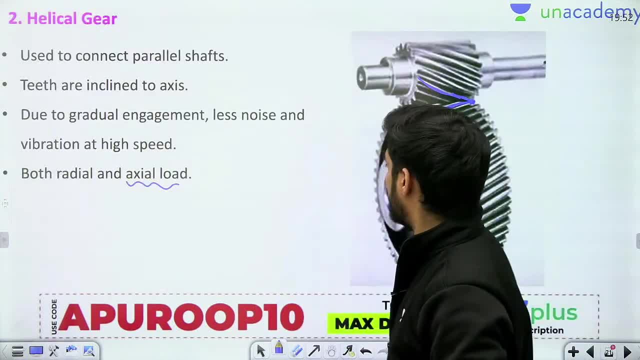 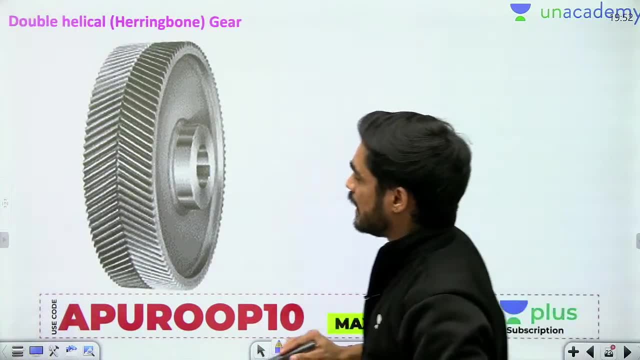 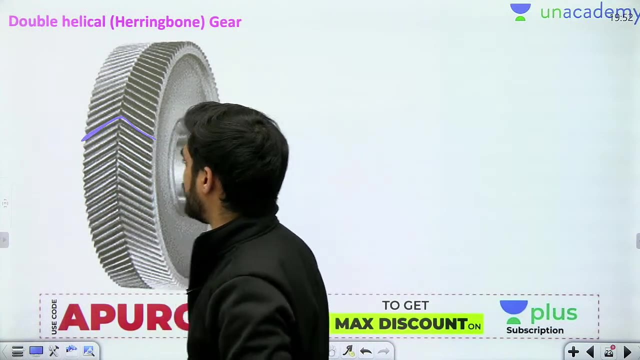 What is double helical gear Understand? In case of helical gear, the entire width of teeth is inclined like this. But in case of double helical, half of the width have inclination of teeth like this And other half have inclination like this: 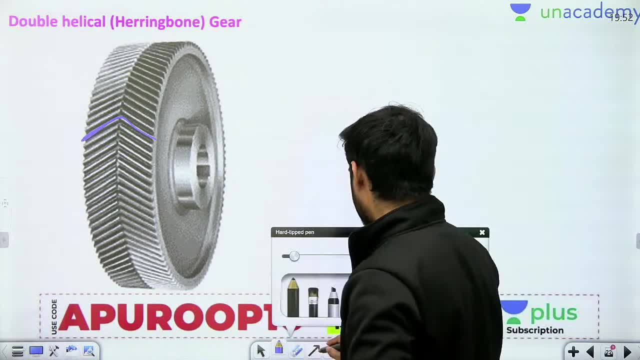 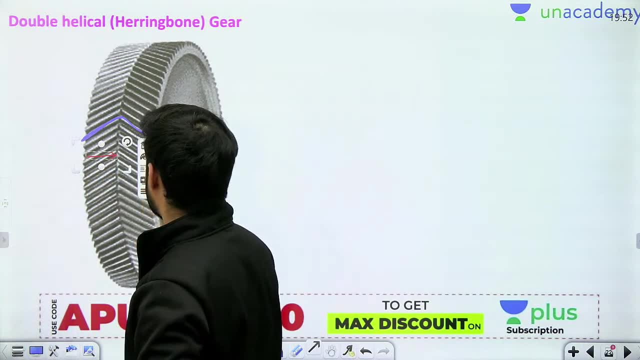 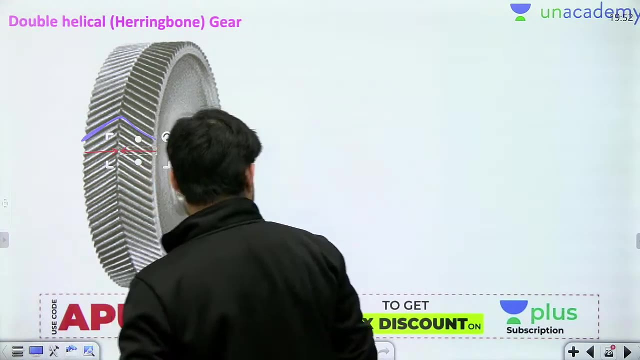 So, due to this, what is going to happen When the axial force will be developed? half of the axial force will be like this. Other half axial force will be like this: So both these axial forces will cancel each other. These two axial forces, this FA and this FA, will cancel each other. 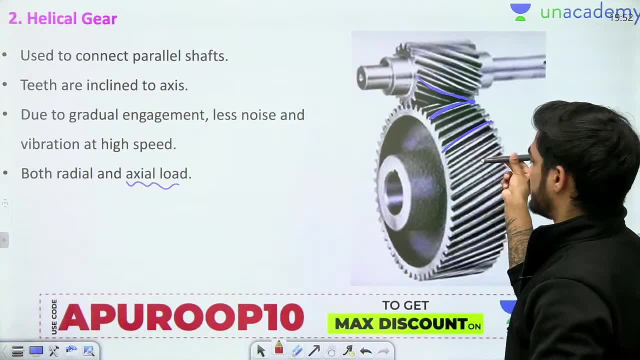 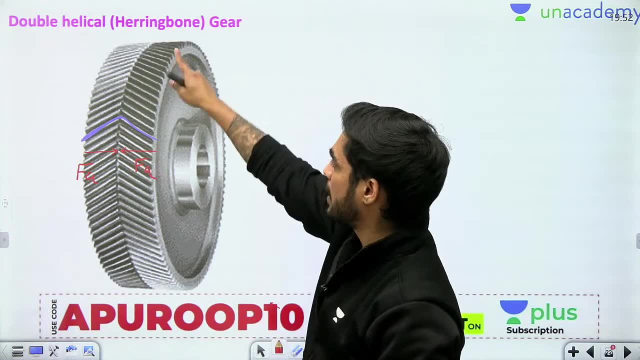 Okay, Here there will be axial force like this, So beta single axial force. Here there are two equal and opposite axial force which nullify each other. So there will be no axial force in double helical gear. Okay. 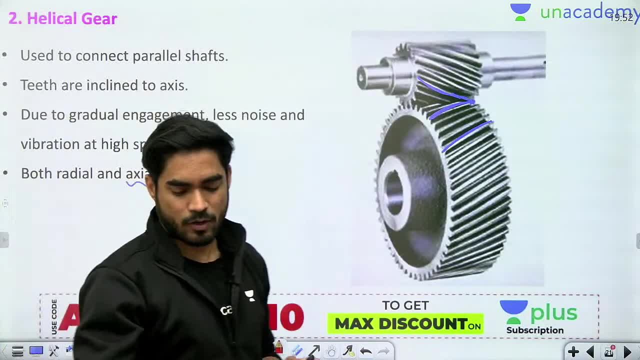 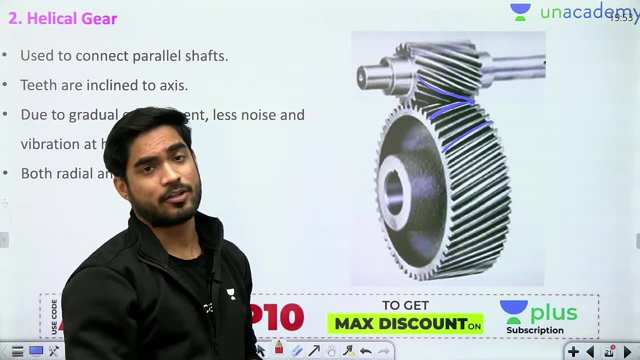 So, beta, do you understand the difference between spur gear, helical gear and what is double helical gear? I hope it is clear to everyone, Right? Please hit the like button Everyone. what you guys are doing, Please hit the like button while watching. 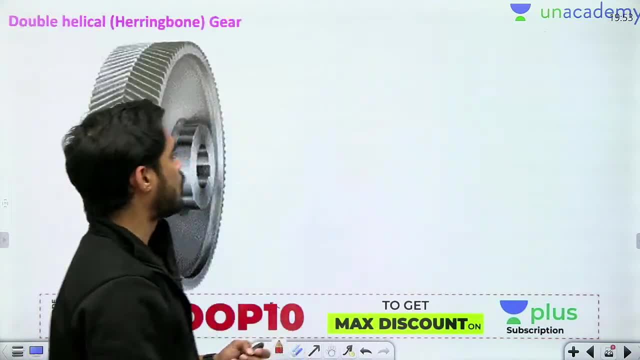 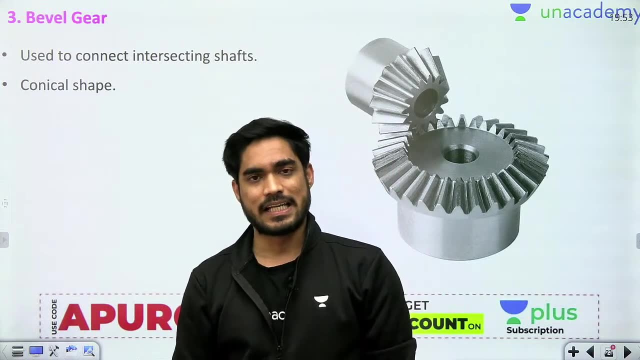 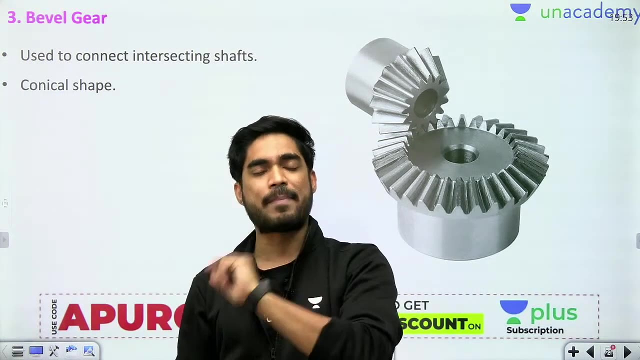 Hit a like button and at least hit a share somewhere. Okay, Next beta bevel gear. Now, what do we mean by bevel gear? Spur gear and helical gears: both are used to connect parallel shafts. In both cases, the axis of the shafts are parallel to each other. 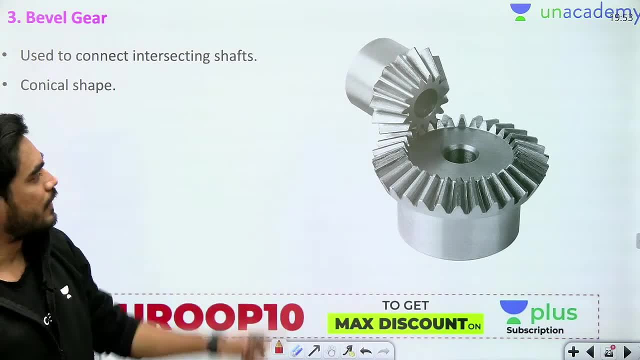 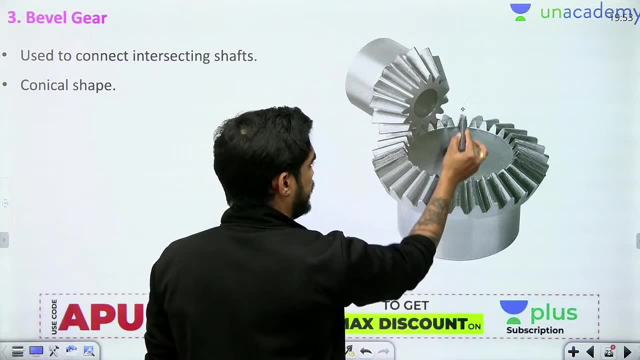 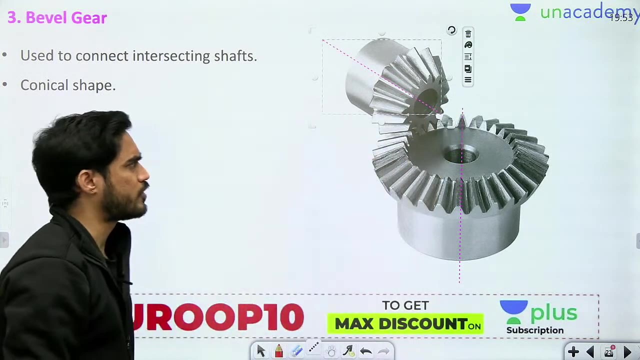 But in case of inclined axis we will use bevel gear, So you can see that the axis of one shaft Is vertical and the axis of another shaft is, like this, Horizontal, almost horizontal. So, beta, they are inclined to each other. 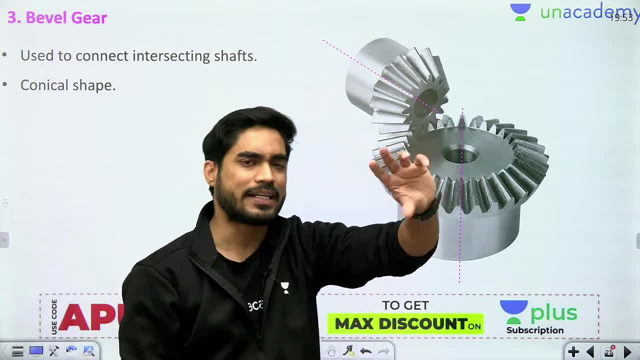 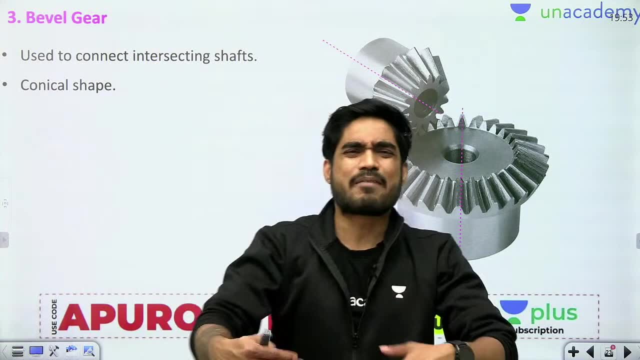 Usually this angle of inclination is 90 degree, But it can be slightly different than 90 degree. also, Okay Inclination means it does not happen at 60 degree, Because there is no application of that type. usually Very rarely you will see the angle of inclination other than 90 degree. 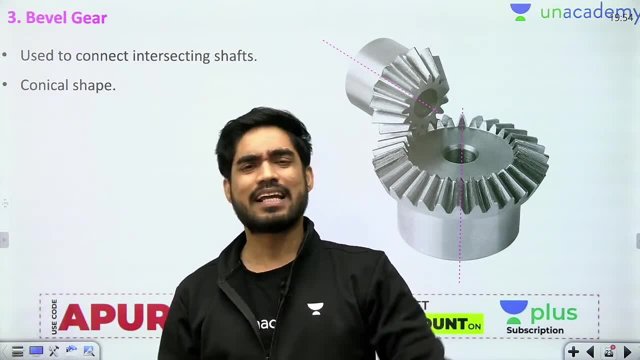 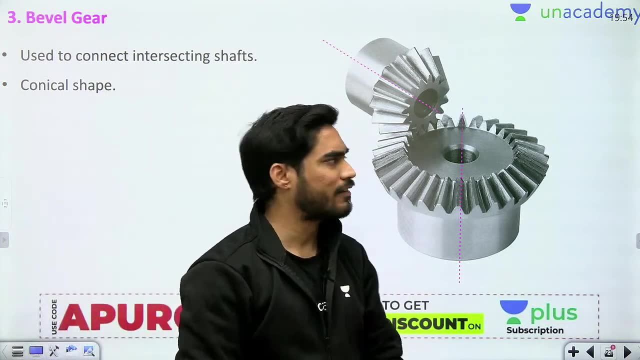 Otherwise, if there are inclined shafts to each other, Then it will be at 90 degree only. Okay. So, my brother, if there are shafts at 90 degree with each other, Then we will use bevel gears, Okay. 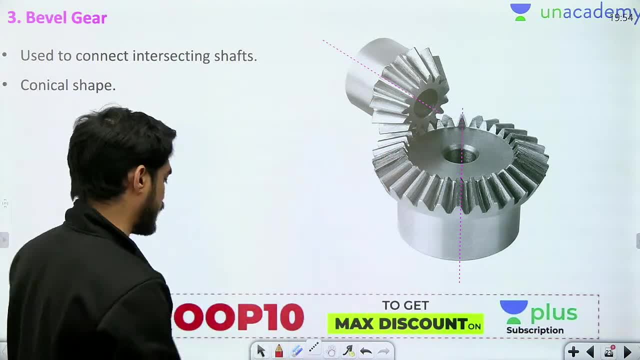 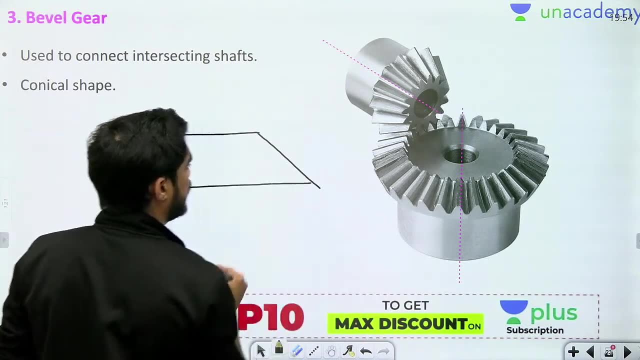 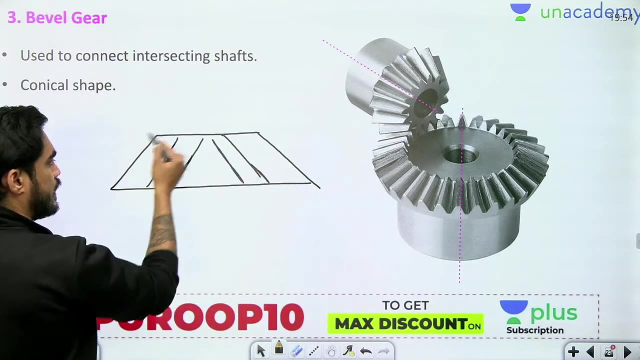 Now, in bevel gears, the shape of gear is conical. You can see that the gear is like this. You can see that the gear is like this. Gear's teeth are like this. So, beta, the shape of the gear is conical. 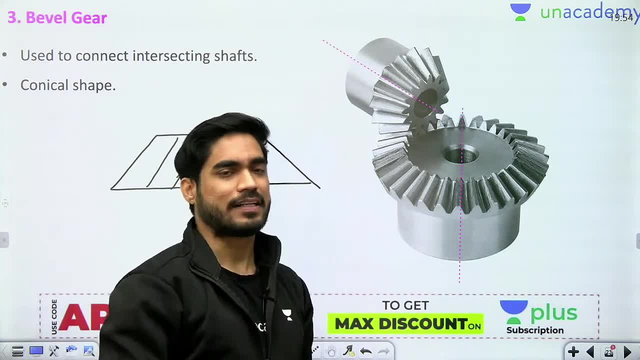 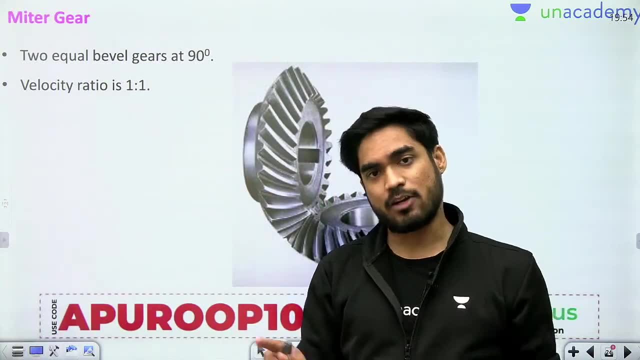 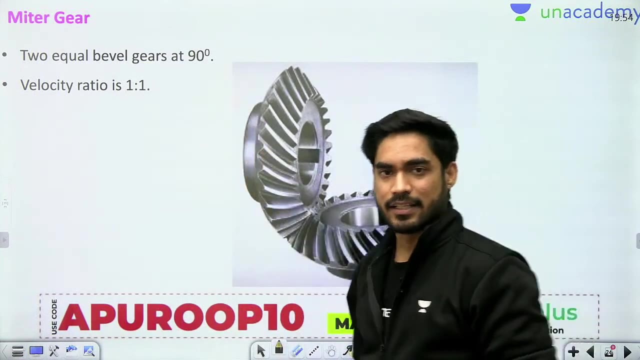 Okay, Now bevel gears have a very specific type, known as meter gear. Now, what is meter gear If there are two equal bevel gears, Equal bevel gear means same size. If there are two same size bevel gear at 90 degree with each other, 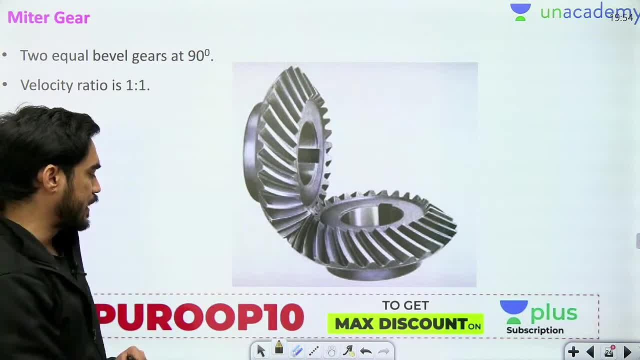 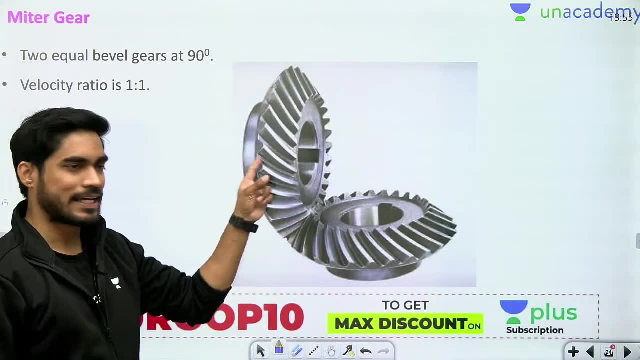 Then it is known as meter. And in case of meter, what will be the velocity ratio? The velocity ratio will be 1 ratio 1.. Because the size of both the gear is same, So beta velocity ratio will be 1 ratio 1.. 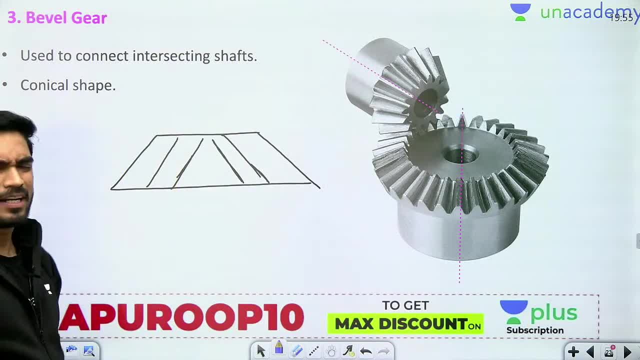 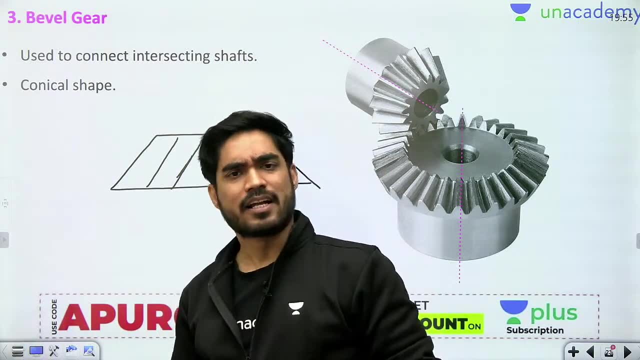 Yes, Very good. So beta, bevel gear is also clear Beta, you don't need to get into details of each and every gear: How it is manufactured, Where exactly it is used. You don't need to remember that. 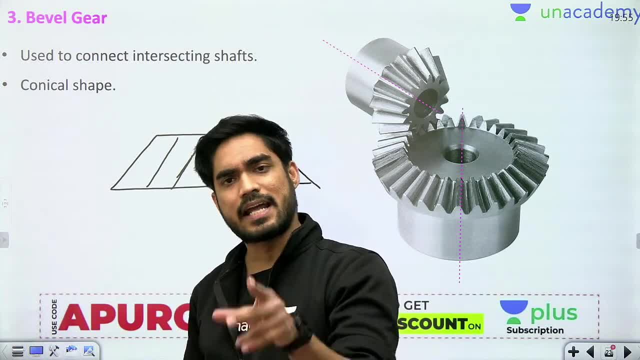 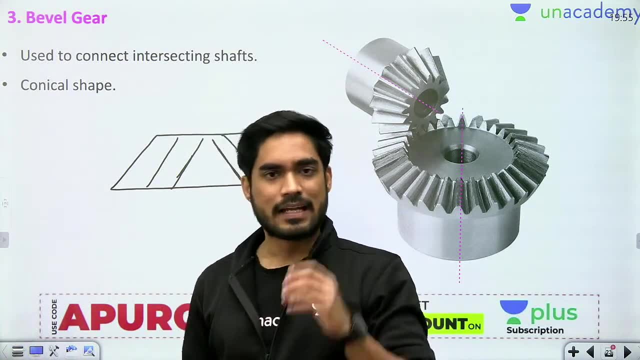 All you need to remember is this special characteristic: Spur gear and helical gear are used to connect parallel shaft, But in spur gear, sudden engagement, noise, vibration, Less speed. In helical gear, smooth engagement, no noise, vibration, high speed. 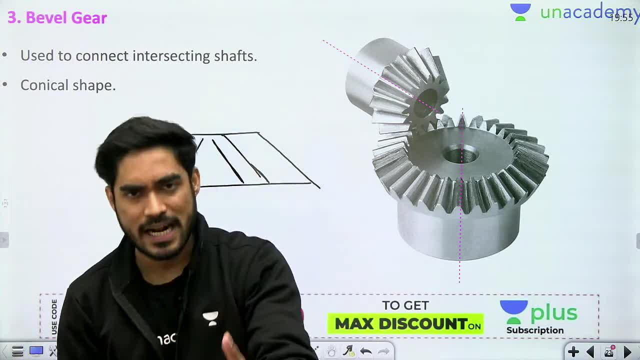 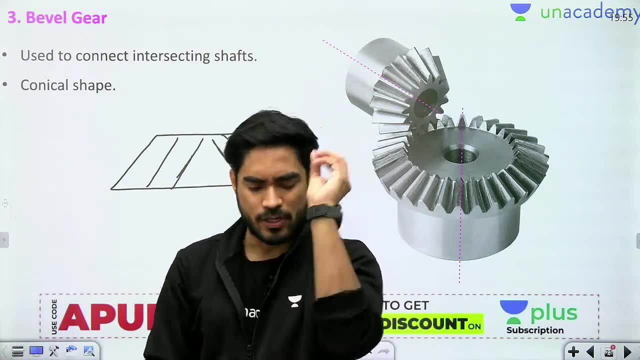 Bevel gear are used to connect inclined shafts, Usually at 90 degree. Meter gear is special bevel gear with velocity ratio 1, ratio 1.. So only one or two points about each gear you need to remember. That's it. 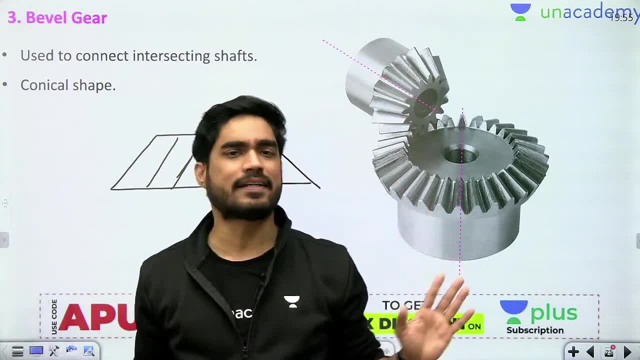 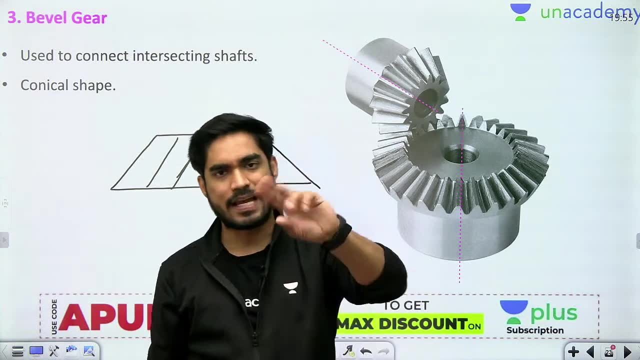 Okay, You will have theory question based on this small characteristic. only, You don't need to read their whole birth chart. Okay, You don't need to read the whole paragraph, You just need to remember these one or two points. That's what I have written. 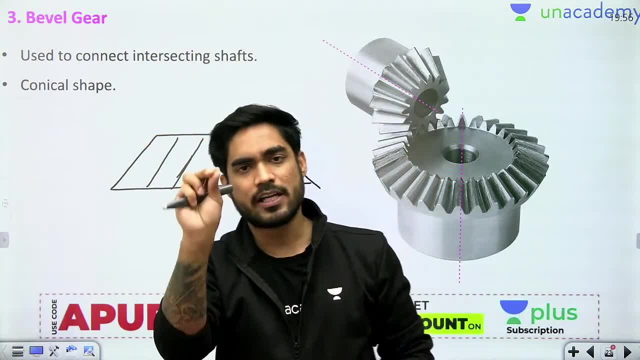 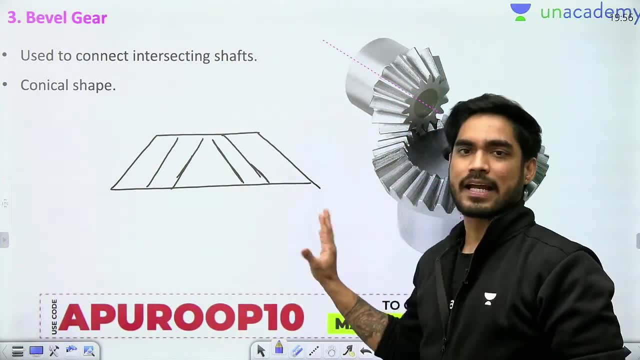 Okay, Whatever, I have written one or two small points That only you need to remember, Because even if I fill this page with information, Then you will enjoy looking at it, But you will not be able to remember it. Okay, If I fill the whole slide with the life of bevel gear. 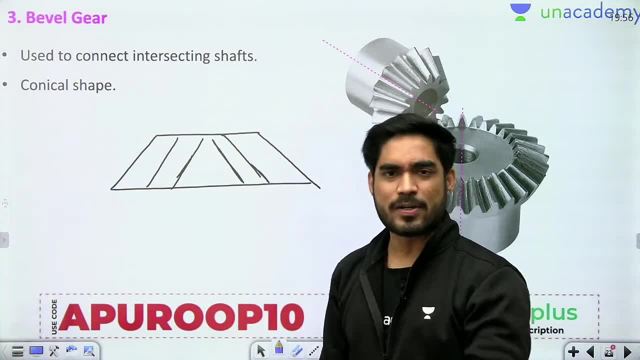 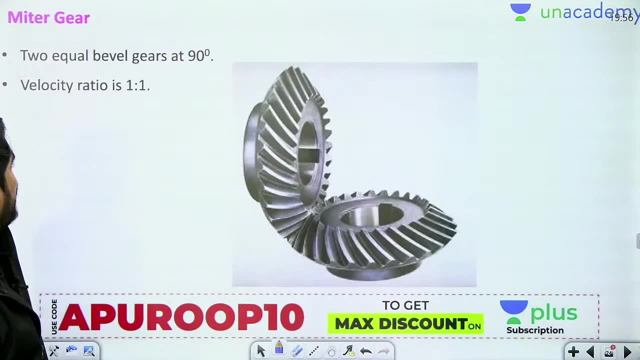 Then it will be fun to read, It will be fun to know, But it will not be remembered. It has no meaning. That's why I have written those points on which the question will come. Okay, Next type of gear is Warm gear. Now, this is a very special type of gear. In case of spur, helical or bevel gear, Maximum speed ratio that you can get is 10 ratio 1.. In case of helical gear, you will get 10 ratio 1.. 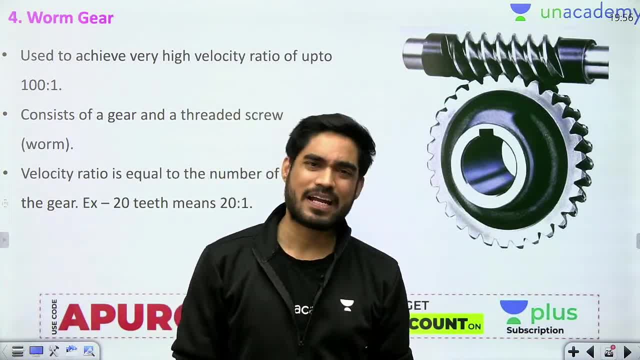 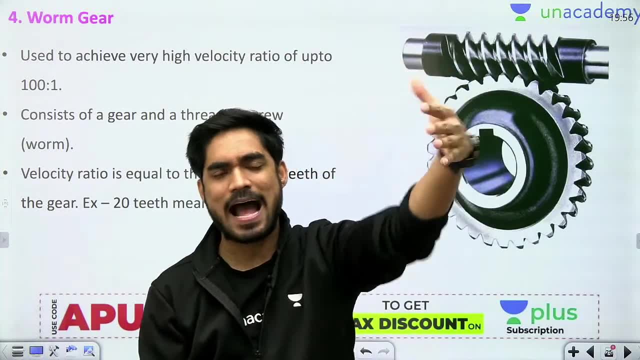 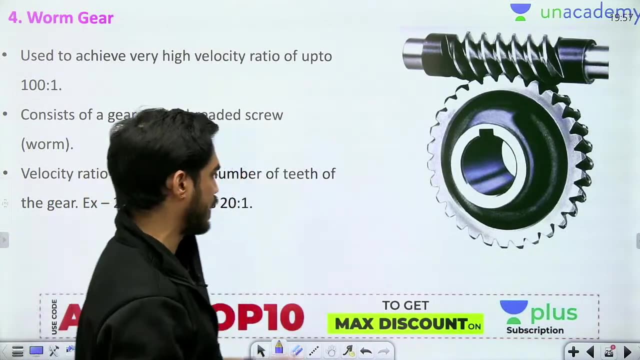 In case of spur gear you will have 6 ratio 1. In bevel gear it is mostly 3 ratio, 1. Okay, So maximum to maximum you can get 10 ratio 1. Why son? Because the velocity ratio is inversely proportional to ratio of diameter. 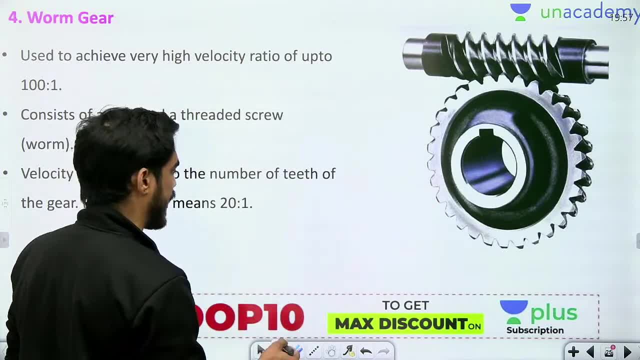 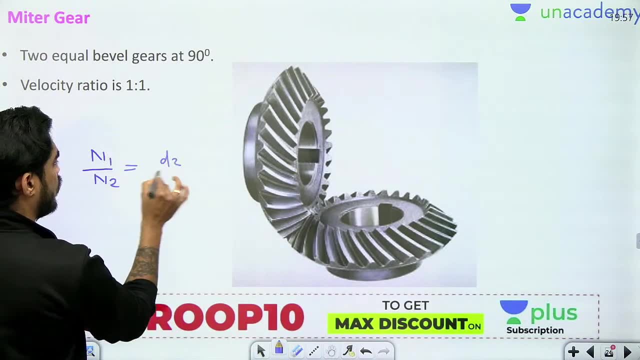 I will prove this. Okay, I will tell you how it happens in future. But son velocity ratio is inversely proportional to diameter. N1 by N2 is equal to D2 by D1.. So, son, if D1 is equal to D2.. 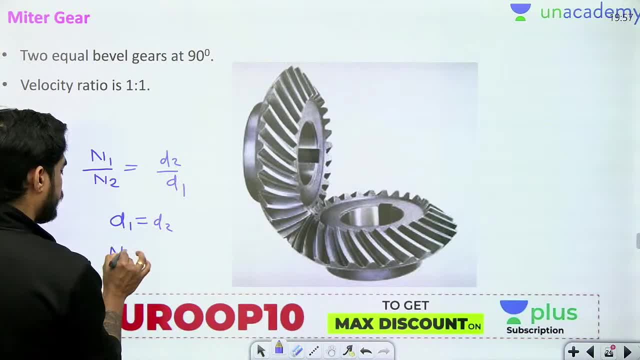 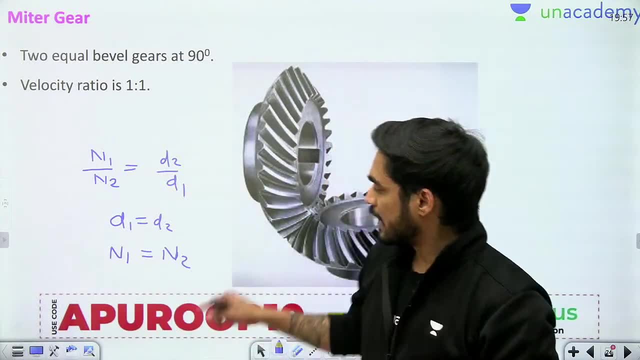 N1 is equal to N2. Isn't it? That's why 1 ratio 1 is coming here. Now, my brother, Imagine if I need 10 ratio 1.. Then, son, what will be the ratio of their diameter? 10 ratio 1 only. 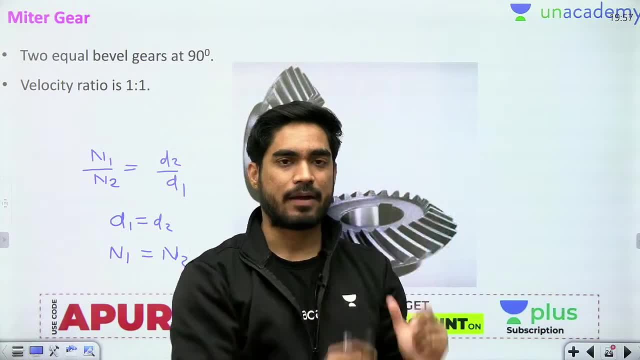 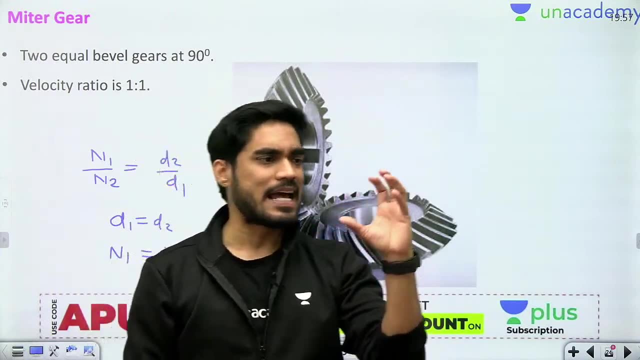 Means. if one is having a diameter of 10 mm, Other one is having a diameter of 100 mm. Thank you so much, Ankit. Thank you so much, Ankit. Okay, So my brother, One's diameter is 10 mm and other's is 100 mm. 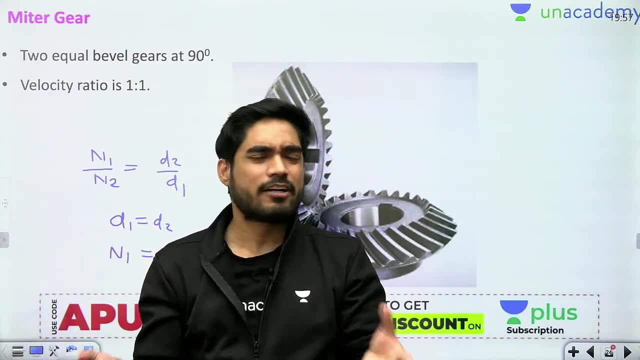 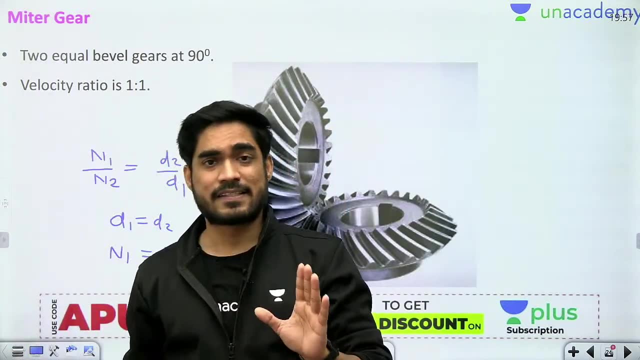 So practically, will it be very feasible? No, It will not be a feasible solution. Right One is 10 mm, Another one is 100 mm. But, son, this is maximum. If you need 50 ratio 1. Then can you imagine what will be the size of the gear. 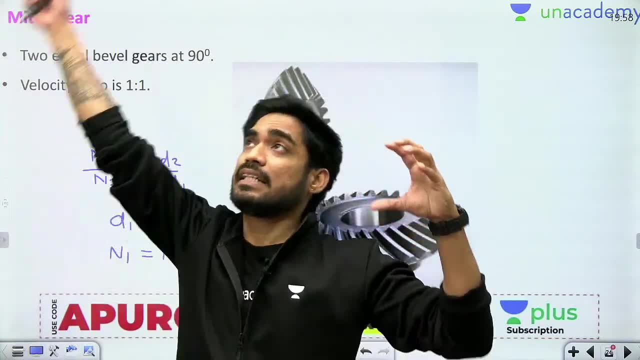 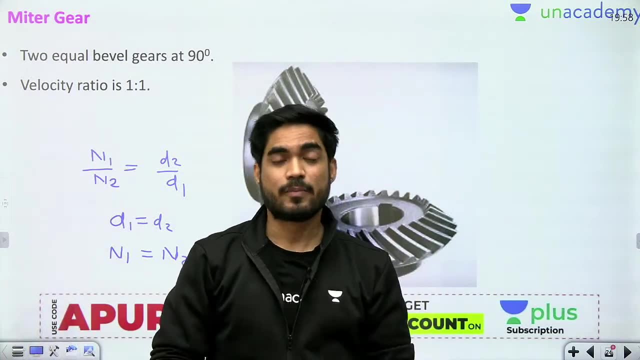 If one is 10 ratio 1., Another will be 5.. Sorry, If one is 10 mm, Another will be 500 mm. If I need 50 ratio, 1.. So, son, that's why, If you need very high velocity ratio, 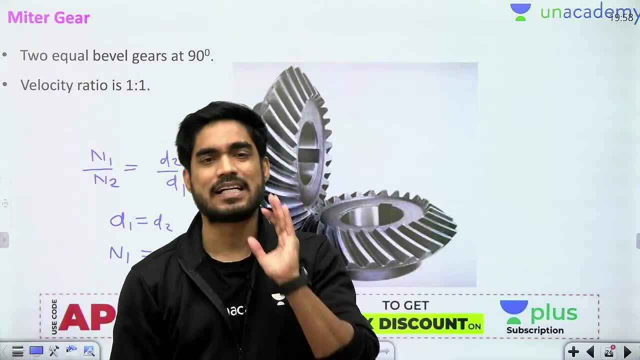 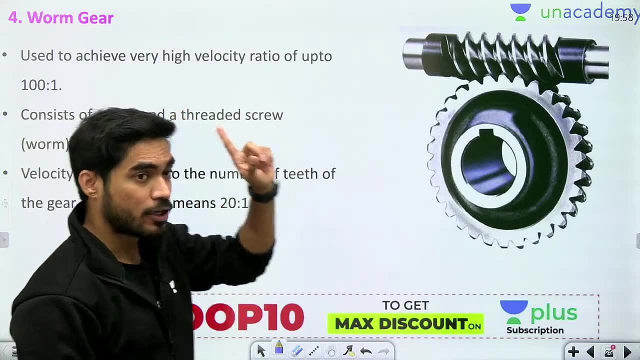 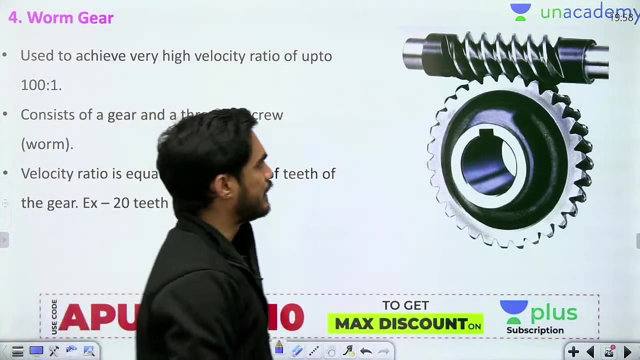 Then you need to use special type of arrangement Known as Known as worm gear. Now, what do we mean by worm gear? Understand What is worm gear. Pay attention. Okay, In case of worm gear, There is a screw Which is in contact with the gear. 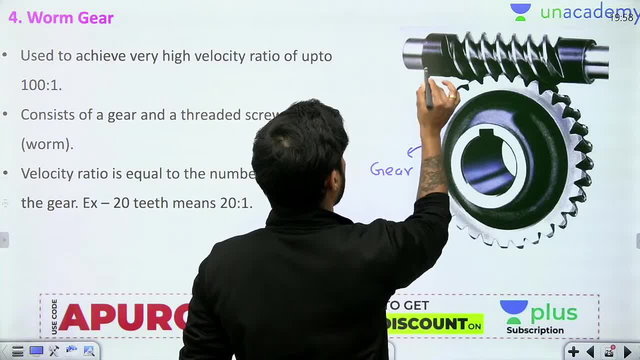 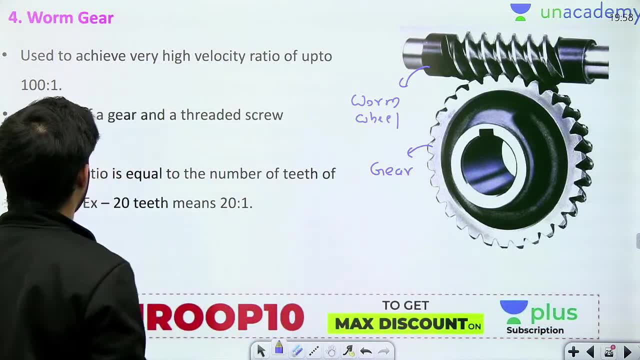 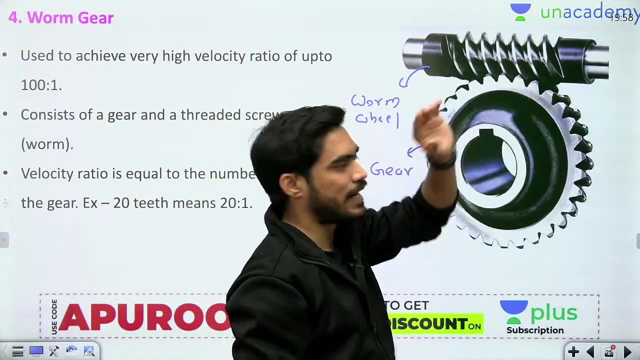 Okay, This is my gear And this is my screw, Which is known as Worm wheel. Okay, This is my gear And this is my screw, Which is known as worm wheel. Okay, This is a threaded screw, a threaded screw. This is a screw which has threads, So these threads are in contact with 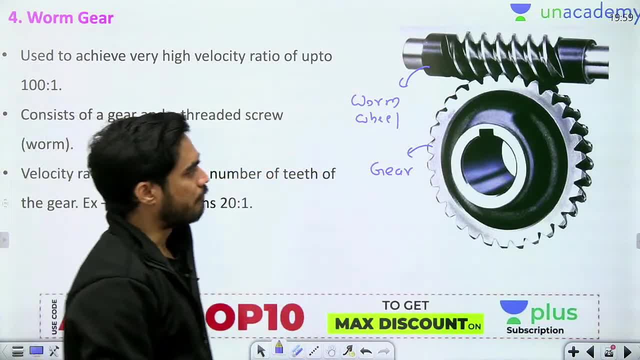 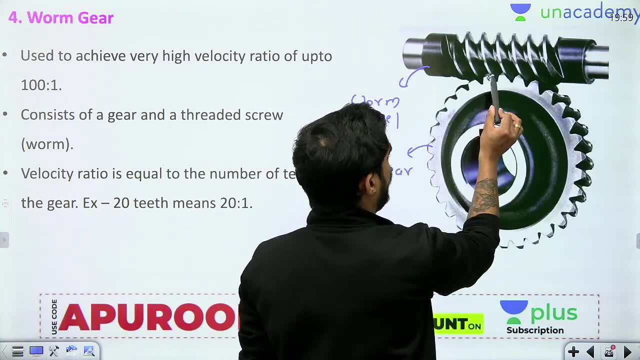 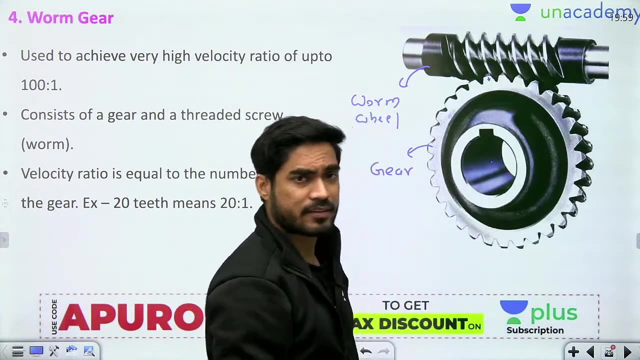 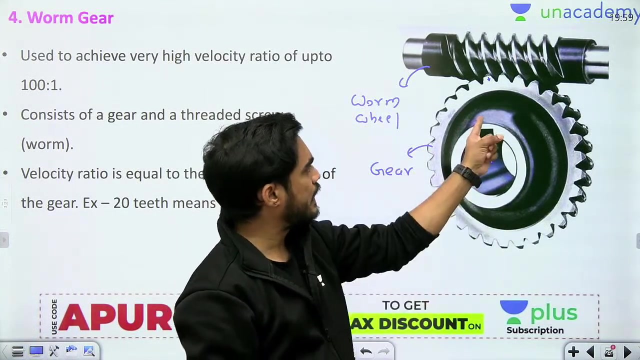 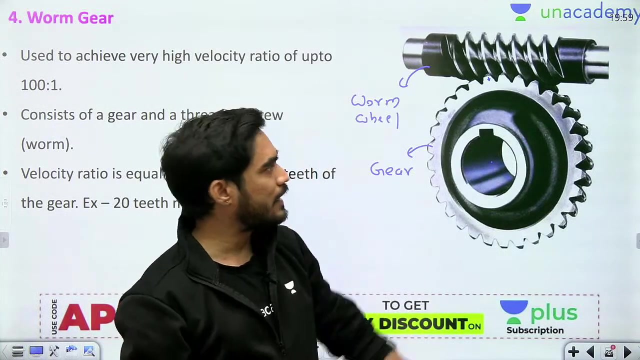 the gear. Now understand what is happening. When this gear will rotate, if one tooth of this gear will move forward. if one tooth, if one tooth moves forward, then this screw will rotate. one complete revolution. If one tooth of this gear advances, then the screw will make one. 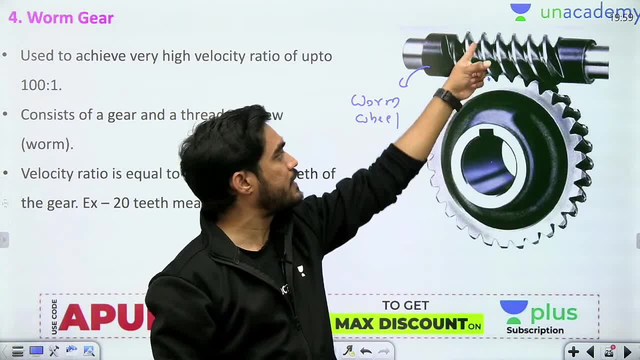 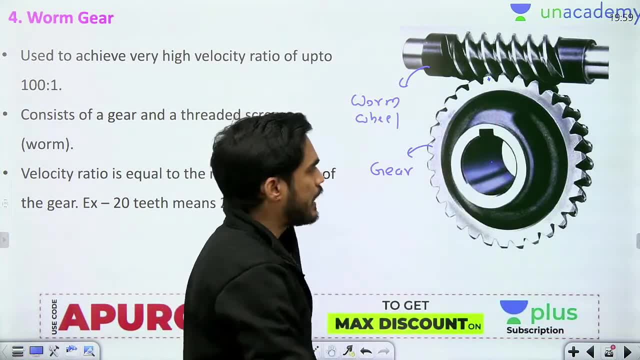 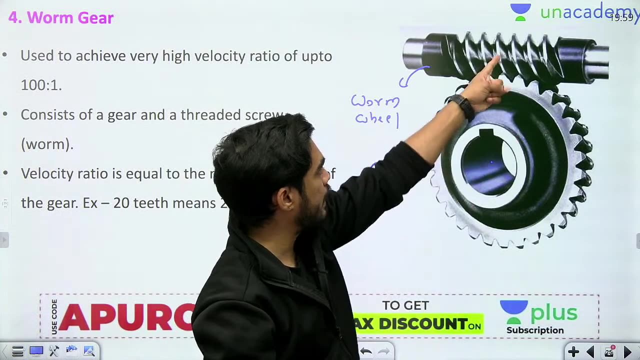 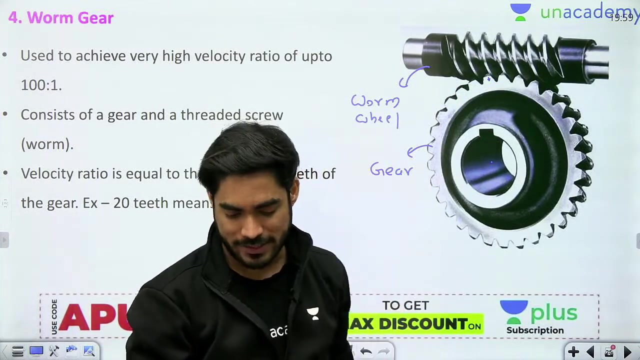 complete revolution. So if it has 50 teeth, if the gear has 50 teeth, then for one revolution of gear, for one complete revolution of gear, how many revolutions the screw will make? How many revolutions the screw will make? The screw will make 50 revolutions, right, The screw will make 50 revolutions. So that means 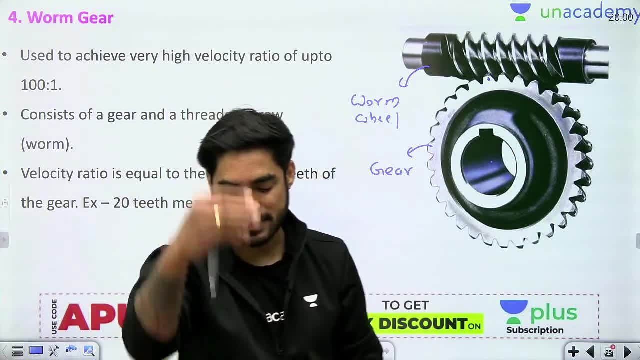 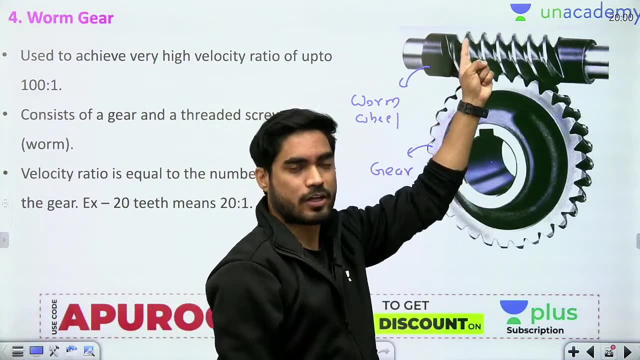 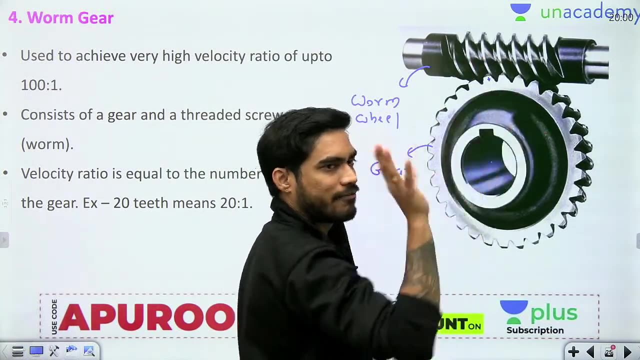 I will get 50 ratio, 1 velocity ratio. Thank you so much, Manoj. Thank you so much, beta. So, beta, do you understand how we can get very high velocity ratio using screw- sorry, warm gear? In case of warm gear, if one tooth of gear advances, the screw will rotate. 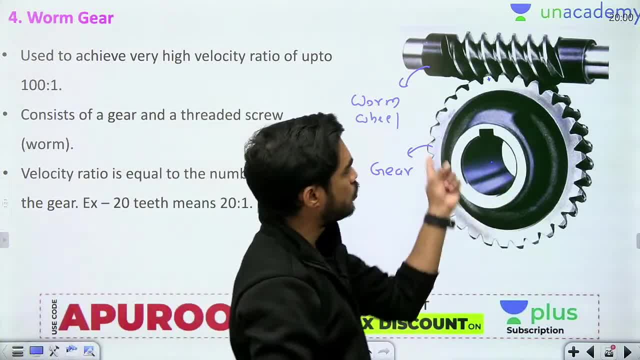 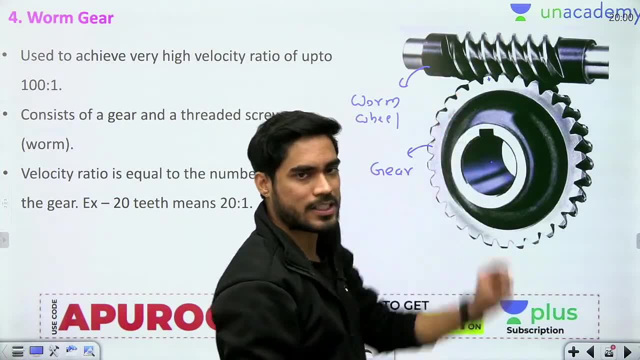 one complete revolution. okay, So if the entire tooth of gear will advance, if one complete revolution of gear is there, then 50 teeth means 50 ratio, 1 velocity ratio. If you want to understand how it is going to work- beta- you can just google it and you see a video. 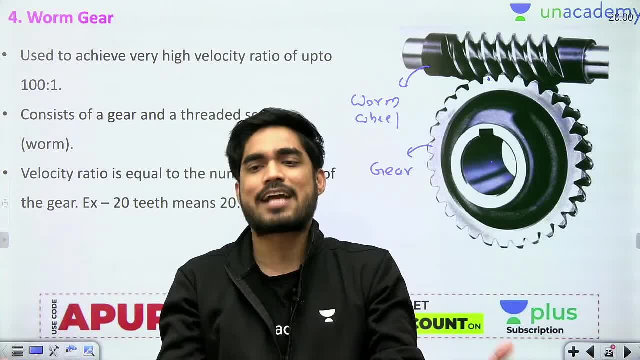 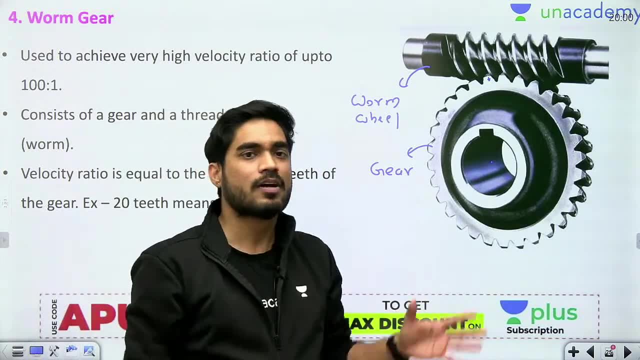 Pick up any video and watch it, you will understand. Okay, Here crash course is going on. There is not much time to show and explain everyone's video. That's why beta I will not be able to show the video and then. 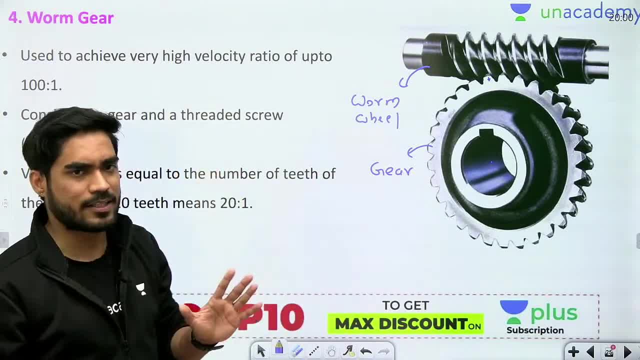 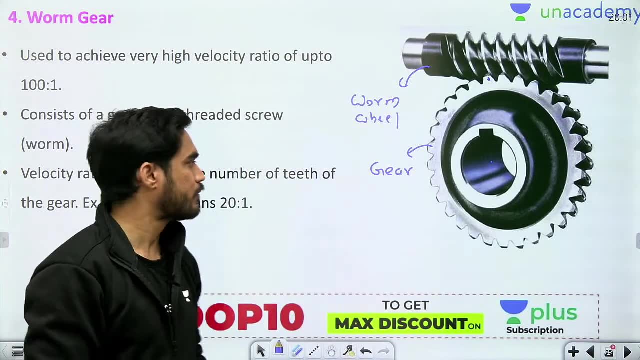 So, beta, if you want to understand how it works, how it works, then google it. Okay, Google it. It is important to make some effort from your side, my brother. Okay, So, beta, do you understand how it works? So if the teeth of gear is 50, then the velocity ratio: 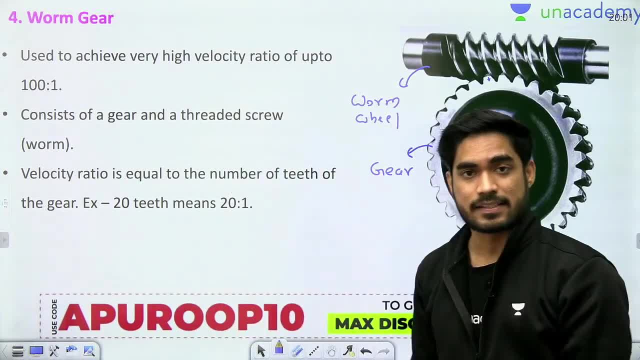 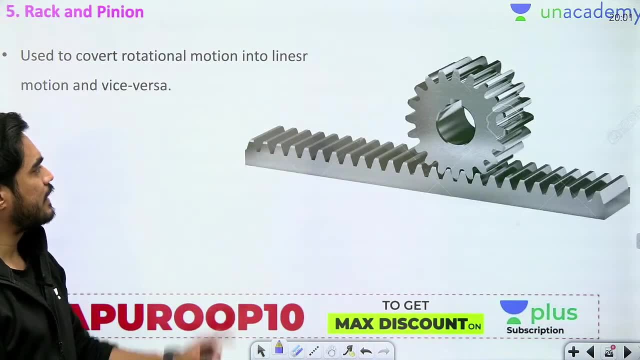 will become 50 ratio, 1.. Okay, So you might get question like this: If we need very high velocity ratio, which gear do we use? So we use warm gear, Okay. Next is rack and pinion arrangement. So you can see that we have a rack and pinion arrangement, So you can. 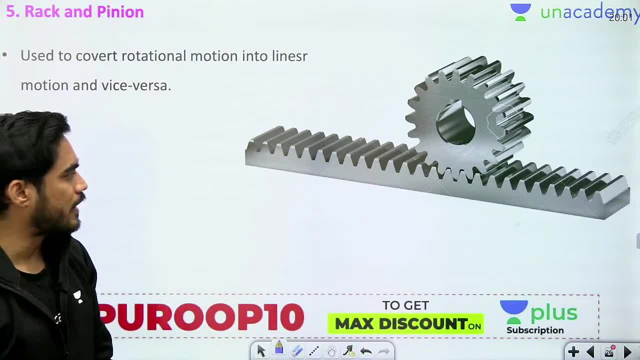 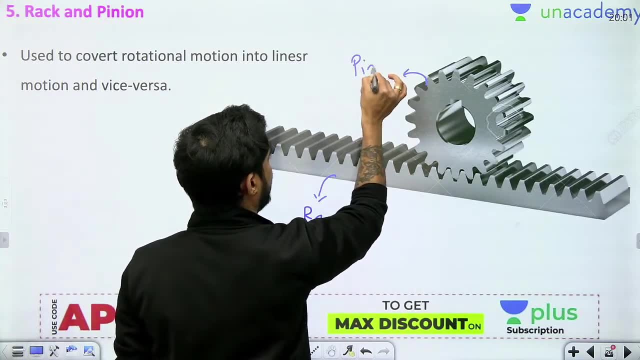 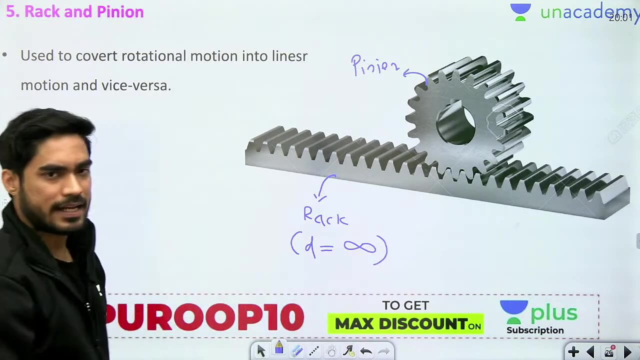 see from this diagram. only, what do we mean by rack and pinion? Right, This is known as rack, This is known as pinion. Both are spur gear. Both are spur gear, But the diameter of this rack is infinite. Right, This is a linear gear. You can see that this is a straight. 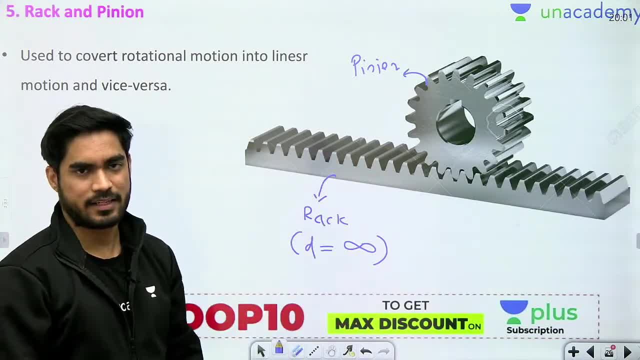 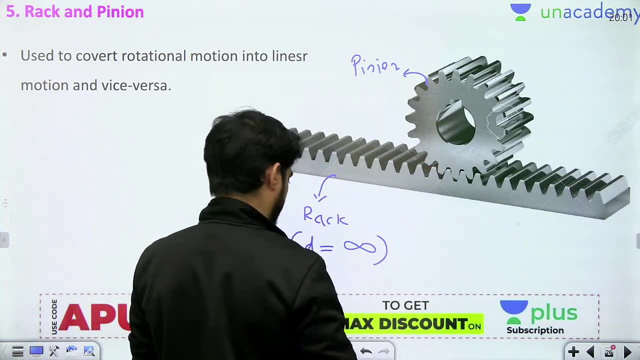 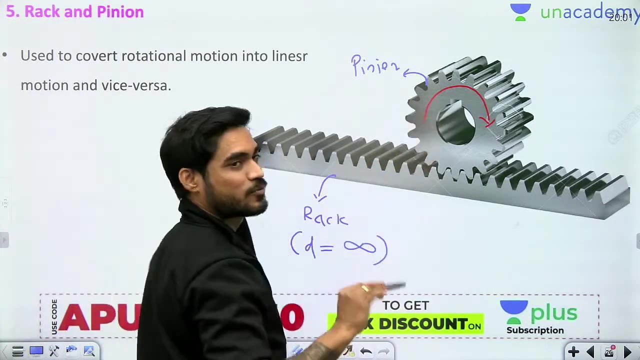 gear Means you can say that diameter is infinite. Okay, So beta, in case of rack and pinion arrangement, If this rack is moving, if this rack is making rotational motion, then this: sorry. if this pinion is making rotational motion, so sorry if the pinion is making rotational motion. 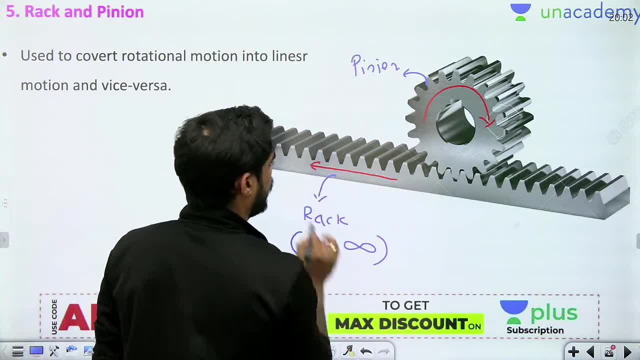 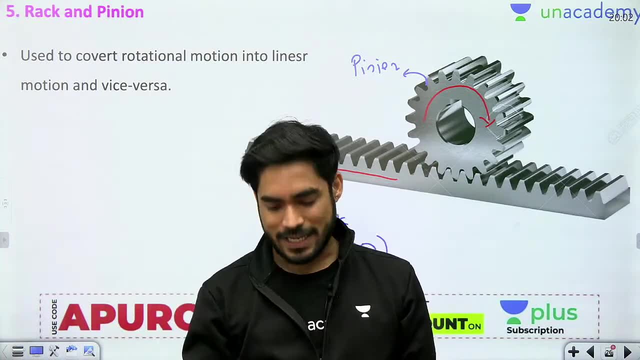 then the rack will make translational motion. So, beta, this type of arrangement is used to convert rotational motion into translational motion or translation motion into rotational motion. Okay, So, beta, if you want to do this type of motion conversion, then you need. 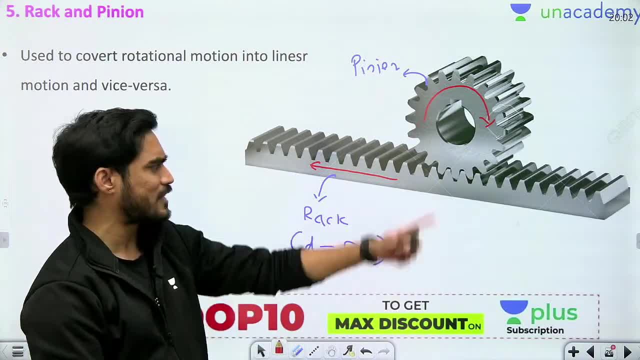 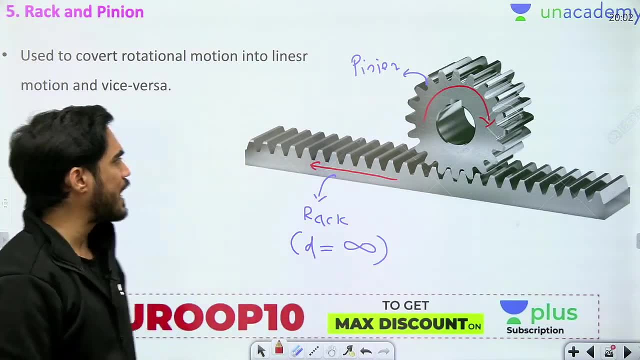 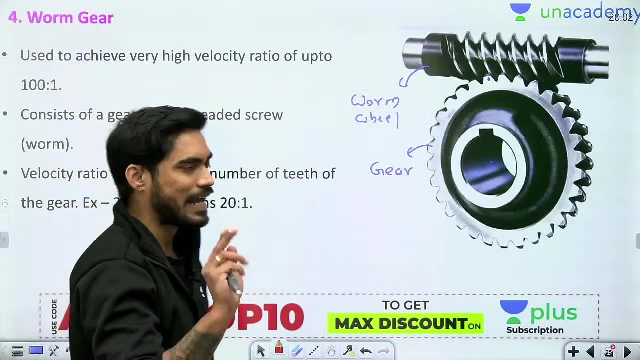 There we use rack and pinion arrangement. okay, Both are spur gears only, but this spur gear rack has infinite diameter, okay, So I hope that all of these types of gear is clear to you. You only need to remember these one or two points that I have mentioned. 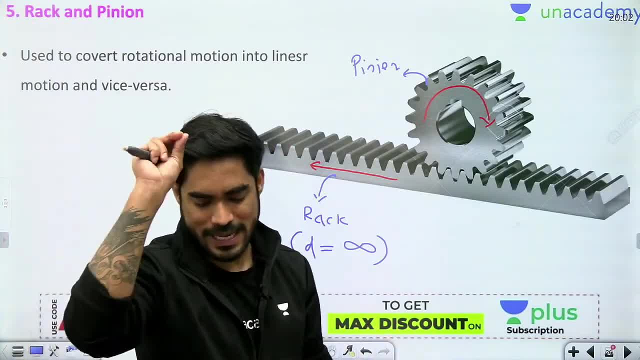 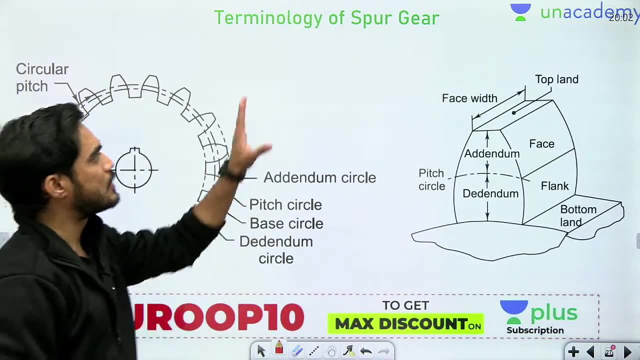 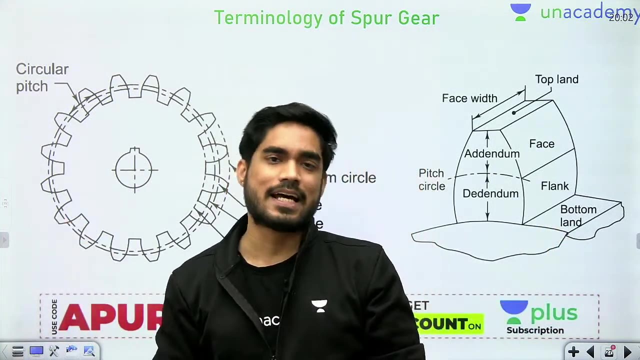 That's it. You don't have to go through the entire paragraph, you just have to remember these 1-2 important points, okay, Okay, now beta. let's move on to the spur gear design. Understand, beta. we have several types of gear, but out of all these gears, you only need to study the design of spur gear. 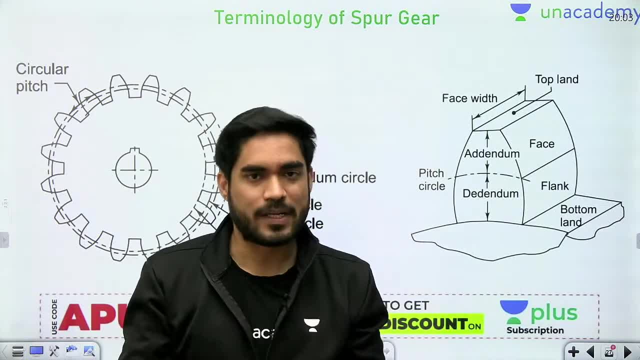 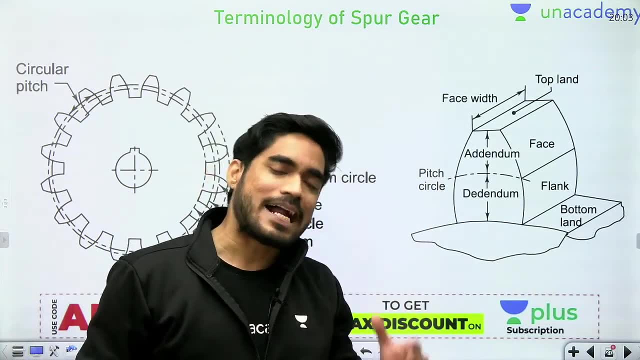 It is not mentioned in the book, but beta years of experience have taught us that what exactly is in the spur gear and from which topics you will get questions. So that's why, if I am telling you that there is only spur gear in your syllabus, please remember. 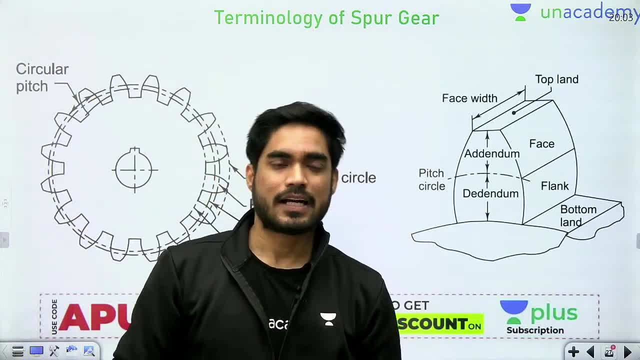 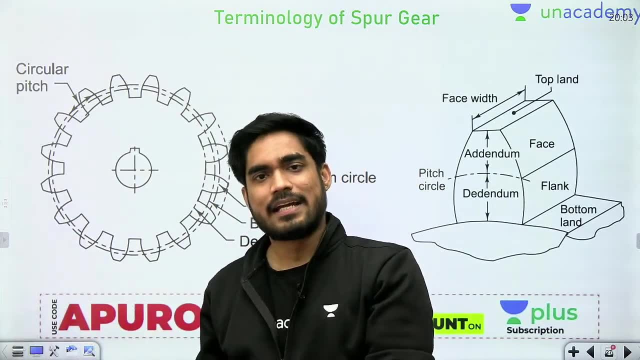 Trust me and just focus on spur gear. okay, If I am telling you, then I mean I have some experience, years of experience, by looking at so many questions, papers, by collecting data from them. after that I am coming in front of you. after that I am telling you. 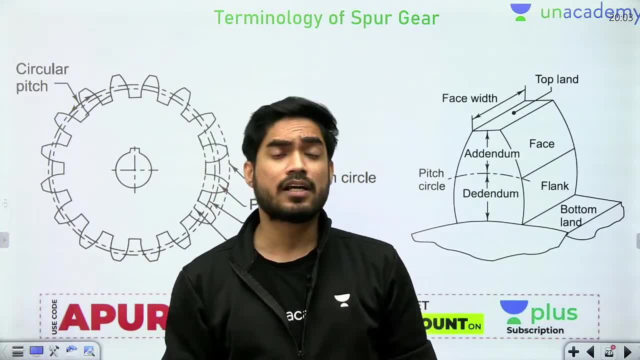 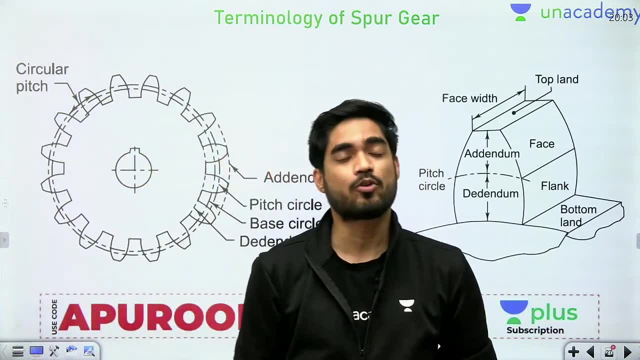 So that's why beta don't think that spur gear sir is teaching. helical gear sir will not know. There is nothing like that, my brother, if he didn't know then I would have studied in so many years. So you don't have to worry about the syllabus. I see, especially in machine design, children are very worried. 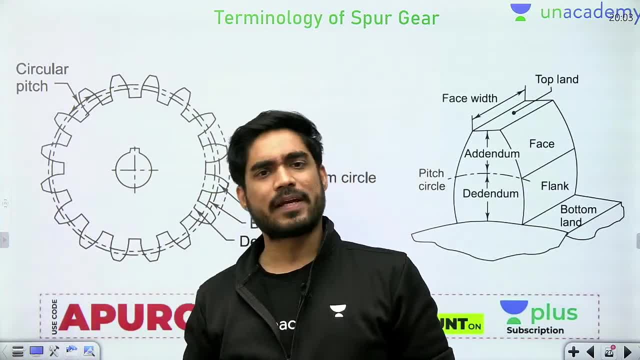 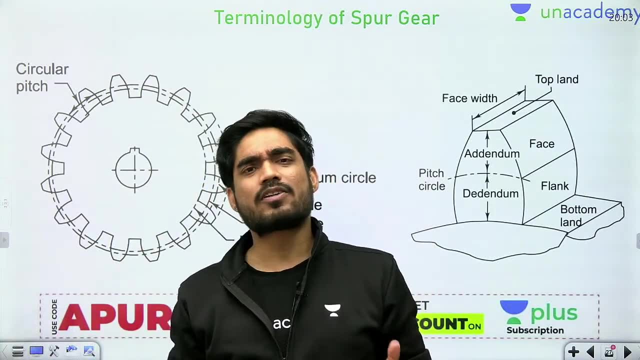 That sir didn't study, this sir didn't do this sir. why this topic, sir? this topic is there or not. So, my brother, simple, you don't have to worry. why are you taking so much tension? Why you are worried about the syllabus so much? 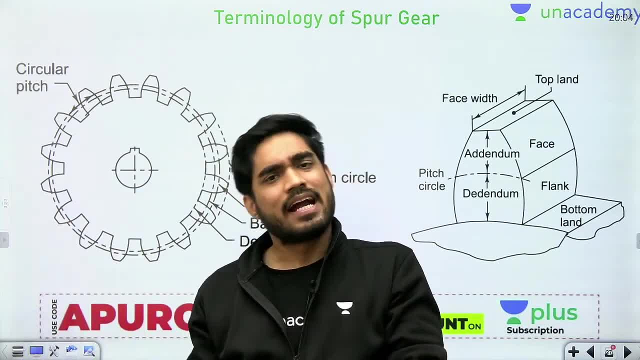 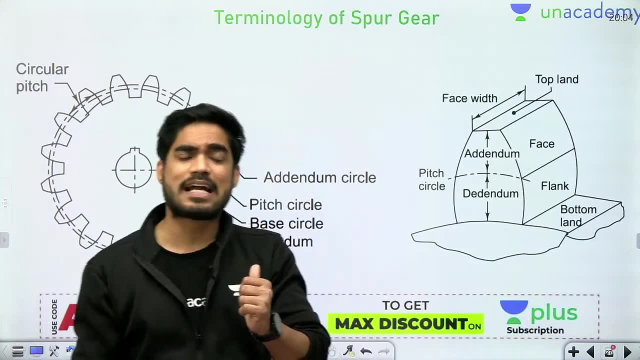 Whatever we are explaining here, that is only in the syllabus, right? And if there is any topic in the syllabus, then I will explain here. I will not skip that topic, okay? So if I am not explaining that topic, that means it is not in your syllabus. you will not get question from that topic, okay? 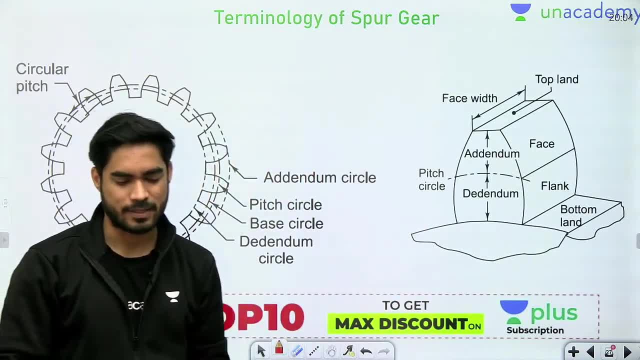 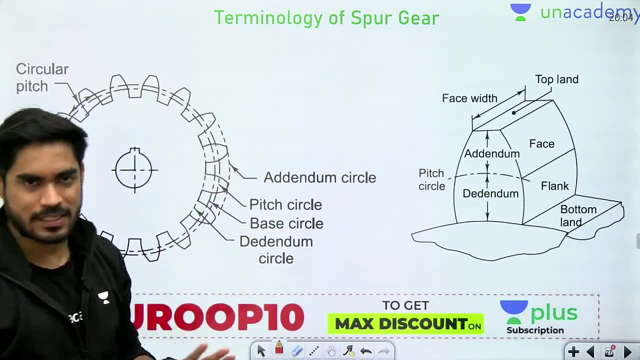 So trust me on that, You have spur gear design in your syllabus. okay, In your syllabus there is only spur gear design. So in spur gear, first of all, we understand the terminology. Let's first understand the terminology of spur gear: different parameters of spur gear- okay, 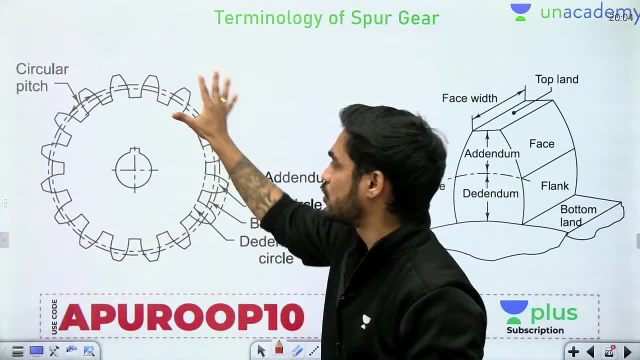 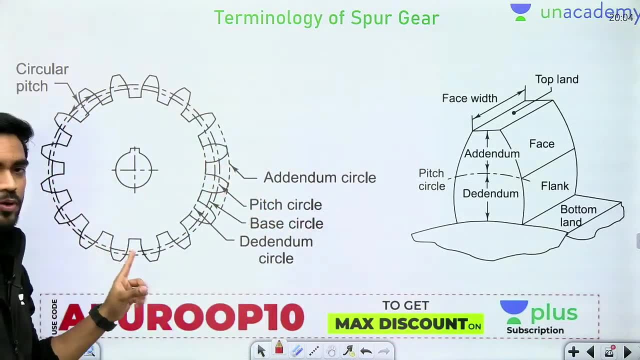 So I am showing you two diagrams. In this diagram the entire gear is shown, and in this diagram only one teeth is shown. okay, So let's first understand the parameters of this diagram. okay, So in this diagram you can see four types of circles. okay, 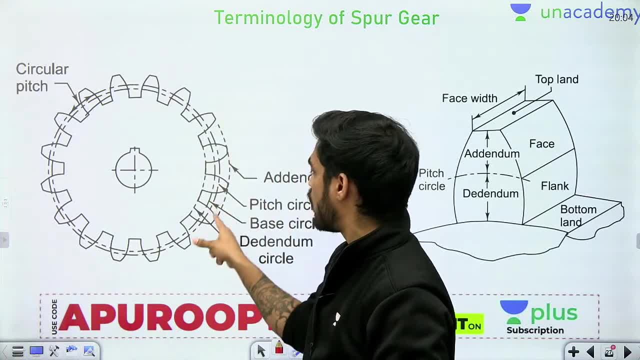 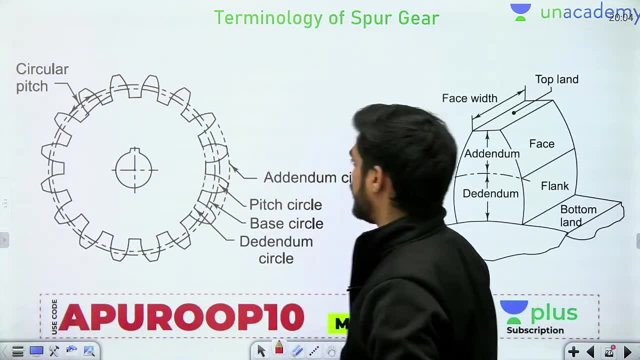 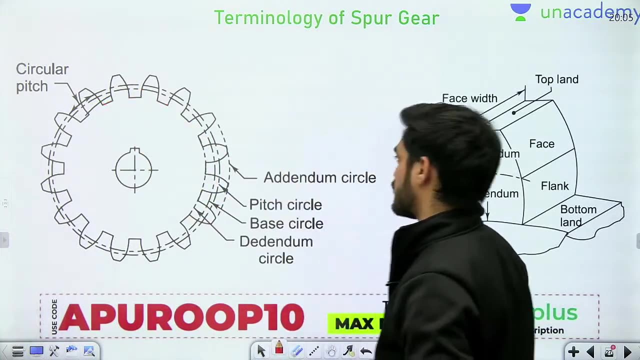 There is one circle which is passing from the top of the tooth, which is known as addendum circle. This circle, which is touching the top of the tooth, is known as addendum circle. Then there is one circle which is touching the bottom of the tooth. this is known as didendum circle. okay, 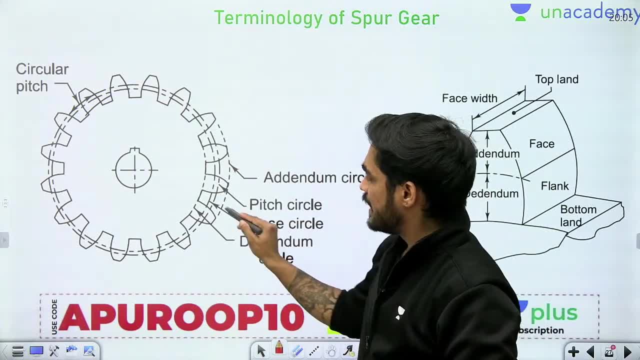 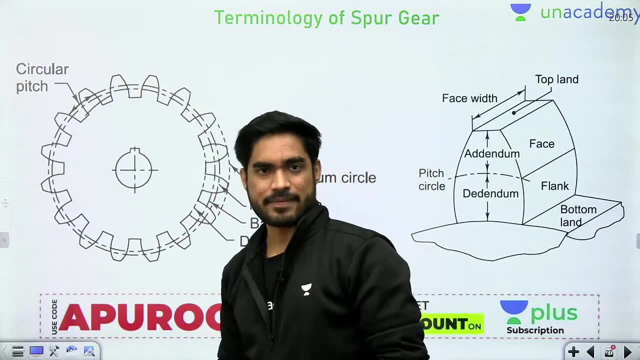 So addendum circle and didendum circle is clear. Then there is a base circle. Now, base circle you will understand when you will understand the type of teeth. okay, And that is not in our syllabus of machine design. 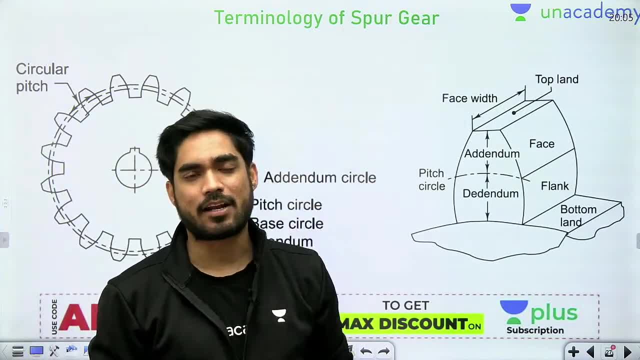 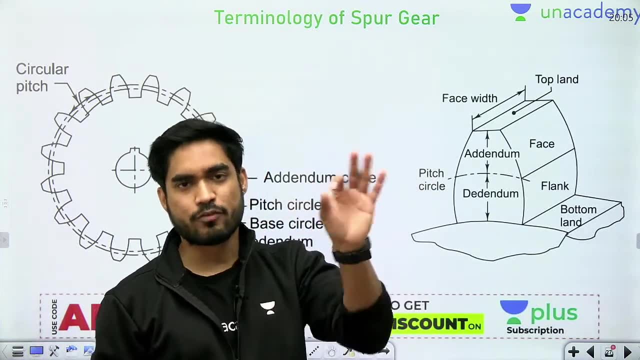 If you want to understand the type of teeth, you can go to see my lecture of theory of machines. So in theory of machine, I have explained the different types of teeth: involute, cycloidal. So if you want to understand base circle, it is something to do with the manufacturing of gear. 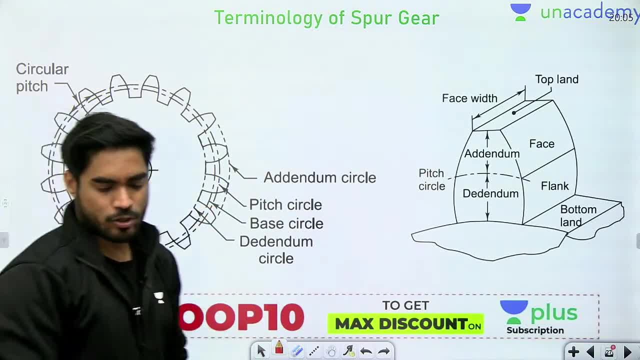 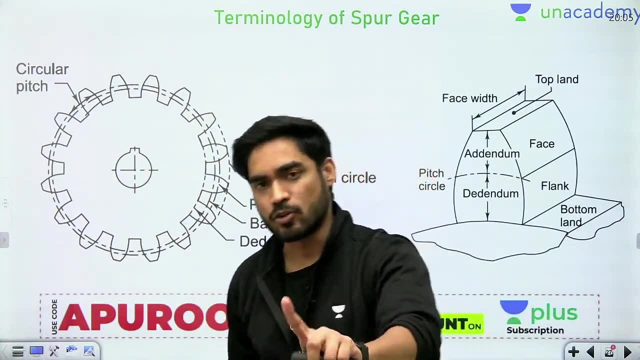 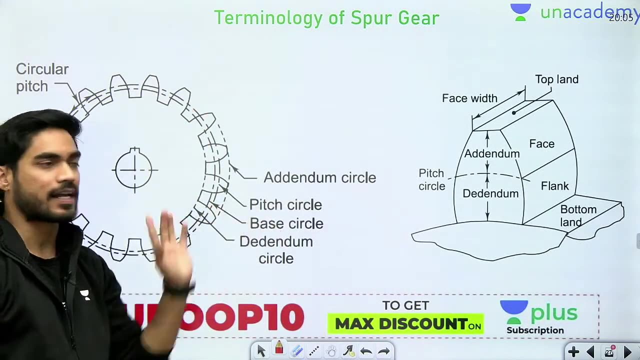 Base circle has to do with manufacturing. So when manufacture gear is cast then we bring this base circle in the picture. Then we understand the base circle, So you don't have to talk about base circle also. So the most important circle here for us in machine design is pitch circle. 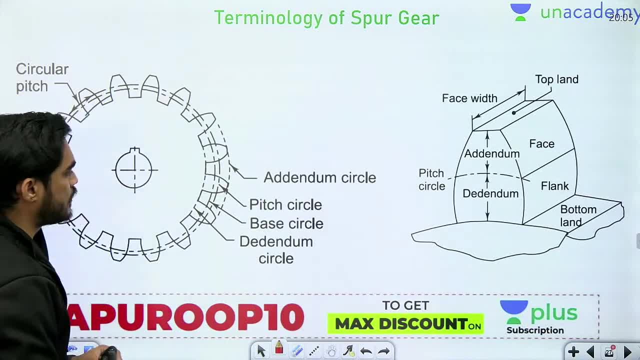 Now what do we mean by pitch circle? Understand, First of all. this pitch circle is between the addendum and addendum. This is the pitch circle. This is between the addendum and addendum and it is just an imaginary circle. 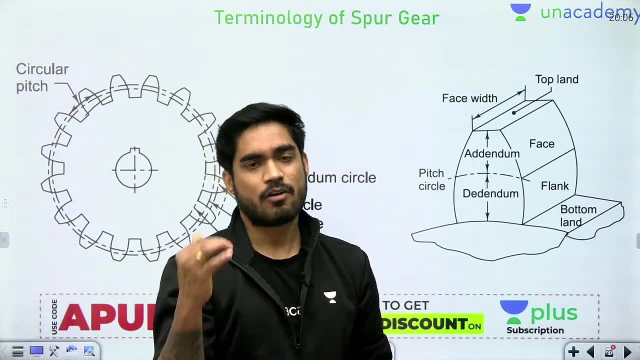 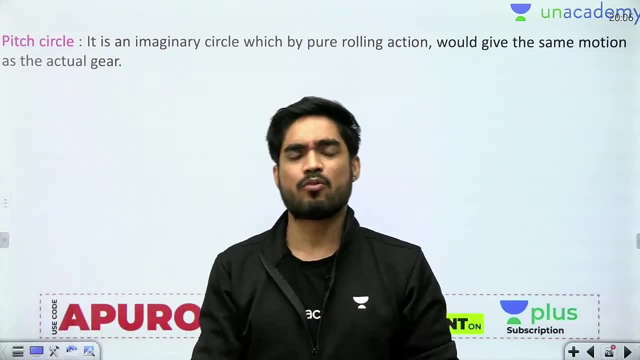 It is not exactly there. It is just an imaginary circle. Now, what is pitch circle? Let's understand. So, Bida, when we study the motion of gear, when we study the motion of gear, we assume that the gears are like two cylinders. 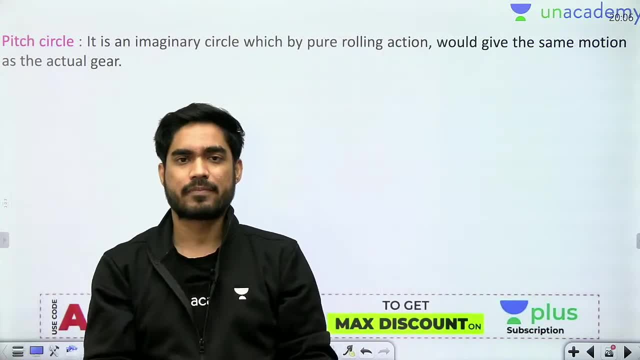 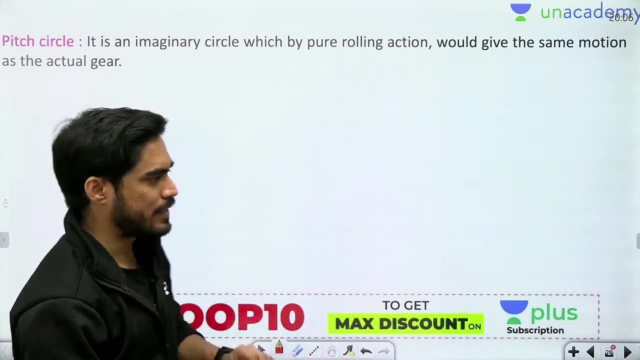 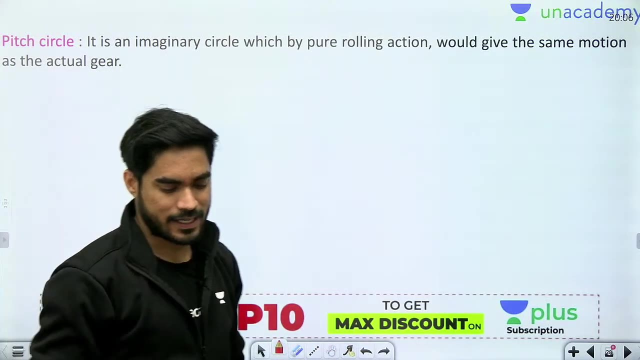 which are rolling over each other without slipping. And when you show these cylinders on a 2D plane, then these cylinders will look like circles. If I show the cylinder in plane, it will look like a circle, So these circles will be known as pitch circle. 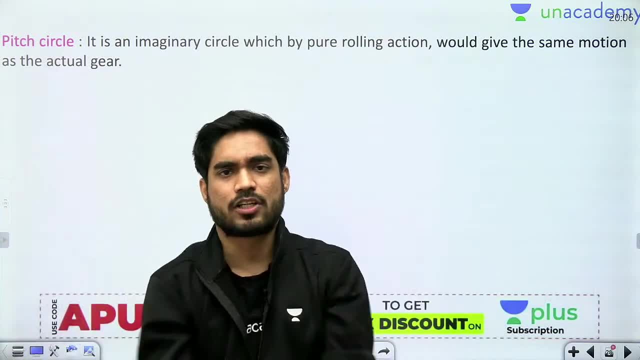 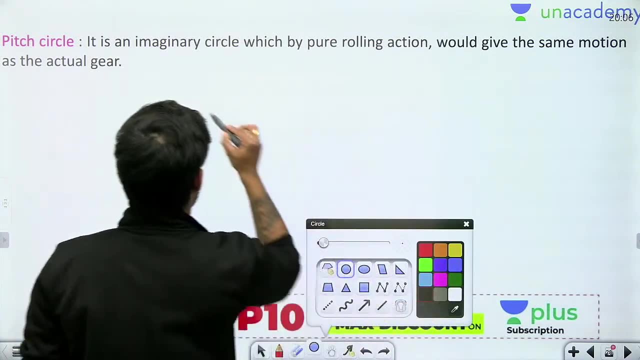 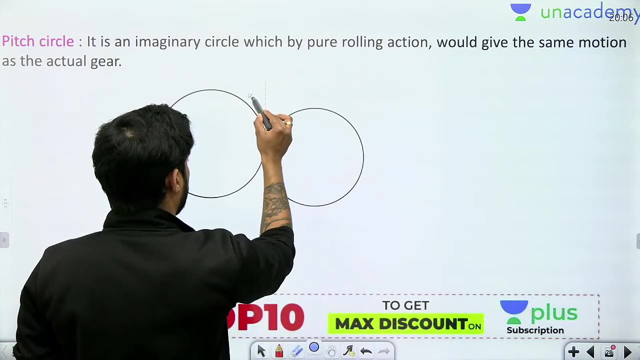 So what is pitch circle? If you want to study the motion of gear, you represent the gear using two circles. You represent the gears with two circles like this. You saw that diagram I have drawn right. You saw that diagram which I had just made. 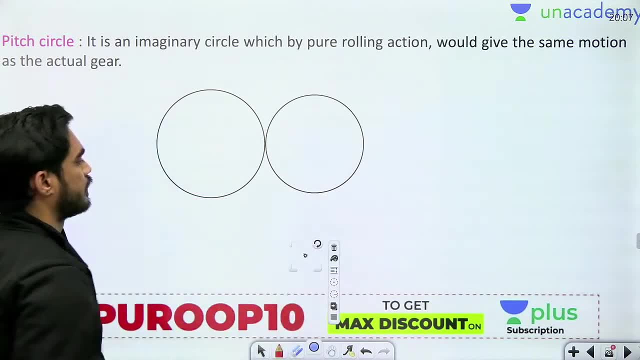 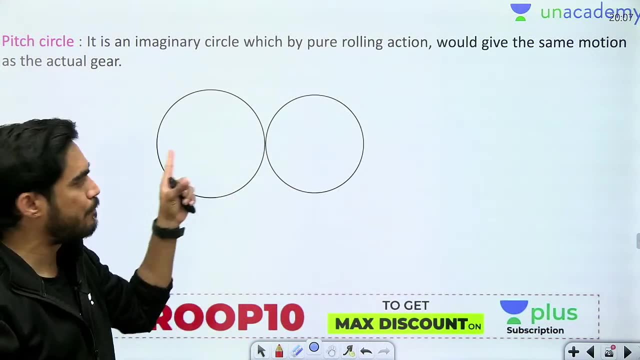 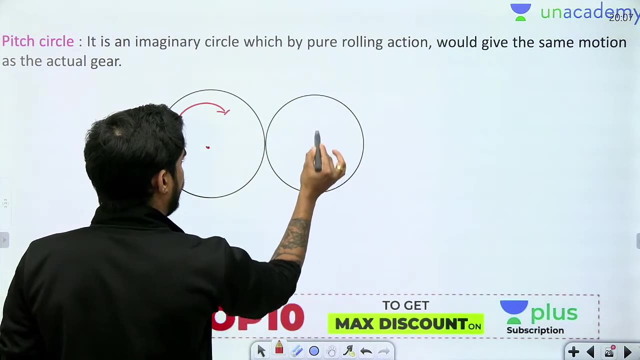 So, Bida, this is what These are: two gears in contact with each other. So if I want to study the motion of the gears, I will represent them as two circles, and I will assume that these two circles are rolling over each other without slipping. 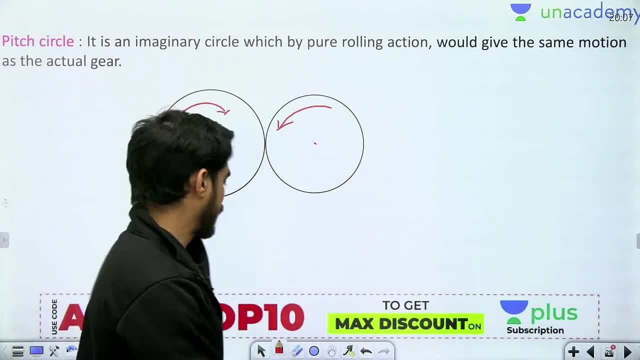 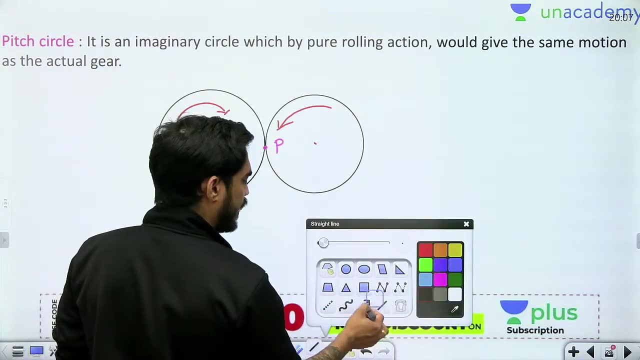 They are rolling over each other without slipping. Let's say: this is the point of contact. Let's say this is the point of contact P. So, Bida, at point P, the relative velocity will be zero. What do we mean by relative velocity? 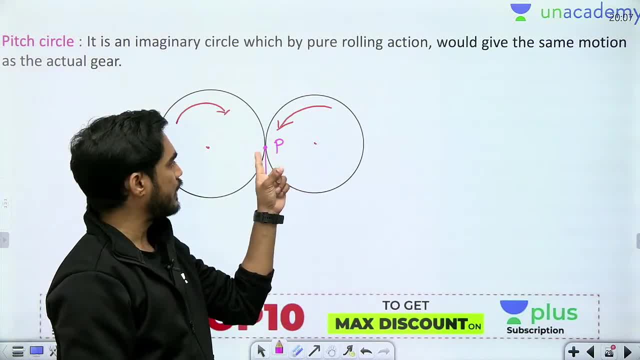 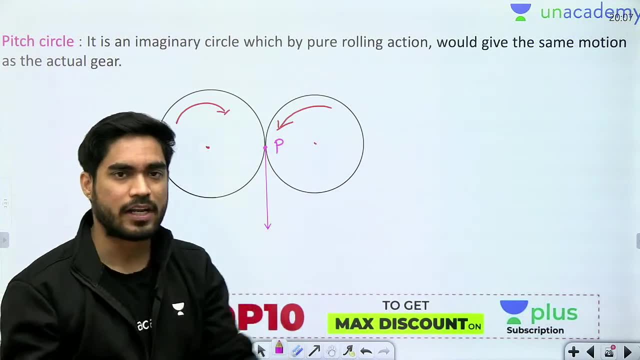 Relative velocity means difference in velocity at these points of two gears. This is a common point for both the gears, right? So, Bida, if the two gears are rolling without slipping, then the relative velocity at point P must be zero. 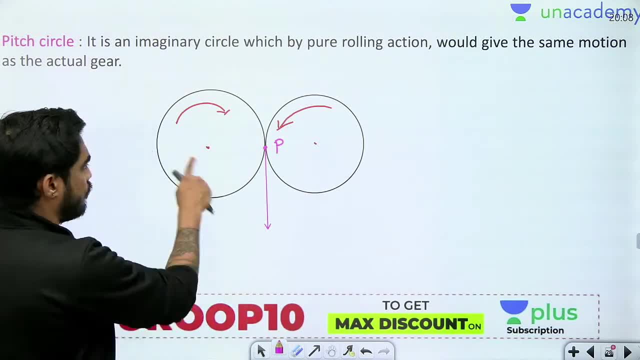 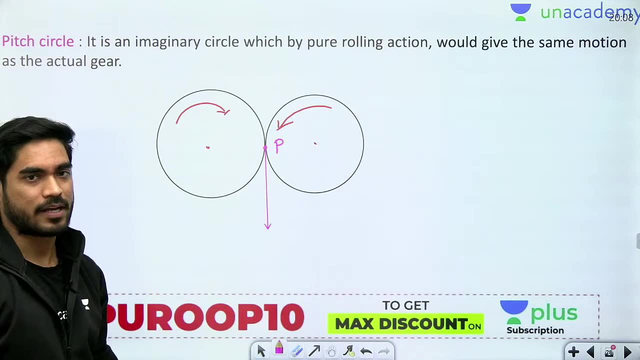 And relative velocity is zero means whatever velocity this first gear will have, second gear will also have the same velocity. Second gear will also have the same velocity. Okay, Now Bida. the diameter of the pitch circle is known as pitch circle diameter. 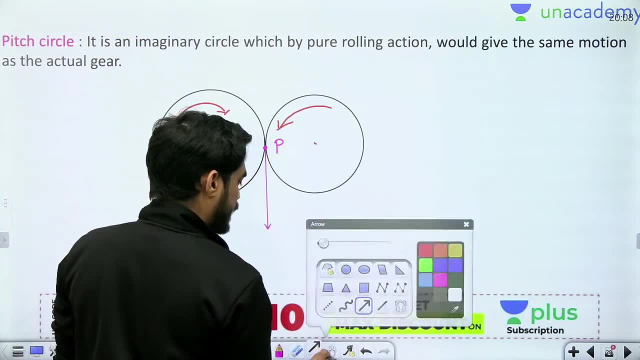 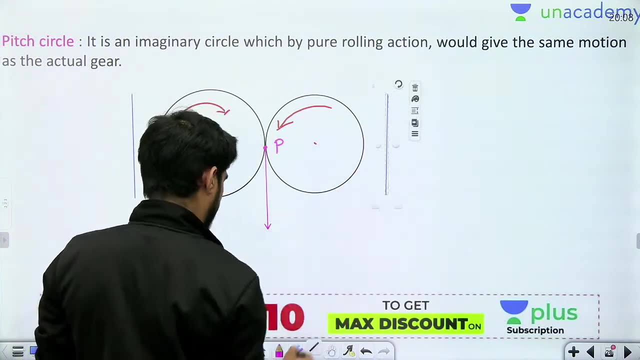 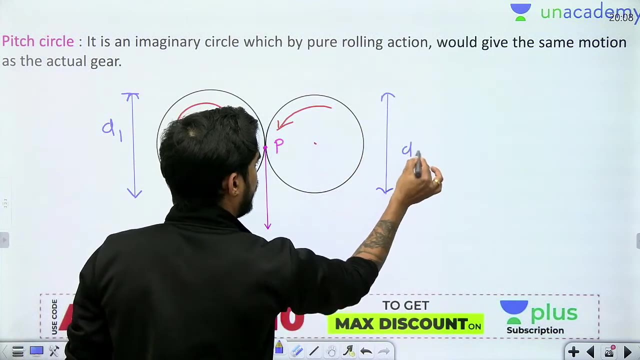 Okay, The diameter of the pitch circle is known as pitch circle diameter. So let's say the diameter of this circle is D1 and the diameter of this circle is D2.. Assume this is D1 and this is D2.. Okay, 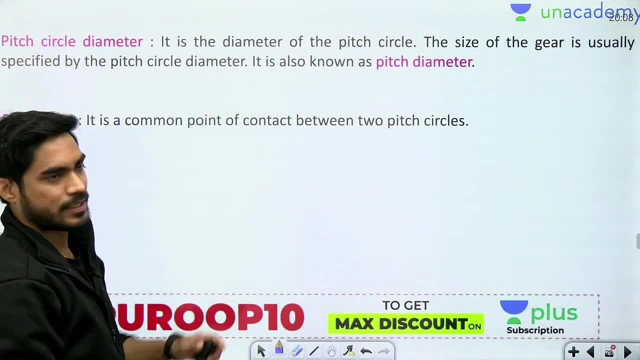 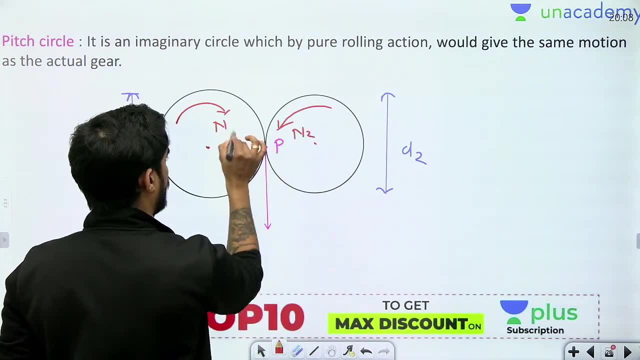 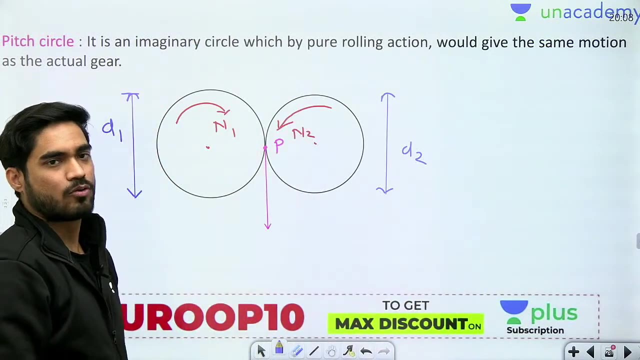 So do you understand? what is D1, D2? It is pitch circle diameter. Okay, Now let's say the speed of this is N1, the speed of this is this is N2.. Okay, So Bida, if the velocity at point P is equal. 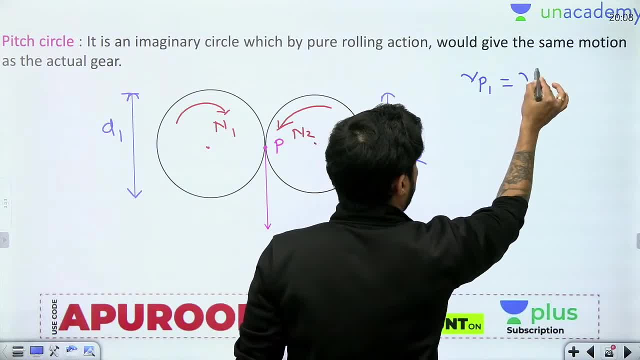 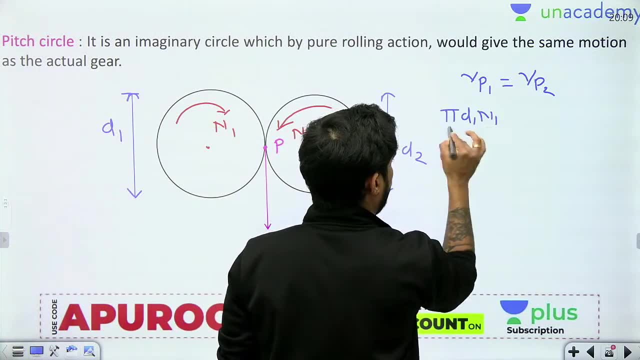 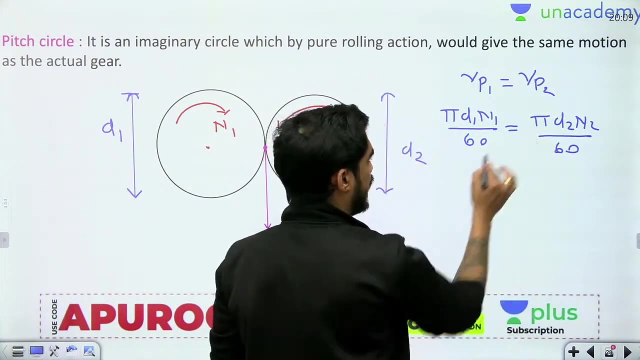 means Vp of 1 is equal to Vp of 2, a velocity at point P can be written like this: pi D1 N1 by 60 equals to pi D2 N2 by 60. So from here can I write it: 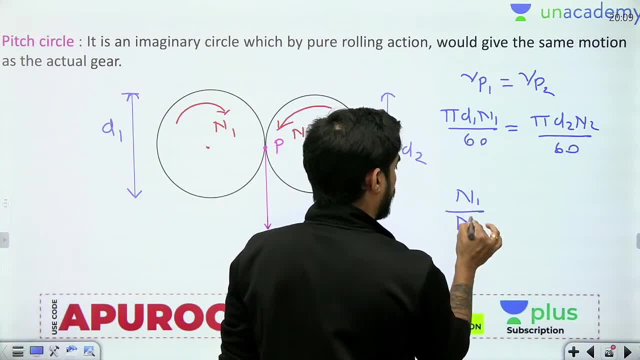 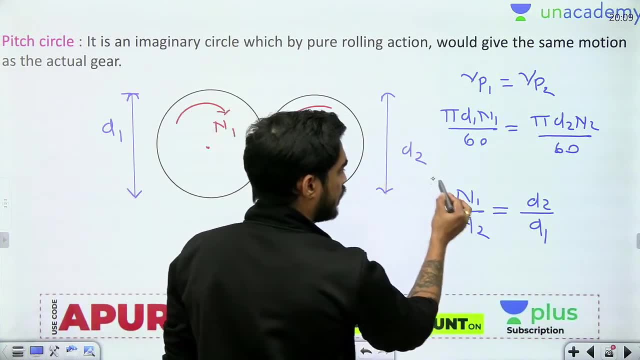 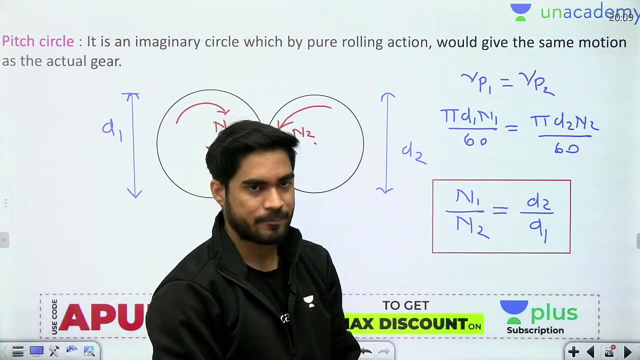 can I write it: N1 by N2 equals to D2 by D1.. What is N1 by N2? It is the velocity ratio. So ratio of velocity is inversely proportional to ratio of pitch circle diameter. N1 by N2 equal to D2 by D1. 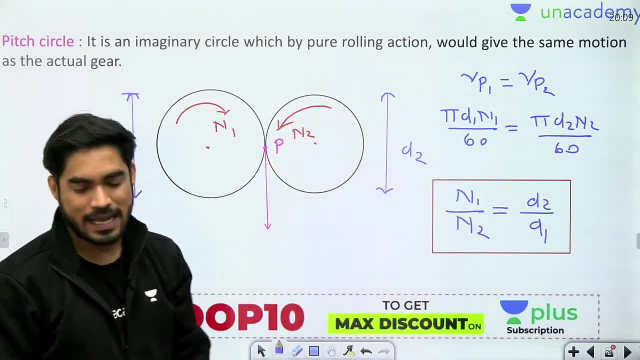 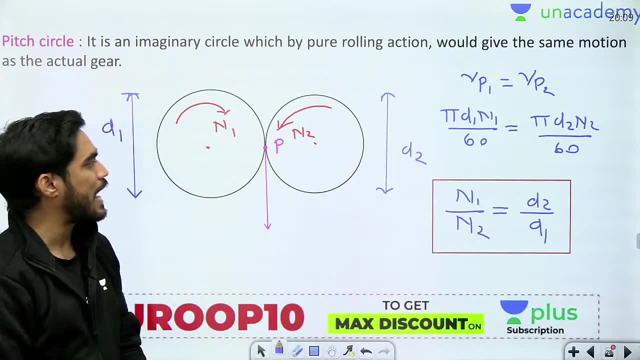 Is this clear to you guys? Is this point clear, my brother? I told you that I will explain where it is coming from. So it is coming from this assumption that pitch circle diameters roll on each other without slipping. And why are we taking this? 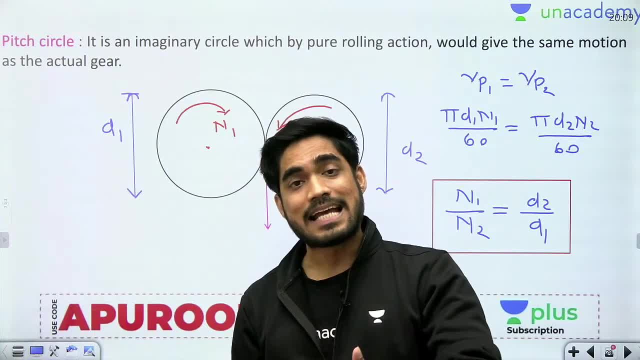 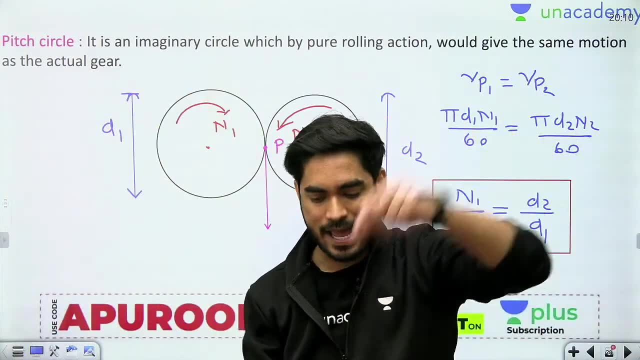 Why we are assuming these circles, So that we can analyze the motion of gear. We have to understand the motion of the gear, that how much force both the gears are applying on each other, what is the velocity, what is the acceleration. So for that we are assuming them as two circles. 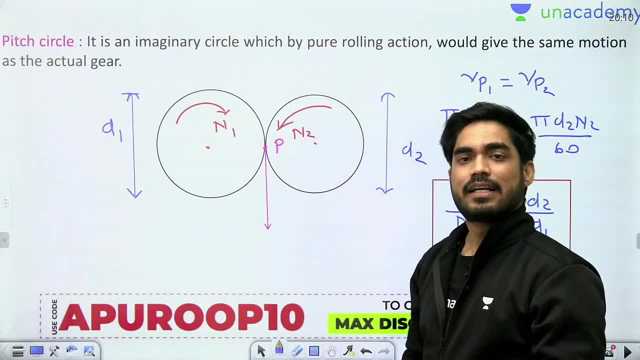 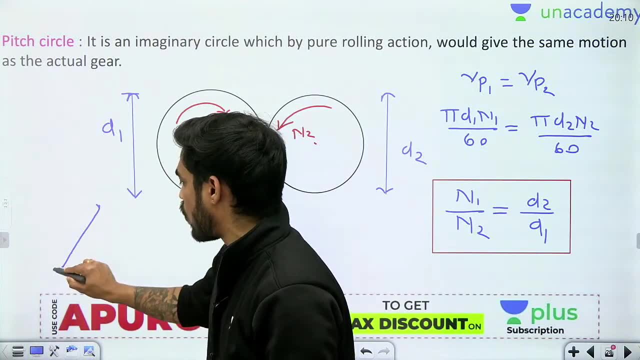 This is a kinematically equivalent diagram of gear. This is the kinematic diagram of the gear. Just like we are assuming solid diameter, we show these bodies with a link. we show them like a rod. we show them like this slider. 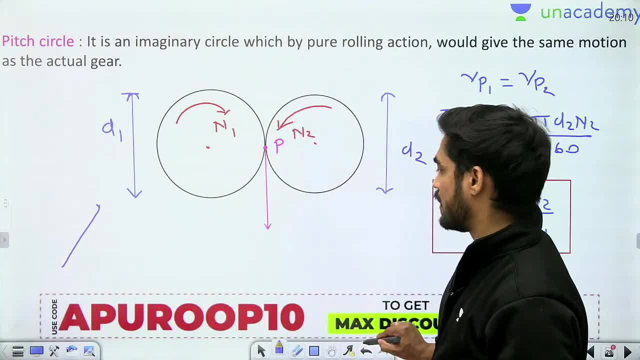 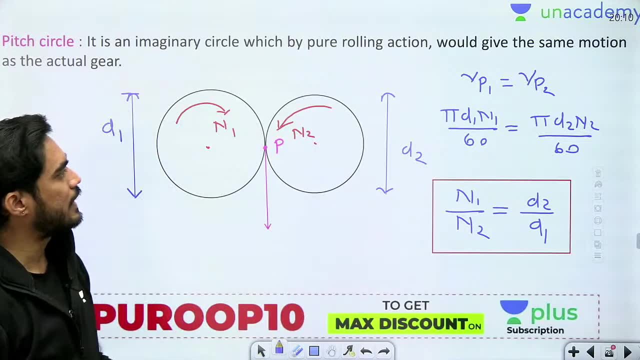 So this is what Kinematic diagram. So pitch circle diameter. pitch circle is a kinematic diagram of gear. It is a kinematic diagram of gear, So I hope pitch circle and pitch circle diameter is clear. What is pitch point? 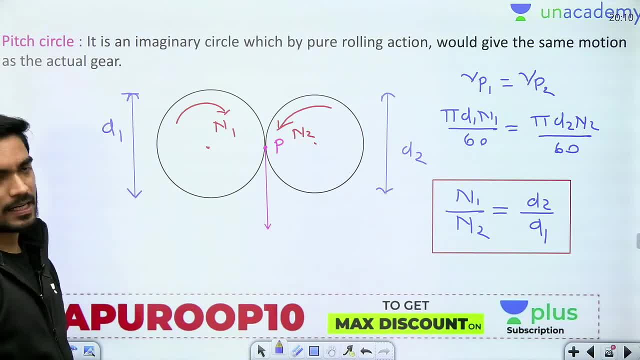 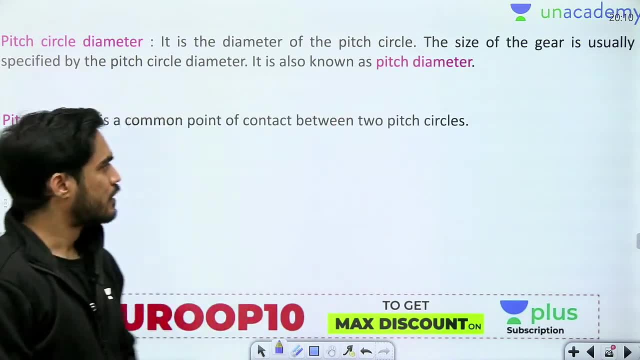 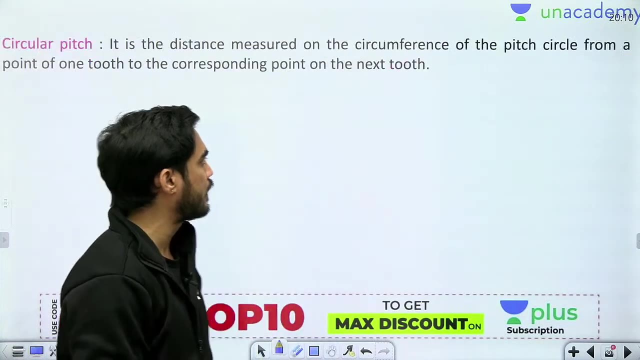 Pitch point is the point of contact of pitch circles, The point at which both the pitch circles come in contact. that is known as pitch point. So pitch circle, pitch circle diameter and pitch point is clear to everyone. Let's move on to the next topic. 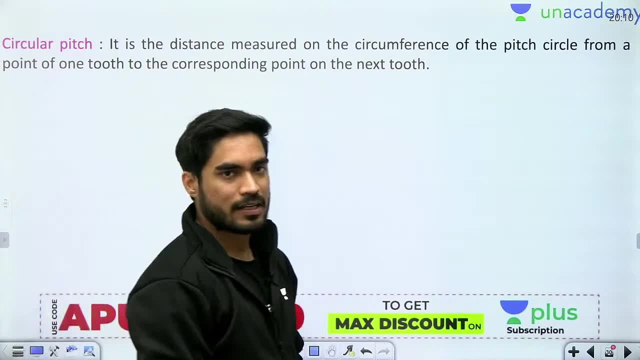 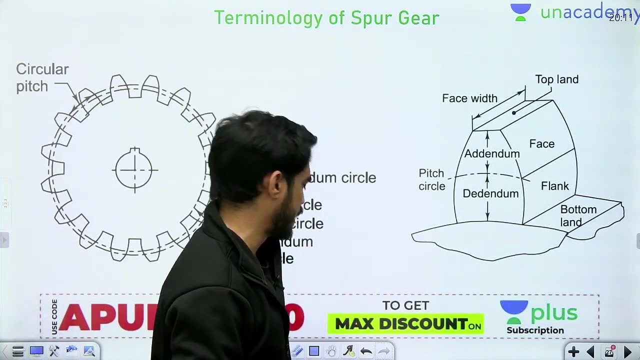 So the next point you need to understand is circular pitch. Now let's understand circular pitch. So let's come to teeth. Now let's understand different things in teeth. So if let's say this is the pitch circle, 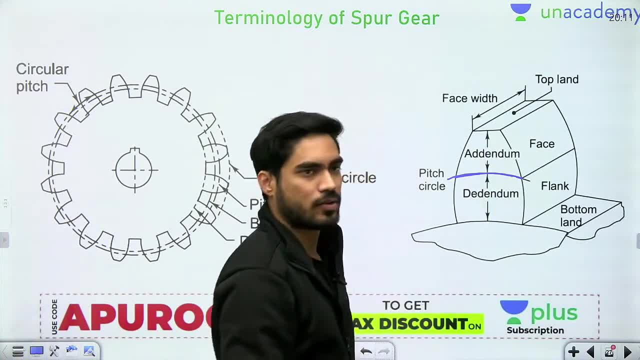 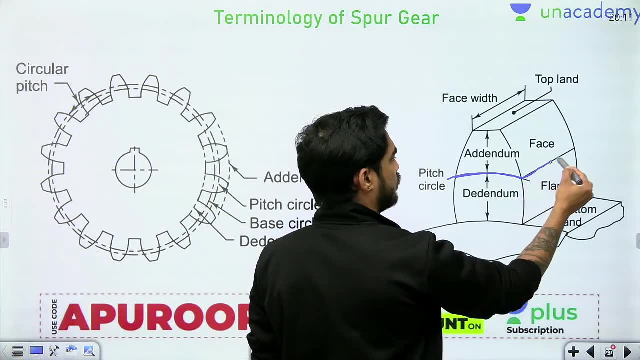 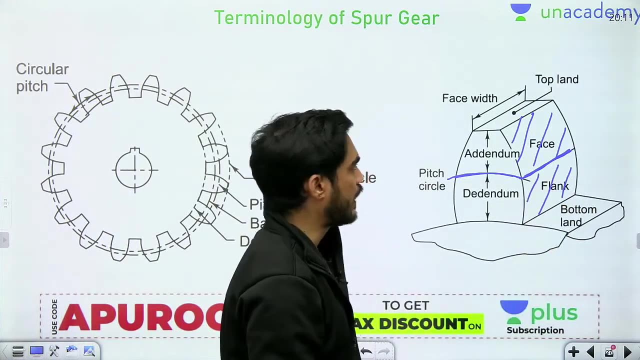 then, above the pitch circle, whatever there is, it is known as addendum, this distance is addendum, this distance is didendum. Then, above the pitch circle, this side view is known as face and this is known as flank. So this is complete side view of the teeth. 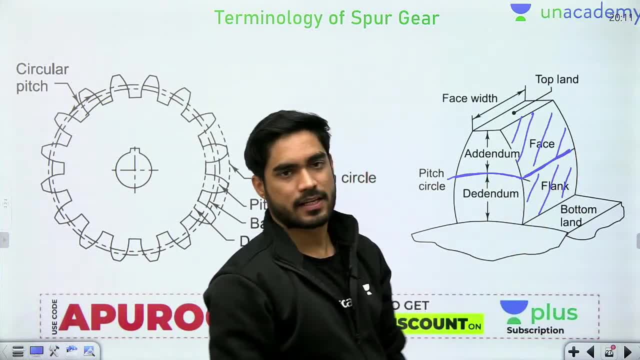 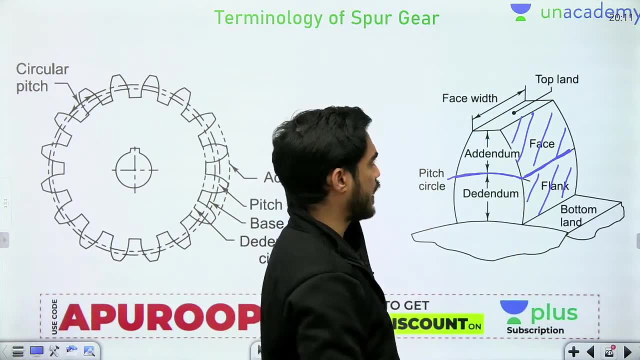 Above the pitch circle, this is known as face. Below the face circle, it is known as flank. But you don't need to worry about these parameters. These parameters will be used in theory of machine. What you need to understand here is circular pitch. 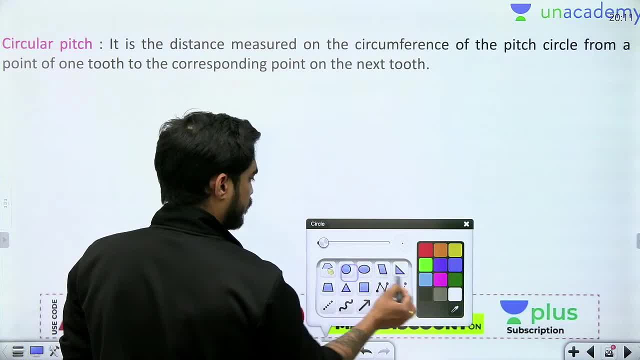 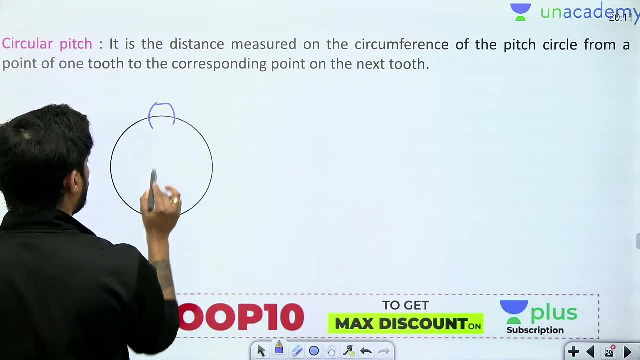 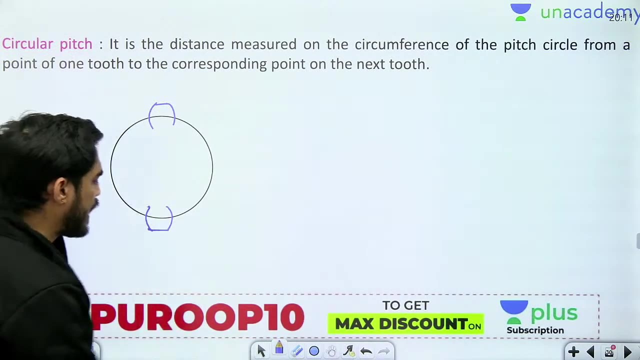 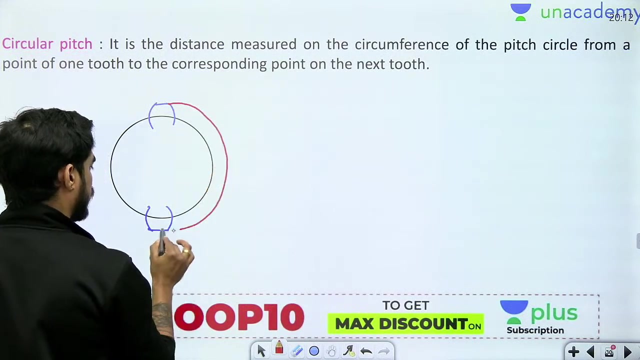 What is circular pitch? Let's say we have a gear. Let's say we have a gear and it only has two teeth. Assume how many teeth are there in this gear. There are only two teeth. Now, if I ask you, what is the distance between one point of this teeth? 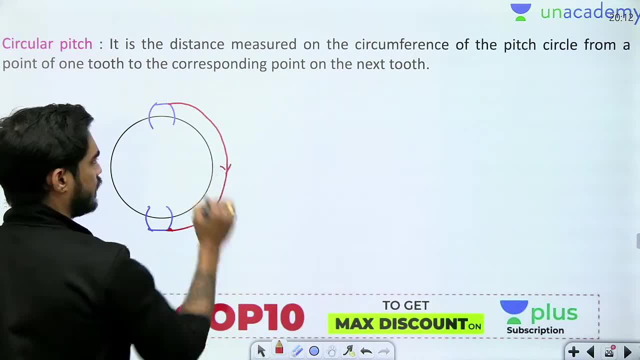 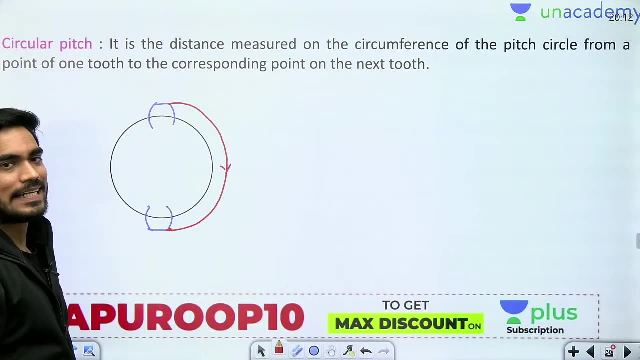 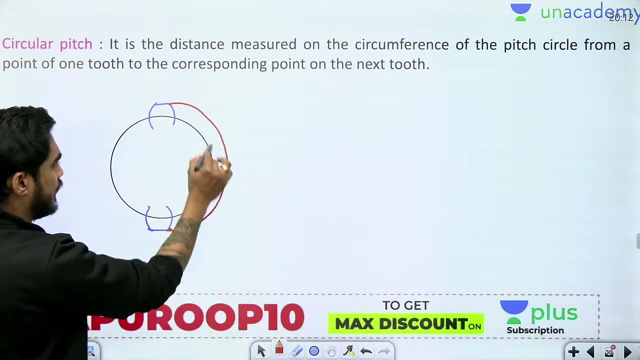 to that same point on another teeth. What will be this distance? What will be this distance? If the diameter of this is d, then this complete circle will be pi d. What will be this complete circle? It will be pi d. This will be what. 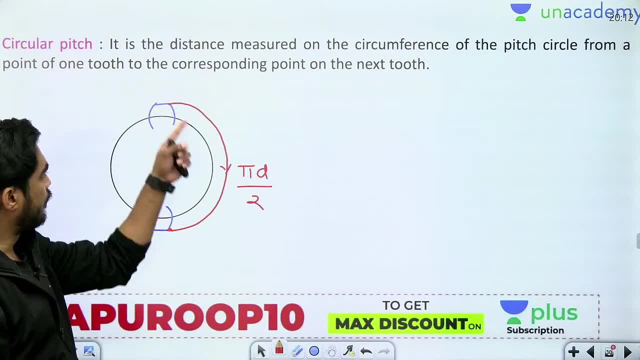 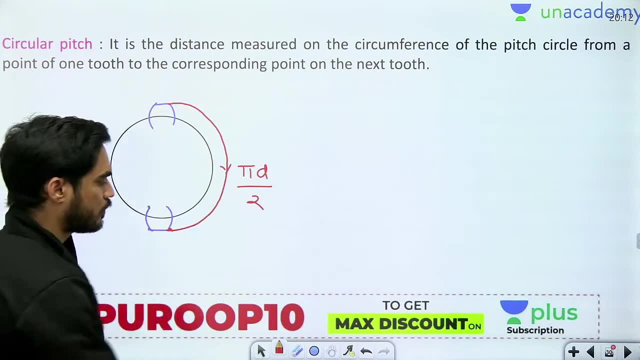 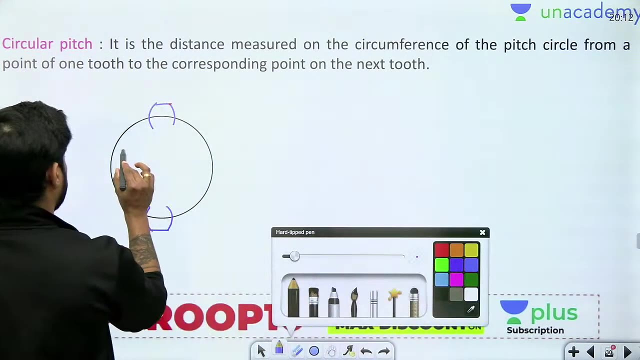 Pi d by 2.. Right, If this complete circle is pi d, if the length of complete circle is pi d, then this half length will be pi d by 2.. Now imagine that instead of two teeth there are four teeth. 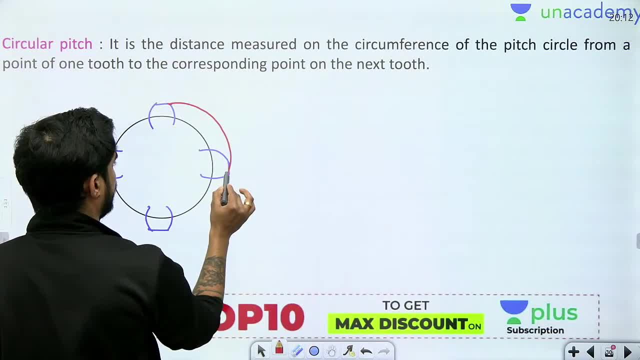 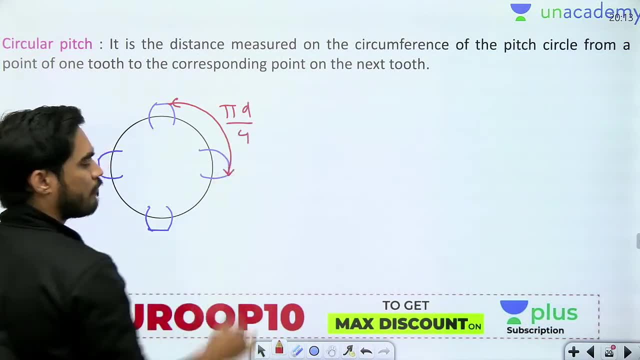 Then what will be the distance between this point and the corresponding point on the second teeth? Now, this distance will be what Pi d by 4.. So, my brother, when there were two teeth, the distance was pi d by 2.. 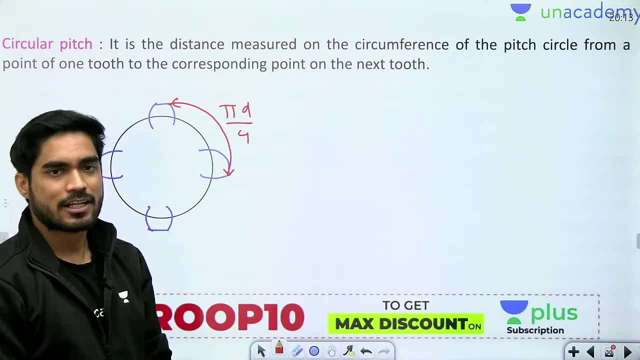 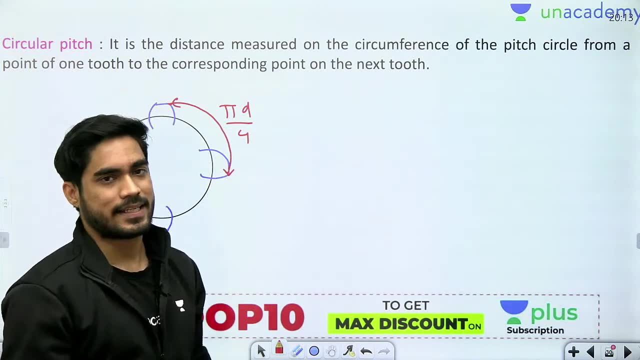 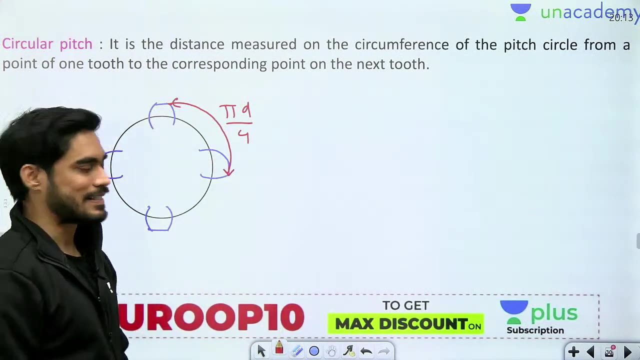 When there are four teeth, the distance is pi d by 4.. So what does it mean? The distance between two adjacent teeth will be pi d divided by number of teeth. This distance is known as circular pitch, So I will show it using this PC. 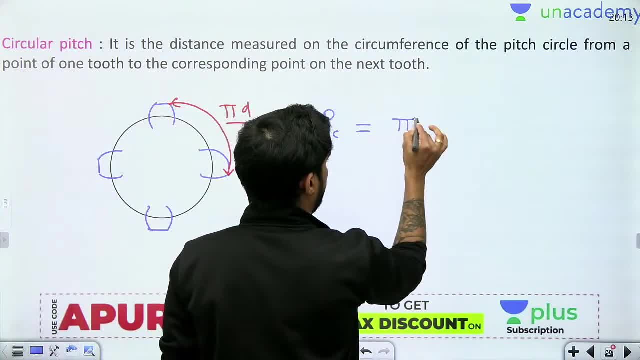 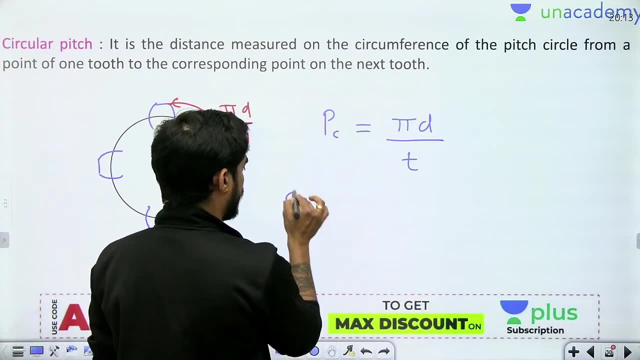 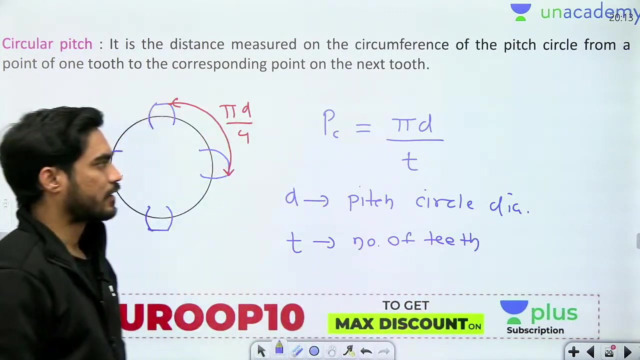 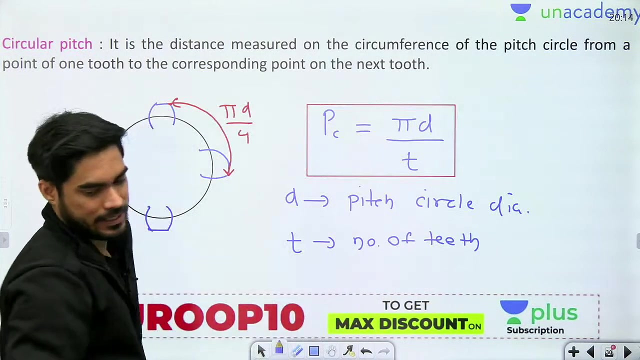 So what is PC? PC will be pi d by t, where d is Where d is the pitch, circle diameter and t is number of teeth. So, my brother, circular pitch is what? Circular pitch is the distance between two adjacent teeth. 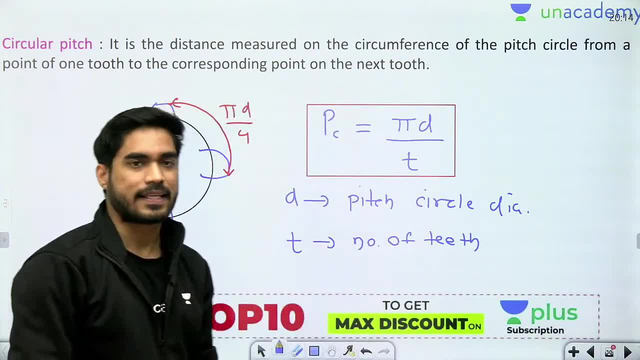 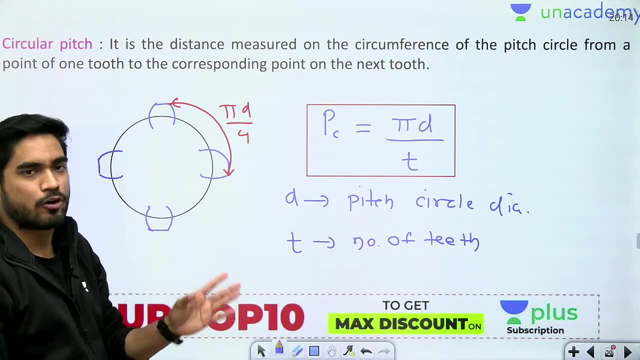 Okay, The distance between two adjacent teeth. And what will be this distance? Pi d divided by number of teeth. When there were two teeth, the distance was pi d by 2.. When there are four teeth, the distance is pi d by 4.. 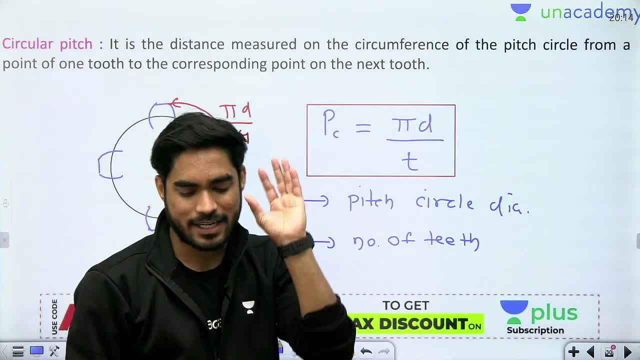 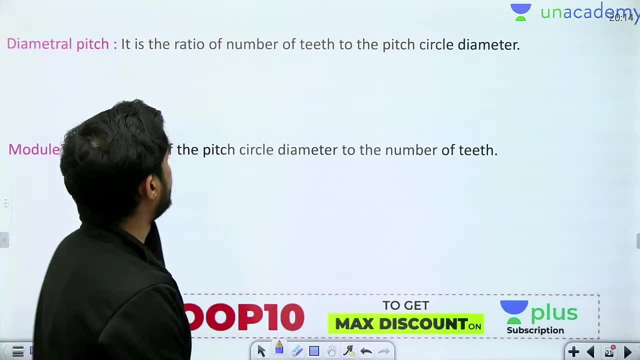 When there are eight teeth, the distance will be pi d by 8.. So pi d divided by number of teeth. Okay, Next is diametral pitch. Now, what is diametral pitch? Diametral pitch is the ratio of: 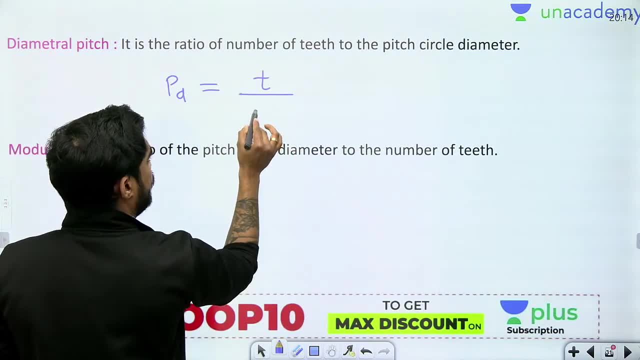 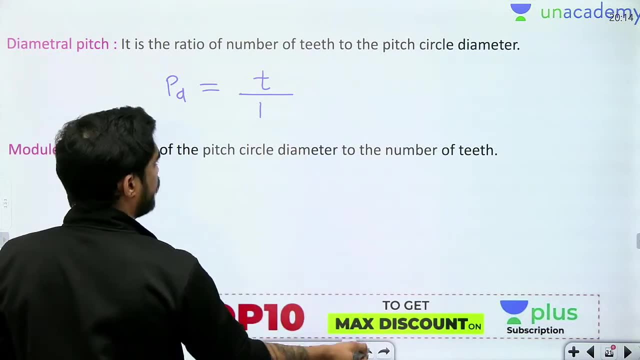 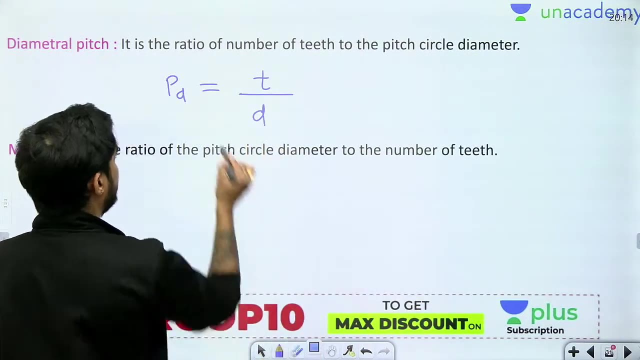 number of teeth divided by pitch circle diameter. Pitch circle diameter. Number of teeth divided by pitch circle diameter. So it is the ratio of t and d. This is what Diametral pitch. Okay, So circular pitch is pi d by t. 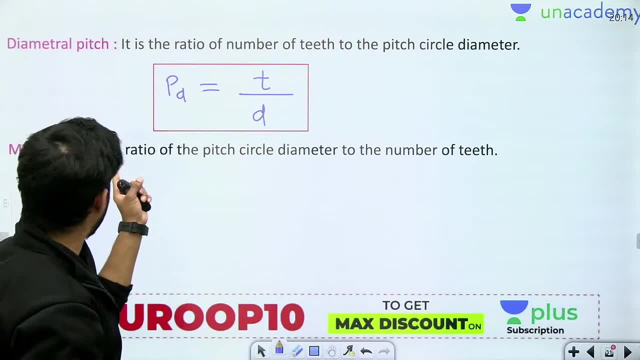 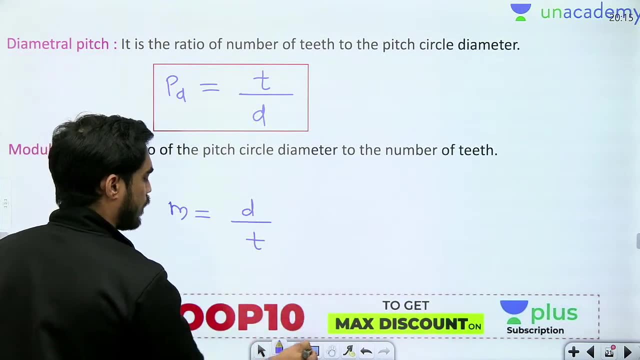 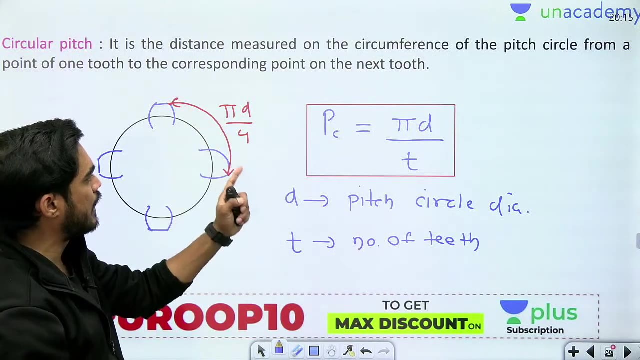 Diametral pitch is t by d And module is the ratio of pitch circle diameter to the number of teeth, So it is inverse of diametral pitch. So these three parameters, all these three parameters, are related to the pitch. 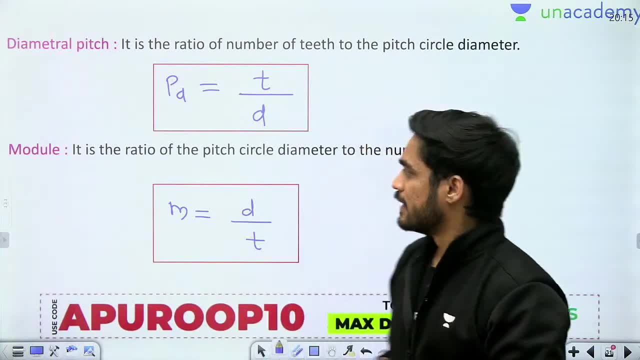 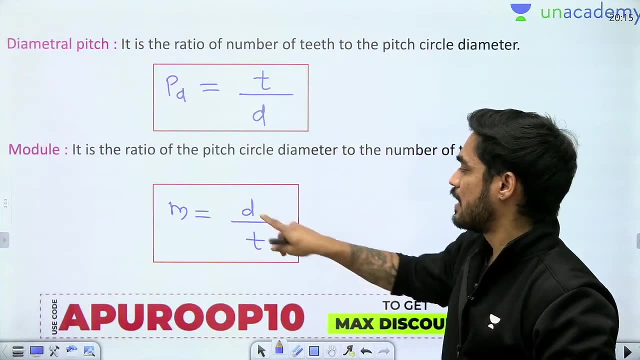 These three parameters define the pitch circle. Okay, This is defining the distance between two teeth. This is defining the ratio of teeth and diameter. And this is defining the ratio of diameter and teeth. Okay, Now my brother. Now my brother. 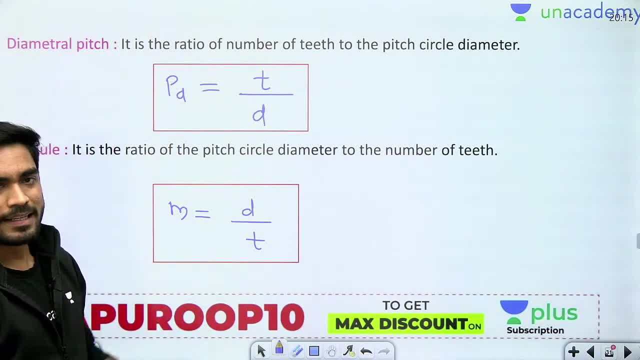 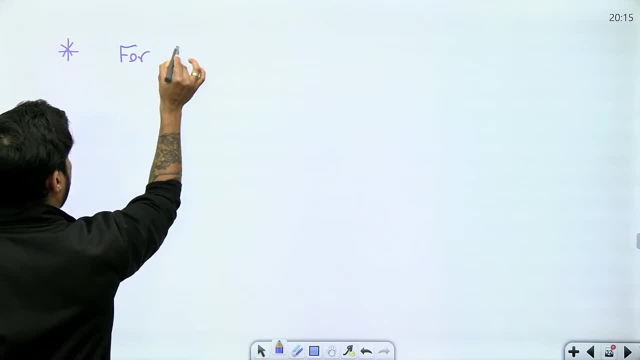 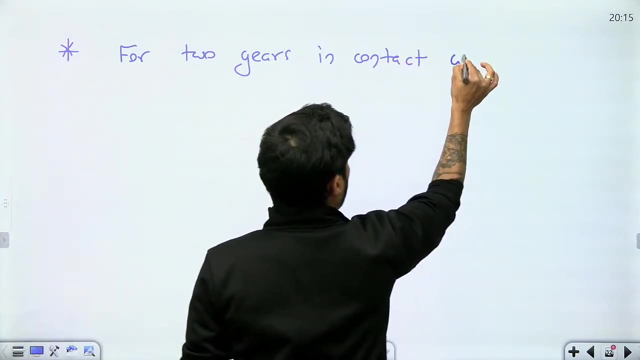 Thank you so much. Thank you so much, decent boy. Thank you so much. Now, my brother, Here you have to remember a very important point. Here you have to remember a very important point For two gears in contact with each other. 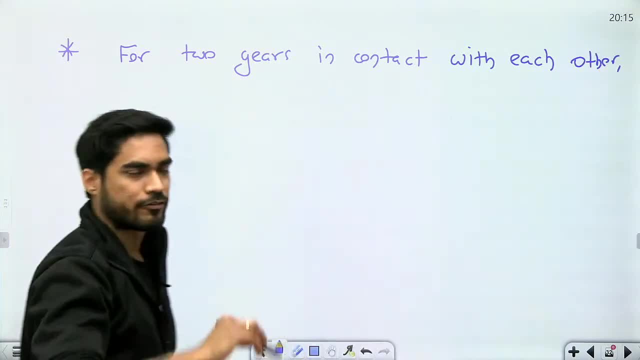 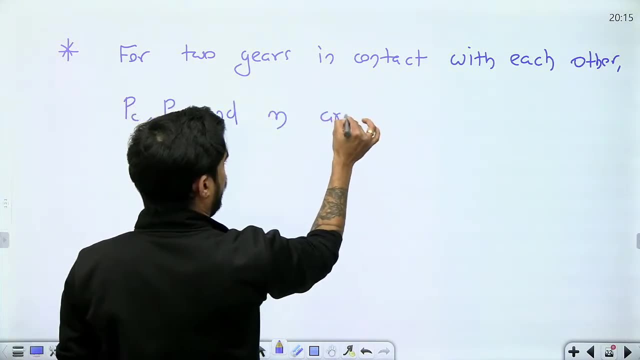 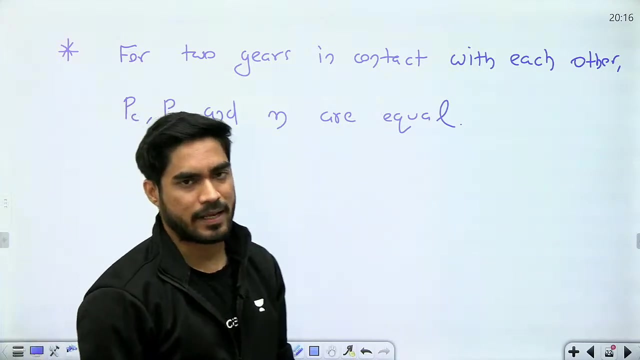 Two gears which are in contact with each other and moving with each other, Pc, Pd and M are equal. That means if two gears are in contact with each other. If two gears are in contact with each other, moving each other, Then they are. 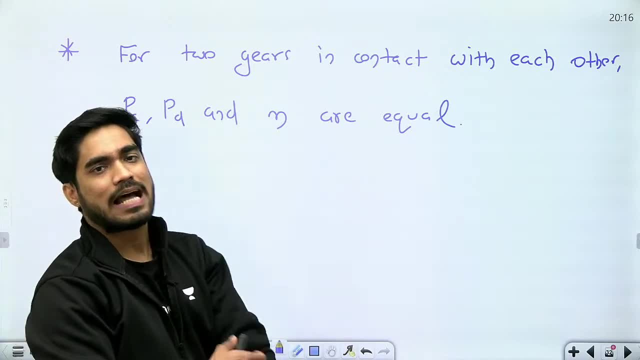 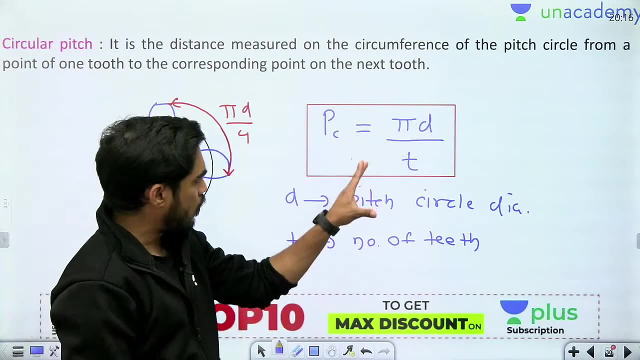 a circular pitch, diametral pitch and module are equal. Now, my brother, All three will be equal. If one is equal, then the other two will also be equal, Because in all three you can see, there is a ratio of D and T. 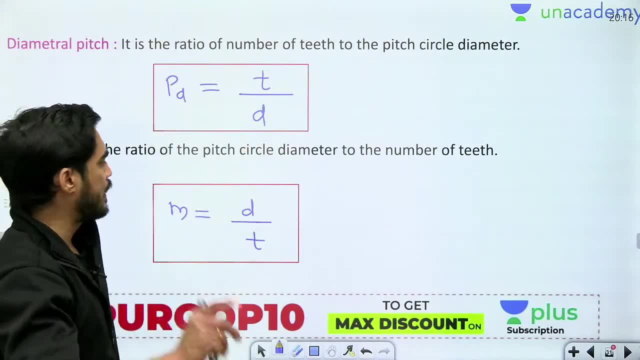 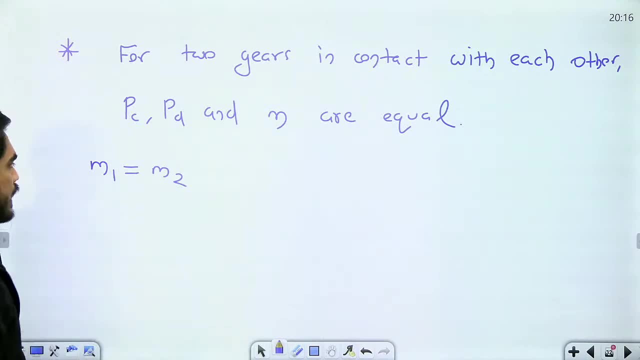 So if one is equal, the other also will be equal. Now, my brother, If the module is equal to both, Let's say M1 is equal to M2. Then it means D1 by T1 is equal to D2 by T2.. 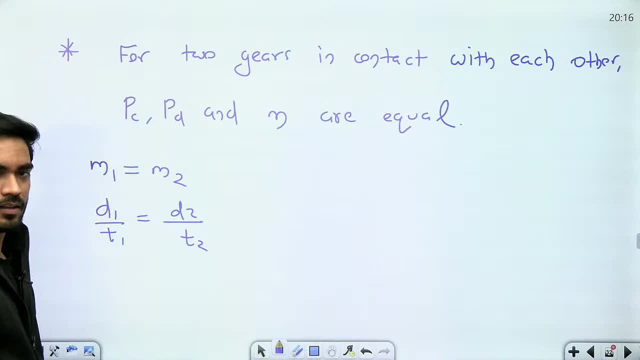 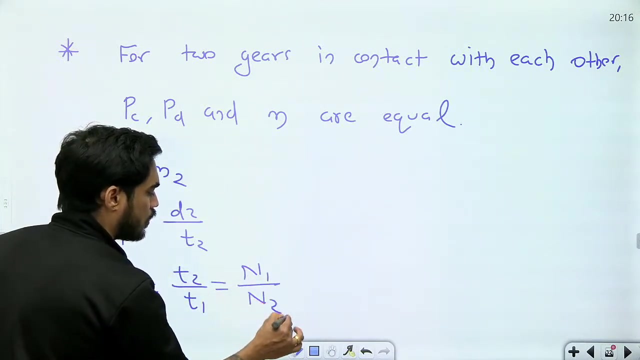 Right: D1 by T2 equals to D2.. So can I write it: D2 by D1 equals to T2 by T1.. D2 by D1 equals to T2 by T1.. And what is D2 by D1?? 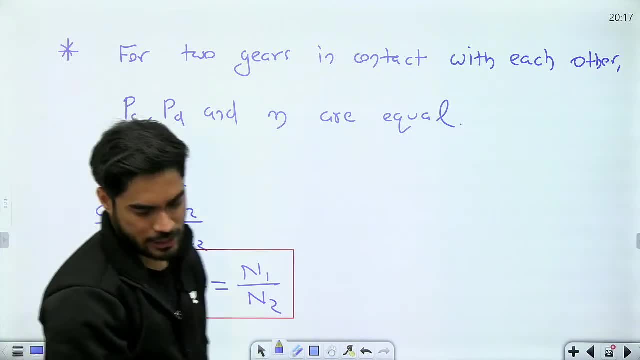 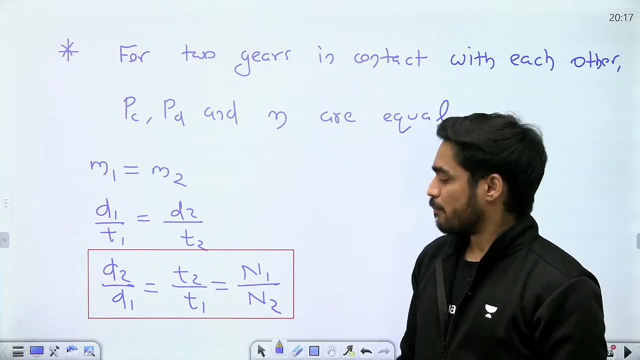 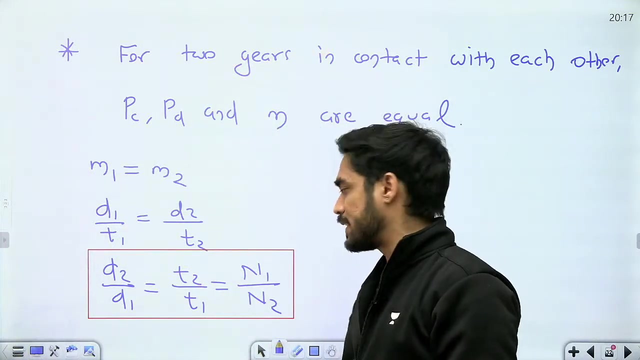 It is N1 by N2.. D2 by D1 equals to T2 by T1 equals to T2 by T1 equals to N1 by N2.. So remember this, Because you might use this in some question, Although it is. 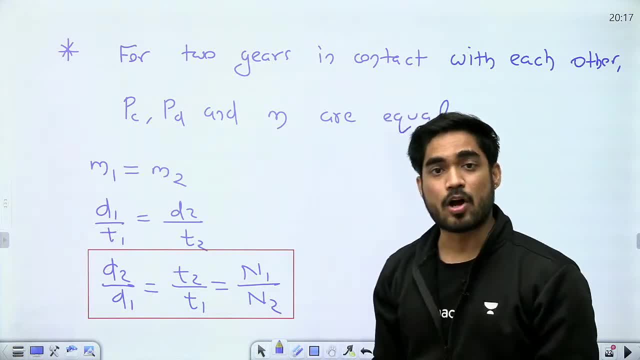 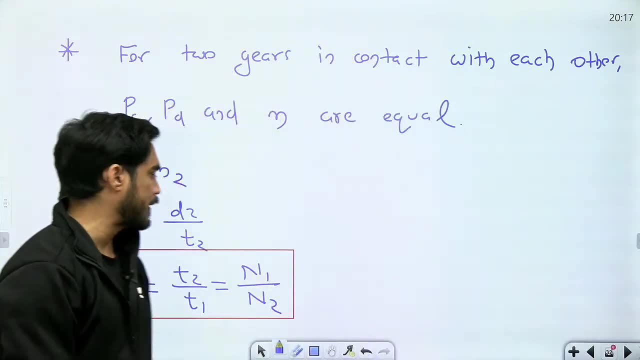 equal to D2 by D1, equals to T2 by T1, equals to N1 by N2.. So remember this, Because you might use this in some question. Although it is not used here, it will be used in theory of machine. 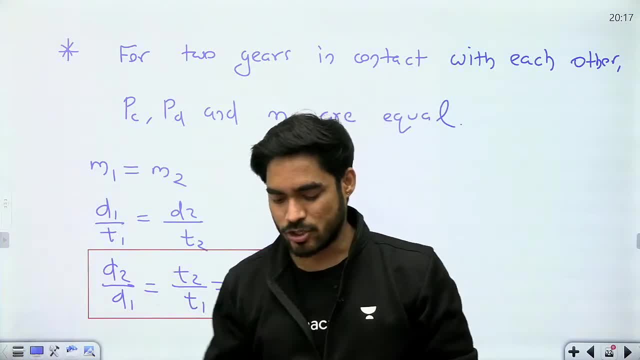 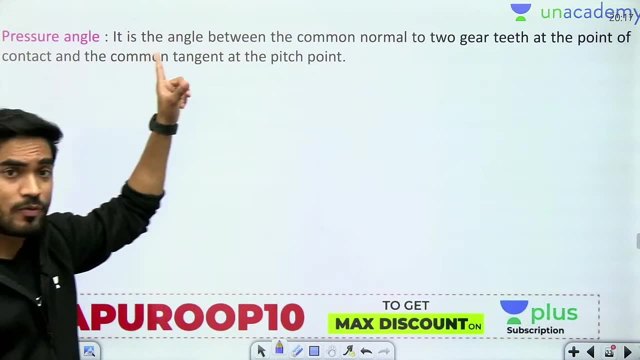 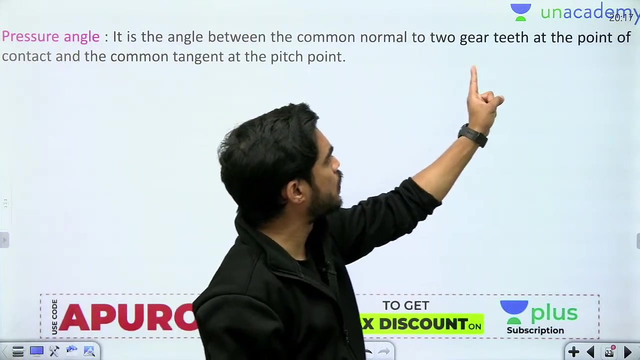 This is used in theory of machine. more Velocity ratio is used in theory of machine. Next very, very important parameter- you might get question from this parameter, which is pressure angle. It is the angle between the common normal to two gear teeth at the point of contact. 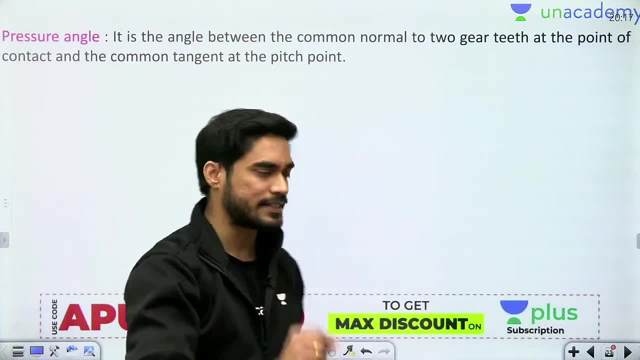 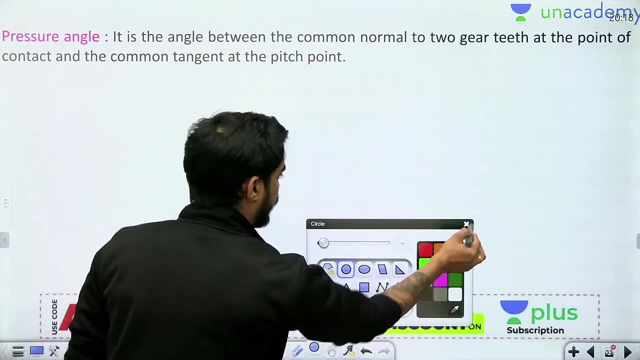 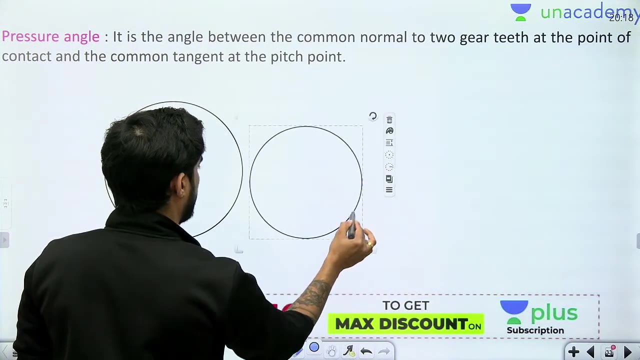 and the common tangent at the point of pitch point. Understand what is normal, understand what is pitch point, Sorry. understand what is common tangent and common normal. So, my brother, let's say there are two gears in contact with each other. 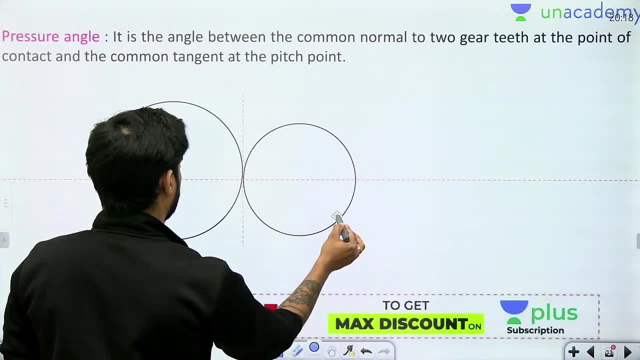 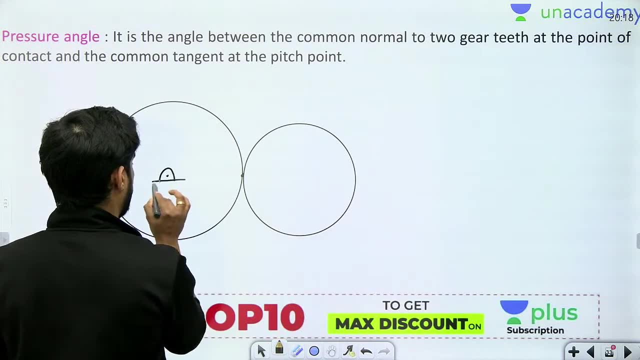 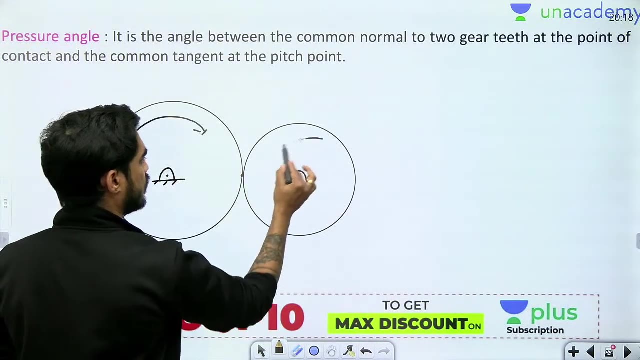 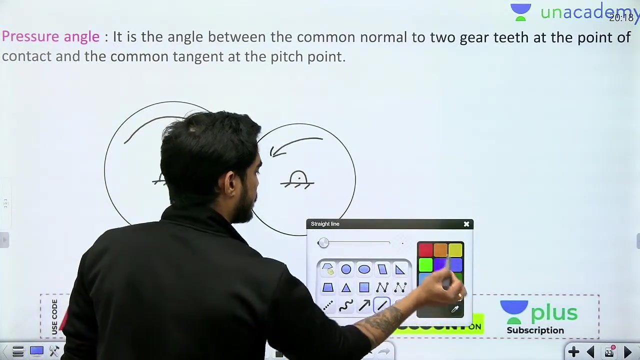 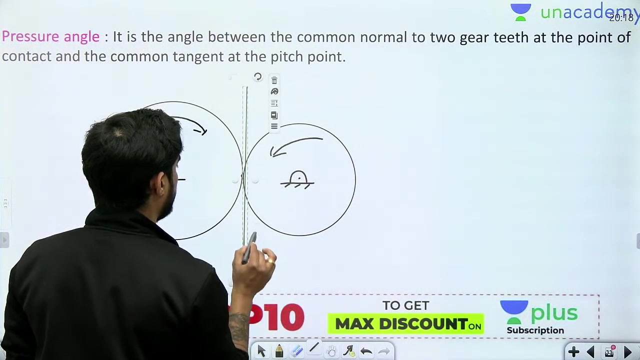 These two gears are in contact with each other at this point. This is the center of this gear. This is the center of this gear. They are rotating like this. Now understand this line which I have drawn, passing through pitch point, this line: 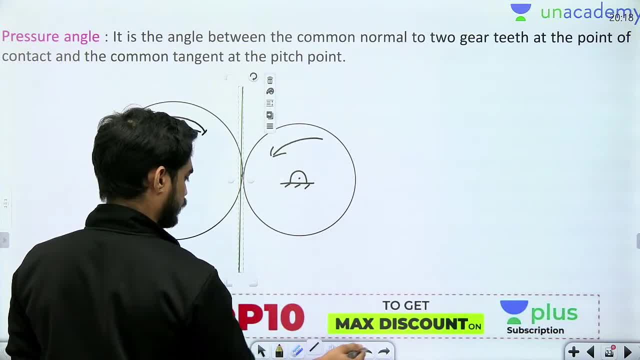 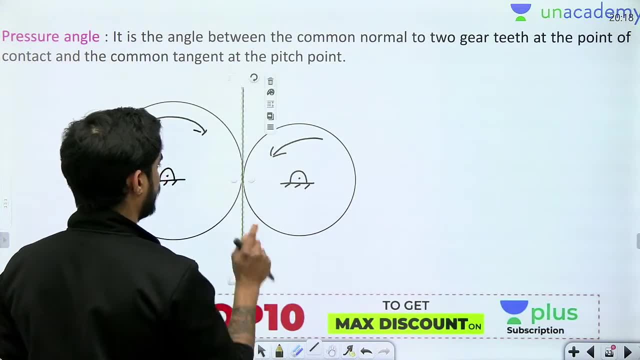 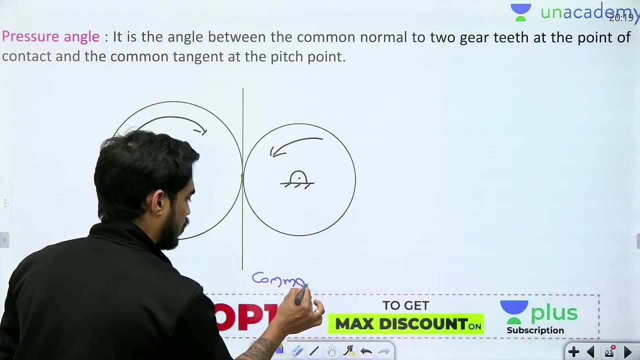 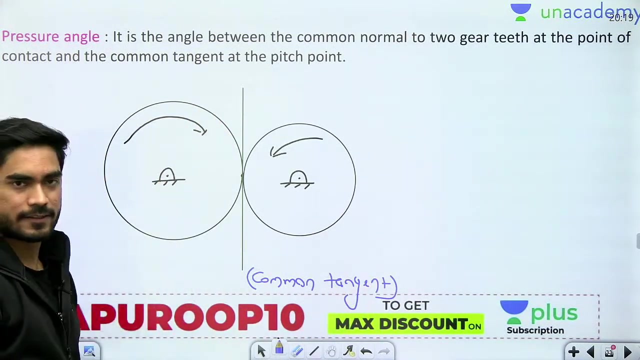 that I have drawn, passing through pitch point this line. this is known as common tangent. What is this, my brother? Common tangent? Why? Because it is tangent to both the circles. right, This is tangent to both the circles Now. 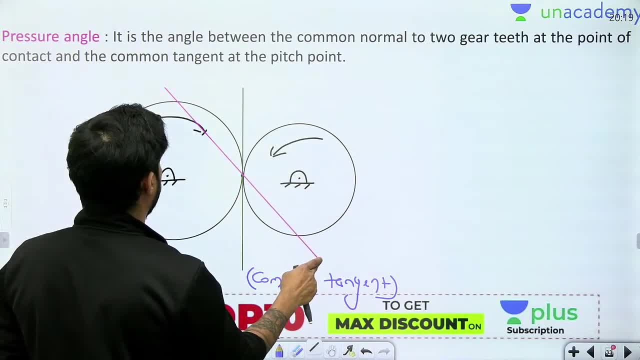 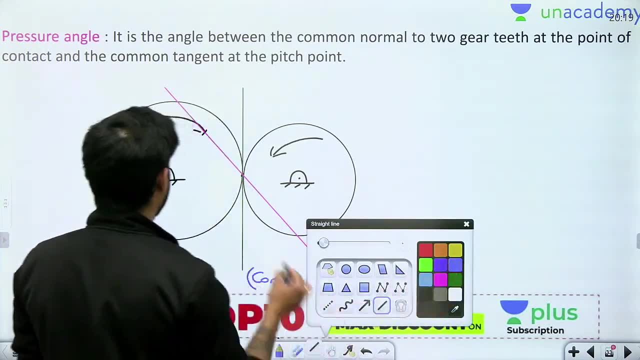 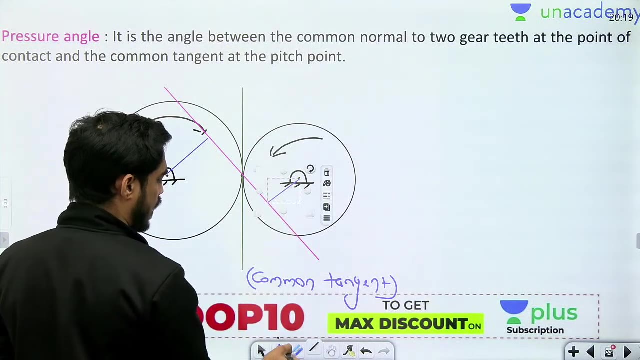 there will be a line passing through the same point which will be inclined. What is this line? This line is known as common normal. Why, my son Understand? because it is normal to these lines passing through the center, This is also normal. 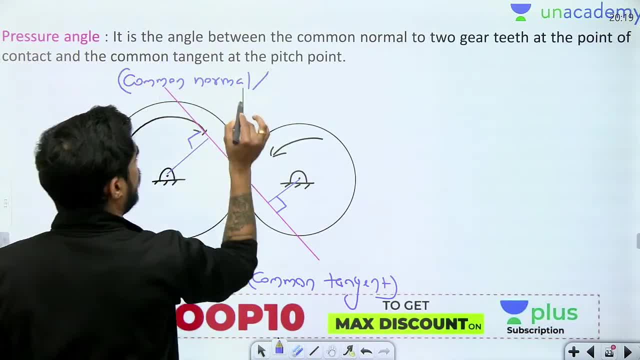 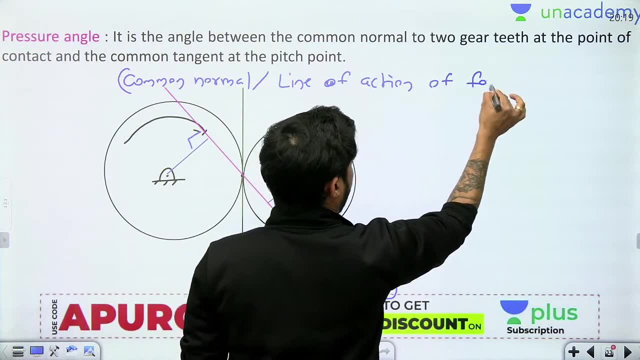 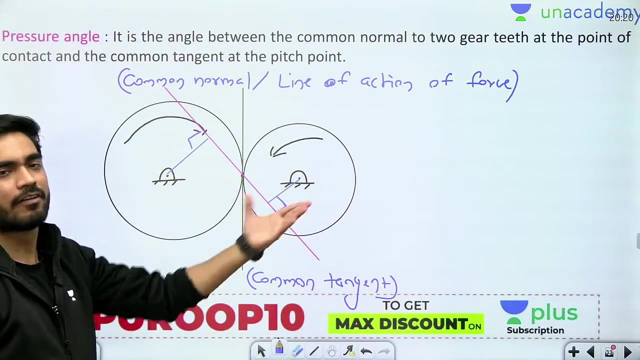 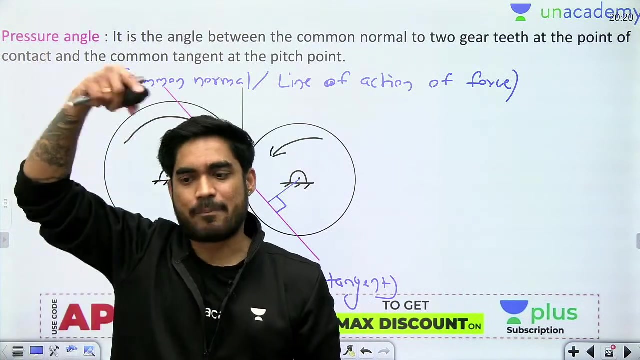 for this, and this is also common normal, And it is also normal for this and this. Now let's see how this line of action of force will rotate this gear. How will it rotate? How will the input gear rotate, the output gear? 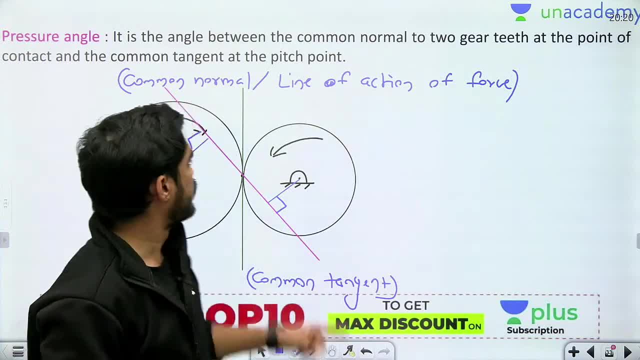 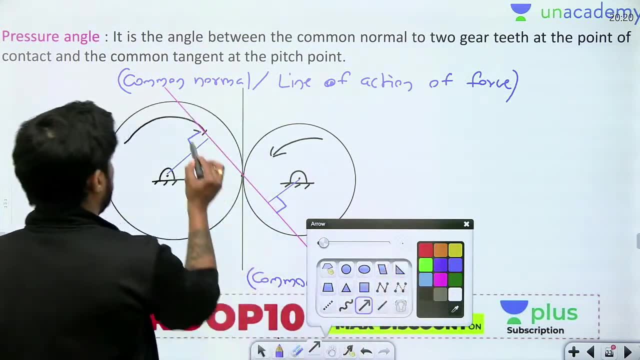 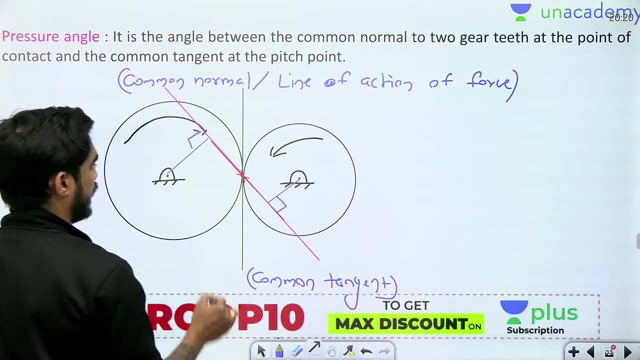 By applying force, input gear will apply force on output gear. then the output gear will rotate, So the force passes through this line. like this: It acts like this: The gears on each other apply force. like this: This gear is on this. 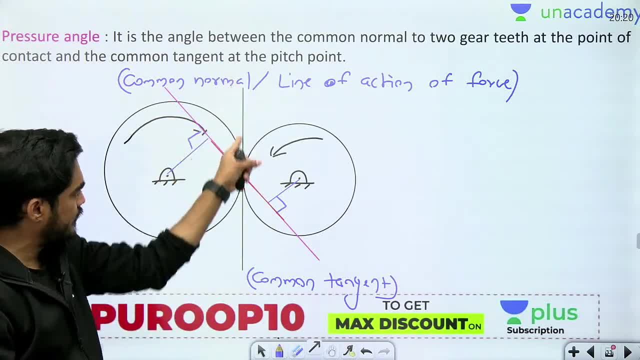 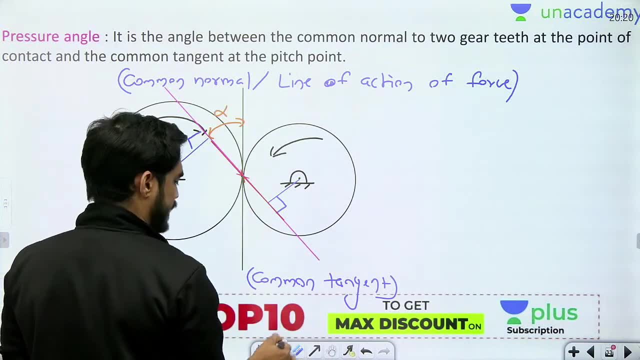 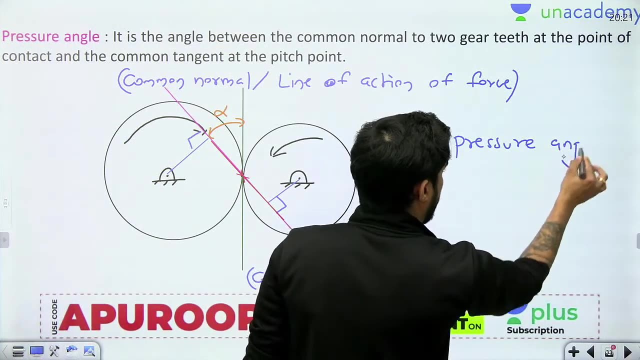 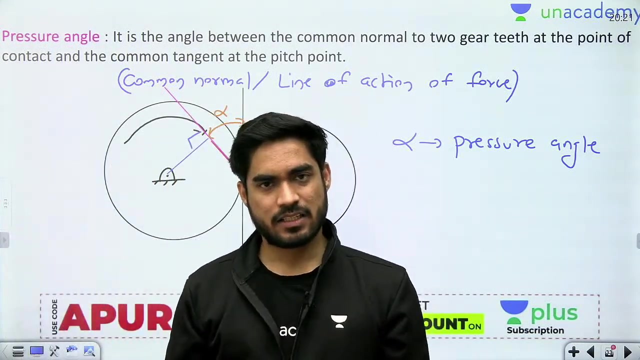 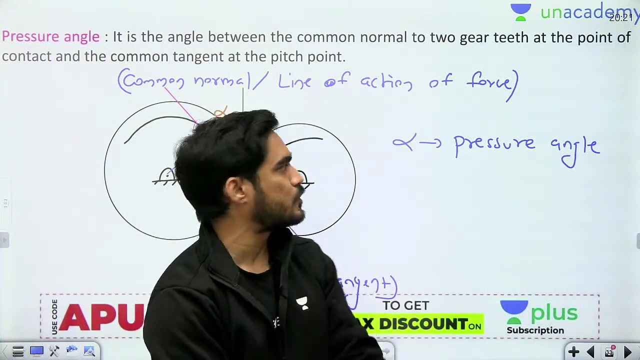 and this gear is on this. So this is the common normal and this is the common normal as pressure angle. and it is very important Why beta? Because beta, this pressure angle will relate all the parameters of the gear, All the parameters of the gear. 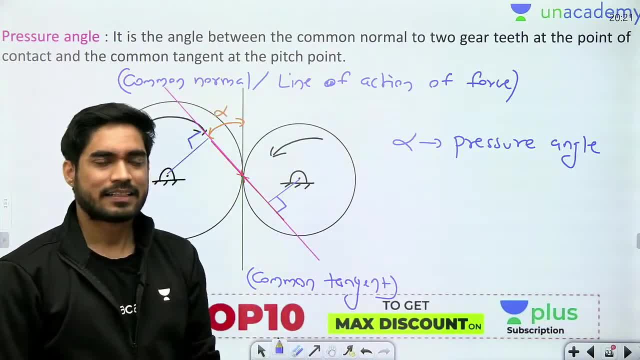 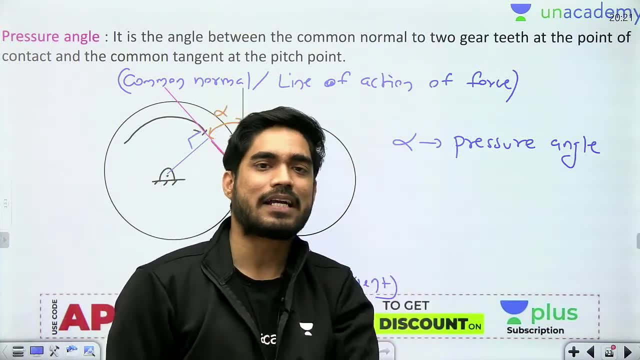 are related by this pressure angle. How they are related, What is the equation? You don't need to get into that, But understand that beta whenever we need to. didendum. nicala, we don't calculate every parameter separately, we only calculate one parameter, which. 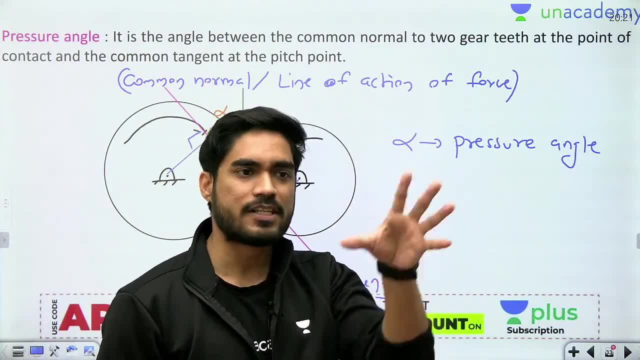 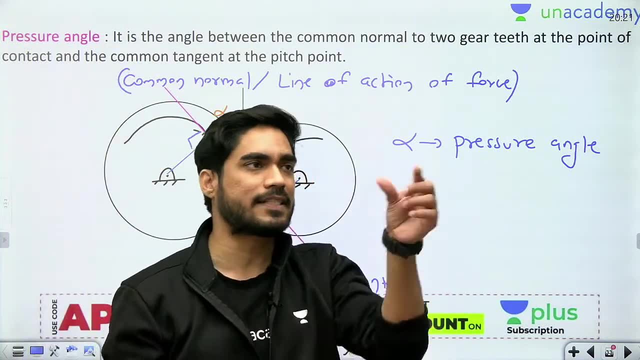 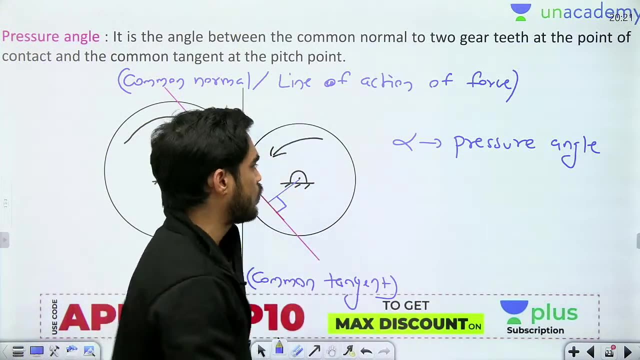 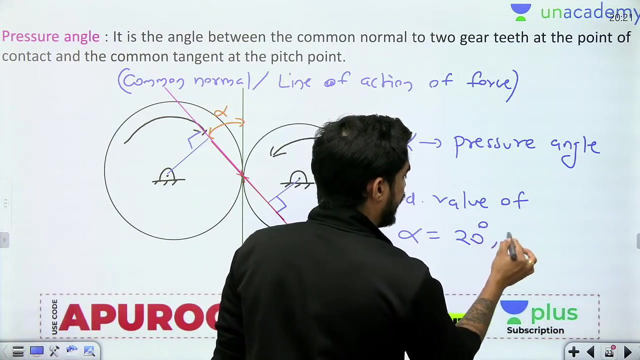 is module, only module is calculated, only module is fixed. then beta: using the module we can find other parameters, because there is a relation between other parameters and module and that relation depends upon this alpha. now alpha has some standard values, alpha standard values. standard values of alpha are 20 degree and 25 degree. okay, only you will see a pressure angle. 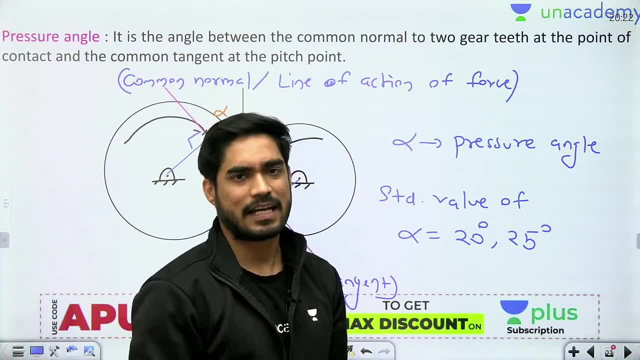 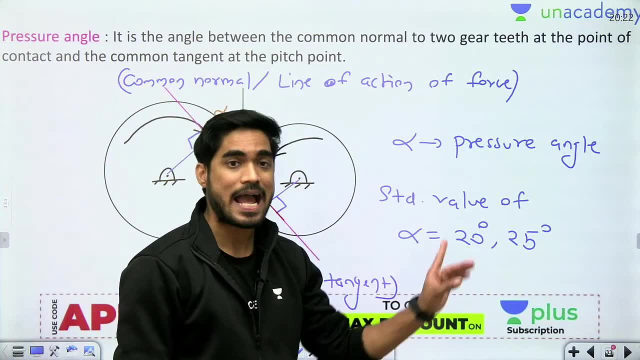 20 degree and 25 degree. earlier there was another pressure angle, 14.5 degree, but that is not used nowadays. okay, so you will only see 20 degree pressure angle, 25 degree pressure angle. why? why can't we use some other pressure angle? because, beta, we only have relations between: 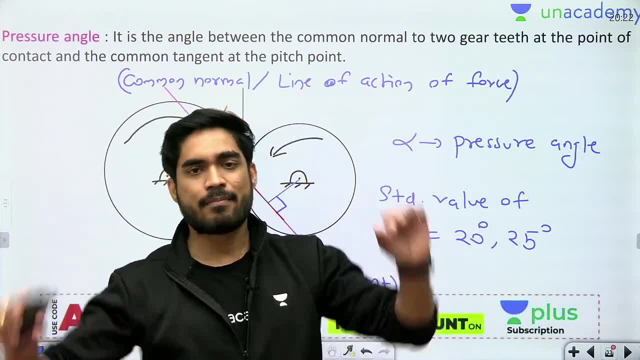 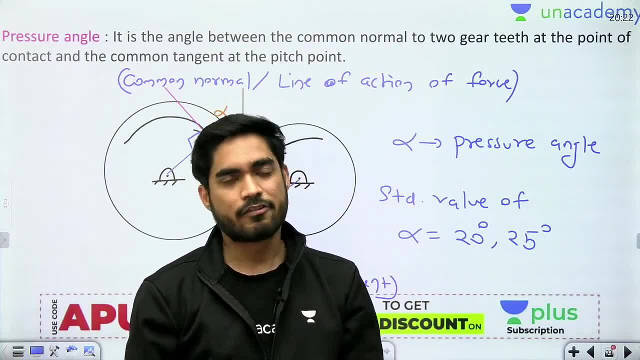 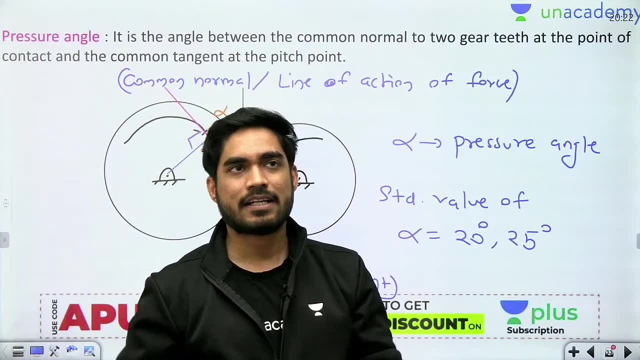 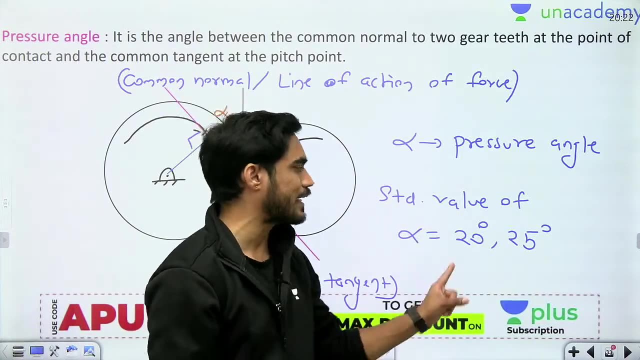 calculate other parameters. okay, we will use the same table given by some person for 20 degree and 25 degree. so if you want to use 20- let's say 2.3 degree, then you will have to make your own table. will it be possible? so that's why you use standard values: 20 degree. 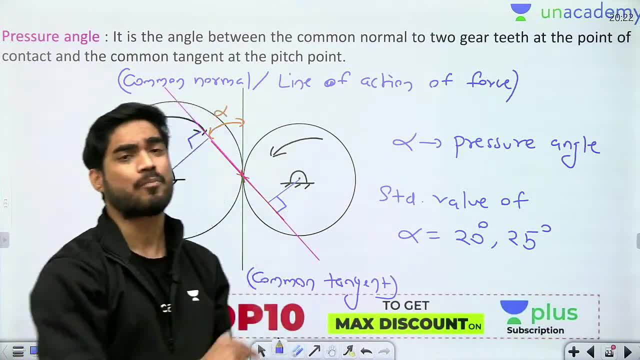 and 25 degree. now we choosing pressure angle. so now, when we talk about overall, you have to pay attention to its different餐. Hehe, تب copperّα. angle is very important. Why pressure angle is only 20 and 25, like this, only Zero degree. 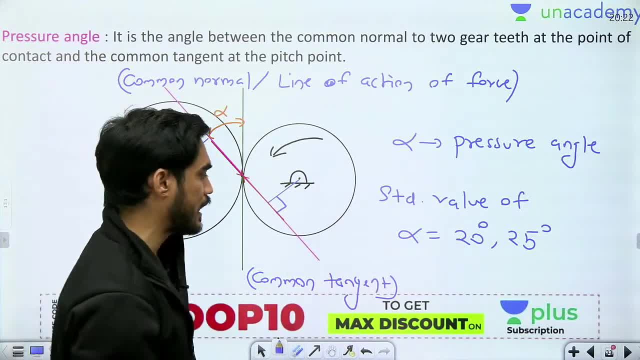 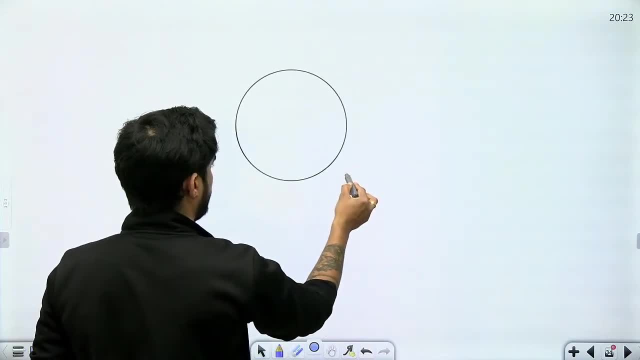 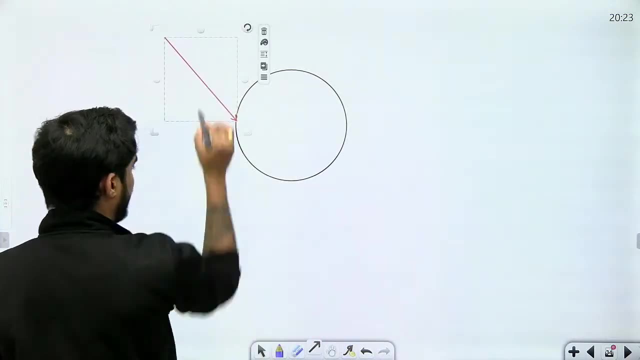 se, 45 degree ke exactly beach mein kyun hai. Pressure angle. understand beta. Let's say this is my input gear. Let's say this is sorry, this is my output gear. Now beta output gear is rotating because there is a force acting by the input gear on the output gear Output. 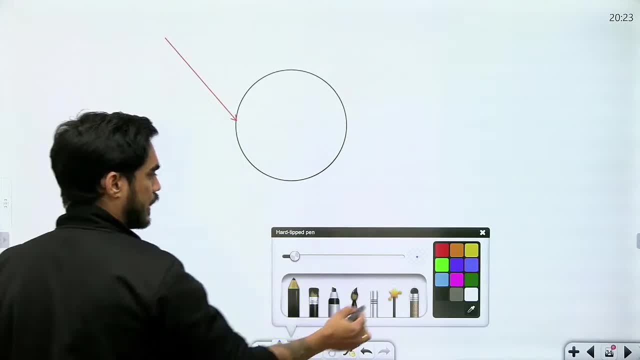 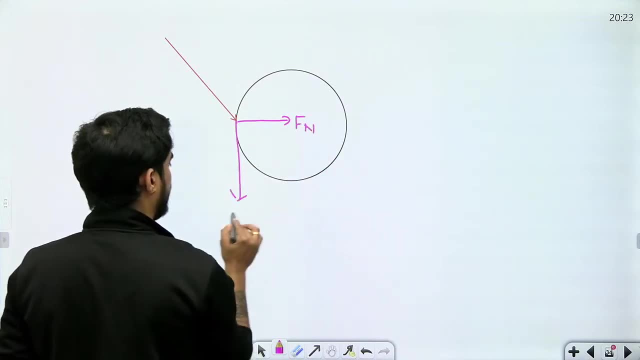 gear kyun ghoom raha hai, Kyunki input gear, output gear ke upar force laga raha hai. Now this force has two components: One component like this- This is known as normal component, and one component like this- This is known as tangential component. Okay, Now beta this. 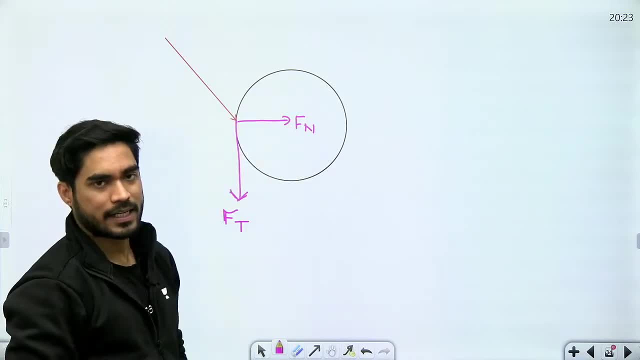 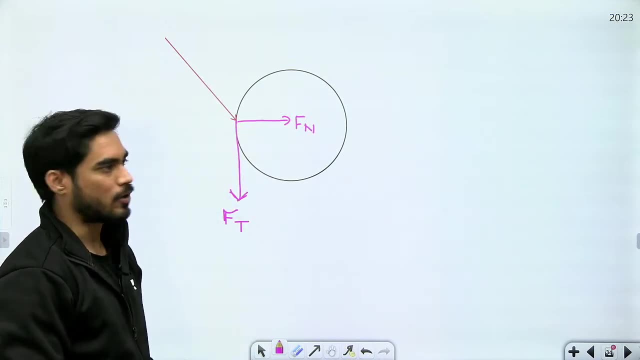 gear will rotate when the forces will apply torque on the gear. Hai na. So, mere bhai, can FN will apply torque. Can FN apply torque on the gear? No, FN can't apply torque on the gear, So which will apply? Who will apply torque on gear? 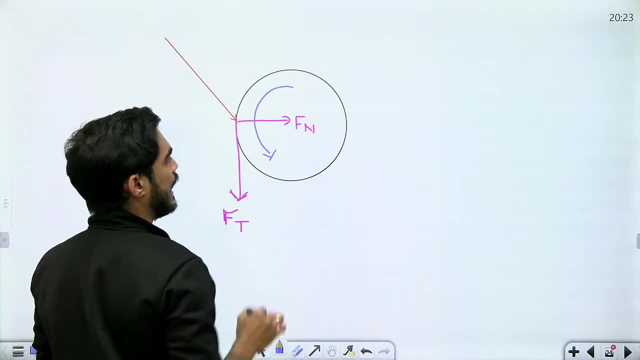 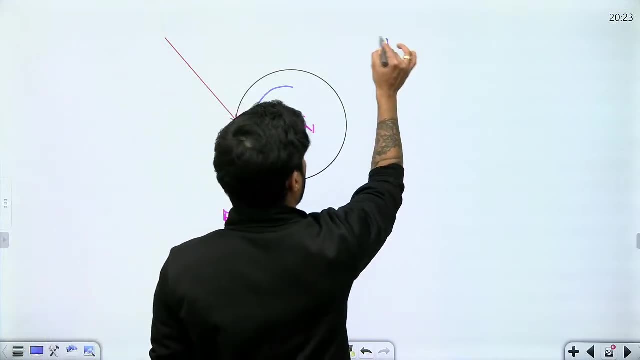 Gear. Gear ke upar torque kon lagaega mere bhai. Gear ke upar torque lagaega FT. Gear ke upar torque lagaega FT. Only FT will apply. torque on gear beta Torque T will be equals to FT. 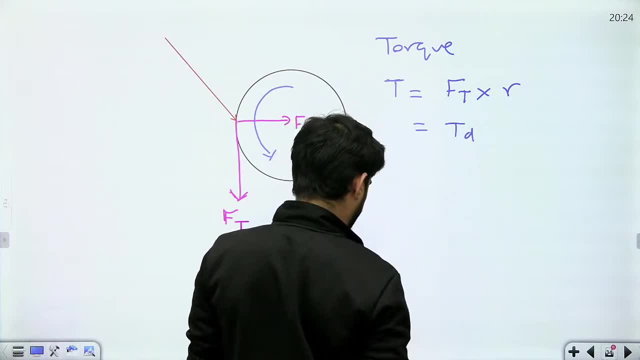 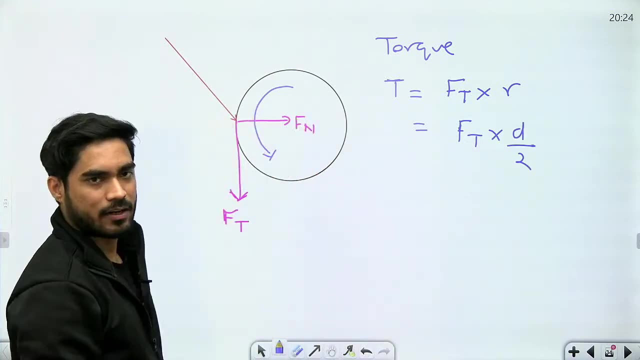 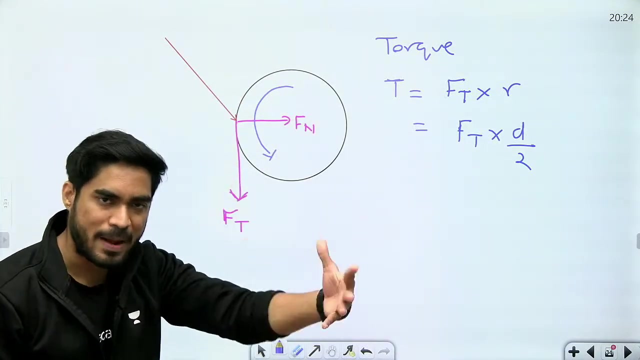 into R or FT into D by 2.. Okay, FT into radius of the gear. Okay, FN cannot apply torque. So, beta, if only FN can apply torque on the gear, So only FT will apply torque. It means if you want more power transfer, FT should be. 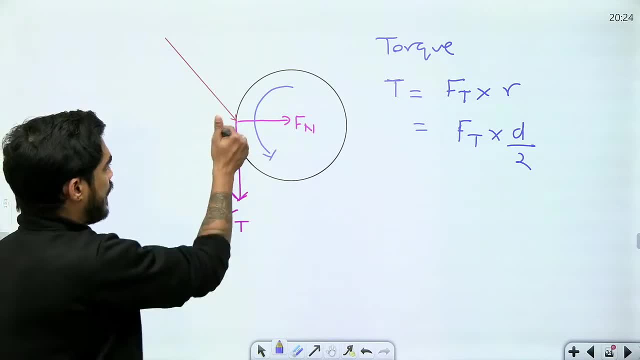 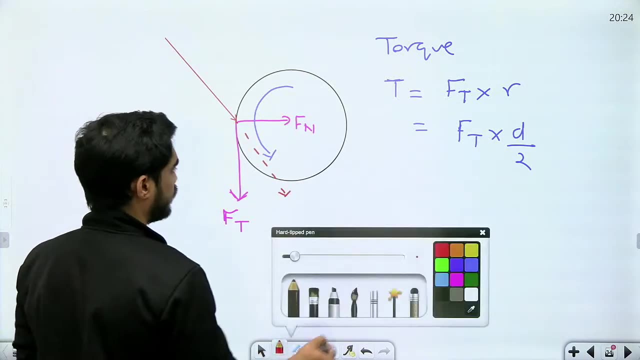 more FN should be less Hai ki na Ab FN or FT ki value jo hai wo kis pe depend karegi, mere bhai, This is my force. Right, This is my force. What is this? This is pressure angle. 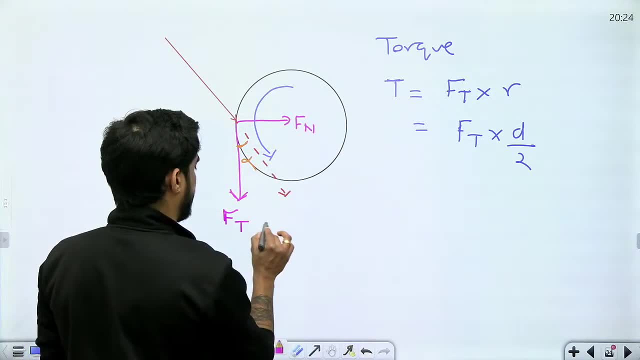 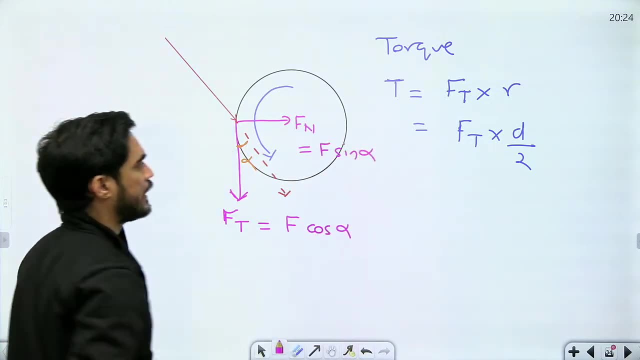 Right. FT is equal to F cos alpha and FN is equals to. This is equal to F sine alpha, Now beta. if I want more power transfer, then beta alpha. sorry, F cos alpha should be more, F sine alpha should be less. Agar mujhe zyada power. 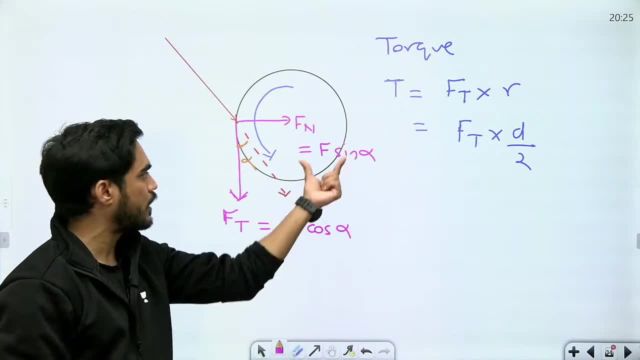 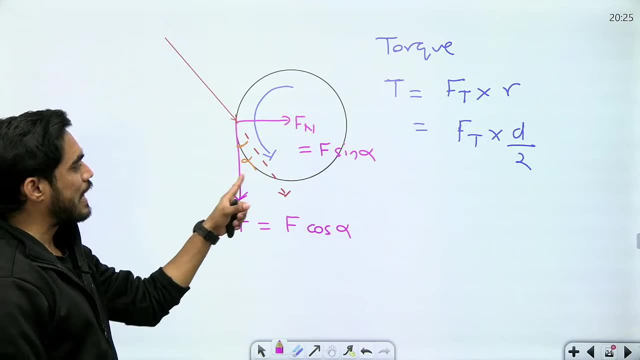 transfer chahiye, toh F cos alpha Komponent zyada hona chahiye, komponent kam hona chahiye. Ab ye komponent zyada kabhoga, or ye kam kabhoga, mere bhai. Agar alpha kam hoga, toh ye komponent. 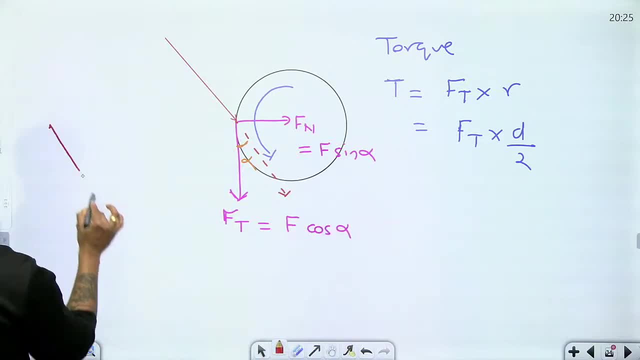 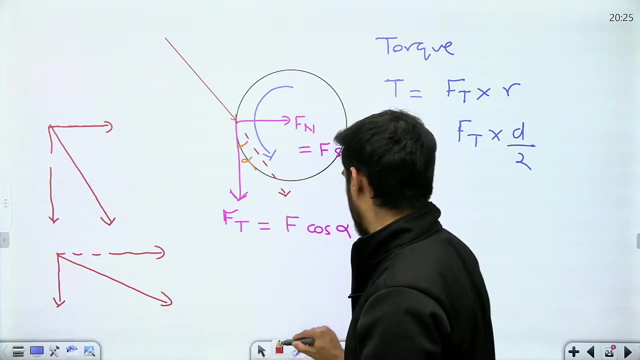 zyada hoga na. Ahah, par main apko toh diagram banake diye. I will show you this diagram. so in this vertical component is more and horizontal component is less, and in this horizontal component is more and vertical component is less. this 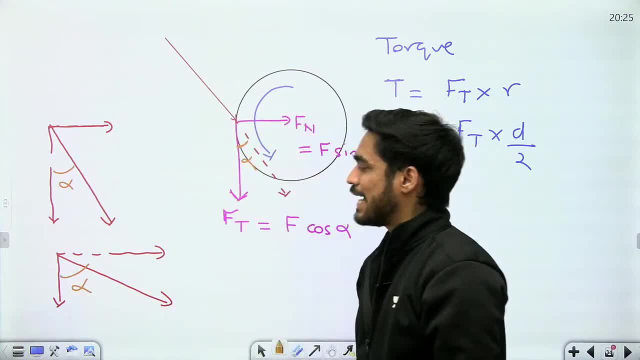 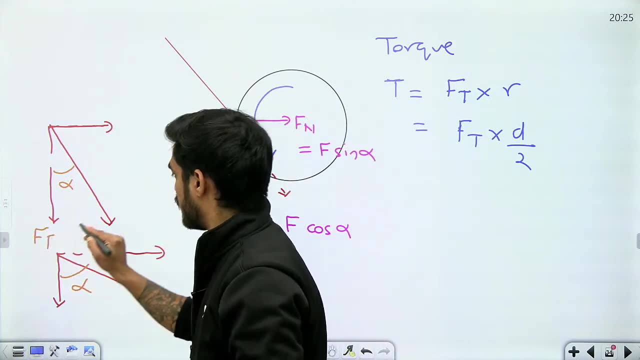 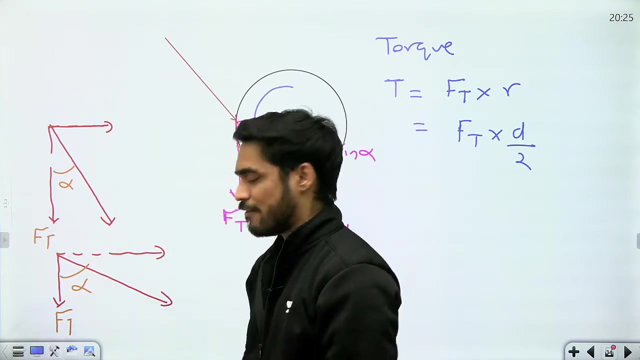 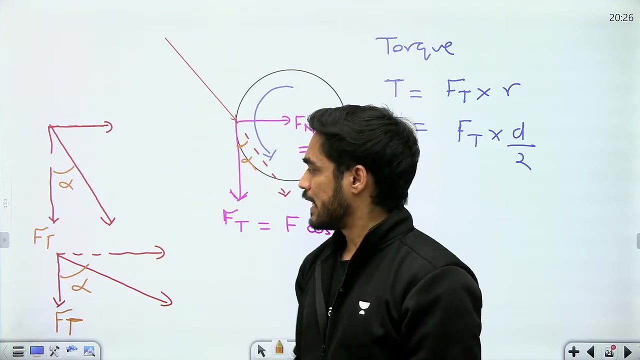 is alpha. so can you see, by increasing or decreasing alpha which one will increase or decrease. this is my FT. so if I decrease alpha, FT will increase. if I increase alpha, FT will decrease. so I want more and more FT. I want more and more tangential force. 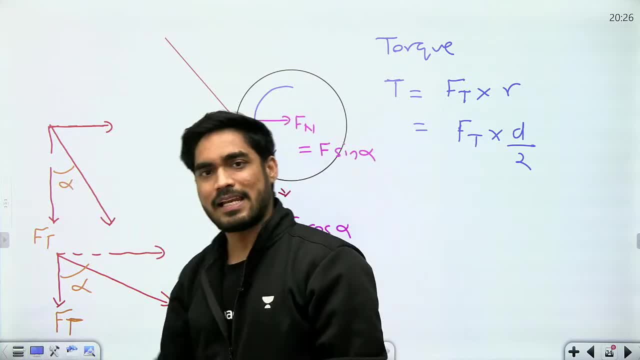 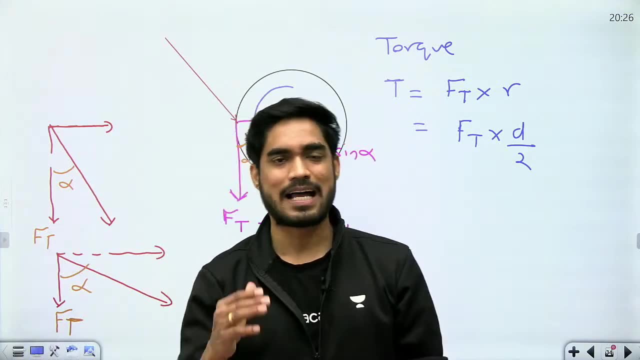 so if I want more and more tangential force, alpha should be less. Yes, I can't increase alpha beyond certain value, So, my brother, my alpha should be less. my alpha should be less. The less it is, the better. 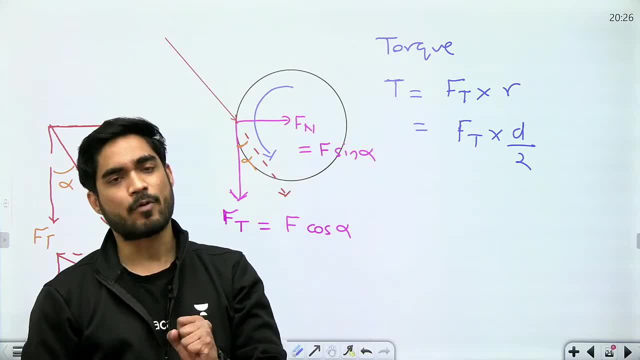 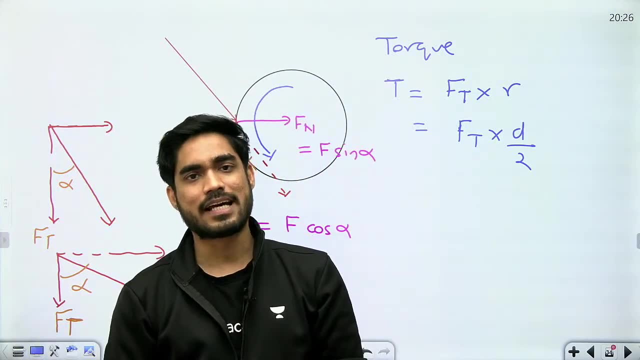 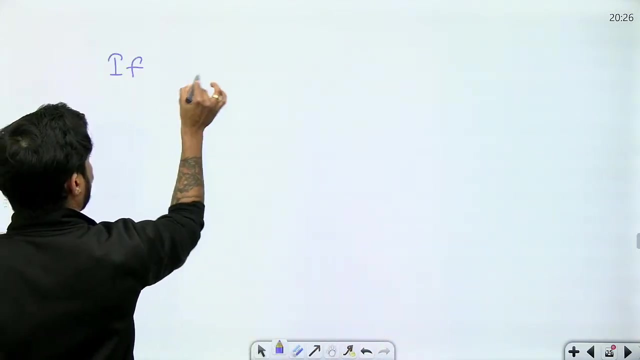 But while decreasing alpha you will reach such a point if the value of alpha is reduced. if alpha reduces, then the strength of gear teeth also reduces. Understand this relation here. If alpha is less, then T is reduced, then T is also reduced. 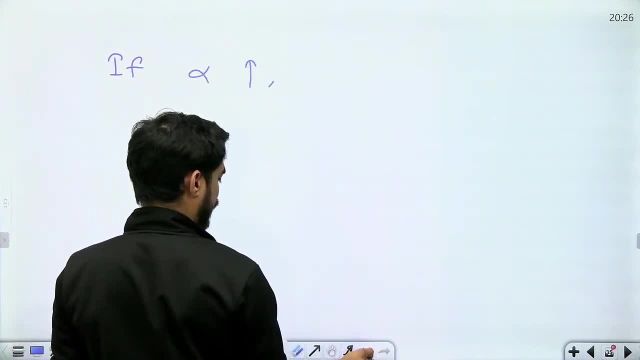 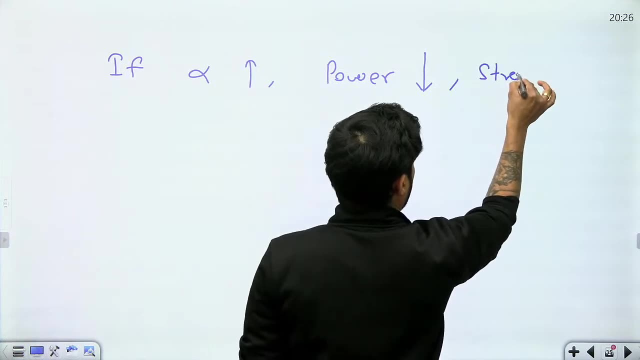 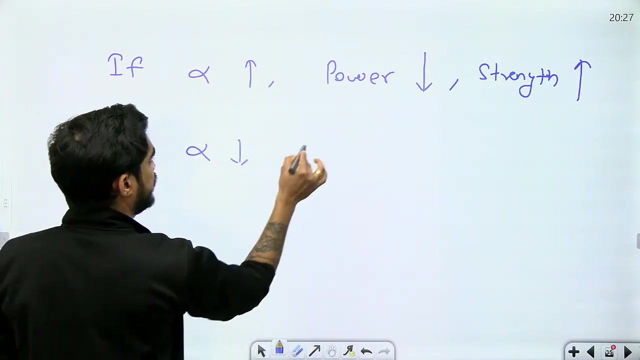 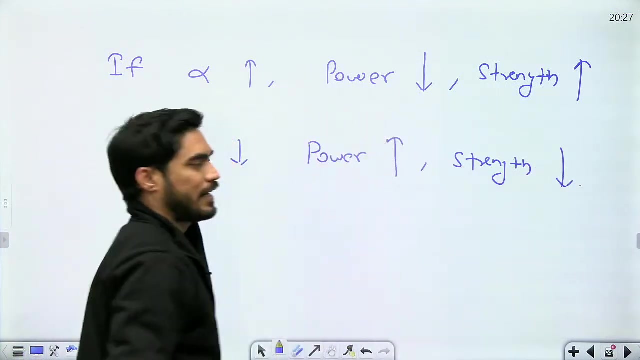 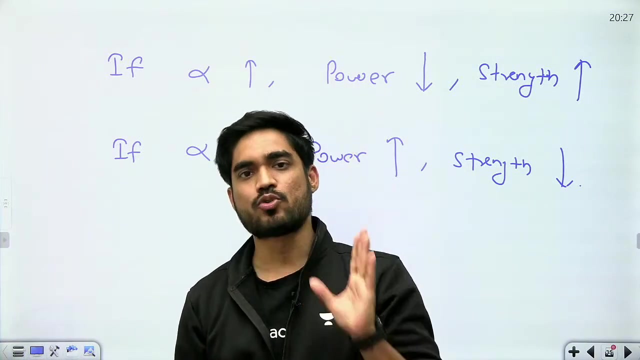 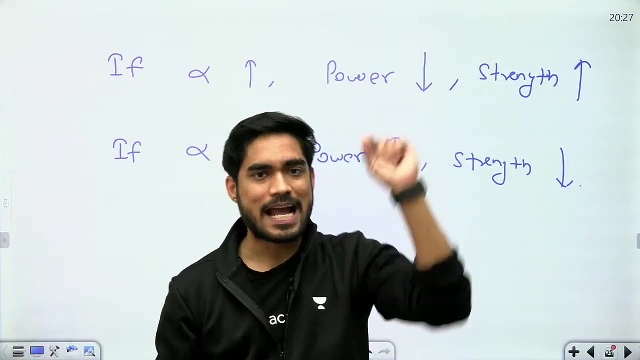 increases. if alpha increases, power decreases but strength increases. and if alpha decreases, then power increases but strength decreases, so many by. that's why we need to choose the value of alpha very carefully. alpha should not be very high or it should not be very less. okay. so the best 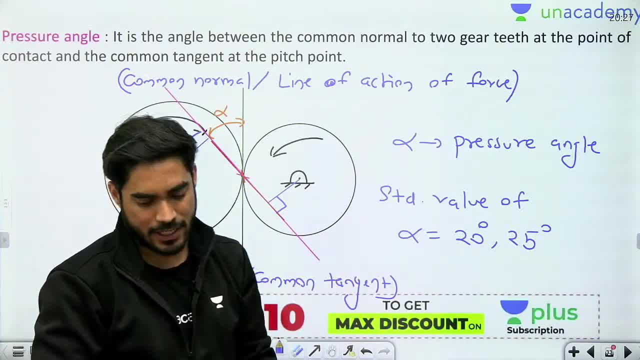 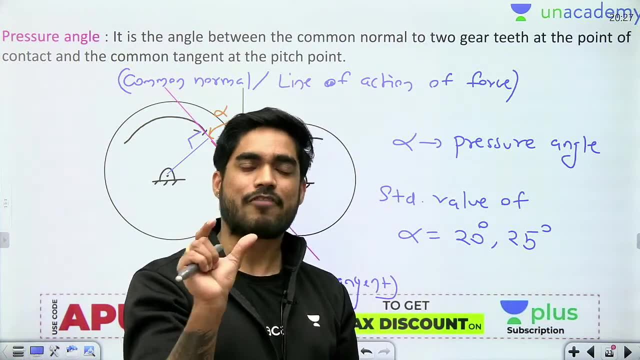 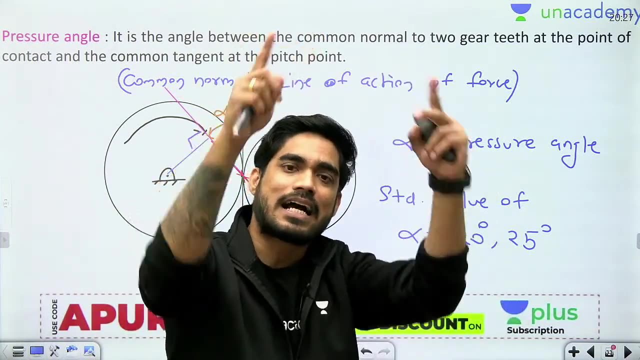 compromise is 20 degree and 25 degree. so I hope that you understand the relation between alpha and the power transfer right, why choosing alpha is very important. strength ke saath relation. aapko aise samajh mein nahi aayega beta, because you will have to then understand the entire curve of the teeth. 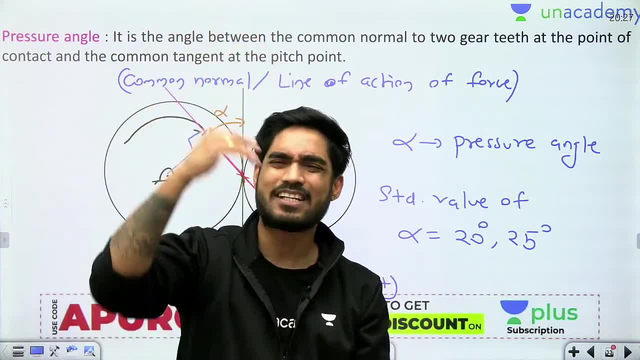 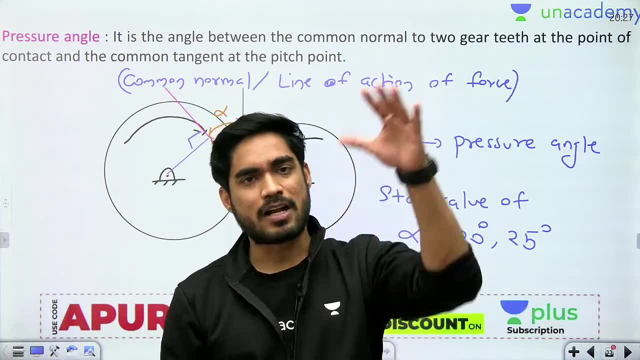 and all. so we will not get into the mathematics of that. okay, because that is useless for us. okay, apne ko utna janani ka zarurati nahi hai, aapko bas itna samjhane ki koshish kar raha tha main, ki alpha ko kam jyada karne pe. kya acha aur bura ho sakta hai? 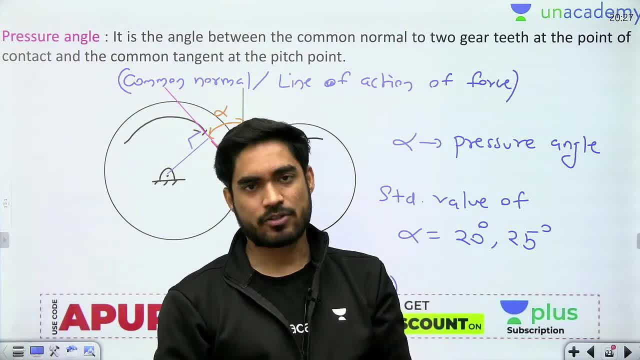 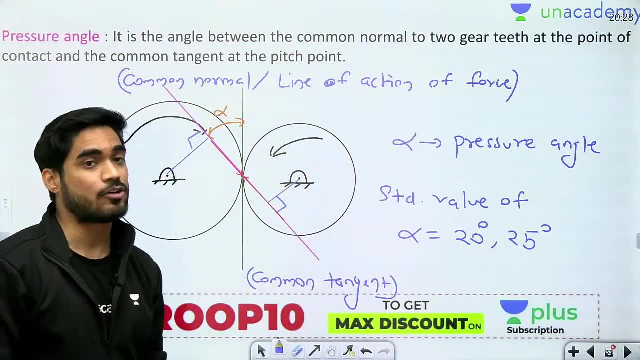 what will be the effect if I increase or decrease alpha. so you understand that. so do you understand why choosing a particular value of alpha is so important and why the standard value of alpha is so important. I hope everyone is clear about this fact. if everything is clear to you, beta. 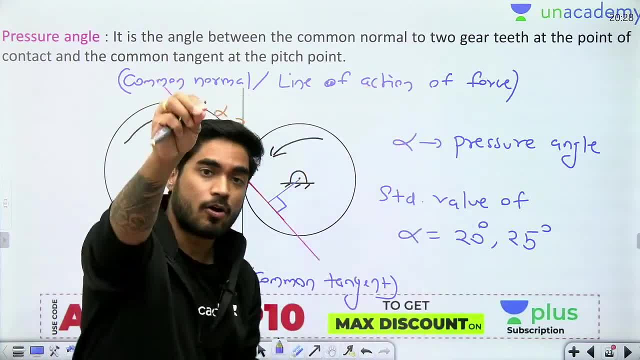 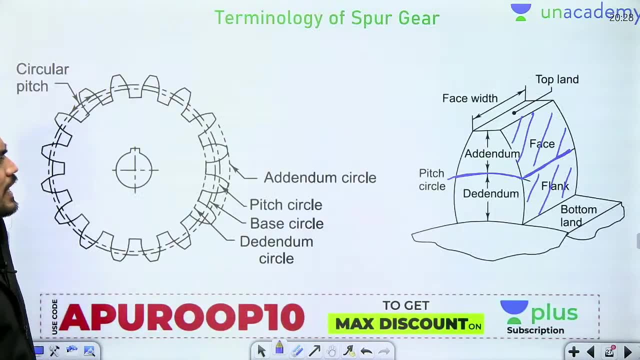 please hit the like button right now. like button. jaldise dabaa do mere bhai, or share, share, share, share kyrna na bhuley, share, kyrna na bhuley to mere bhai aanch ke lecture ke liye. itna kaafi hai gear ka. 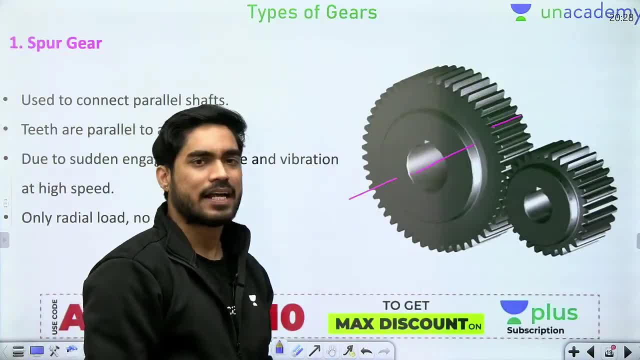 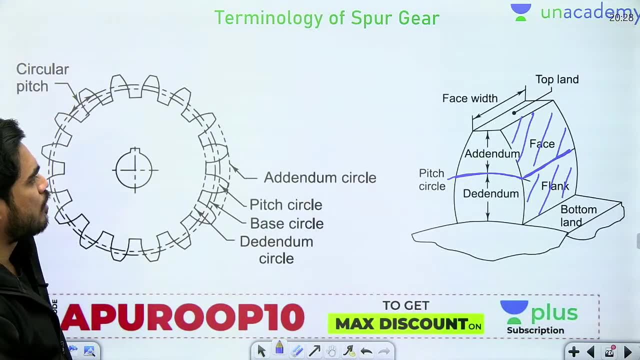 introduction: mil gaya gear kya hota? yeh dekh liya gear ke different types. characteristics of each and every type of gear is clear and beta. we have haven see the terminology of each and every gear. sorry, the The terminology of spur gear. we have seen each and every parameter. 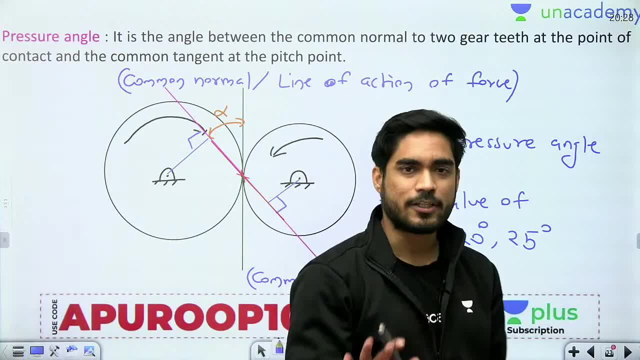 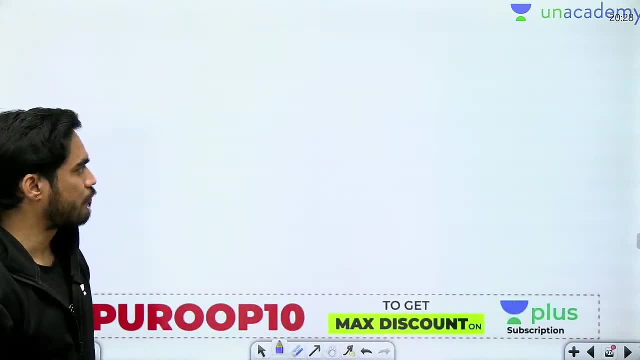 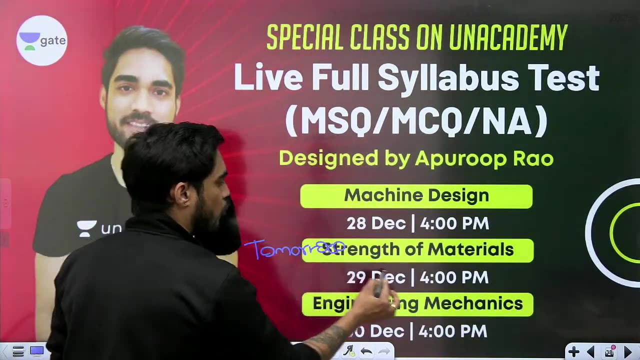 We have seen pressure angle, which is very precious. Okay, So for today this much is enough. From tomorrow we will start the design of gear. From tomorrow, we will start the design of gear, But tomorrow we have a test on strength of material at 4 pm. 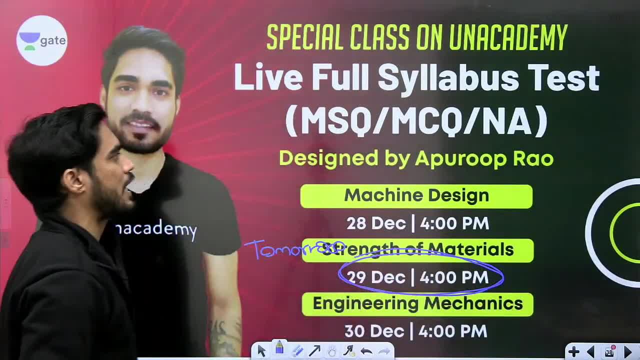 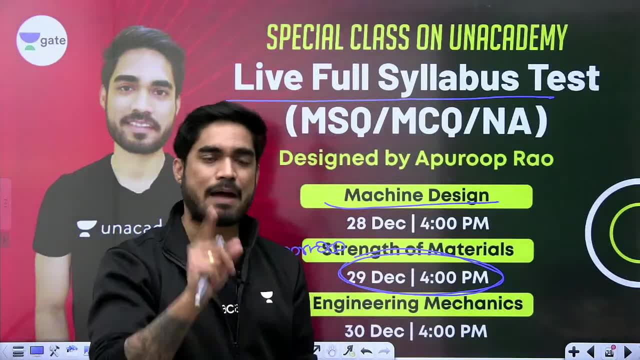 Okay, Yesterday at 4 pm there was a test on strength of material- Live full syllabus test. Today there was a test on machine design. If you have missed it, you can still watch it. You can still watch it. 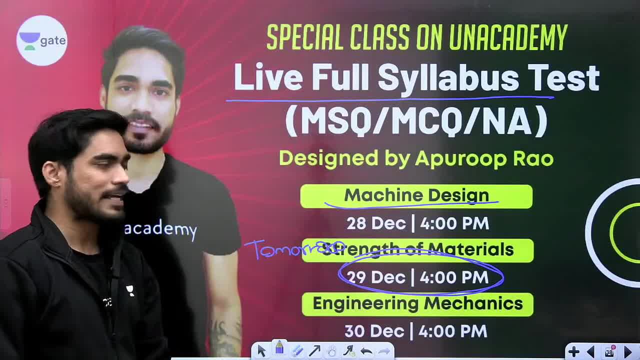 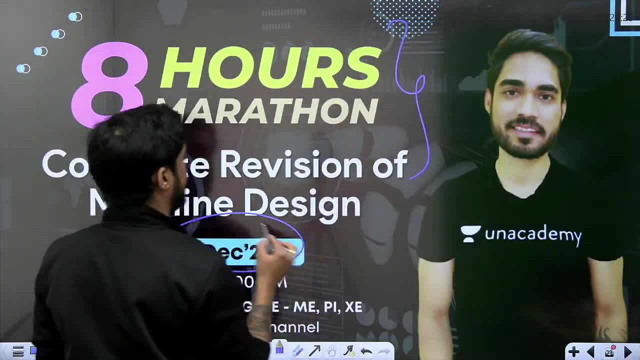 The link is there. You can still watch it. Okay, Tomorrow there is a test on strength of material And on Thursday 31st of December we have an 8-hour marathon session on complete revision of machine design. Where? 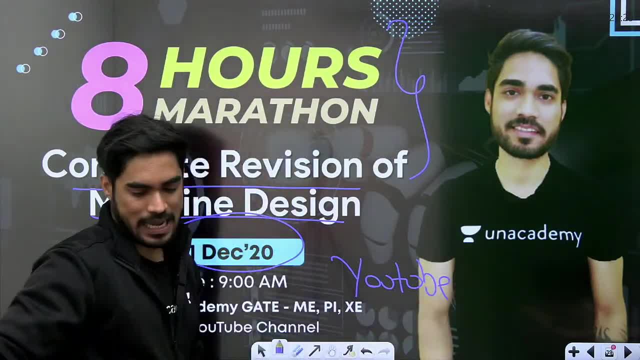 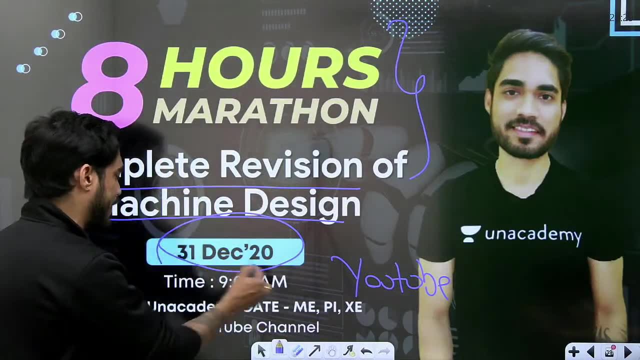 On YouTube channel. There is a continuous 8-hour class on YouTube channel. There is a continuous 8-hour class on YouTube channel, my brother. So Thursday at 9 am with me. Don't forget to revise the entire machine design. 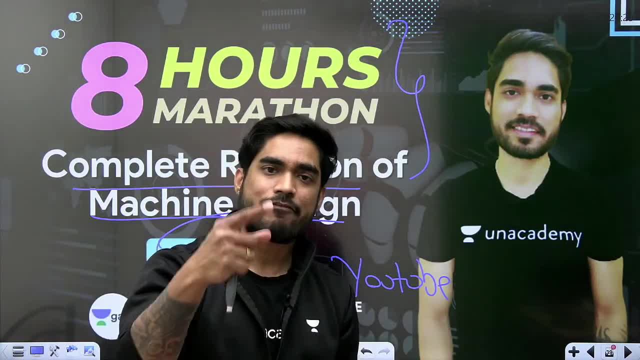 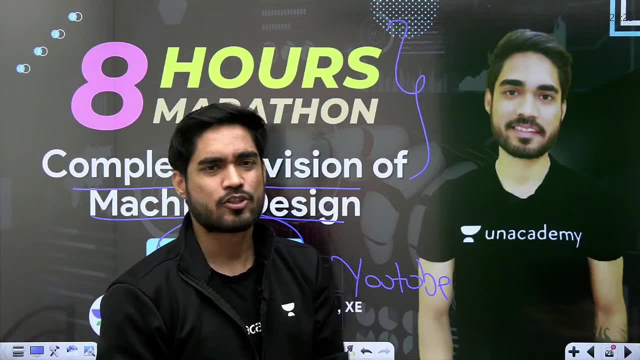 30th of December, your syllabus will end. Okay, We will have one more lecture on gear And then we will have last lecture on spring. Spring is a very small topic, So we will complete the entire syllabus on Wednesday. 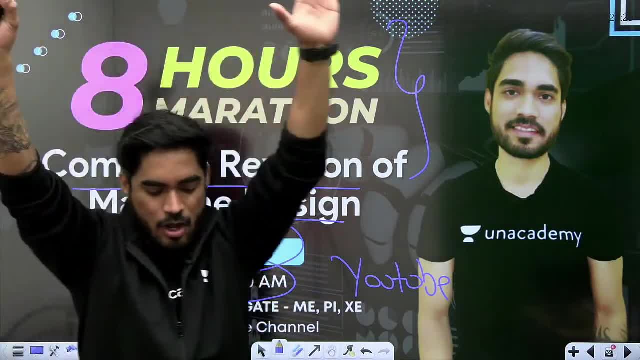 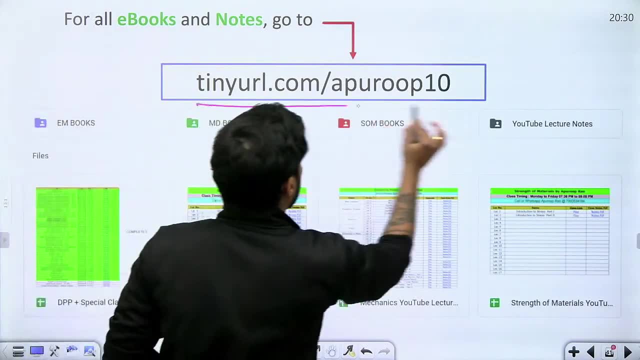 30th of December, On Thursday, we will have complete revision of machine design in one lecture. Okay, And my brother, if you want to watch all my lectures at one place, then you can use this. tinyurlcom slash approved. 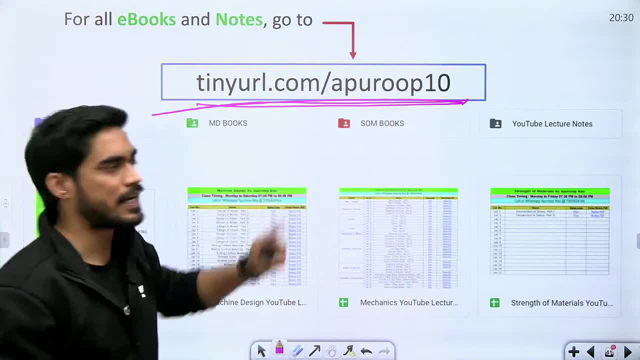 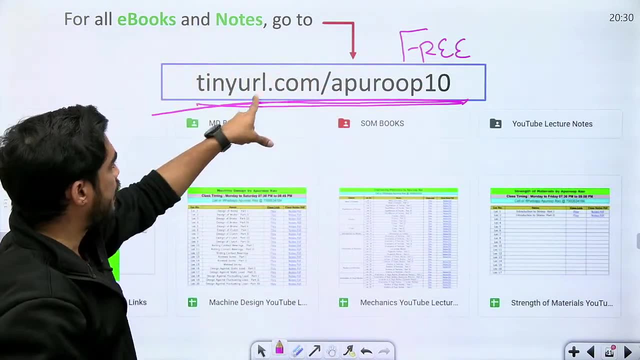 And whatever lectures I have taken till now, you can get all the lectures here completely free of cost. Okay, How to access this? Just like you, open facebookcom, youtubecom. just like that, open tinyurlcom, slash approved, And go to your web browser. 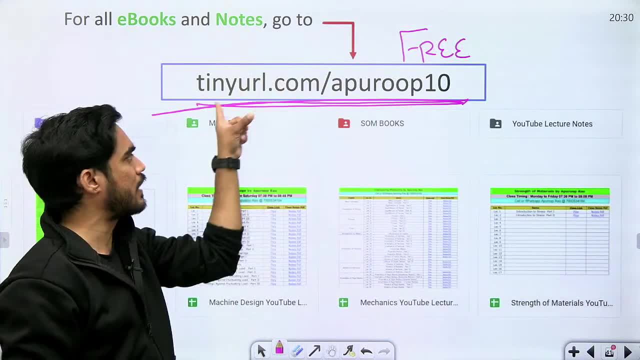 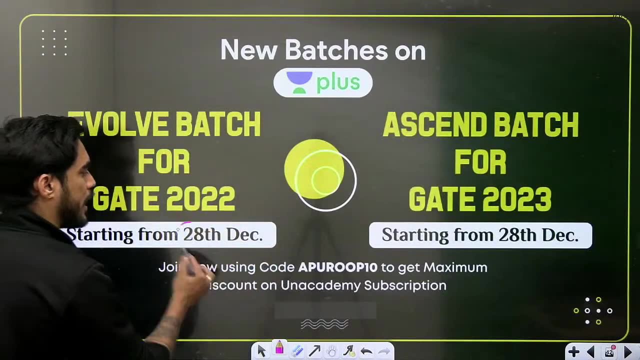 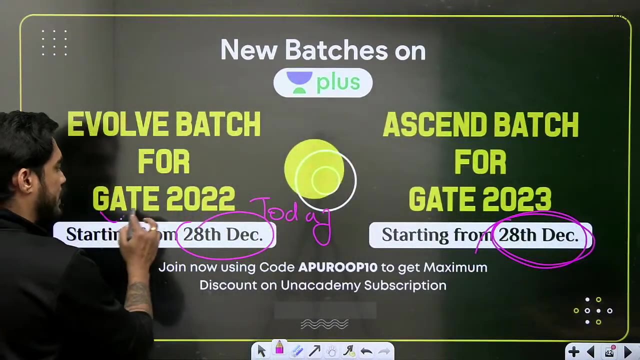 Don't search. Don't search Google. Just type in the address. Just type in the address bar: tinyurlcom. slash approved. Okay, And my brother. from today, the new batch is off. Gate has been launched And the response is very good. 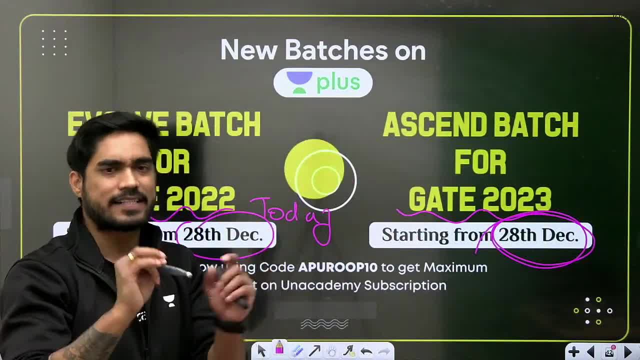 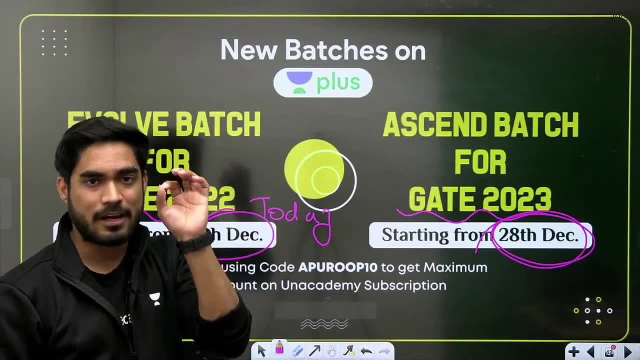 Very good. A lot of students have joined my brother, So it's a great success. So, my brother, if you don't want to miss studying with them, If you don't want to miss the lectures from legendary teachers, then join Evolve batch and Ascend batch for Gate 23.. 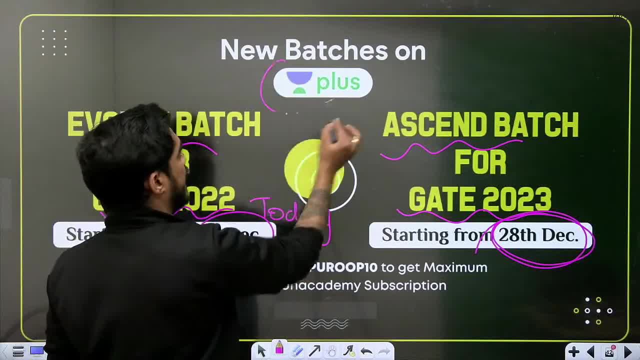 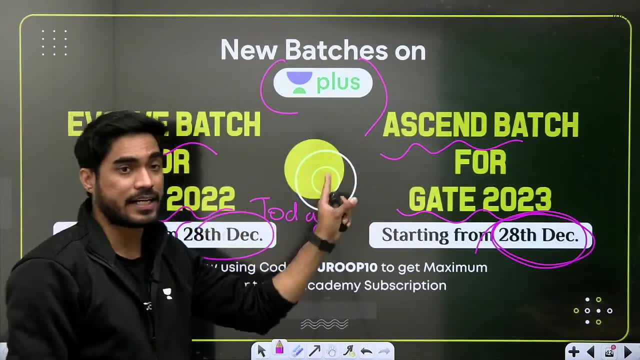 Start it today. Go to Unacademy and take Unacademy plus subscription. Go to Unacademy app and take Unacademy plus subscription. And join these batches quickly, because legendary teachers are coming to teach together for the first time in one batch. 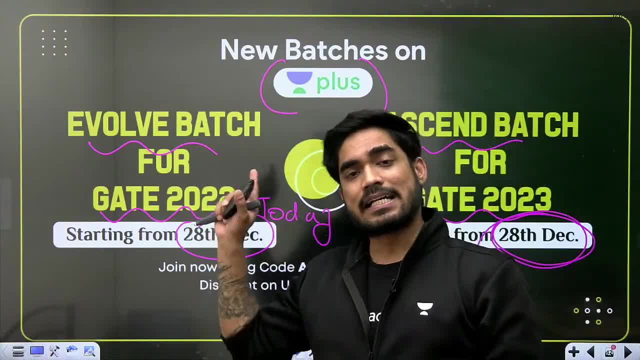 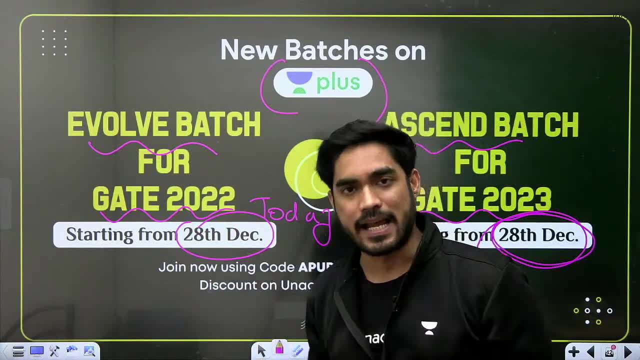 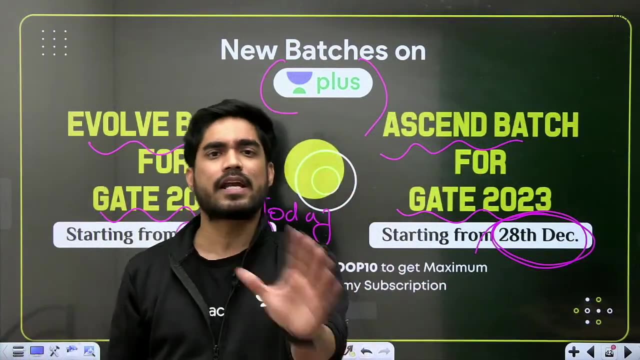 And this is the biggest opportunity that you are going to get. If you miss this, then, my brother, you will do a big loss, And if no one gets ranked after attending this, then it will be his own mistake Because, son, you cannot get a better opportunity, better guidance, better platform than this to start preparation for Gate. 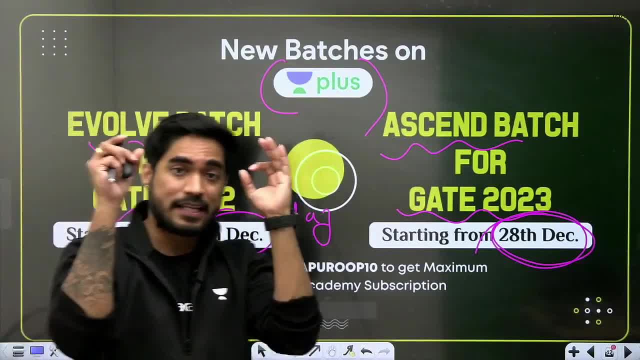 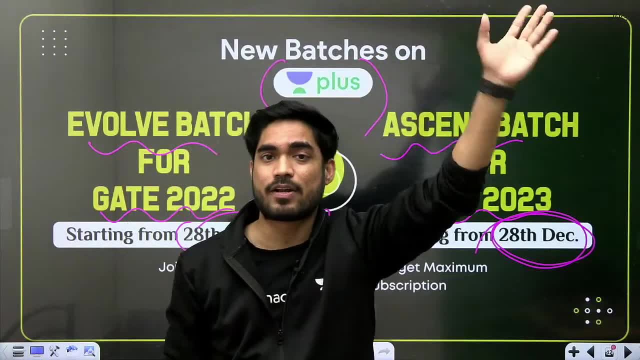 The best of the best teachers in one place, in one place, In one single batch, and that, too, online. So, my son, you don't have to go anywhere, You don't need to go to those states and study, You don't need to spend lakhs of rupees. 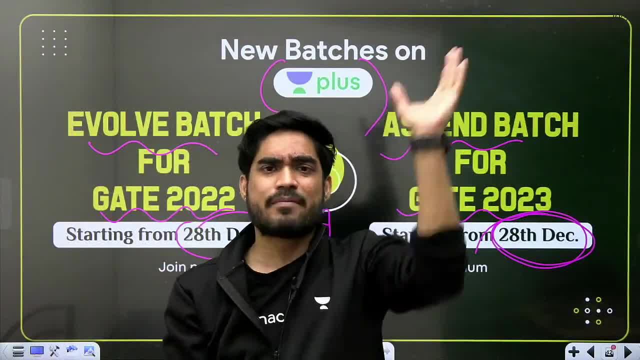 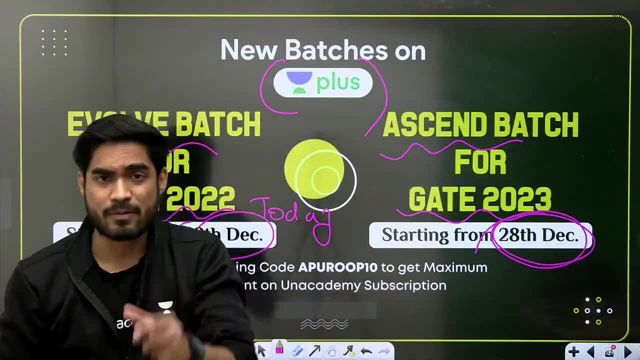 Sitting at home, all those lecturers who used to give lakhs of rupees in Delhi and Hyderabad and teach you. they are coming on one platform today, And that, too, at such an affordable price. Such an affordable price that you won't believe it. 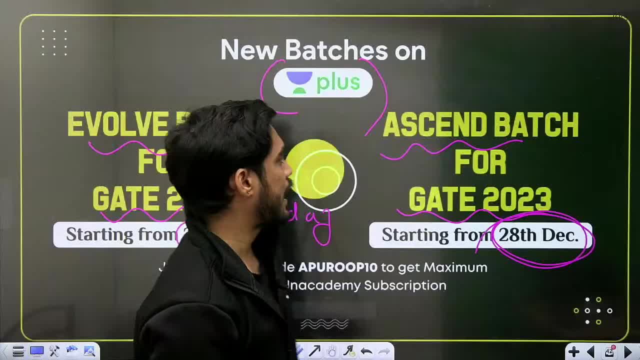 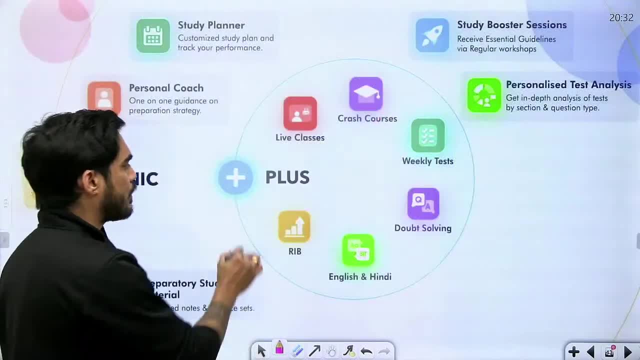 Only 54 rupees per day. 54 rupees per day And you can watch the lectures of these legendary teachers. 54 rupees per day. I will show you how. So my son Unacademy plus platform will give you live classes in English as well as in Hindi. 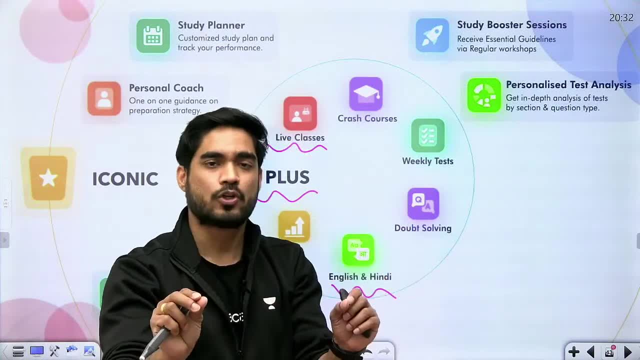 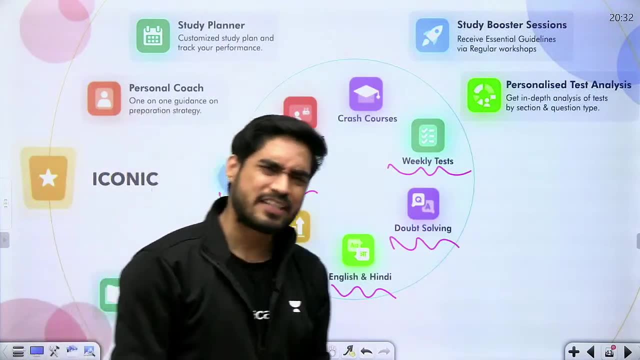 Entire lectures will be in Hindi and English separately, So you won't have to face the communication problem. Then, my son, there will be weekly tests, There will be doubt clearing sessions, So everything that people think is not possible offline in classrooms. 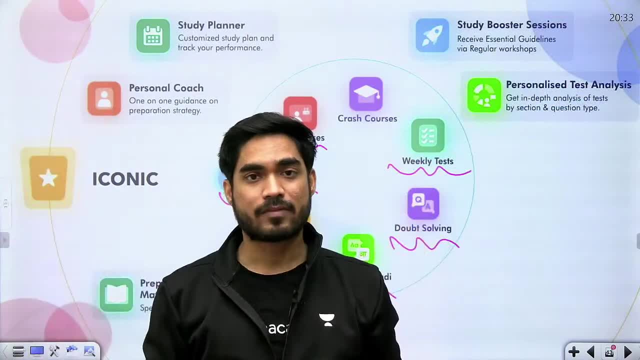 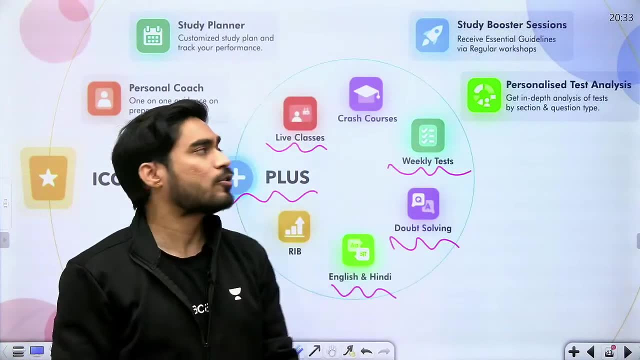 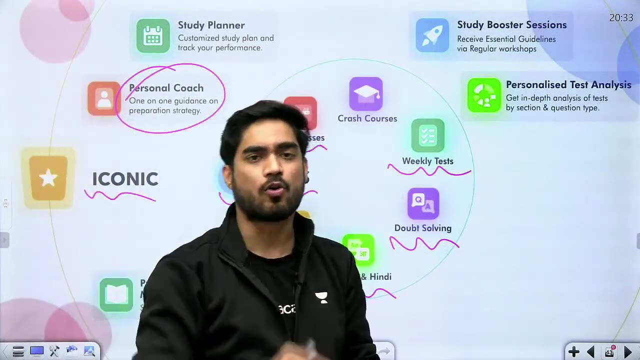 All that is possible online. my son on Unacademy And if you want to learn at a more personalized level, then you can take iconic subscription Where my son. you will have a personal coach who will push you personally towards your goal. 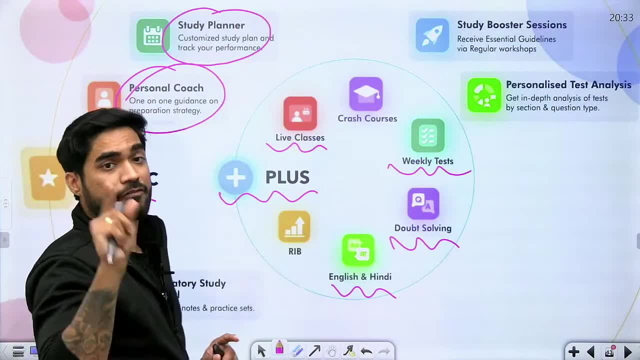 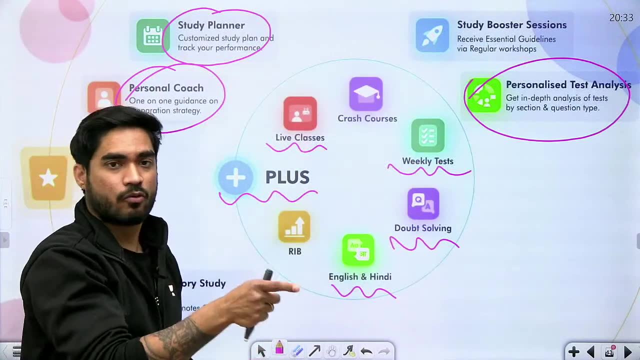 He will make the entire schedule for you and he will make sure that you are following that schedule. He will analyze all your test scores and he will make sure that you will improve wherever you are lacking. He will prepare entire study material for you. You don't have to worry about anything. 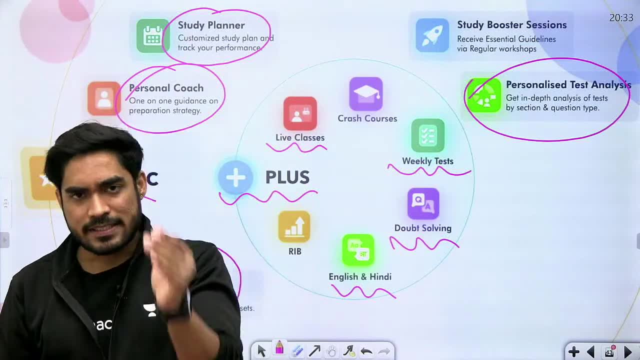 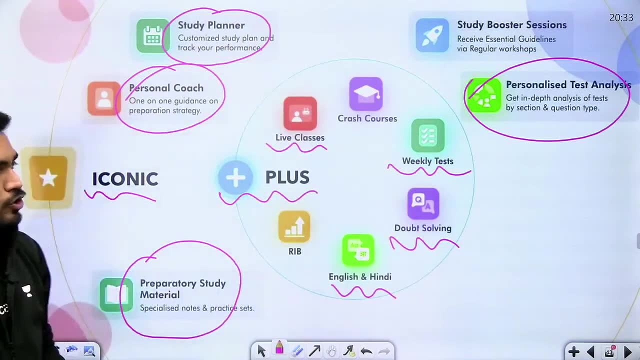 So you get a personal level of push. That means there is a person who will constantly follow you to see whether you are going in the right direction or not, Whether you are not making any mistake. So, my son, what will be the advantages of this platform? 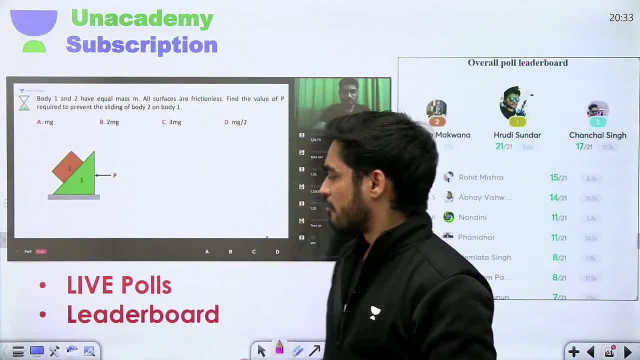 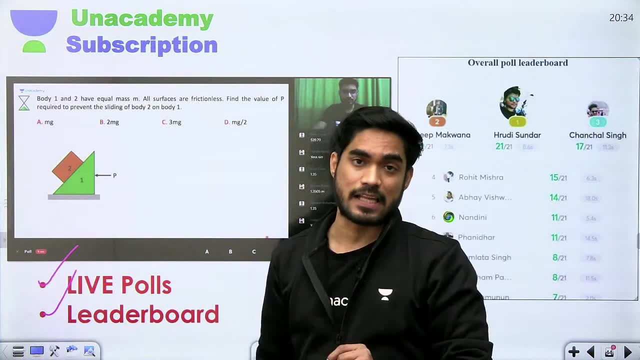 So there are a lot of features which are there on Unacademy plus platform Which you will not find anywhere else, And this will really help you in improving yourself. My son, 40 to 50 marks come easily, But above 50 marks 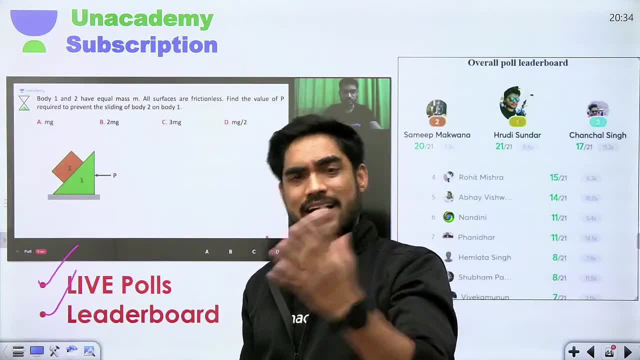 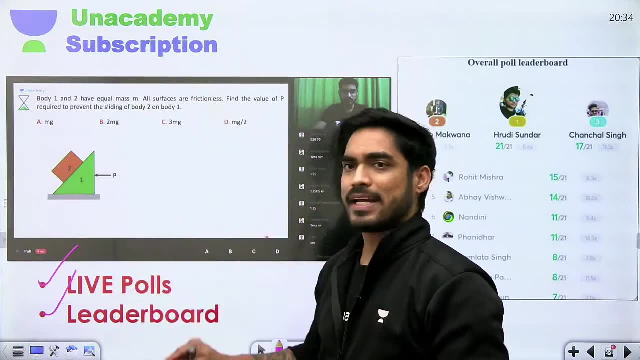 You have to fight for each mark, You have to struggle a lot for each mark. So, my brother, with these small things, each mark improves. So what is there in Life Polling Leaderboard? We do polling of your objective questions. 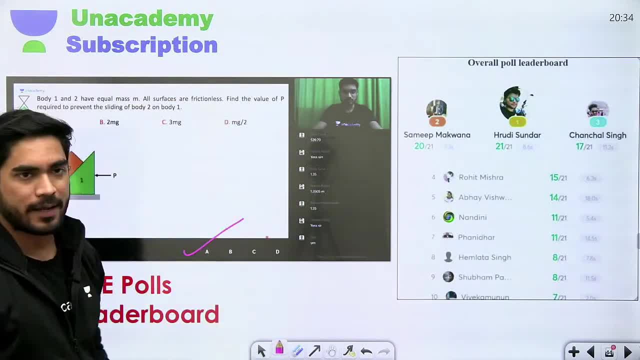 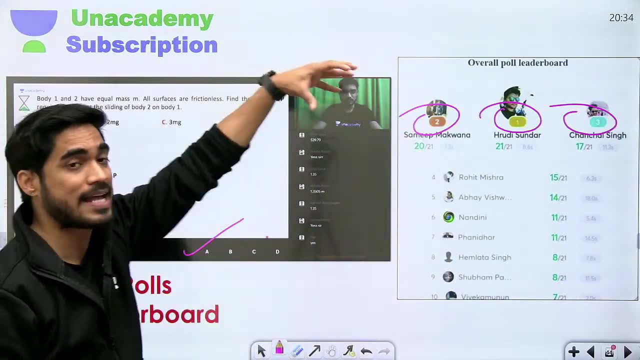 In which, if you give one answer from A, B, C, D, So your scoreboard will be ready, in which you will get to know your ranking After every question. you will get to know your ranking Where you are standing. 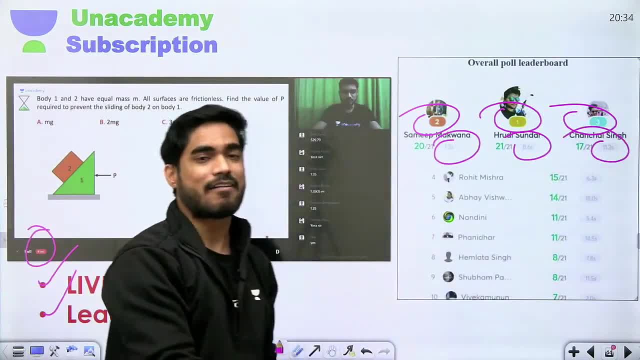 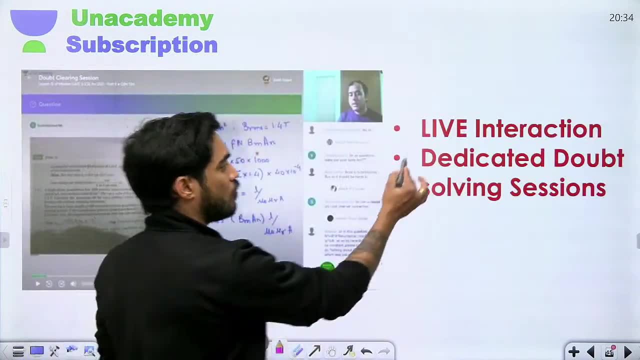 You will get to know your timing In what time you answered. So with this your time management skill will also improve And your answer giving skills will also improve. There will be live interaction in the class, Meaning you will feel that you are sitting in front of the teacher. 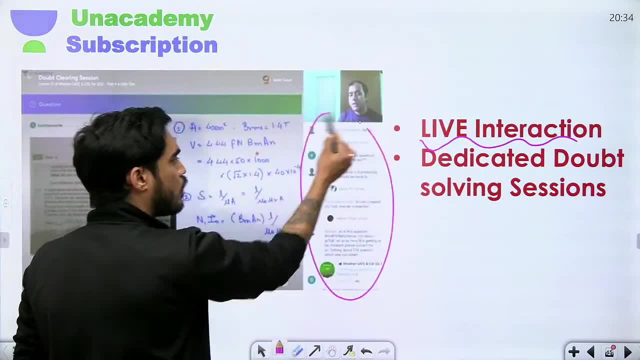 The comment section of this is so interactive That you will feel that you are talking to the teacher And you can send all your doubts to the teacher in the form of an image. You will not even need to write, You can send the image directly to the teacher. 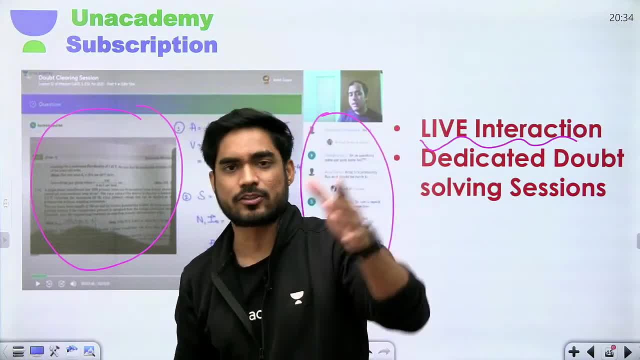 So that the teacher can solve the whole question by looking at the image. And my son, you will get a dedicated doubt solving session, Meaning you will not have to think about this. You will not have to think about this. You will not have to think about this. 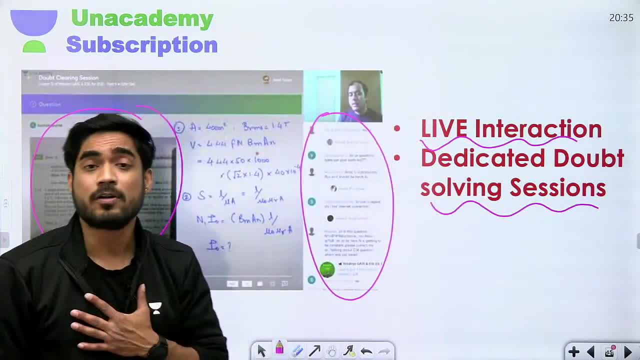 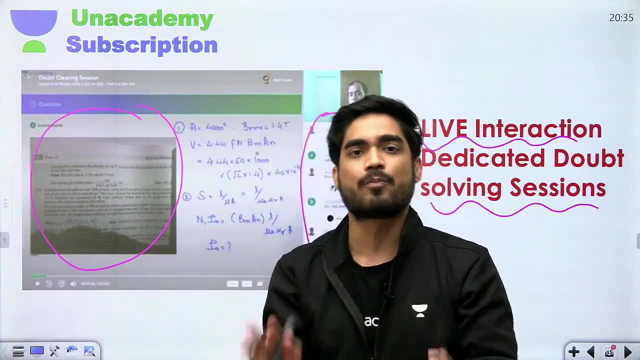 That if my doubt is solved, If the teacher leaves the class, then it will not be like this: Every fourth class will be for doubt. only Every fourth class will be for doubt. only That means you can ask all the doubts. That means you can ask all the doubts. 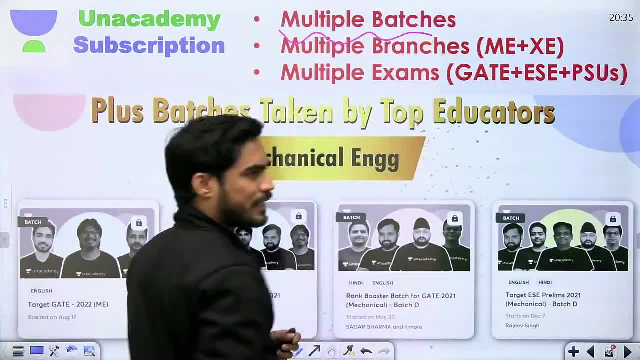 And my brother here, multiple batches will be applied. And my brother here, multiple batches will be applied. That means not only one batch is being made. So many batches are being made That you can study according to your choice. 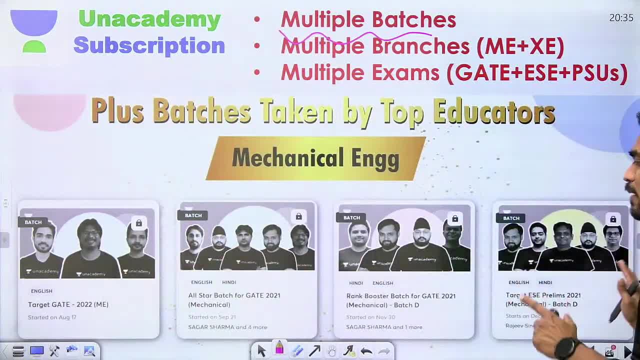 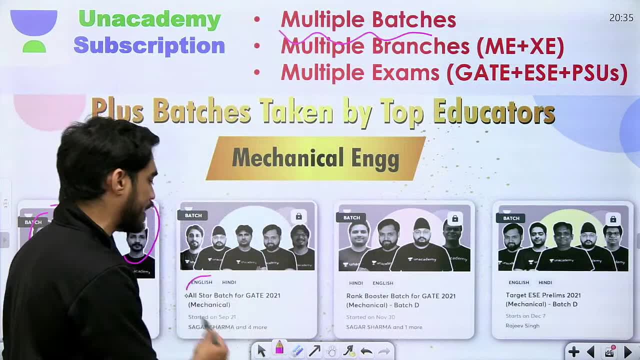 That you can study according to your choice. I am showing some batches of top educators here. You can see my batch with Negi sir. We started with Pallav sir. We started with GATE 22 batch, Then GATE 21 batch. 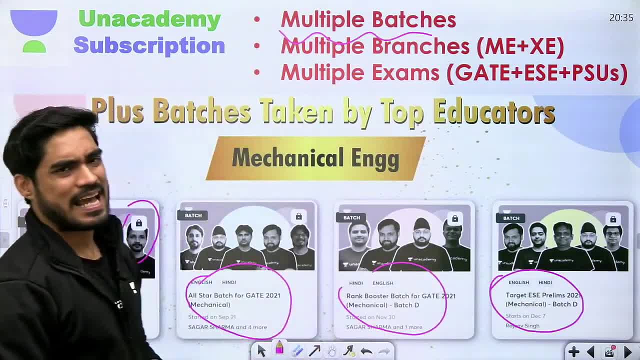 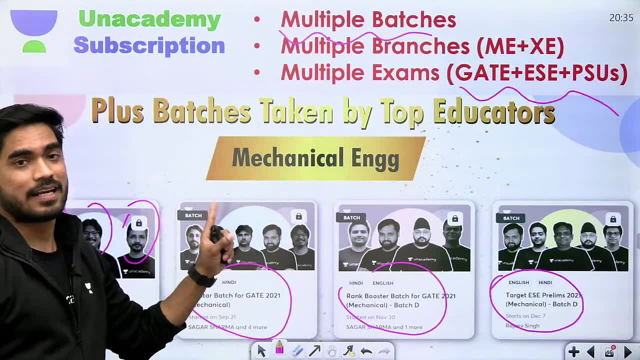 Then Rank Booster batch, Then Target ESC batch. There are so many batches You can study according to your choice. And it has happened for the first time in 17-18 years. And it has happened for the first time in 17-18 years. 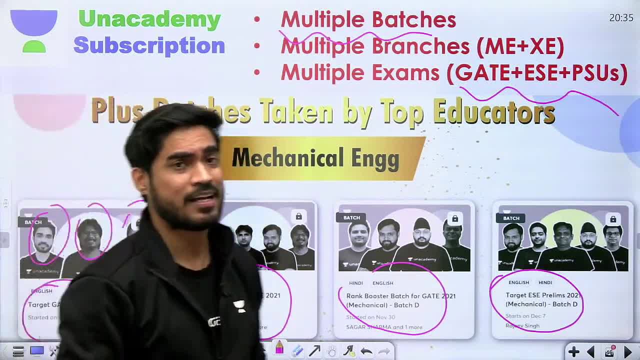 So my brother Unacademy has brought that revolution in education field. So my brother Unacademy has brought that revolution in education field. Children were waiting for years. Children were waiting for years. They used to think that we should have the power in our hands. 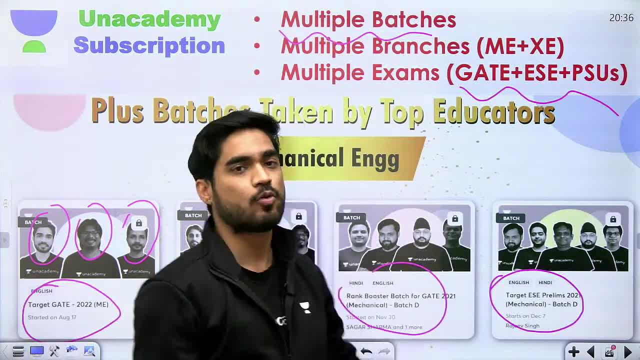 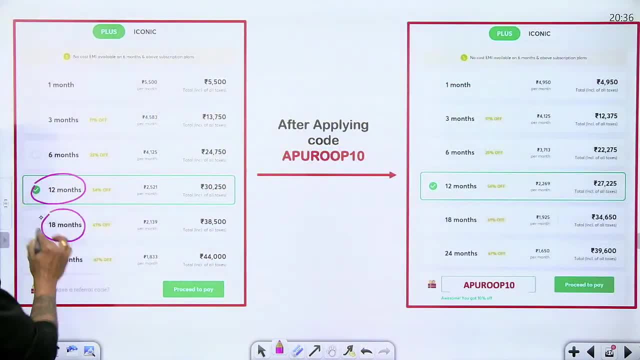 They used to think that we should have the power in our hands. So this is possible with Unacademy. So to take full advantage of this, take one year, one and a half year or two year subscription plan, If you compare per month cost of small plans and big plans. 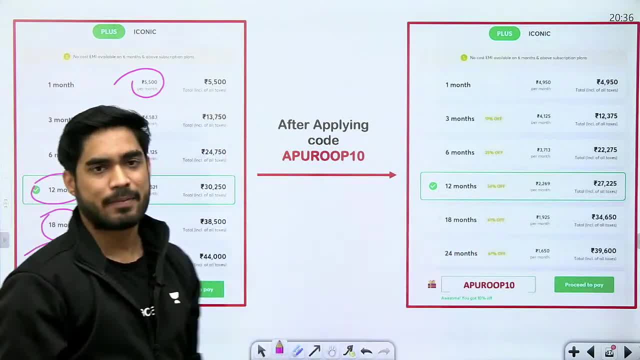 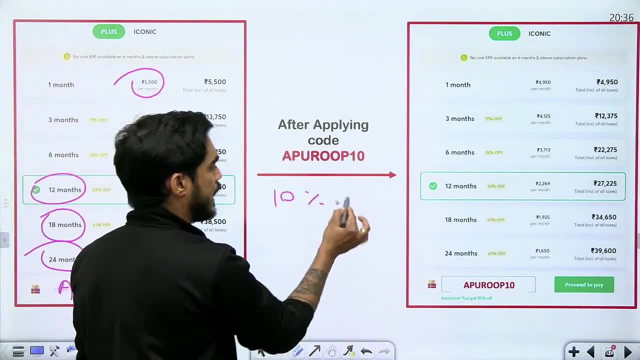 then of course you will understand that big plans are more beneficial. And if you have a referral code- APPROVETEN- then you will also get 10% off. You can see by comparing how much difference it will make in cost And if you are using APPROVETEN. 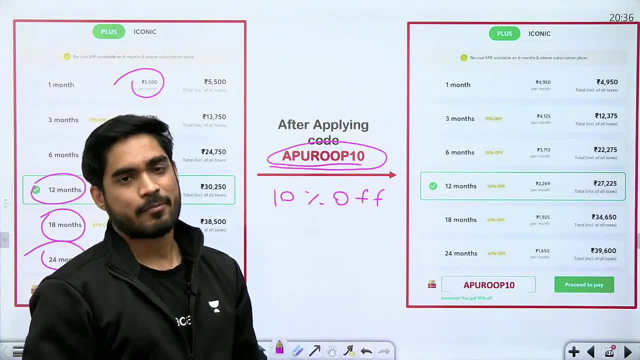 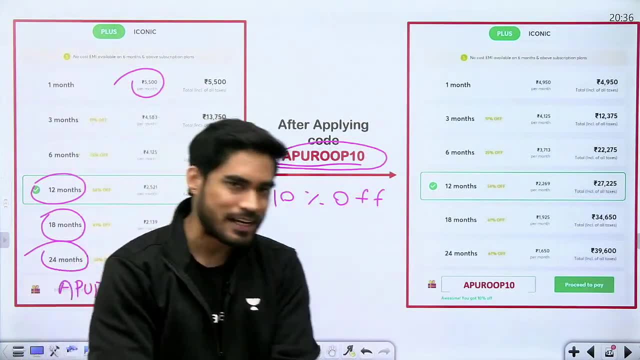 whenever you will use it, then I will also get a notification Means I will feel that you have shown your trust in me. And if you will show your trust in me, then why will I let down? I will never let down my friends. 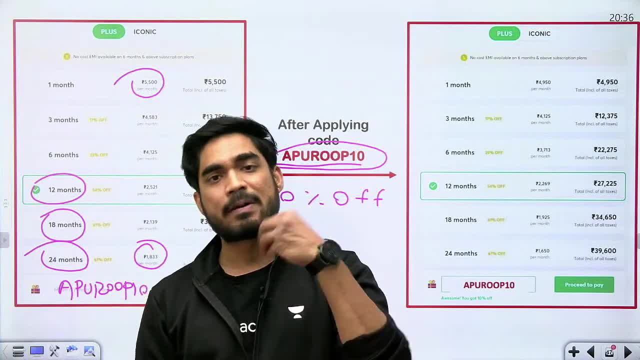 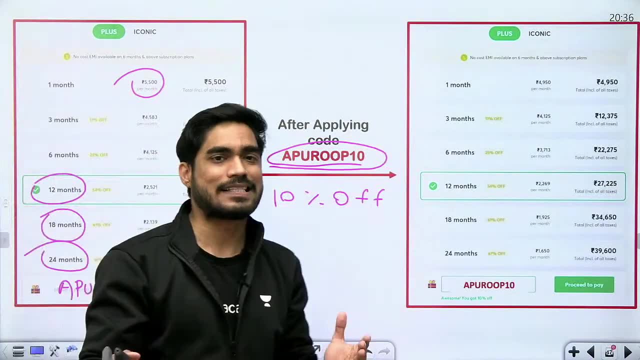 I will never let down those students who are believing in me. If someone joins by trusting me, then I will never disappoint him. I will support him in full preparation. Anyway, I support everyone, But if you are going by using the code, 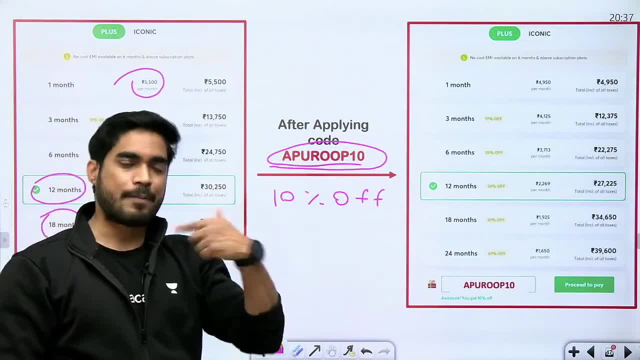 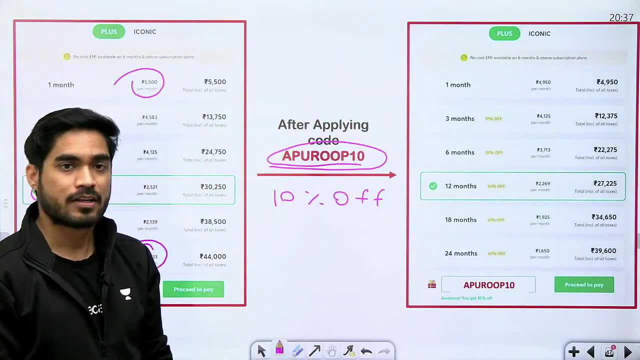 means you are telling that you have come through me. then if you have come through me, then you are my responsibility. I will guide you, I will mentor you and I will make sure that you achieve your goal. And the fees if you want to give it in EMI. 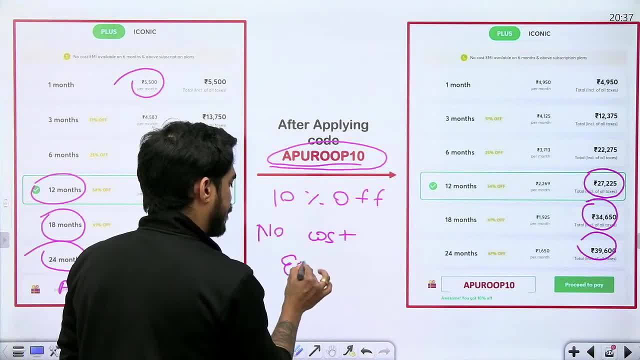 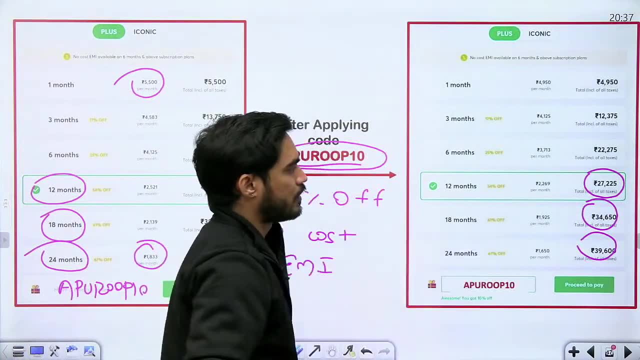 then you can also give it in EMI. EMI is no cost Means. you can pay this fee in monthly installment without paying any additional fee. And pay attention here: if you divide this per month cost by 30, then this will be roughly. 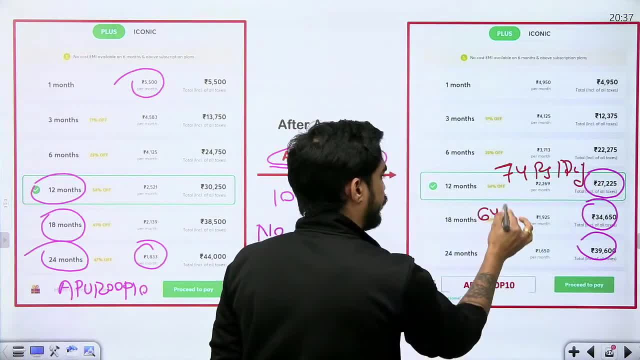 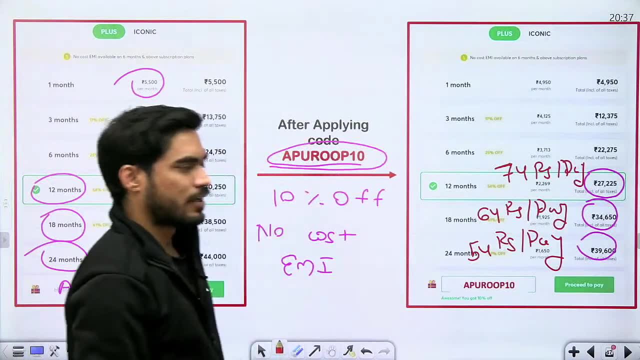 ₹74 per day. This will be ₹64 per day And this will be ₹54 per day- Means in 50 rupees per day. you can sit with legendary teachers and study for hours In this 50 rupees per day. 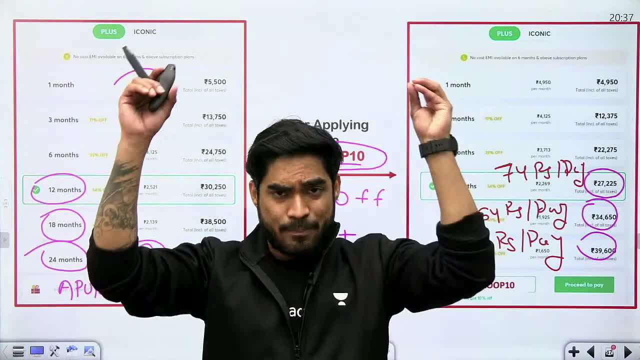 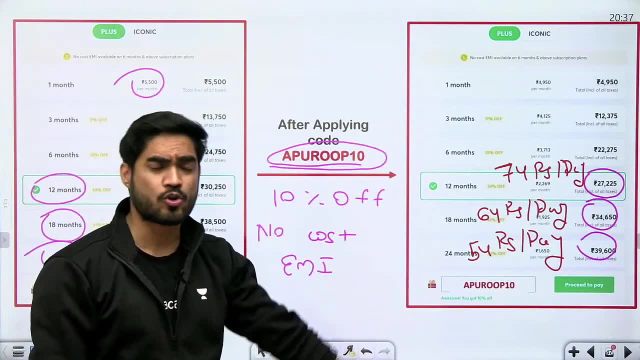 you can attend so many lectures that there is no limit. You can solve so many practice problems that there is no limit. You can solve so many doubts that there is no limit. So dear, only 50 rupees per day, which people throw in the data.